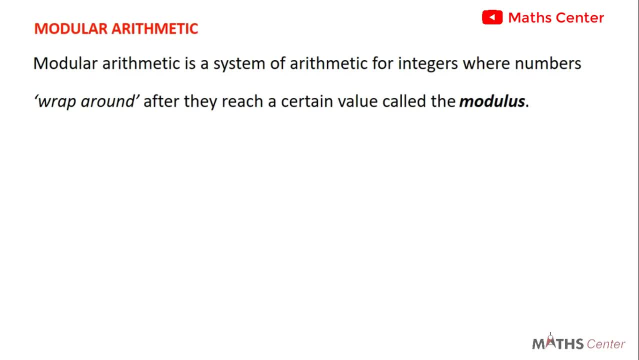 What does this statement mean? To help us understand it, let's consider this simple circular surface that is numbered from 0 to 3.. We want to move around the circular surface in a clockwise direction. We will begin at the 0 mark, So, before we start moving, our arrow points to the 0 mark. We are moving. 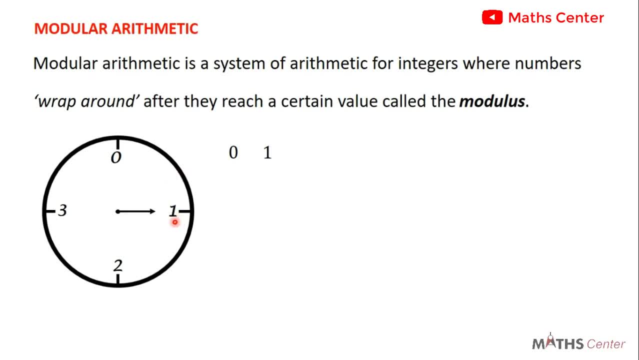 in a clockwise direction. so we move from 0 to 1, from 1 to 2, from 2 to 3, then from 3 we will move back to 0., 2,, 2 to 3, then we move back to 0, from 0 to 1,, 1 to 2,, 2 to 3, and the process continues. 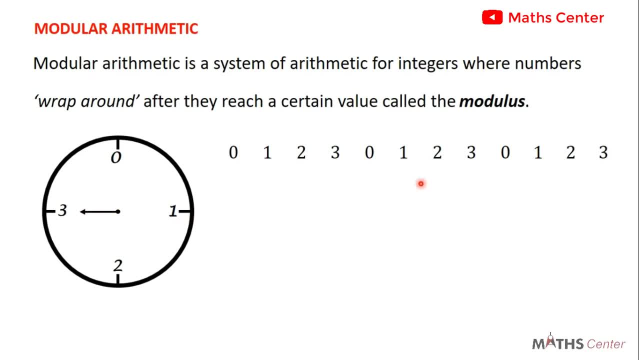 on and on. Now let's consider this set of numbers very carefully. If we look at it closely, we can see that something interesting is happening here. We move from 0 to 1, 1 to 2,, 2 to 3.. 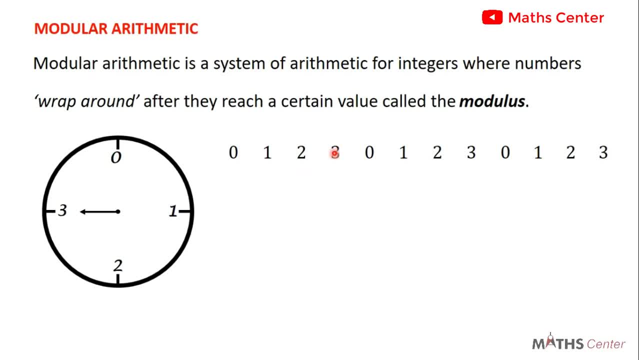 We know that if we continue in this manner, then we should move from 3 to 4.. But look at something: when we get to the number 4, the numbers will wrap around or they will end, and then we begin the whole process all over again. 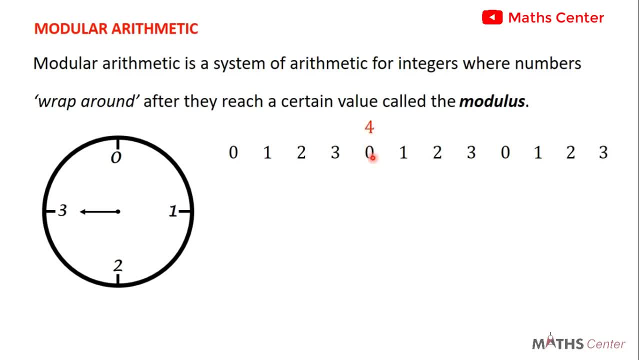 So when we get to the number 4, the numbers wrap around or they end. then we begin counting from 0 all over again. So when we get to 4, we will have 0, then 1,, 2,, 3.. 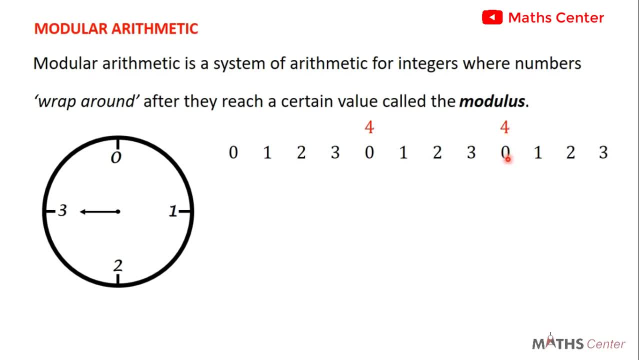 When we get to 4, again the numbers wrap around or they end. then we begin counting all over again. So when we get to 4, we write 0,, then 1,, 2,, 3, and the process will continue on and on. 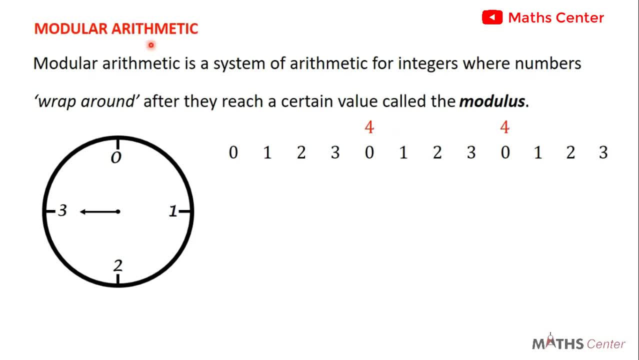 This system of writing numbers is what is known as Modular Arithmetic, A system where numbers wrap around after they reach a certain value called the modulus. So we can see from here that After we reach the number 4, the numbers will wrap around or they will end. then we begin. 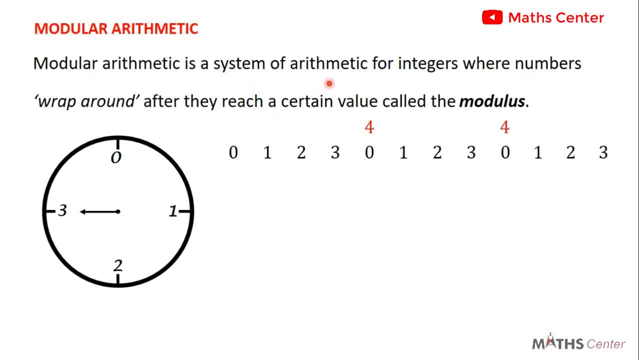 the whole process all over again. The point is that Modular Arithmetic is a system for integers where numbers wrap around after they reach a certain value called the modulus. In this example, when we reach the number 4, the numbers will wrap around. so it means: 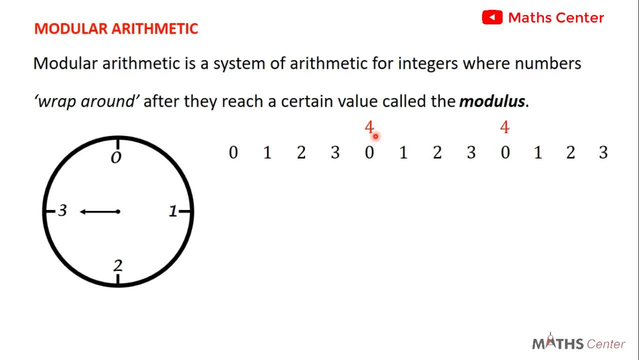 that in this case 1,, 2, 3.. The modulus is the number 4.. So in our example here the modulus is 4, or, as is commonly said, these numbers are in mod 4.. Let's consider another example. 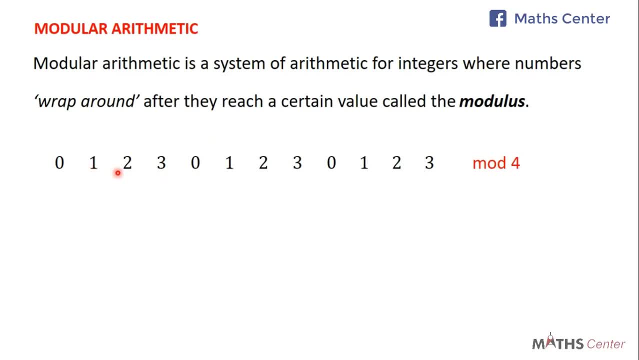 We have seen that these numbers are in mod 4.. So we have 0, 1, 2, 3,, 0, 1, 2, 3, 0, 1, 2, 3, and the order will continue on and on. 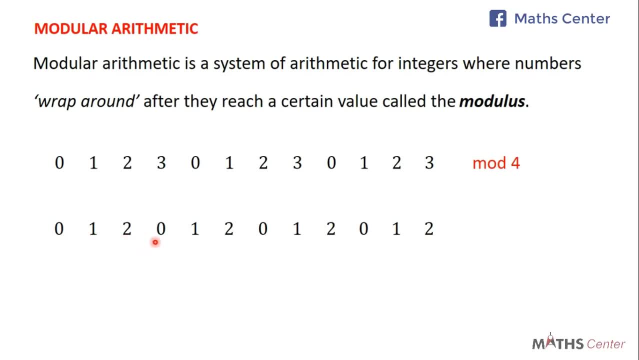 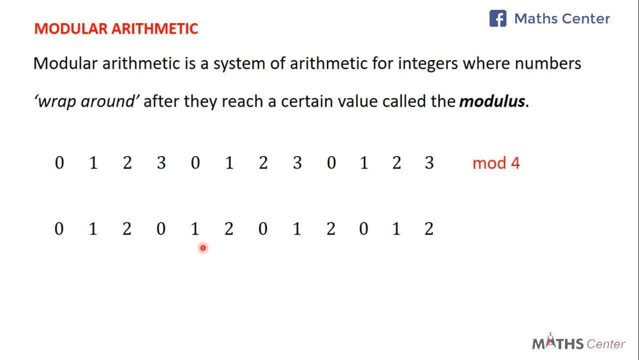 If you look at this one also very carefully, we can see that after we get to the number 3, the numbers will wrap around or they will end and the whole process begins all over again. So we have 0,, 1,, 2.. 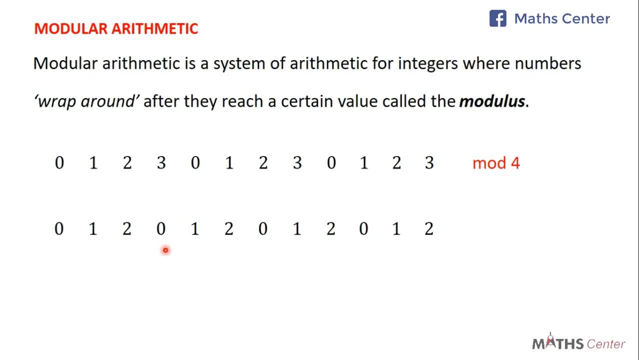 But when we get to the number 3, we will end and begin all over again. So we have 0, 1, 2.. When we get to 3, we will end and begin all over again. So we have 0, 1, 2.. 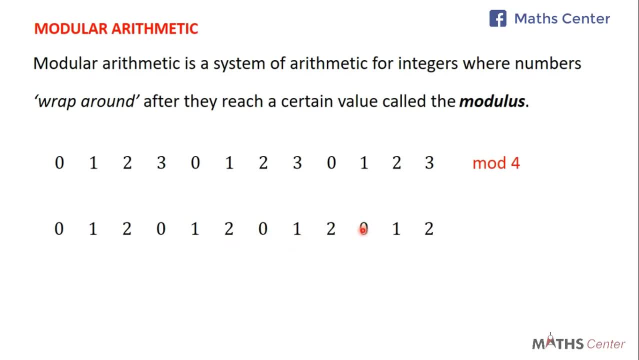 When we get to 3, we have 0,, 1,, 2.. So in this set of numbers the mode loss is 3, because when we get to the number 3, the numbers will wrap around or they will end, and then we begin counting again. 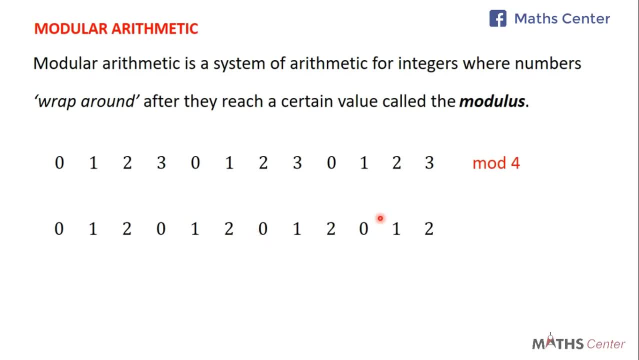 So the mode loss is 3, or we say that these numbers are in mode 3.. So the mode loss here is 3.. Let's consider another one. We have 0,, 1,, 2,, 3,, 4.. 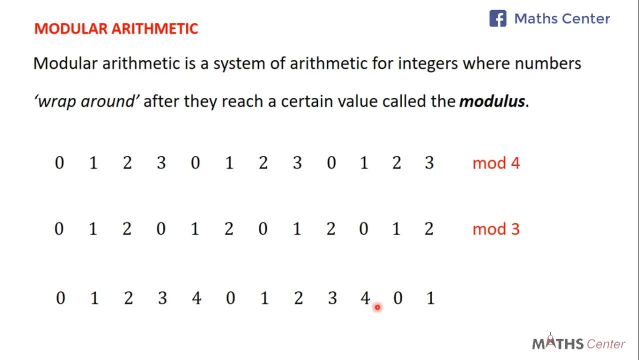 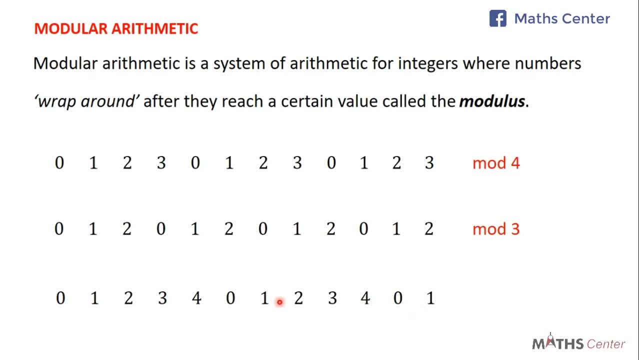 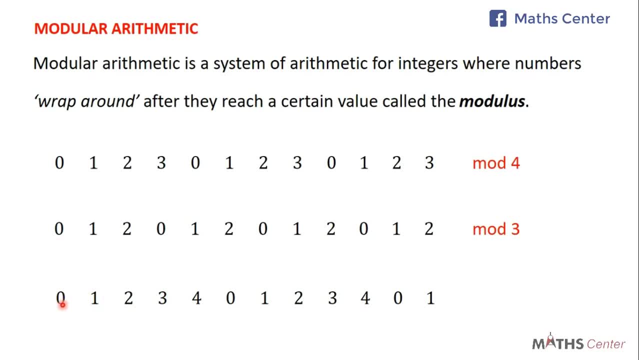 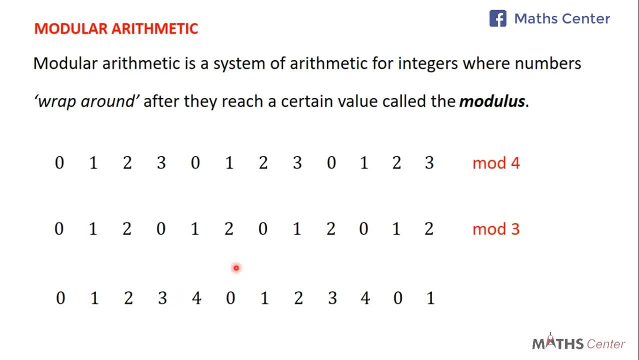 2 to 3,, 3 to 4.. But when we get to the number 5, the numbers will wrap around or they will end. then we begin counting all over again. these numbers are in mode five. so modular arithmetic is very simple. it is a system for. 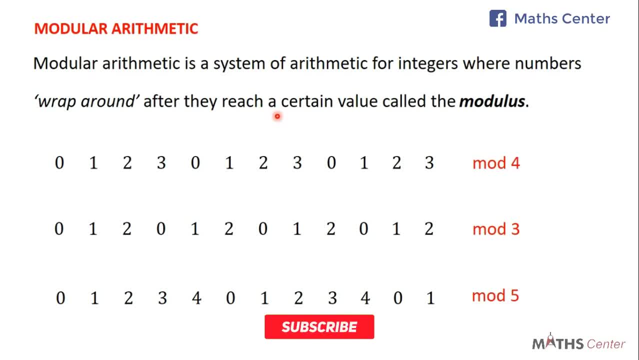 integers where the numbers will wrap around after they reach a certain value, and that value is called the modulus. in the first set we can see that after we reach the number four the numbers will wrap around. so we say that these numbers are in mode four or the modulus is four. in the 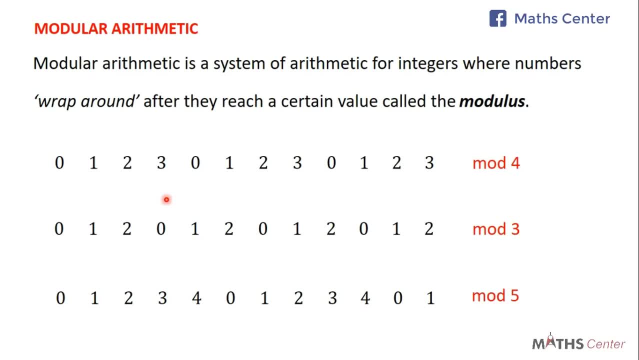 second set: after we reach the number three, the numbers will wrap around. so we say that these numbers are in mode three or the mode loss is three. and in the third set the numbers wrap around after we reach five. so the modulus is five or we say that these numbers are in. 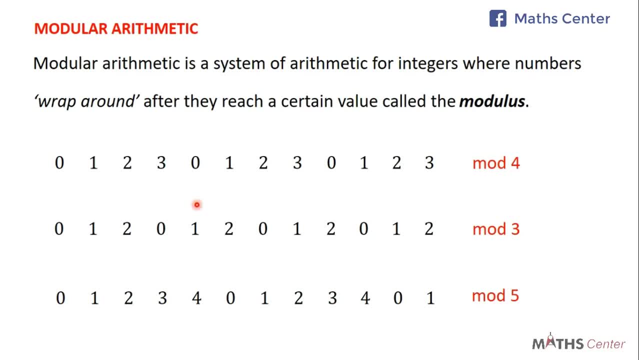 mood five. let's consider another thing. if you look at these numbers very carefully, we can see that in mode four, the set of numbers used are 0, 1, 2, 3.. In mode 3, the set of numbers used are 0, 1, 2.. In mode 5, the set of numbers 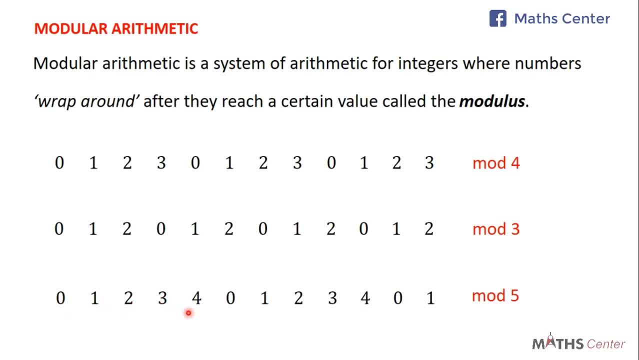 used are 0,, 1,, 2,, 3,, 4.. So if we follow in this same order, then it means that in mode 6, the set of numbers used will be 0,, 1,, 2,, 3,, 4, 5.. In mode 7, the set of numbers will be from 0 to 6.. In mode 8,, 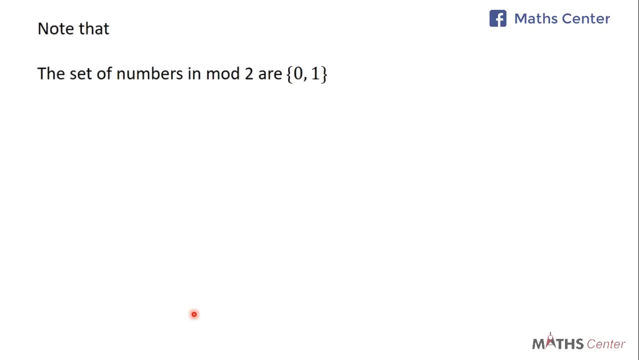 the set of numbers will be from 0 to 7.. So let's note that the set of numbers in mode 2 are 0 and 1.. The set of numbers in mode 3 are 0, 1, 2.. The set of numbers in mode 4 are 0, 1,, 2, 3.. The set of 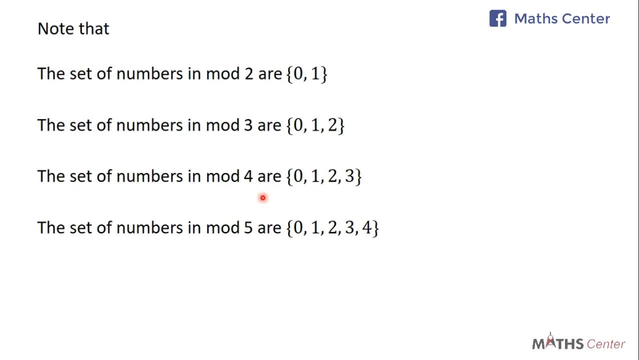 numbers in mode 5 are 0,, 1,, 2,, 3.. The set of numbers in mode 5 are 0,, 1,, 2,, 3.. The set of numbers in mode one, two, three, four, and the order continues on and on. so, in mode six, the set of numbers. 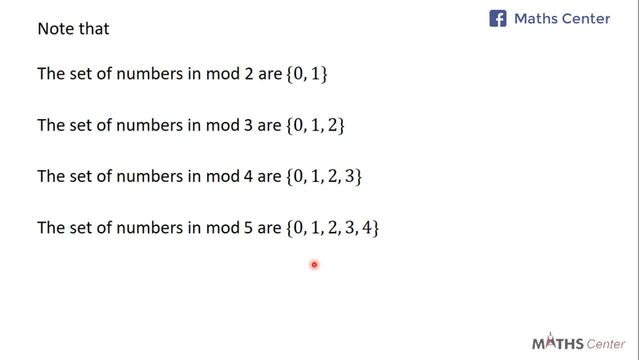 will be zero, one, two, three, four, five. in mode seven, the set of numbers will be from zero to six and so on. so we can see that in each mode we have a specific set of numbers that we can use. thank you for watching this video. subscribe to this channel for more videos. 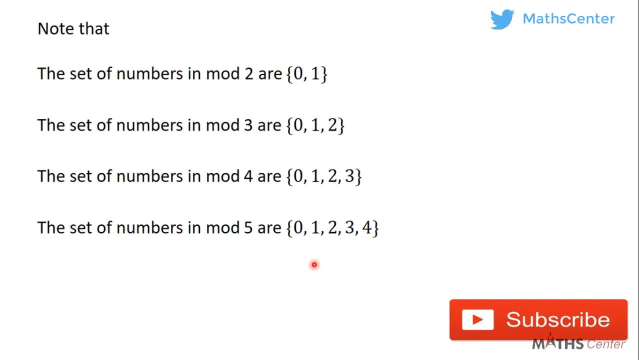 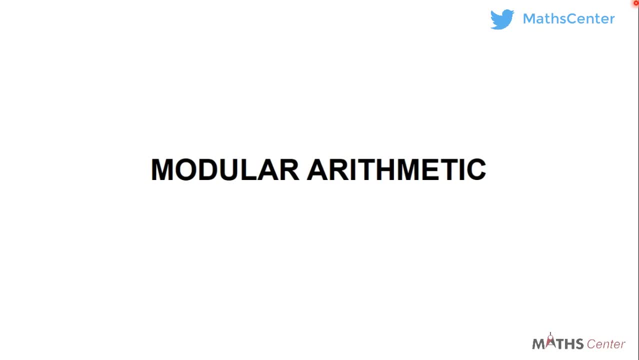 in the next video we are going to learn how to find the value of a number in a given modulus. bye, bye, welcome back. we are on the topic modular arithmetic. in the previous video we learned the definition of modular arithmetic. we also learned how to find the set of numbers used. 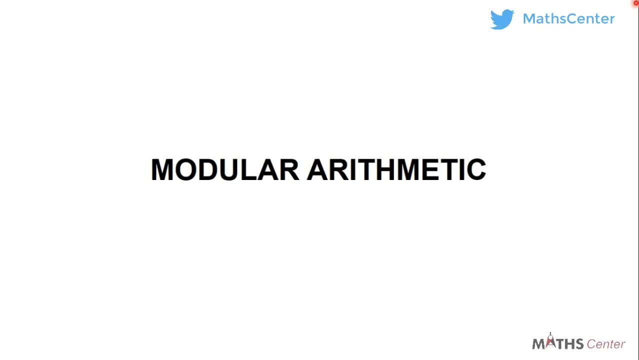 in a given modulus. in this video, we are going to learn how to find the value of a number in a given modulus. let's consider this number line. on this number line we have the set of whole numbers from zero to ten. in the previous video we learned that in any given modulus we have a set of 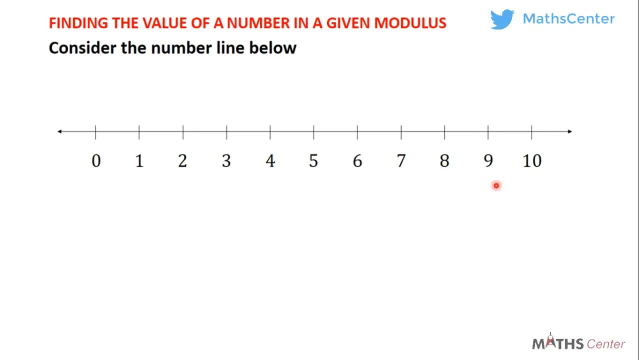 values that are used. so, for example, in mode two, the set of values used are zero and one. in mode three, the set of values used are zero, one and two. in mode four, the set of values used are zero, one, two and three. this means that the value 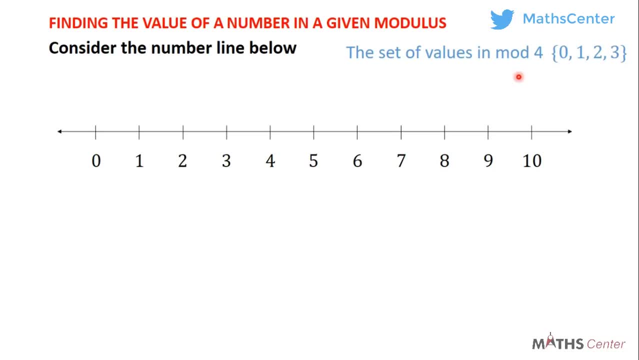 of any number in mode four will be either zero, one, two or three, because the set of values in mode four are zero, one, two and three. so the value of any number in mode four will be either zero, one, two or three. let's say that we want to find the value of any number. in mode four, we will be either zero, one, two or three. let's say that we want to find the value of any number. in mode four, we will be either zero, one, two or three. let's say that we want to find the value of any number. in mode four, we will be either zero, one, two or 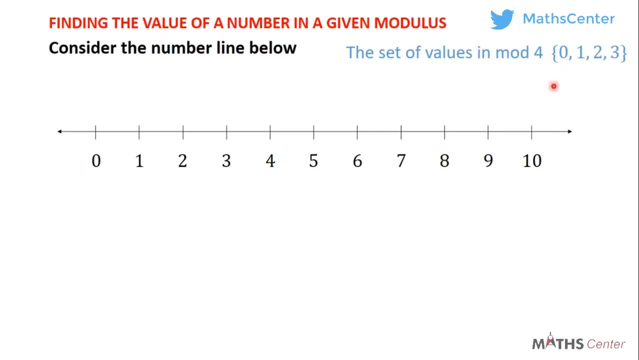 let's say that we want to find the value of 7 in mode 4.. how are we going to do that? we are going to list the set of values in mode 4 alongside the set of whole numbers that we have on our number line. then we pick the number that corresponds to 7.. now, this is what i mean. 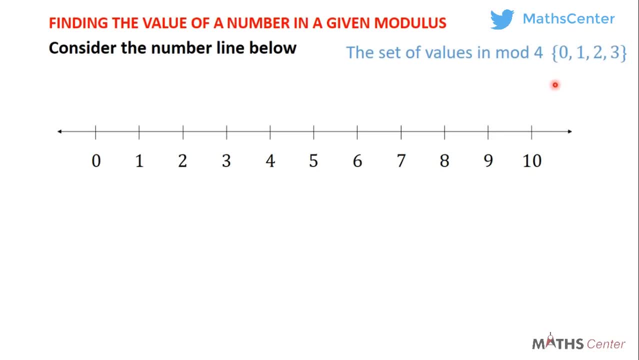 we know that in mode 4 the set of values we use are 0, 1, 2 and 3, so we will list these values alongside the set of whole numbers that we have on our number line. this is the starting point, so we are going to start from here. the first number is 0, the second 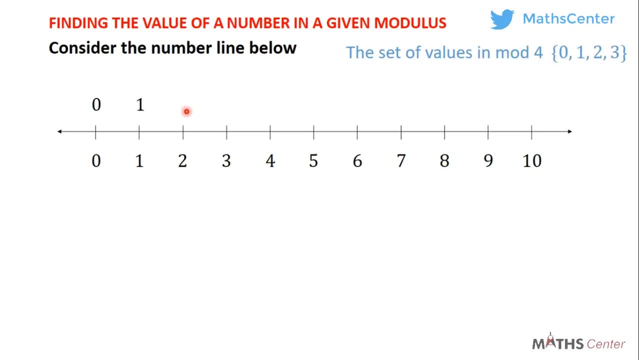 number in mode 4 is 1. the third number in mode 4 is 2. the fourth number in mode 4 is 3.. we learnt in the previous video that in mode 4, when we get to the number 4, the numbers will wrap around that. 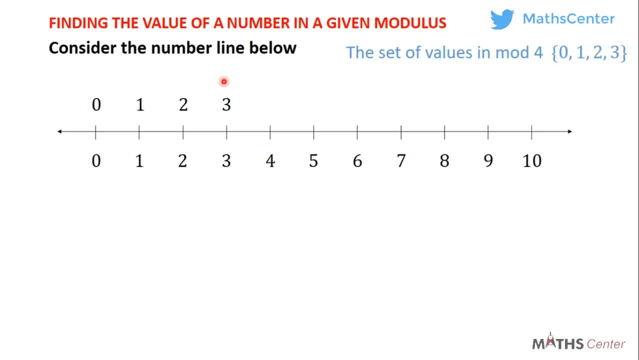 is they will end and we will begin counting from 0. so when we get to 4, the numbers will end and we will begin counting from 0. so 4 will be 0, then the next one will be 1. we have 2, 3. when we get to 4, the numbers will wrap around and we will 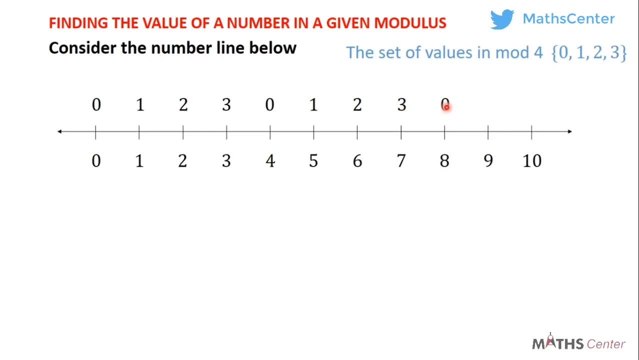 begin counting all over again. so it means that after 3 you have 0, 1 and 2. so you can see that we have written the numbers in mode 4 alongside the set of whole numbers. so on this number line the down part is the set of whole numbers and the top part is the numbers in mode 4. 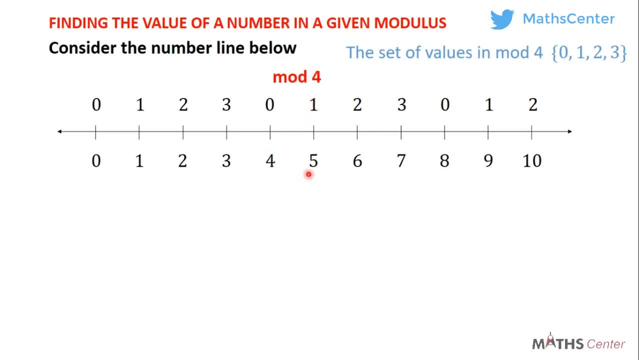 so the numbers we have here are in mode 4 and this is the set of whole numbers. we want to find the value of 7 in mode 4. the value of 7 in mode 4 is written as 7 mode 4. the value of 7 in mode 4 is written as 7 mode 4. 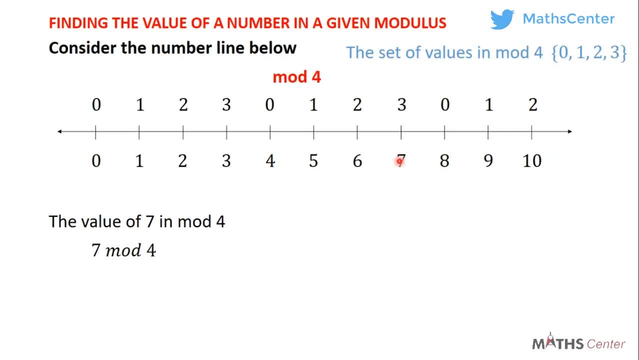 as i said previously, to find the value of 7 in mode 4 you will list the set of numbers in mode 4 alongside the set of whole numbers. then you pick the value that corresponds to 7. on this number line we can see that 7 corresponds to 3, so it means that the value of 7 in mode 4 is 3. the value of 7 in mode 4 is 3. 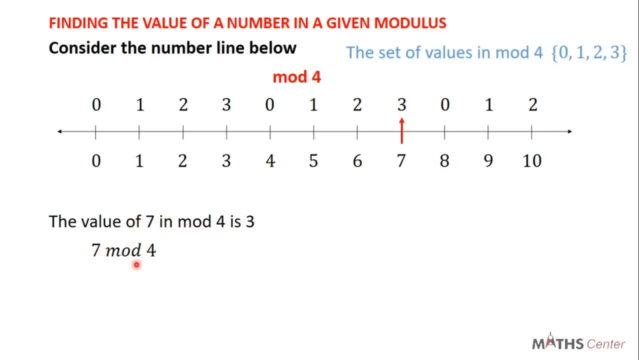 we have seen that the value of 7 in mode four is written as 7 mode 4, so it means that 7 mode 4 is equal to 3. here is another example. we want to find the value of 2 in mode 4. 2 in mode 4 is written as 2 mode 4. 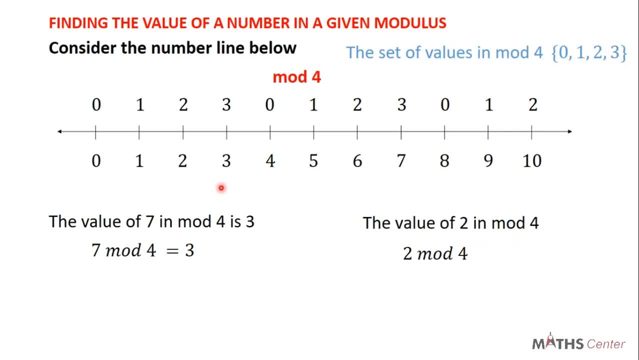 to find the value of 2 in mode four. we are going to look for the number that corresponds to 2 in mode 4 from our number line. the number that corresponds to 2 in mode four is not 2 in mode 4 number line. the number that corresponds to 2 in mode 4 is 2.. So it means that the value 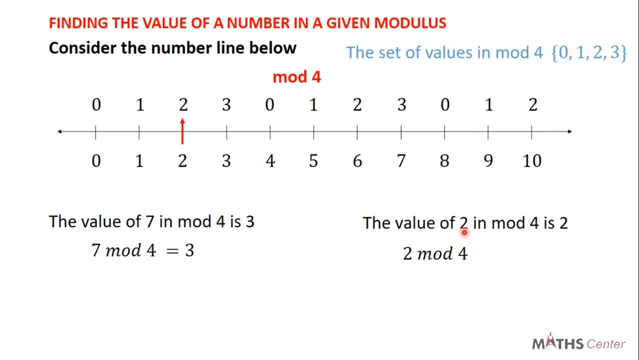 of 2 in mode 4 is 2.. We have seen that the value of 2 in mode 4 is written as 2 mode 4.. So 2 mode 4 is equal to 2.. Let's consider another example. We want to find the value. 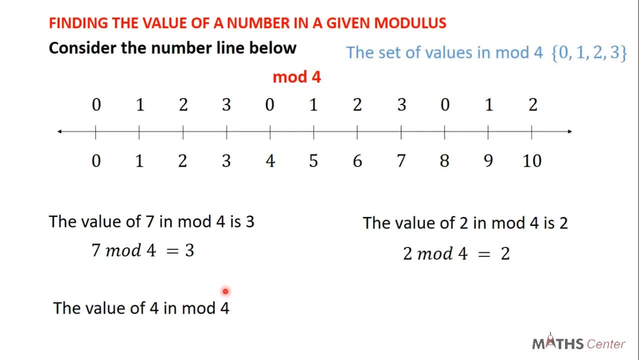 of 4 in mode 4.. The value of 4 in mode 4 is written as 4 mode 4.. So, for example, the value of 5 in mode 3 will be written as 5 mode 3.. The value of 1 in mode 2 will be written. 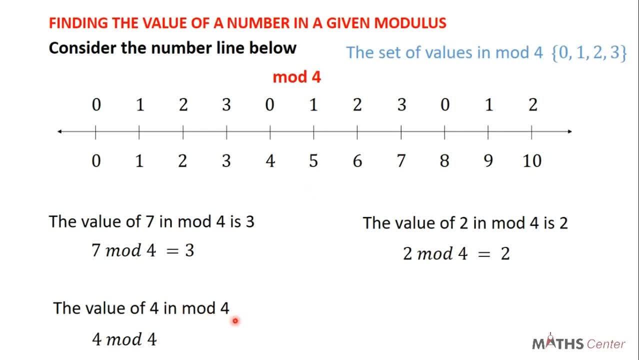 as 1 mode 2.. So the value of 4 in mode 4 is written as 4 mode 4.. So anytime you write 4 mode 4, it means the value of 4 in mode 4.. To find the value of 4 in mode 4, we look for the number that corresponds to 4 in mode. 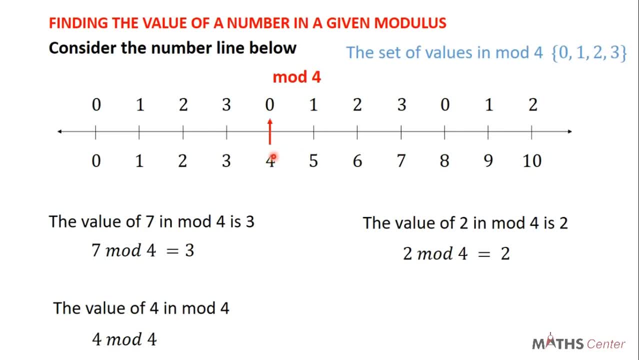 4.. From our number line, the number that corresponds to 4 in mode 4 is zero. So it means that the value of 4 in mode 4 is zero. This means that 4 mode 4 is zero. So you can see that using this approach, we can find the value of any number in any given. 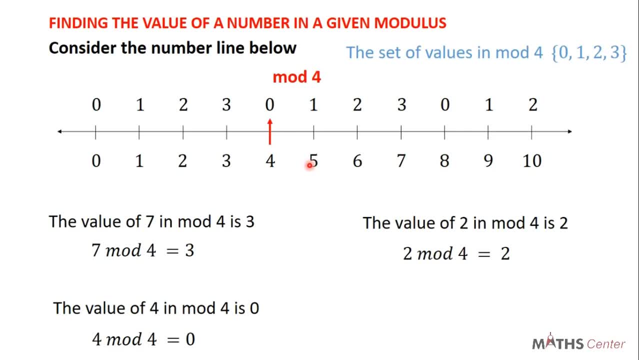 mode. So, for example, if you want to find the value of 5 in mode 5, all you do is to list the set of numbers in mode 5 against this set of whole numbers, then the one that corresponds to 5. that will give you the value of 5 in mode 5. 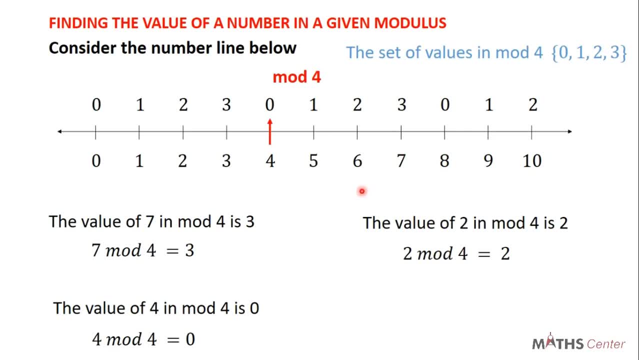 now let's look at something here. what if we want to find the value of 20 in mode 4 from our number line? if you want to find the value of 20 in mode 4, you will have to extend this number line to include 20. then we list the set of values in mode 4. against it, the one that will correspond to 20. 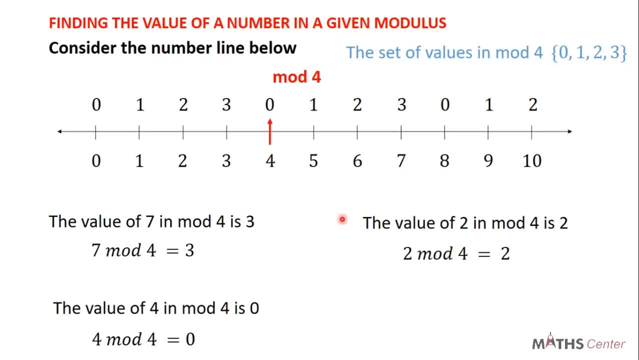 will give us the value of 20 in mode 4. that will be time consuming but fortunately for us, we have a very simple method of doing it. we are going to consider that method in the next video. thank you for watching this video. subscribe to this channel for more videos. in the next video, we are going to consider a very simple 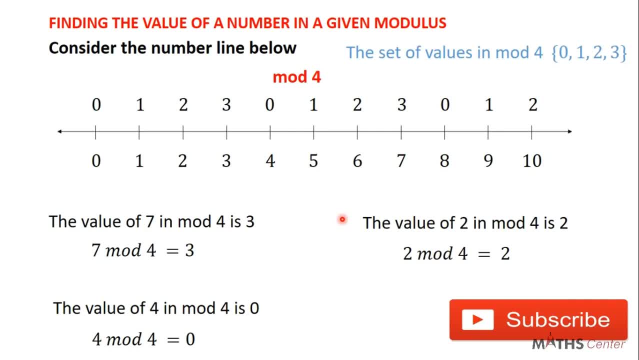 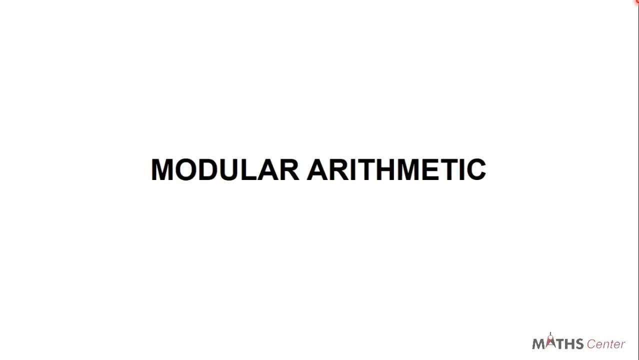 method of finding the value of a positive number in a given modulus. bye, bye, welcome back. we are on the topic: modular arithmetic. in the previous video, we learned how to use the number line to find the value of a number in a given modulus. in this video, we are going to learn how to find the value of a. 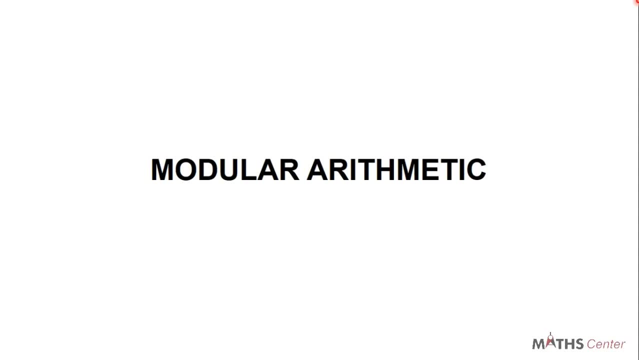 learn a very simple method of finding the value of a number in a given mood loss: Finding the value of a positive number in a given mood loss. We will learn how to find the value of a positive number in a given mood loss under three conditions. 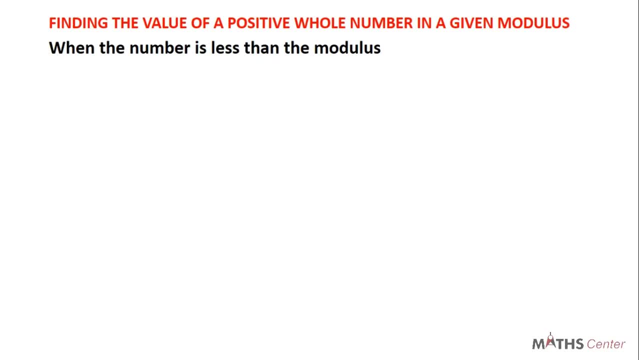 The first one is when the number is less than the mood loss. The value of x in mode y, which is written as x mode y, is x if x is less than y. The value of x in mode y, which is written as x mode y, is x if x is less than y. 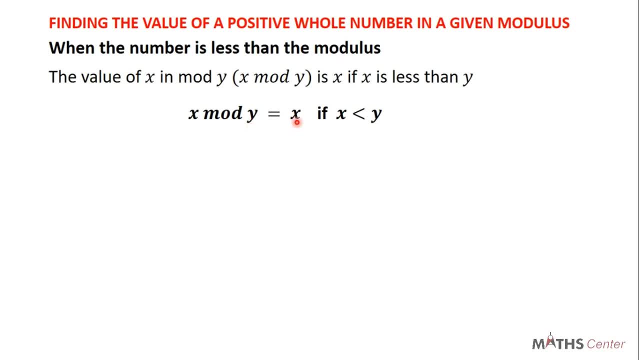 This means that x mode y is equal to x if x is less than y. So if the number x is less than the mood loss y, then x mode y is equal to x. So, for example, 2 mode 3 is equal to 2, 2 is less than 3, so 2 in mode 3 will give us: 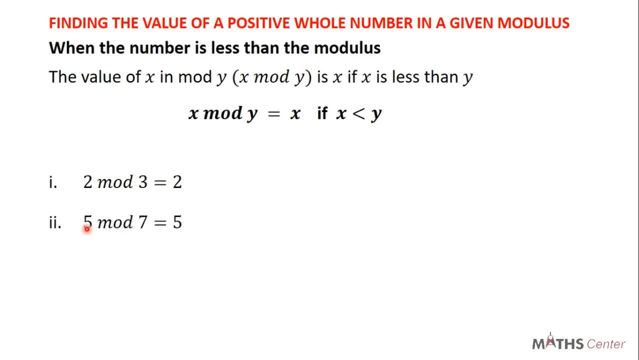 2.. Here is another example: 5 mode 7 is equal to 5, the number 5 is less than the mood loss 7. so 5 in mode 7, which is written as 5 mode 7, is equal to 5.. 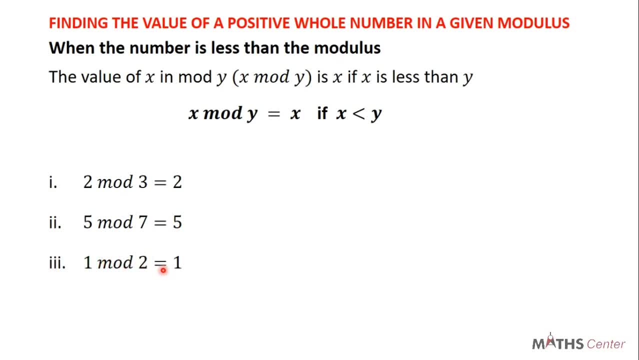 Here is another example: 1 mode 2 is equal to 1, the number 1 is less than the mood loss, which is 2, so 1 mode 2 is equal to 1.. Another example is 15 mode 24 is equal to 15, the number 15 is less than the mood loss. 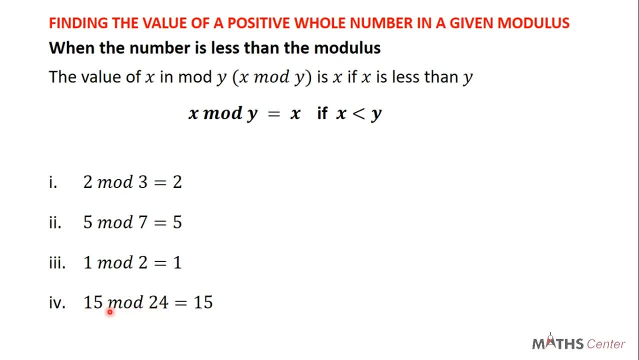 which is 2, so 1 mode 2 is equal to 1.. So 15 in mode 24, which is written as 15 mode 24, will give us 15.. So if the number x is less than the mood loss y, then x mode y is equal to x. 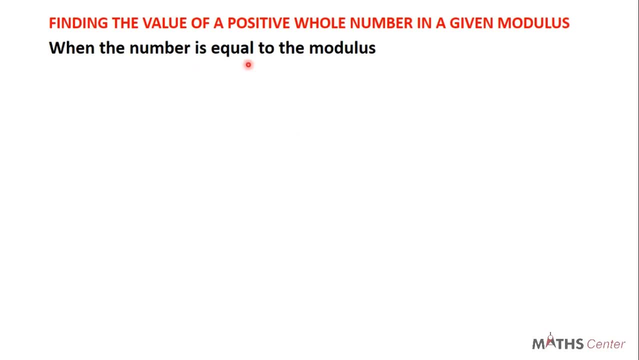 Let's consider the second condition. When the number is equal to the mood loss, the value of x in mode x, which is written as x mode x, x is zero. so x mod x is equal to zero. this means that when the number is equal to the modulus, 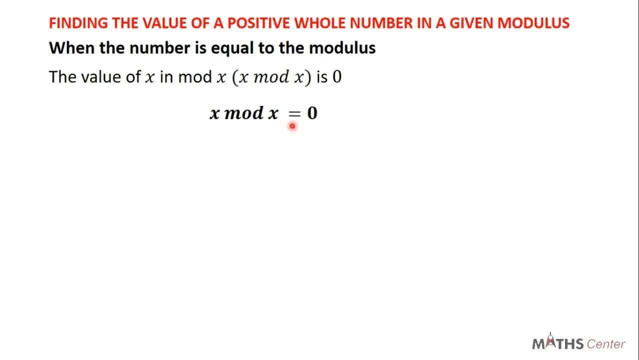 then the value of the number in that modulus is zero. so the number x is the same as the modulus, which is x. so x mod x will give us zero. for example, three mod three is equal to zero, five mod five is equal to zero, two mod two is equal to zero and 13 mod 13 is equal to zero. 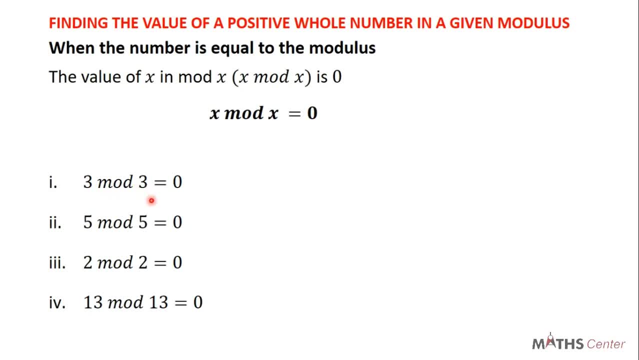 so if the number is equal to the modulus, then the value of that number in the modulus is zero. so three mod three is zero, five mod five is zero, two mod two is zero and 13 mod 13 is zero if the number is the same as the modulus. 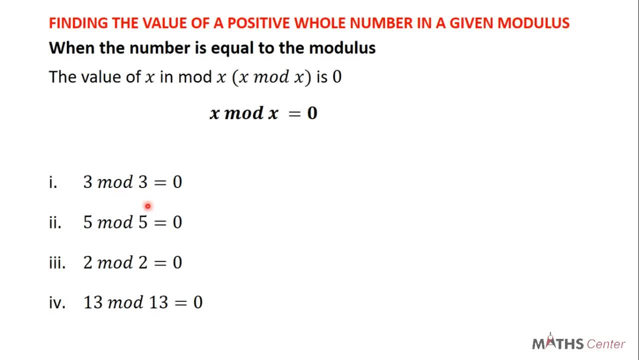 then the value of the number in the modulus is zero. so three mod three is zero, five mod five is zero, two mod two is zero and 13 mod 13 is zero. then the value of the number in that modulus is zero. The third condition is when the number is greater than the modulus. 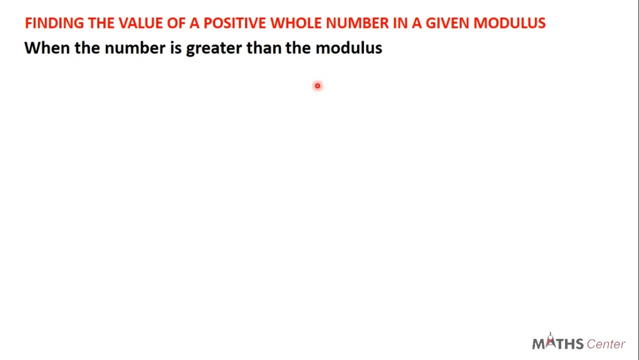 When the number is greater than the modulus. We have considered when the number is less than the modulus and when the number is equal to the modulus. We are now going to consider when the number is greater than the modulus. If x is greater than y. 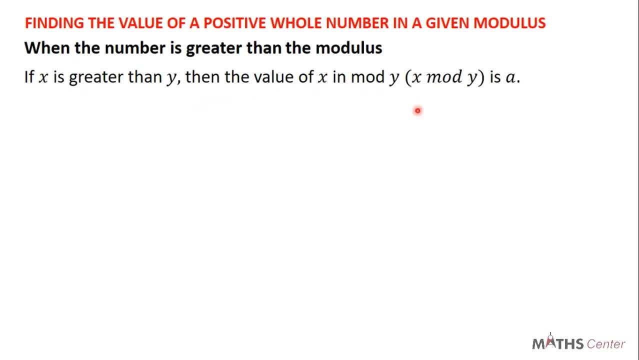 then the value of x in mode y, which is written as x mode y, is a and a is the remainder when x is divided by y. this means that if x is greater than y, then x mode y is equal to a, where a is the remainder when x is divided by y. so, for example, 5 mode 2 is equal to 1. we can see that. 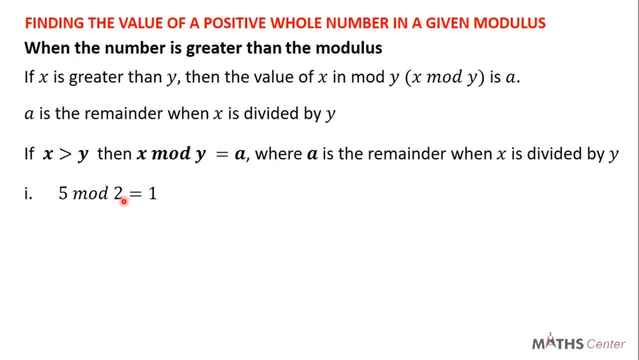 5, which is the number, is greater than the modulus, which is 2. so here to find the value of 5 in mode 2, what you are going to do is that you will divide 5 by 2. 5 divided by 2 will give us 2, remainder 1. 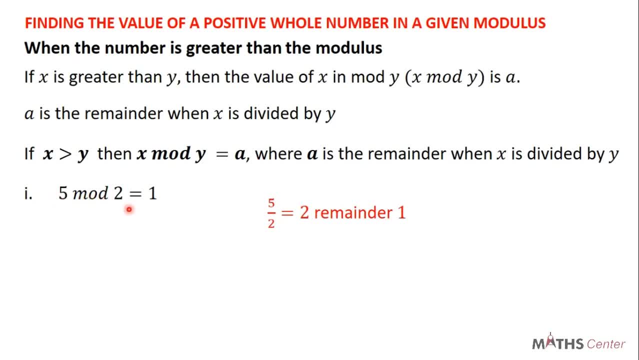 so the value of 5, mode 2, is equal to 1 and the remainder, when x is divided by y, is equal to 1, and the remainder, when x is divided by y, is equal to 1. so the value of 5 in mode 2 is the. 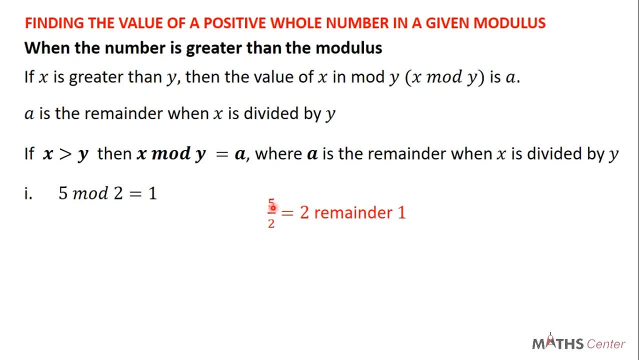 remainder when you divide 5 by 2. when we divide 5 by 2, we will get 2 and a remainder of 1, so 5 in mode 2 is equal to 1, because when we divide 5 by 2 we get a remainder of 1. another example is: 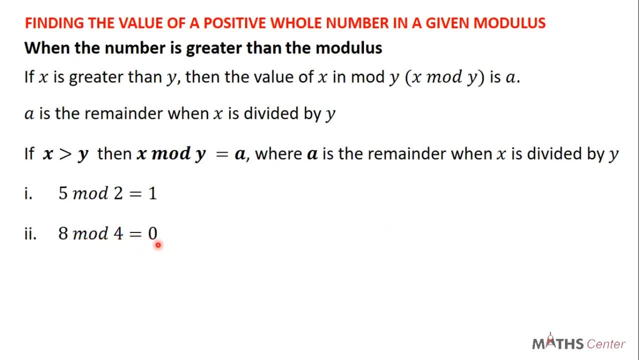 8 mode 4. 8 mode 4 is equal to 0. we have learned that if the number is greater than the modulus, then the value of that number in the modulus is the remainder when we divide a number by the modulus. so here, to find the value of 8 in mode 4, we will divide 8 by 4.. 8 divided by 4 will give us 2. 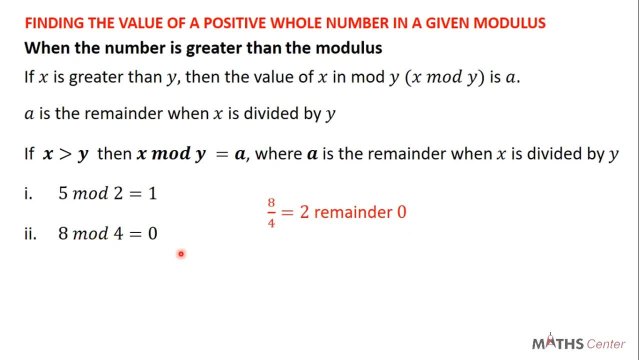 remainder 0.. the value of 8 mode 4 is the remainder when we divide 8 by 4. when we divide 8 by 4, we get a remainder of 0. so 8 mode 4 is equal to 0.. the next example is 27 mode 5. 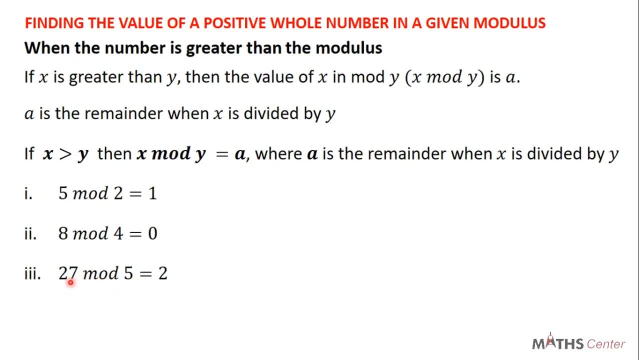 27, which is the number is greater than 5.. the value of 27 in mode 5 is the remainder when we divide 27 by 5.. when we divide 27 by 5, you will get five remainder two. so the remainder when we 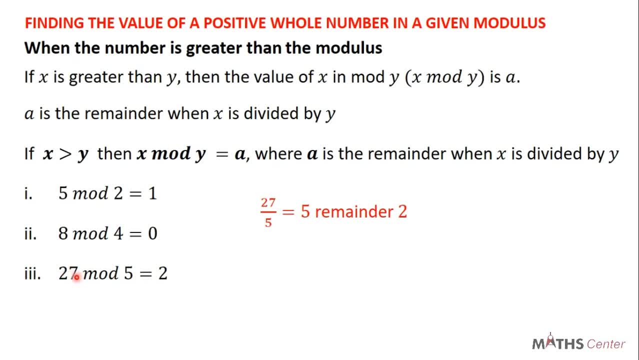 divide 27 by five is 0. for any number which is greater than a number, in the remainder 2, it means that 27 mode 5 is 2. another example is 10 mode 3. 10 is greater than 3, so the value of 10 in mode 3 is the remainder. when we divide 10 by 3, when 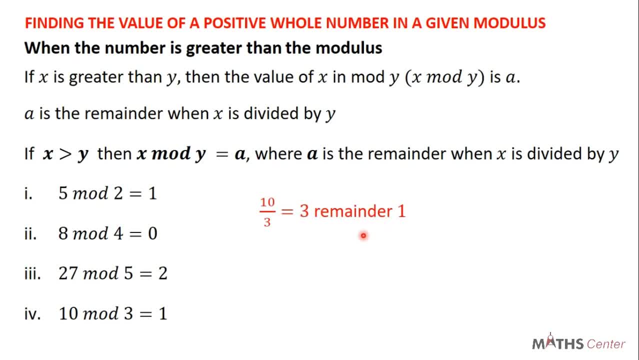 you divide 10 by 3, you will get 3 remainder 1. the value of 10 in mode 3 is the remainder. when we divide 10 by 3, 10 divided by 3 will give us 3 remainder 1. so 10 mode 3 is equal to 1. so when the number is greater than the modulus, the 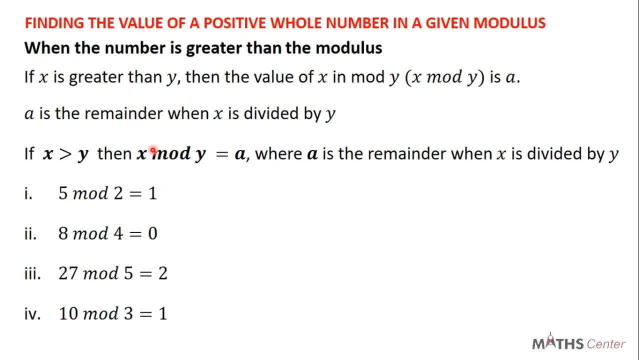 value of the number in that modulus is the remainder when we divide a number by the modulus. thank you for watching this video. subscribe to this channel for more videos. in this video, we have learnt how to find the value of a positive whole number when the number is less than the modulus. 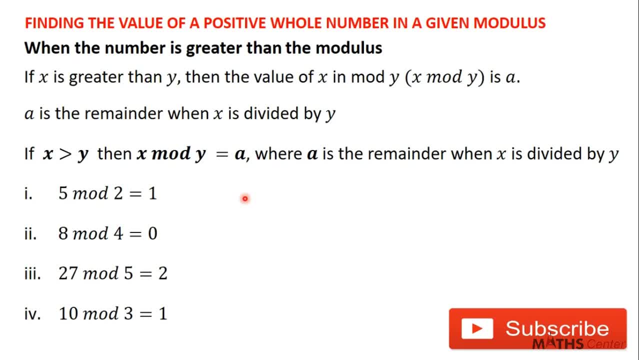 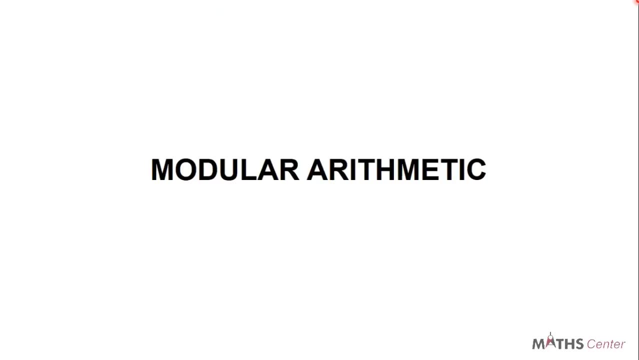 when the number is less than the modulus, when the number is less than the modulus, when the number is equal to the modulus and when the number is greater than the modulus. in the next video, we are going to learn how to find a value of a negative whole number in a given modulus. bye, bye, welcome back. we are still on the. 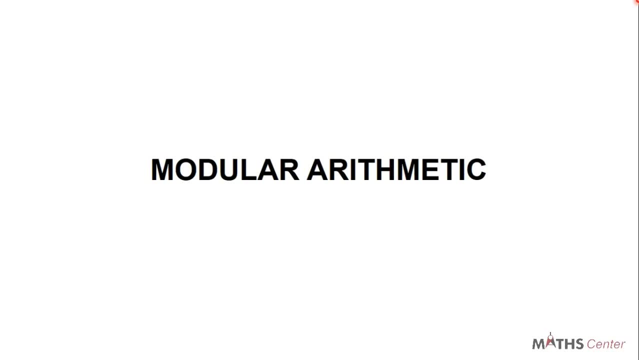 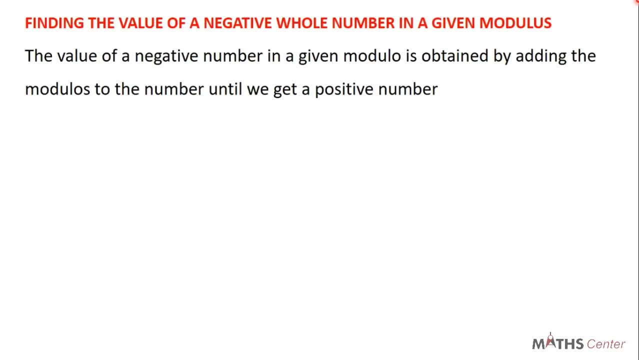 topic: modular arithmetic. in the previous video we learnt how to find the value of a positive whole number in a given modulus. in this video we are going to learn how to find the value of a negative whole number in a given modulus. finding the value of a negative whole number in a given modulus: the value. 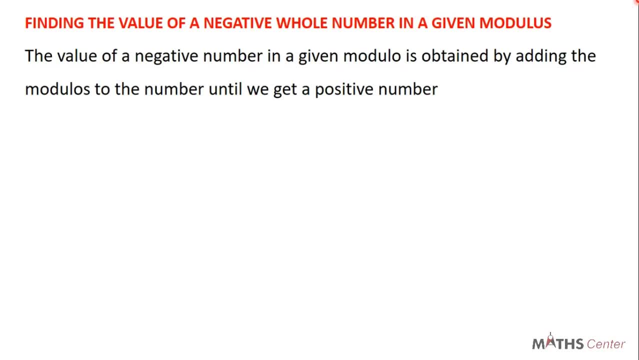 of a negative number in a given modulus is obtained by adding the modulus to the number until we get a positive number. the value of a negative number in a given modulus is obtained by adding the modulus to the number until we get a positive number. so, for example, to find a value of negative 7 in mode 2, we will add the modulus, which is 2. 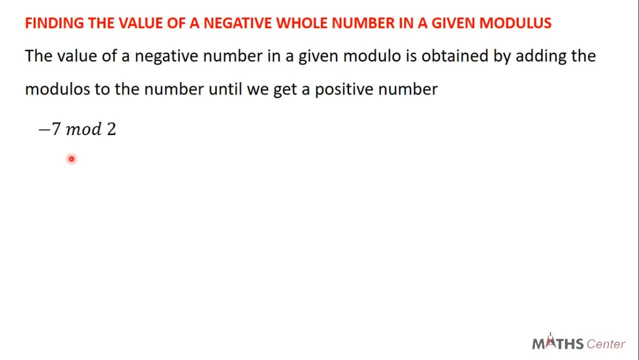 to the number until we get a positive number. so to begin with we will add 2 to the number, which is negative 7. so we have negative 7 plus 2 and that will give us negative 5.. we will keep on adding 2 to the number until we get a positive number. when we added 2 to 7, we had negative 5. 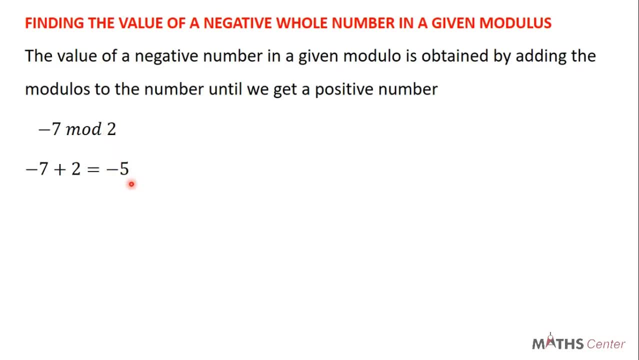 negative 5 is not a positive number, so you add 2 to it again, so you have negative 5 plus 2. negative 5 plus 2 will give us negative 3. negative 3 is not a positive number, so we will add 2 to the number until we get a positive number. negative 3 is not a positive number, so we 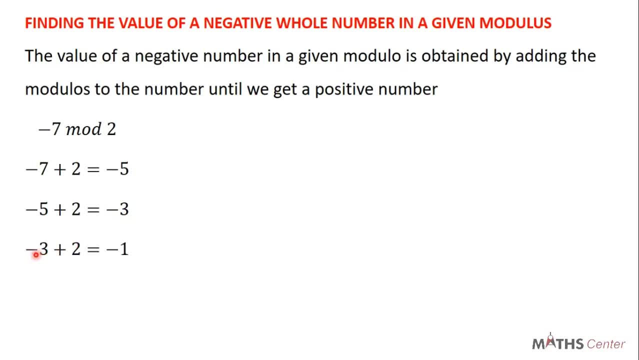 will add 2 to it again, and that will give us negative 3 plus 2.. Negative 3 plus 2 will give us negative 1. Negative 1 is still not a positive number, so we will add 2 to it again, and that will. 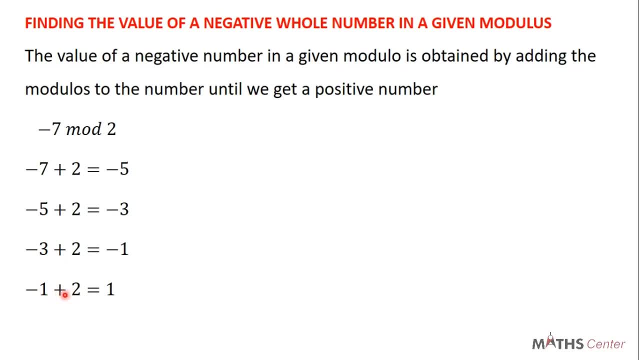 give us negative 1 plus 2.. Negative 1 plus 2 is 1.. The first positive number you have is the value of that number in the modulus. So here, the first positive number we are having is 1.. It means that 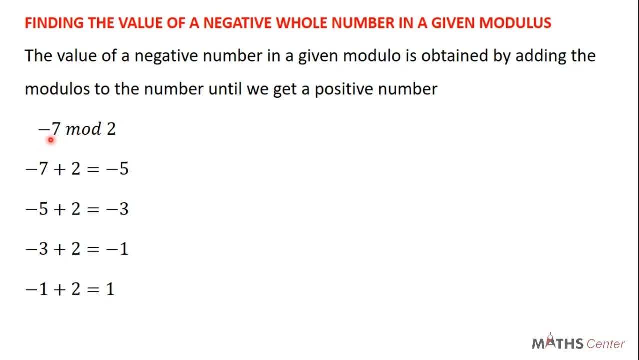 the value of negative 7 in mode 2, which is written as negative 7, mode 2 is 1.. So negative 7, mode 2 is equal to 1.. So to find the value of a negative number in a given modulus, all you need to do is: 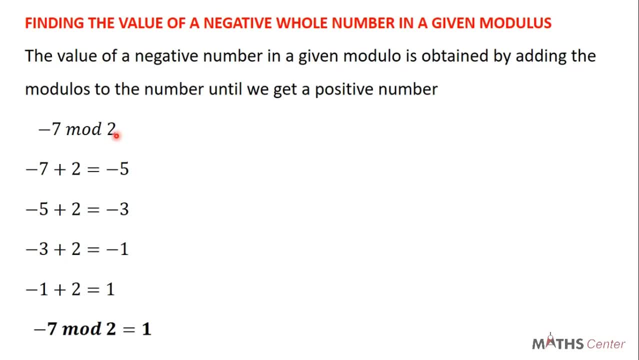 to keep on adding the modulus to the number until you get the first positive number. Here is another example. We want to find the value of negative 6 in mode 4.. So you want to find negative 6, mode 4.. We will add 4 to negative 6.. We will have negative 6 plus 4 and that will. 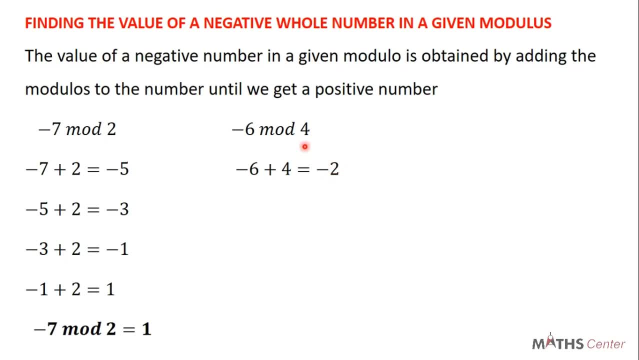 give us negative 2.. Negative 2 is not a positive number, so you add the modulus to it again. We have negative 2 plus 4.. Negative 2 plus 4 will give us 2. We now have a positive number. 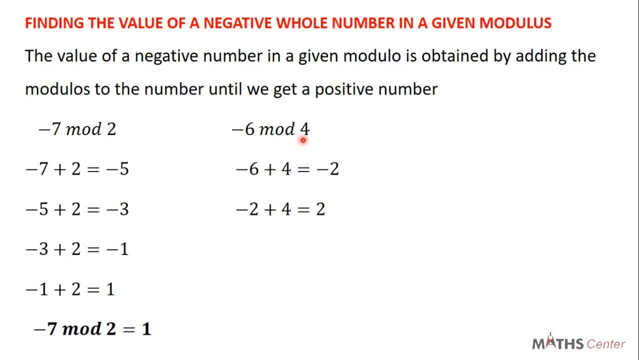 So it means that the value of negative 6 in mode 4 or negative 6, mode 4 is equal to 2.. Let's consider another example: Negative 2, mode 3.. We want to find the value of negative 2 in mode 3.. We have 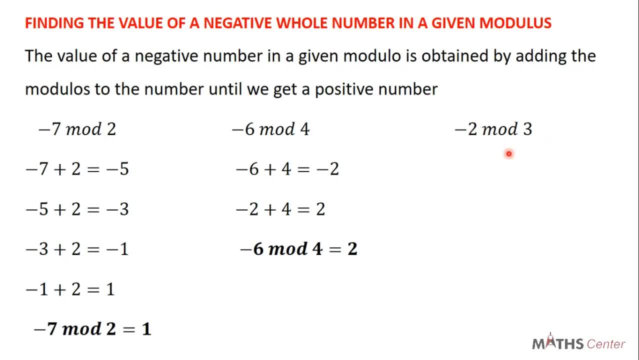 seen that to find the value of a negative whole number in a given modulus you add the modulus to the number until you get a positive number. So here we are going to add the modulus to negative 2. So you have negative 2 plus 3.. Negative 2 plus 3 is giving us 1. So we have a positive number here. 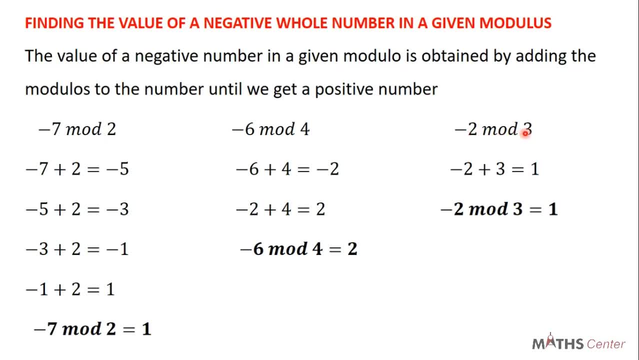 It means that the value of negative 2 in mode 3, or negative 2 mode 3, is equal to 1.. So you can see that to find the value of a negative whole number in a modulus is very simple. You keep on adding. 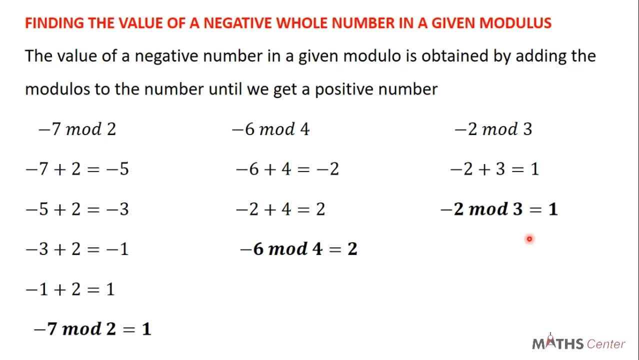 the modulus to the number until you get a positive number. Thank you for watching this video. Subscribe to this channel for more videos. In the next video, we are going to learn how to add, subtract and multiply numbers in a given modulus. Bye. 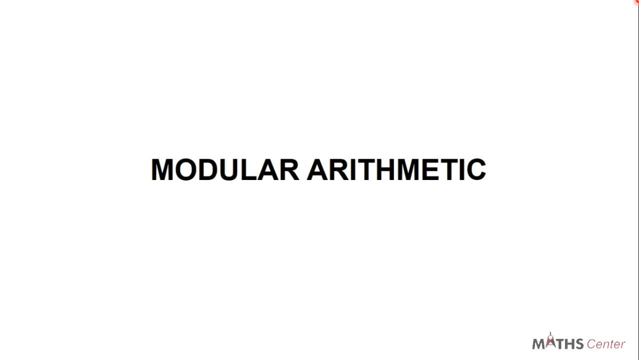 bye, Welcome back. We are on the topic Modular Arithmetic. In the previous video we learned how to find the value of a negative whole number in a given modulus. In this video, we will learn how to add, subtract and multiply numbers in a given modulus. 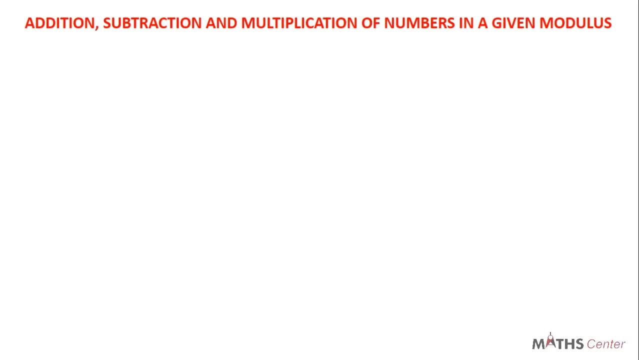 Addition, subtraction and multiplication of numbers in a given modulus. We will begin with addition. If we have a plus b mode y, it is equal to a plus b mode y. So, for example, 7 plus 3 mode 4.. 7 plus 3 will give us 10.. So 7 plus 3 mode 4 will give us 10 mode 4.. We have learned how to find the. 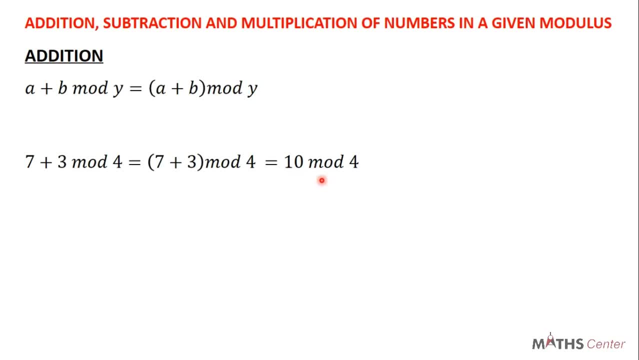 value of a number in a given modulus. We learned that if the number is greater than the modulus, then the value of that number in the modulus is the remainder when we divide the number by the modulus. Here 10 is greater than 4.. So the value of 10 in mode 4 is the remainder when we divide 10 by 4.. 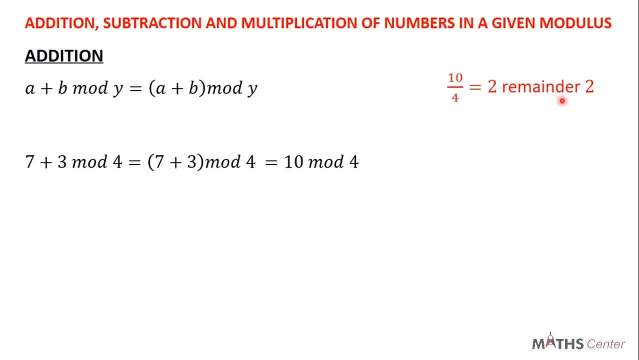 10 divided by 4 will give us 2 remainder 2.. So it means that when we divide 10 by 4, we will get a remainder of 2.. So 10 mode 4 is equal to 2, which is the remainder. 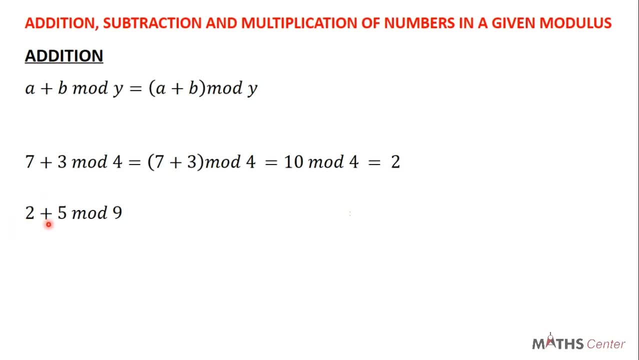 Let's consider another example. We have A 2 plus 5 mode 9.. So 2 plus 5 mode 9 will give us 2 plus 5 mode 9.. 2 plus 5 is 7.. So you have 7 mode 9.. 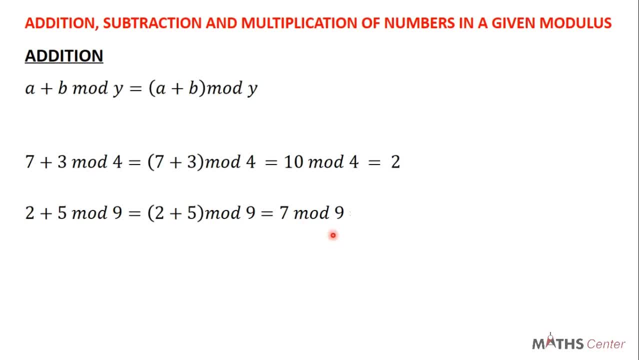 We have learned that if the number is less than the modulus, then the value of the number in the modulus is the same as the number. Here, 7 is less than 9.. So it means that the value of 7 in mode 9. 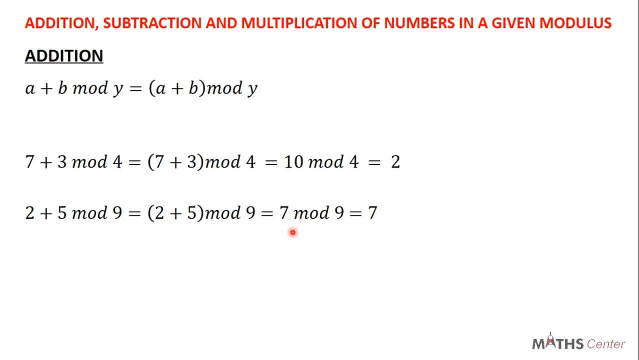 nine is equal to seven. let's consider another example. we have four plus four, mode eight. this will be equal to four plus four into brackets, then mode eight. four plus four will give us eight. so you have eight mode eight. we have learnt that if the number is the same as the modulus, 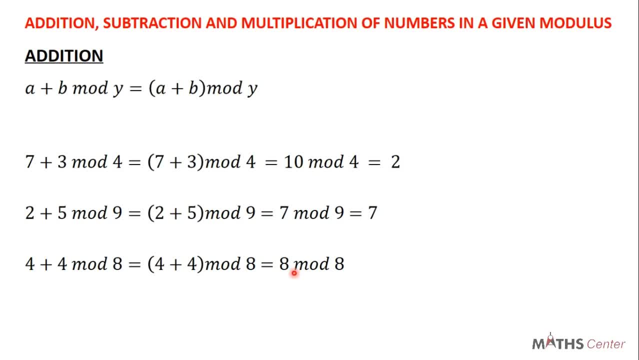 then the value of the number in the modulus is zero. eight is equal to eight. so eight mode eight will give us zero. let's consider another example. we have minus seven plus fifteen mode three. this will give us minus seven plus fifteen. into brackets, mode three minus seven plus fifteen will. 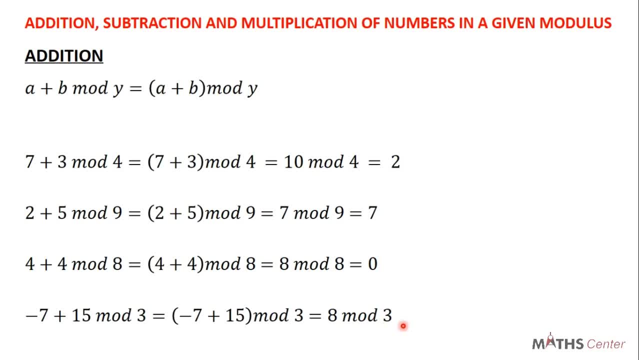 give us eight, so you have eight mode three. eight is greater than three, so the value of eight in mode three is the remainder. when we divide eight by three, when we divide eight by three, we will get two remainder two. so the value of eight in mode three, or eight mode three, is equal to the remainder, which is two. so this is how to add numbers in a. 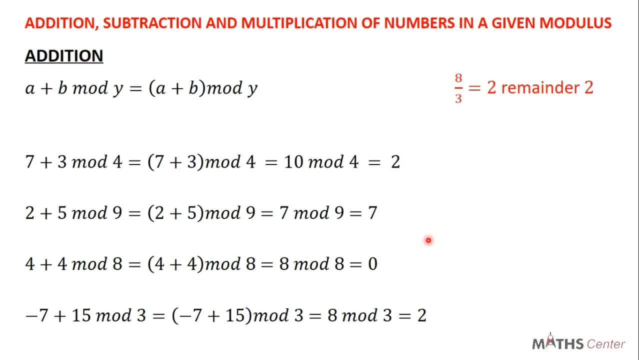 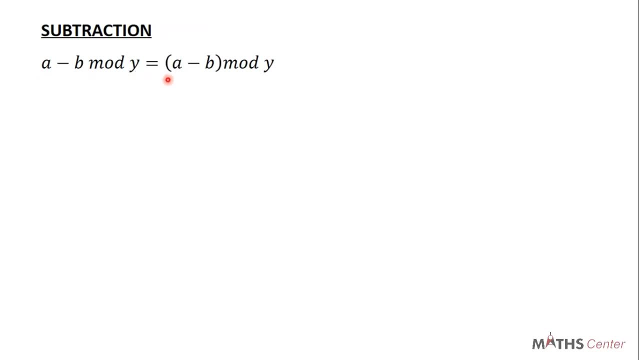 given modulus. let's learn how to subtract numbers in a given modulus. subtraction a minus b, mode y is equal to a minus b, into brackets, then mode y. so for example, eight minus two more three will be equal to eight minus two into brackets. more three: eight minus two give us six, so you have six more three. we have learnt how to find the value of a. 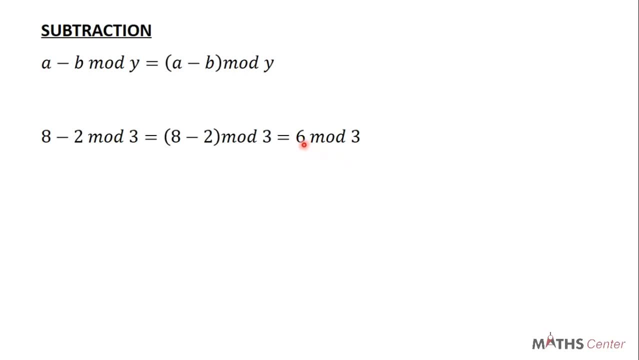 number in a given modulus. we have learned how to find the value of a number in a given modulus. we learnt that if the number is greater than the modulus, then the value of the number in the modulus is the remainder when we divide the number by the modulus. so here the value of six in mode three. 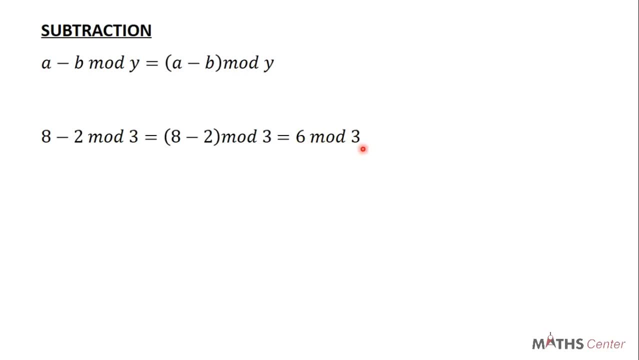 is the remainder that we will get when we divide six by three. six divided by three will give us two remainder zero. so it means that the value of six in mode three is equal to zero, because when we divide six by three we get a remainder of zero. let's consider another example. we have two minus. 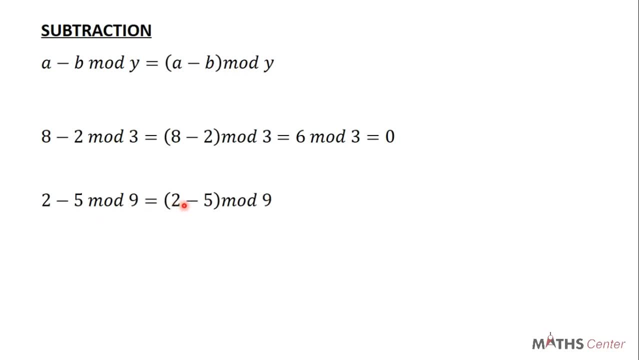 five. mode nine: this will be equal to two minus five. into brackets. then mode nine: two minus five will give us minus three. so you have minus three. mode nine: we have a negative number. we learnt in the previous video that number in a given modulus. you add the modulus to the number until you get a. 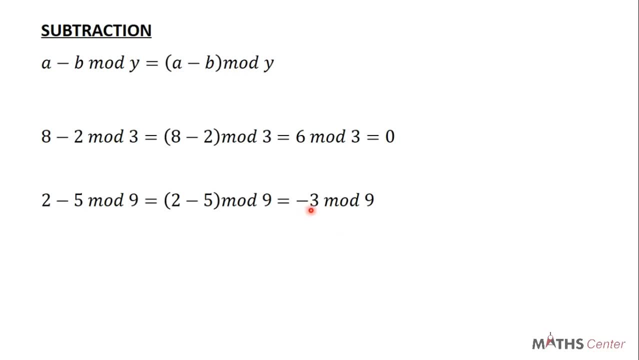 positive number. So here to find a value of negative 3 in mode 9, you add 9 to negative 3.. Negative 3 plus 9 will give us 6.. 6 is a positive number. so the value of negative 3 in mode 9 is 6.. Let's consider another example: 3 minus 1- Hearing. 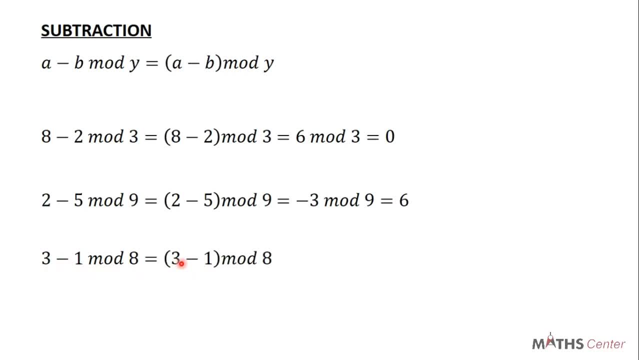 note here: this will be equal to 3 minus 1. Hearing note here: 3 minus 1 will give us 2, so you have 2. 2 is less than 8, so the value of 2 in mode 8 or 2 Carwynlate z ett over is equal. to 2.. Here the value of 3 in Mode 9 is given as negative 3, and this is now less than 8 to you. Let's suppose, bring 8 to the rescue to code 8, technical errorunivers might happen. 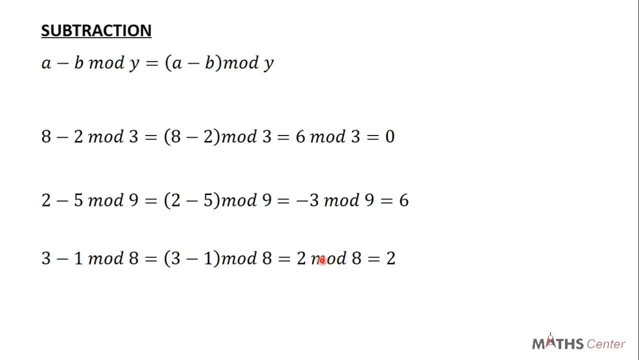 is less than the modulus, then the value of the number in the modulus is equal to the number itself. so 2 in mode 8 is equal to 2. we have learned how to add and subtract numbers in a given modulus. now let's learn how to multiply numbers. 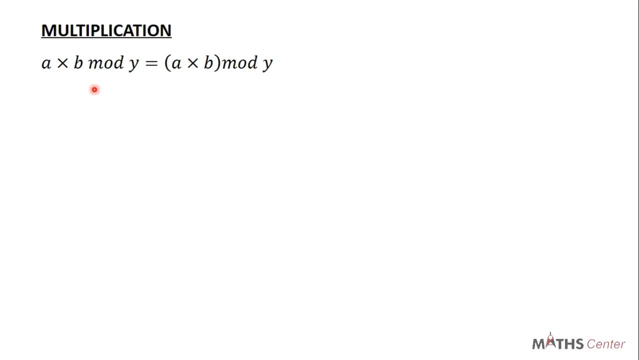 in a given modulus multiplication, a times b mode y is equal to a times b into brackets mode y. so for example, 2 times 2 mode 6 will be equal to 2 times 2 into brackets mode 6. 2 times 2 give us 4, so we have 4 mode 6. we have seen that. 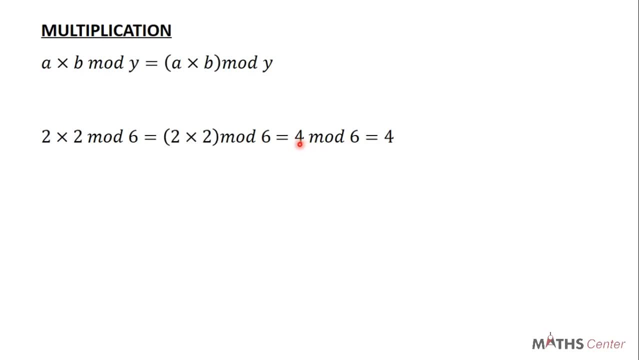 4. mode 6 is equal to 4, since 4 is less than 6, 2 times 5. mode 9 is equal to 2 times 5. into brackets, mode 9. 2 times 5 will give us 10. so you have 10 mode 9. 10 is greater than 9. 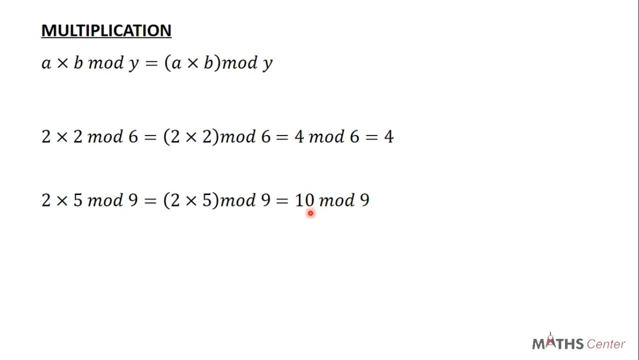 so the value of 10 mode 9 is the remainder. when we divide 10 by 9, 10 divided by 9 will give us 1 remainder, 1. so 10 mode 9 is equal to 1, 3 times 0. mode 5 will be equal to 3 times 0. into brackets. 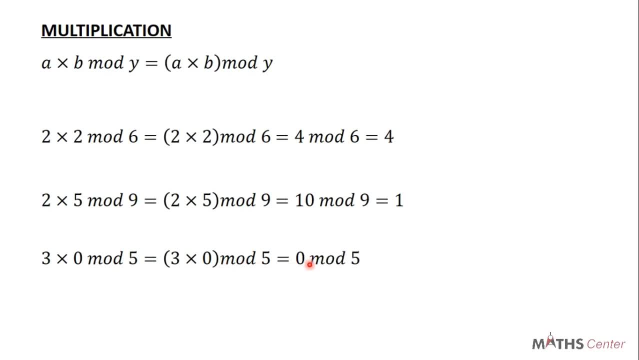 mode 5: 3 times 0 is 0, so you have 0 mode 5. 0 is less than 5, so 0 in mode 5 or 0 mode 5 is equal to 0. finally, 1 times 1, mode 3 will be equal to 1 times 1. into brackets: mode 3: 1 times 1 is 1, so you have 1 mode. 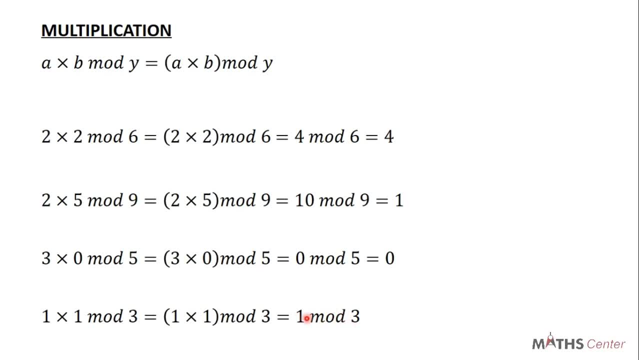 3. 1 is less than 3, so the value of 1 in mode 3 is equal to 1. so you can see that addition, subtraction and multiplication of numbers in a given modulus is very simple. you add, subtract or multiply the number. you add, subtraction and multiplication of numbers. 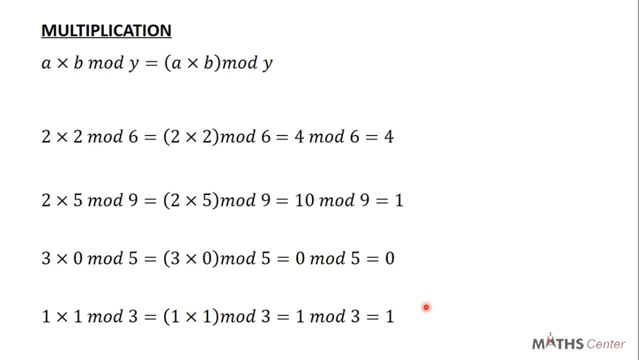 then you find the value of that number in the given modulus. thank you for watching this video. subscribe to this channel for more videos. now we know how to add and multiply numbers in the given modulus. in the next video, we are going to learn how to draw addition and multiplication tables for a set of numbers in a given modulus. 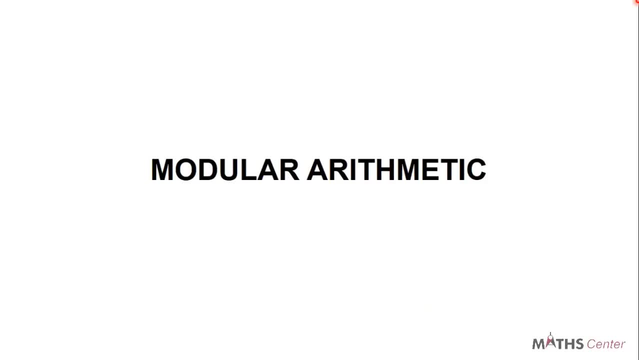 bye-bye, welcome back. we are on the topic modular arithmetic. in the previous video we learned how to add, subtract and multiply numbers in a given modulus. in this video we are going to learn how to draw a table for an operation in a given modulus. tables in modular arithmetic: to draw a table. 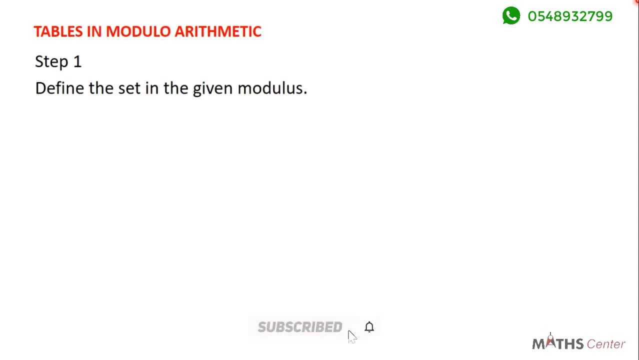 for an operation in a given modulus, the first thing you have to do is to define the set of values in that modulus. we have learnt that in every modulus there are a set of values that are used. so, for example, in mode 2 the set of values used are 0 and 1 the set of values used. 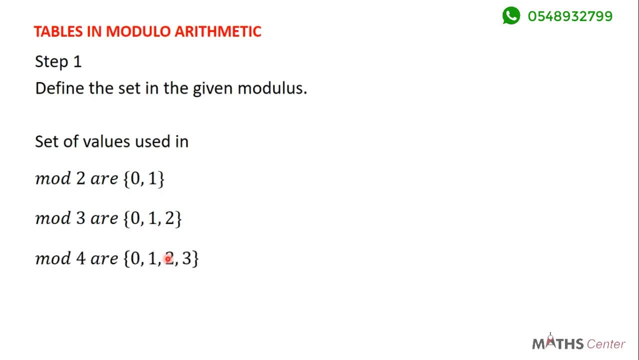 in mode 3 are 0, 1, 2. in mode 4, the values are 0, 1, 2, 3. in mode 5, the values are 0, 1, 2, 3, 4. so So to draw a table for an operation in a given modulus, the first thing you do is that you 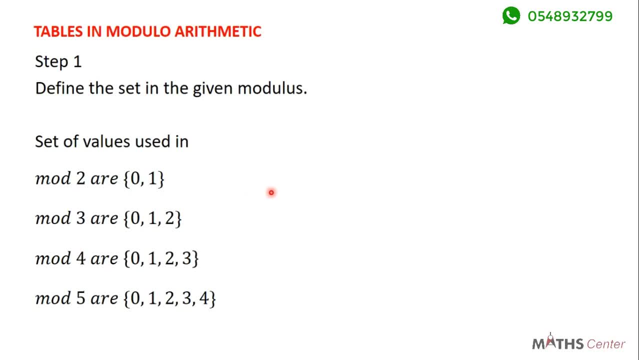 define the set of values in that modulus. So if you want to draw an addition table for mode 4, you will first have to define the set of values in mode 4.. They are 0,, 1,, 2, and 3.. 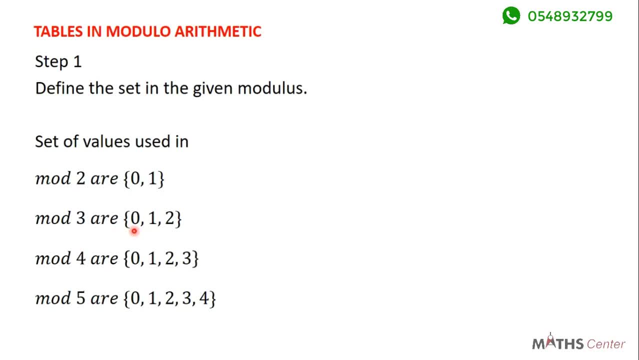 If you want to draw a table in mode 3, the set of values are 0,, 1, and 2. So you define the set of values in that modulus. After you have defined the set of values, you will use it to draw the table. 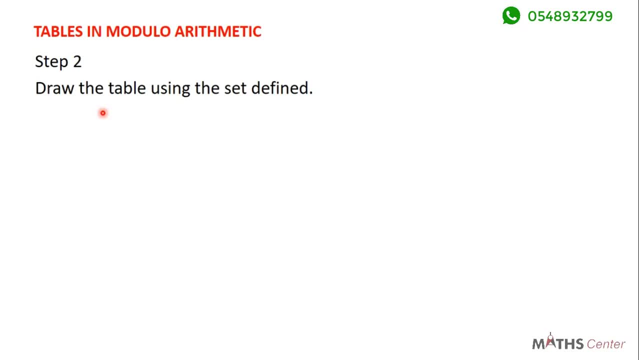 So you draw the table using the set defined. For example, if you want to draw an addition table for mode 5, the first thing you have to do is to define the set values in mode 5.. The set of values used in mode 5 are 0,, 1,, 2,, 3,, 4.. 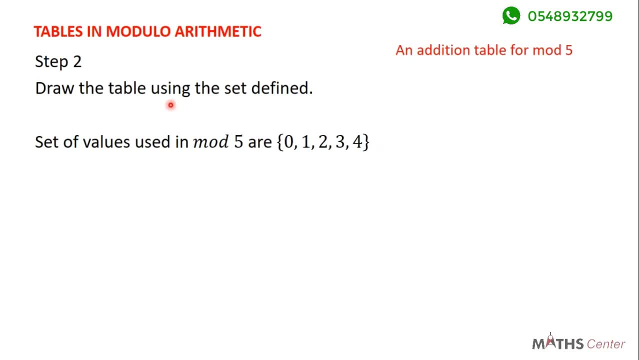 After you have defined the set of values in mode 5, you can draw a table. This is called missing table. we use it to draw the table. we have five values here. so you draw a table with six columns and six rows. so in this table the number of columns are one, two, three. 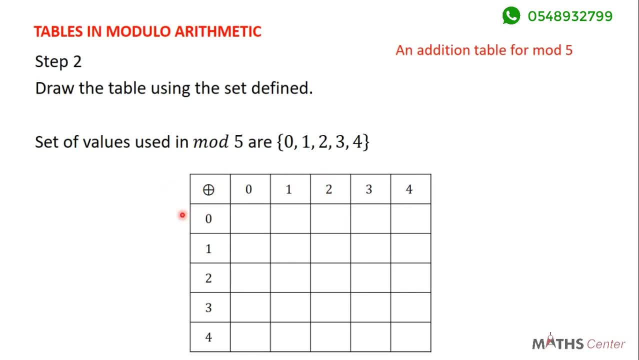 four, five, six, and the number of rows are one, two, three, four, five, six. in the first cell you write the sign of the operation you are going to perform. we want to draw an addition table, so the operation is addition. so in the first cell of the table you write the addition sign. so you write an addition sign. then we draw a. 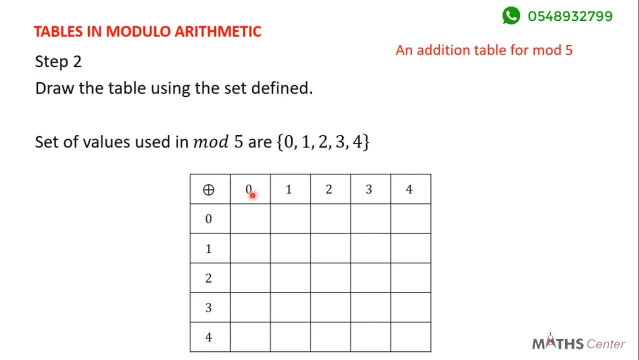 circle around it. you the list, the set of numbers in the first rule and the first column, just as we have here. after we have drawn the table like this, you fill it out completely by performing the operation in the given modulus. so here we are going to fill this table by adding the numbers. 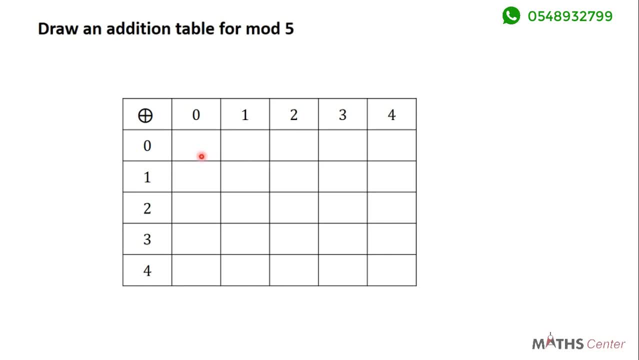 in the first cell. we are going to fill in the numbers in the second table. the Quiz rotten can make, but we willwerk them together, so give the rest given. so here you mode five. so we have our table here and we are going to fill it out by adding the numbers in. 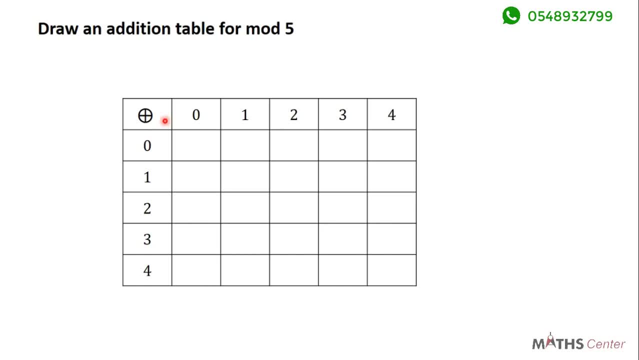 mode five, the first one will be zero plus zero. zero plus zero is zero. then you find the value of zero in mode five: zero in mode five or zero. mode five is equal to zero. so it means that here will be zero. we have zero plus one. zero plus one is one. one move. five is one. zero plus two zero. 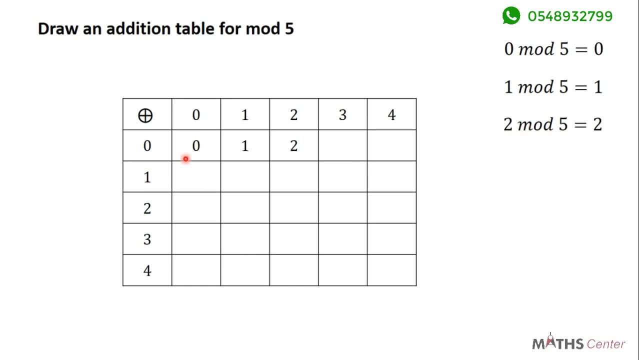 plus two is two. two mode five is two. zero plus three. zero plus three is three. 3om you'd 5 is 3, 0 plus 4 is 4. 4 mode 5 is 4. after you've completed the first rule, You come to the second rule. you have 1 plus 0,. 1 plus 0 is 1, 1. in mode 5 is 1, 1 plus. 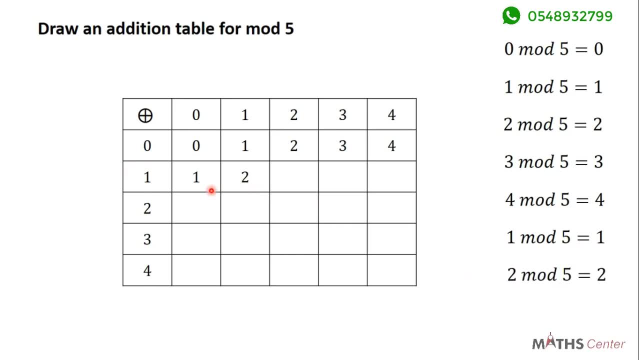 1 is 2,. 2 in mode 5 is 2, 1 plus 2 is 3,. 3 in mode 5 is 3, 1 plus 3 is 4,. 4 in mode 5 is 4, 1 plus 4 is 5,. 5 in mode 5 is 0,. 2 plus 0 is 2,. 2 in mode 5 is 2, 2 plus 1 is 3, 3 in. 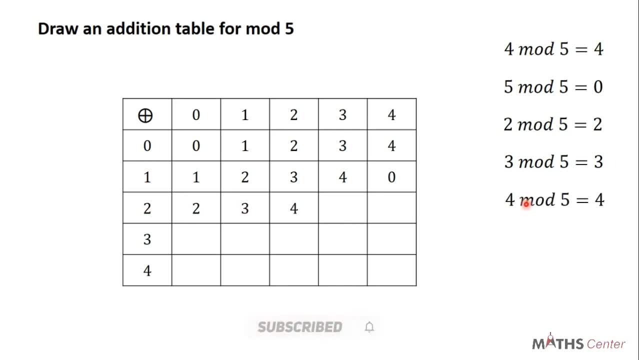 mode 5 is 3,. 2 plus 2 is 4,. 4 in mode 5 is 4,. 2 plus 3 is 5, 5 in mode 5 is 0,. 2 plus 4 is 6. 6 in mode 5 is 1, because you divide 6 by 1 and you have 1 remainder 1. 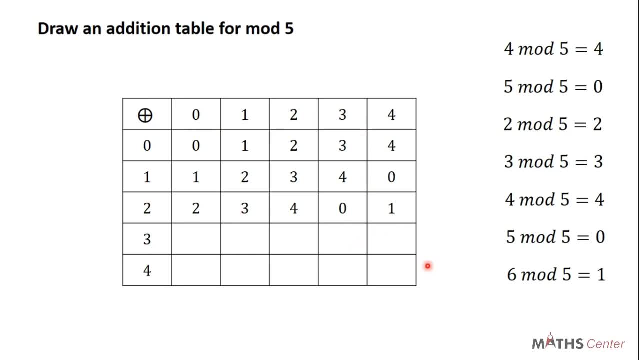 so you write the remainder: 2 plus 4 is 6 and 6 in mode 5 is 1. let's move on to the next rule. you have 3 plus 0, which is 3, 3 in mode 5 is 3, 3 plus 1 is 4, 4 in. 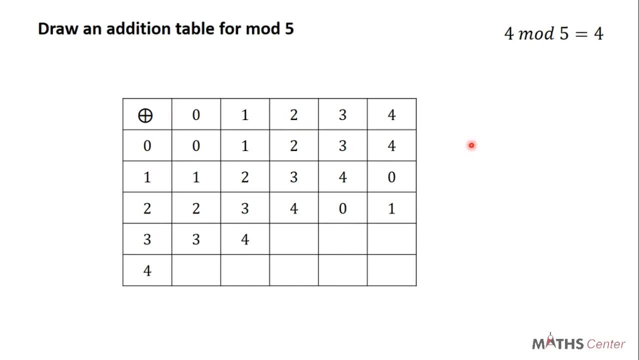 mode 5 is 4. 3 plus 2 is 5. 5 in mode 5 is 0. 3 plus 3 is 6. 6 in mode 5 is 1. 3 plus 4 is 7. 7 in mode 5 is 2. the number is bigger than the modulus, so you divide. 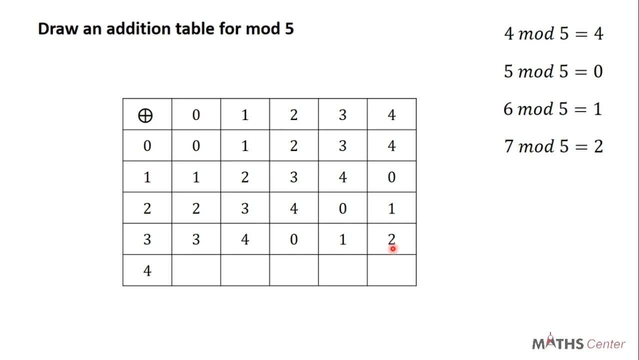 7 by 5 and that will give us 1 remainder 2. you write the remainder. so 3 plus 4 is 7, and 7 in mode 5 is 2. let's move on to the last rule: 4 plus 0 is 4, 4 in mode 5 is 4, 4 plus 1 is 5, 5 in. 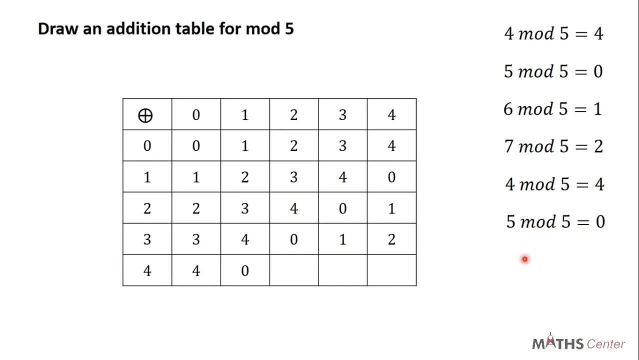 mode 5 is 0, 4 plus 2 is 6, 6 in mode 5 is 1, 4 plus 3 is 7, 7 in mode 5 is 2 and finally, 4 plus 4 is 8, 8 in mode 5 is 3. so we 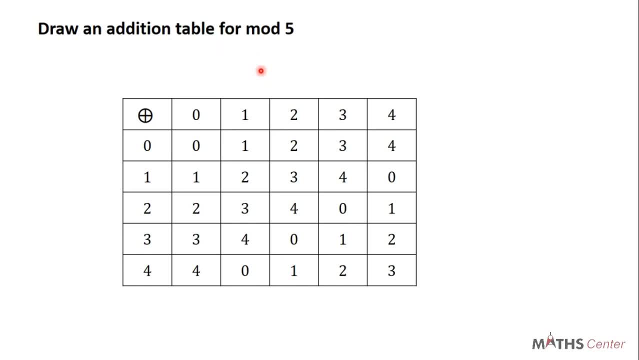 have 3 in mode 5 and 4 in mode 5 is 1. so we have 3 in mode 5 is 2 and 4 plus 4 is 8. 8 in mode 5 is 3. so we have now completed our addition table for mode 5. you can see that is very simple. 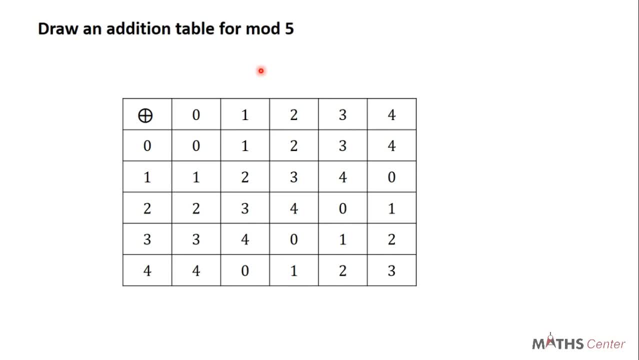 to draw a table for an operation in giving modulus, the first thing you have to do is to define the set of values in that modulus. after that you use the set of values to draw the table. then you fill out the table by performing the operation in the given modulus. so if the operation is addition, you add the. 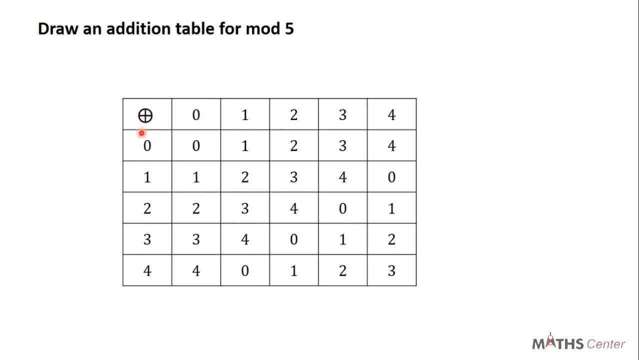 numbers in the modulus. if the operation is multiplication, you multiply the numbers in the modulus. Thank you for watching this video. Subscribe to this channel for more videos. In the next video we are going to solve another question on drawing a table for an operation in a given modulus. Bye-bye. 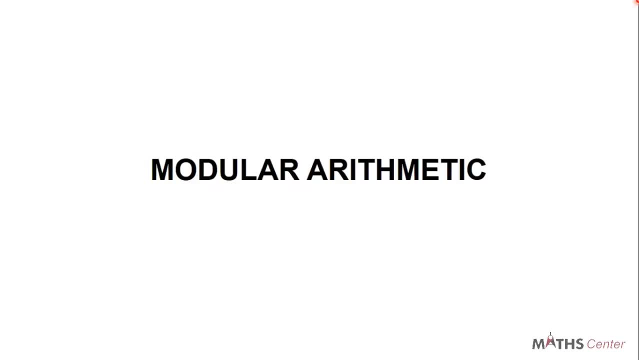 Welcome back. We are on the topic Modular Arithmetic. In the previous video we learnt how to draw a table for an operation in a given modulus. In this video, we are going to solve a question on drawing tables for an operation in a given modulus. 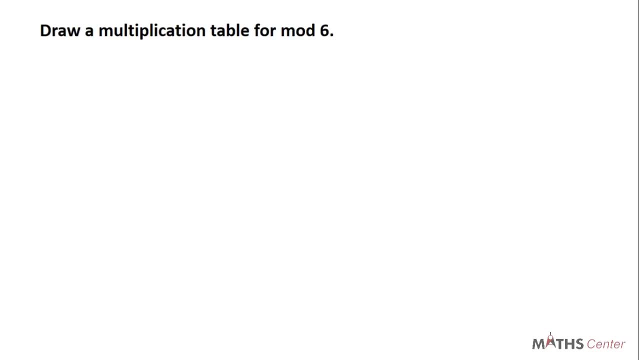 The question for this video is: Draw a multiplication table for mode 6.. We learnt in the previous video that when you are asked to draw a table for an operation in a given modulus, the first thing you have to do is to define the set of values in that modulus. 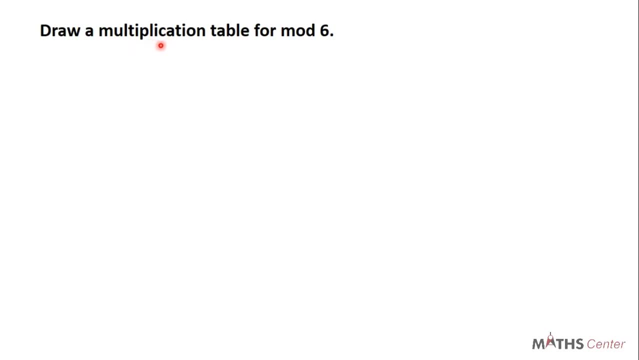 Here we are being asked to draw a multiplication table for mode 6.. So the first thing you do is to define the set of values used in mode 6.. The set of values used in mode 6 are 0,, 1,, 2,, 3,, 4, 5.. 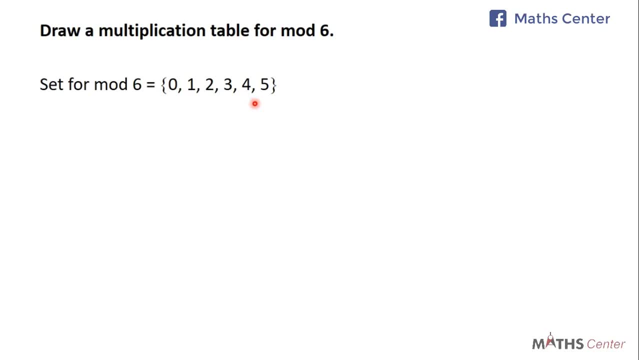 After you have defined a set of values, the next thing we have to do is to use this set of values to draw the table. We have six values in total, So we are going to draw a table with seven columns and seven rows. In the first cell of the table, you write the sign of the operation we are going to perform. 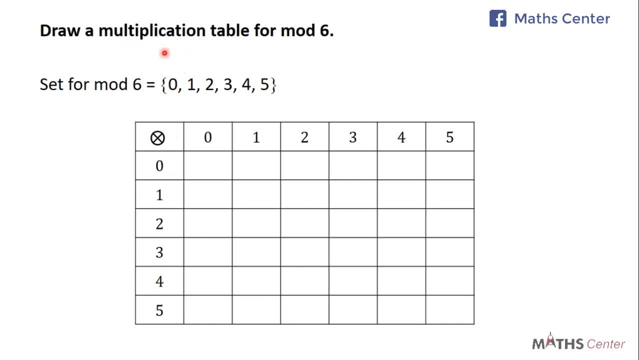 We are going to draw a multiplication table, So the operation is multiplication. In the first cell of the table you write the multiplication sign, then you draw a circle around it, Then you list the set of values in the first row and the first column, just as we have in this table. 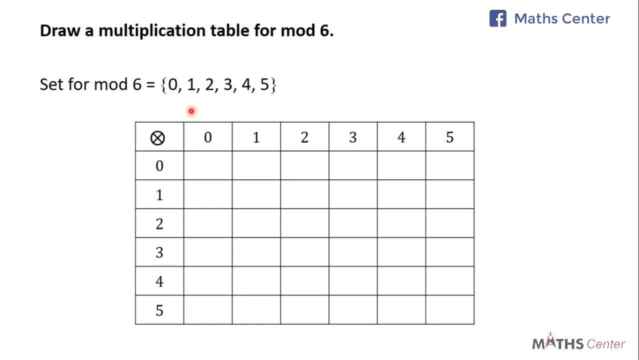 After you have drawn the table like this, you fill it out by performing the operation in the modulus. The operation is multiplication and the modulus is 6.. So we are going to multiply these numbers in mode 6.. The first one is 0 times 0.. 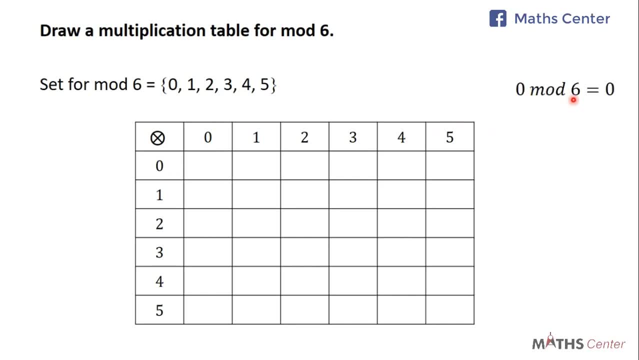 0 times 0 is 0.. 0 in mode 6 is 0.. So we have 0 here. 0 times 1 is 0.. 0 in mode 6 is 0.. 0 times 2 is 0.. 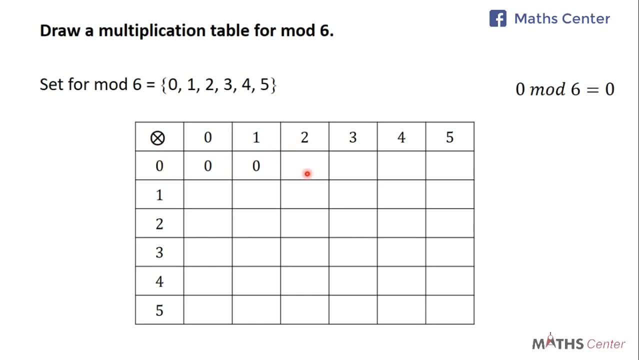 0 in mode 6 is 0.. 0 times 3 is 0.. 0 in mode 6 is 0.. 0 times 4 is 0.. 0 in mode 6 is 0.. 0 times 5 is 0.. 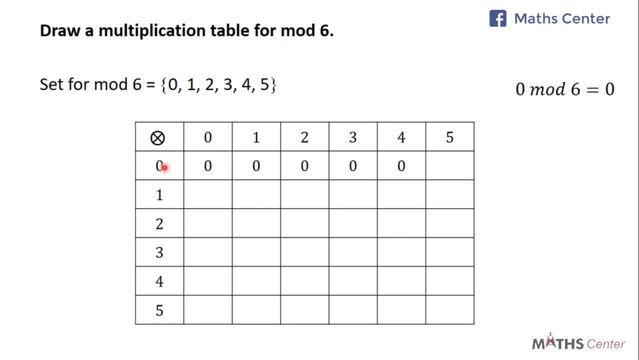 0 in mode 6 is 0.. 0 times 5 is 0.. 0 in mode 6 is 0.. 0 in mode 6 is 0.. So in the first rule all the numbers are 0.. 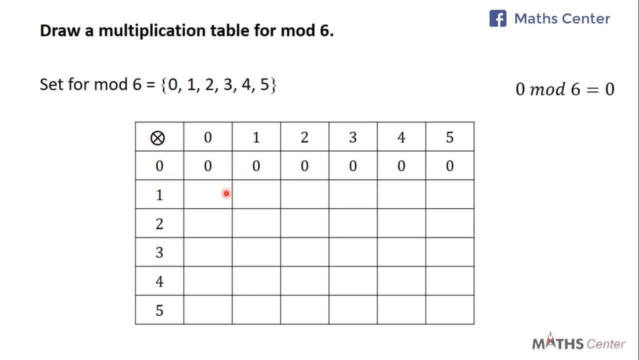 Let's move on to the next rule: 1 times 0 is 0.. 0 in most 6 is 0.. 1 times 1 is 1.. 1 in most 6 is 1.. 1 times 2 is 2.. 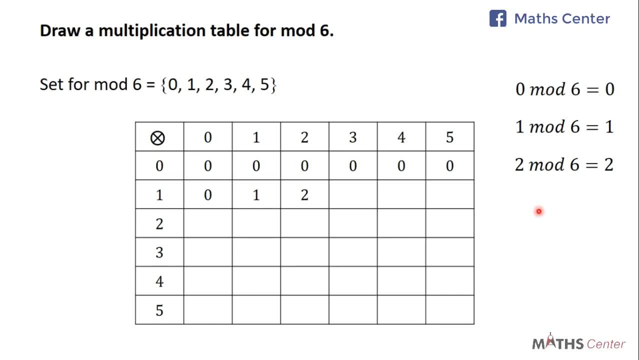 2 in most 6 is 2.. 1 times 3 is 3.. 3 in most 6 is 3.. 1 times 4 is 4.. 4 in most 6 is 4.. 1 times 5 is 5.. 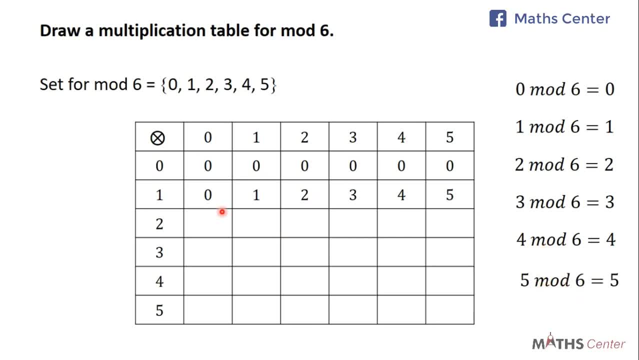 5 in most 6 is 5.. Let's move on to the next rule: 2 times 0 is 0.. 0 in most 6 is 0.. 2 times 1 is 2.. 2 in most 6 is 2.. 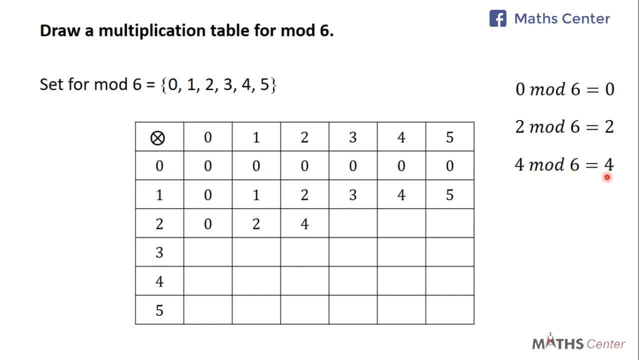 2 times 2 is 4.. 4 in most 6 is 4.. 2 times 3 is 6.. 6 in most 6 is 4.. 6 in most 6 is 0.. 2 times 4 is 8.. 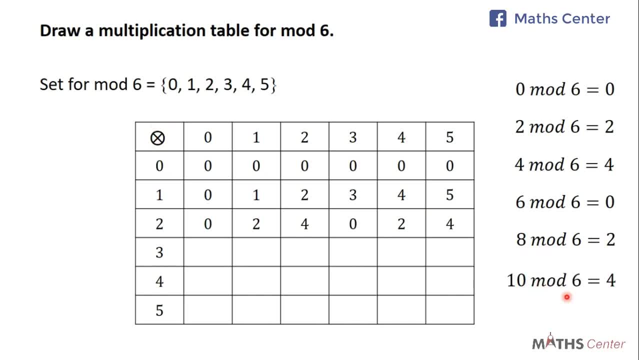 8 in most 6 is 2.. 2 times 5 is 10.. 10 in most 6 is 4.. Let's move on to the next rule. We have 3 times 0.. 3 times 0 is 0.. 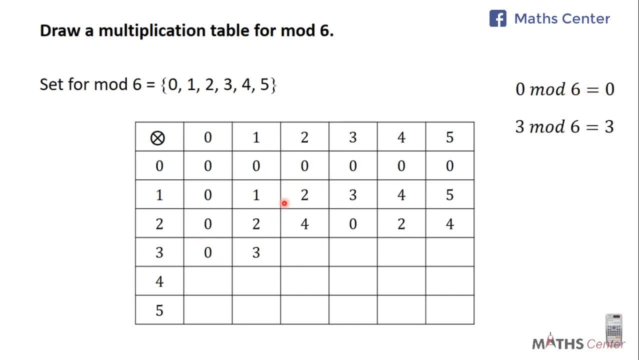 0 in most 6 is 0.. 3 times 1 is 3.. 3 in most 6 is 3.. 3 times 2 is 6.. 6 in most 6 is 0.. 3 times 3 is 9.. 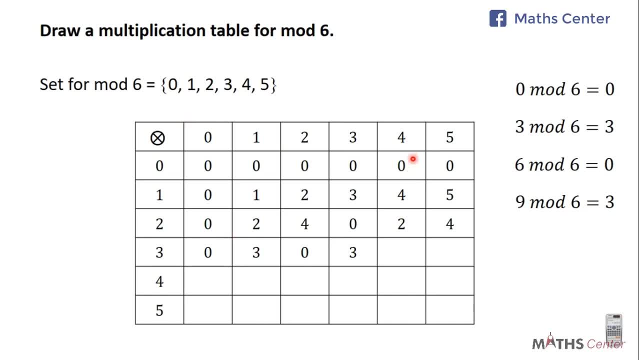 9 in most 6 is 3.. 3 times 4 is 12.. 12 in most 6 is 0. Because 12 divided by 6 will give us 2 in most 6 is 0. So we write the remainder. 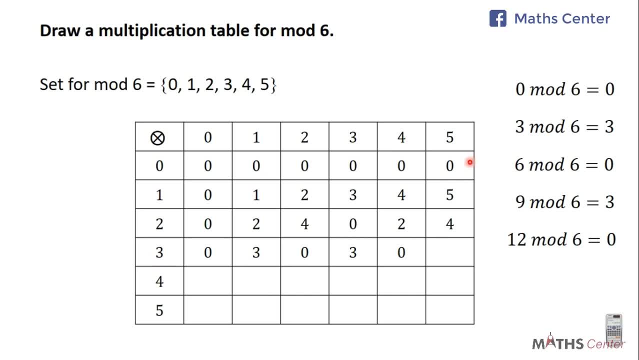 So 12 in most 6 is 0.. 3 times 5 is 15.. 15 in most 6 is 3.. We divide 15 by 6.. You have 2 in most 6 is 3.. 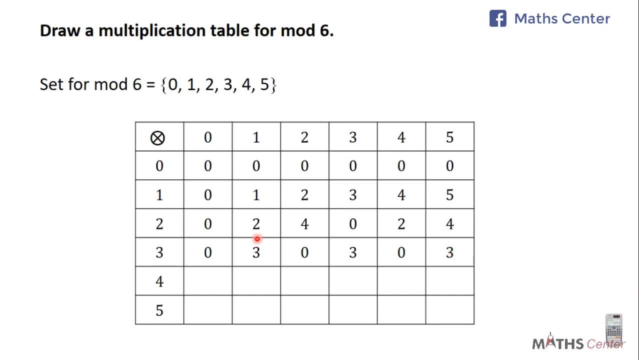 So 15 in most 6 is 3. is 3.. Let's move on to the next rule. 4 times 0 is 0.. 0 minus 6 is 6.. 4 times 1 is 4.. 4 minus 6. 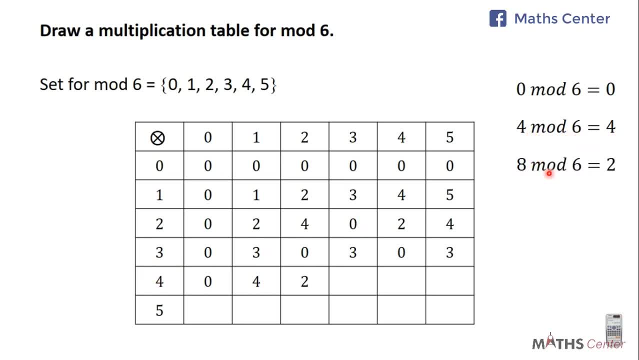 is 4.. 4 times 2 is 8.. 8 minus 6 is 2.. 4 times 3 is 12.. 12 minus 6 is 0.. 4 times 4 is 16.. 16 minus 6. 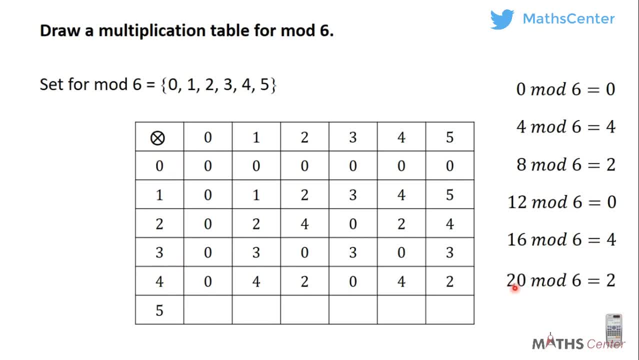 is 4.. 4 times 5 is 20.. 20 minus 6 is 2, because 20 divided by 6 will give us 3 remainder 2.. Let's move on to the last rule We have: 5 times 0.. 5 times 0 is 0.. 0 minus 6 is 6.. 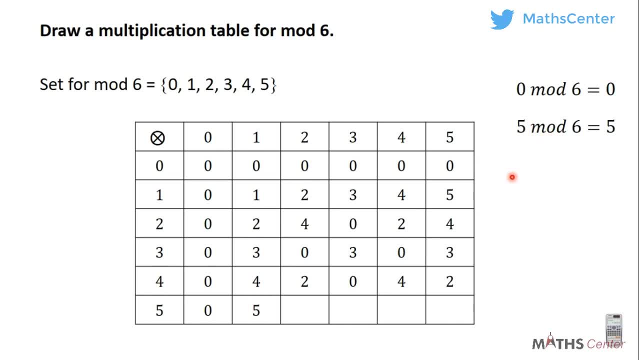 5 times 1 is 5.. 5 minus 6 is 5.. 5 times 2 is 10.. 10 minus 6 is 4.. 5 times 3 is 15.. 5 times 3 is 6.. 5 times 3 is 5.. 5 minus 6 is 6.. 5 minus 6 is 5.. 5 times 1 is 5. 5 minus. 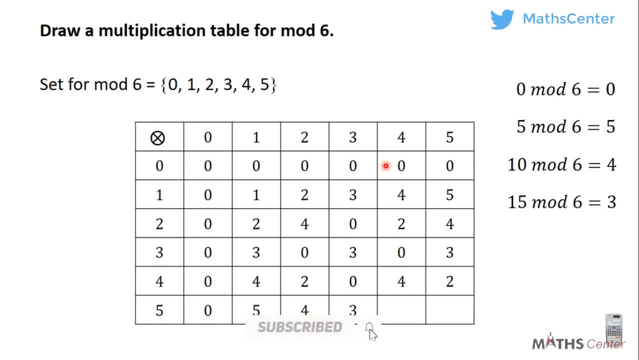 15.. 15 mod 6 is 3.. 5 times 4 is 20.. 20 mod 6 is 2.. And finally, 5 times 5 is 25.. 25 mod 6 is 1, because 25 divided by 6 will give us 4 remainder 1.. I'm going to show you a very simple trick: that. 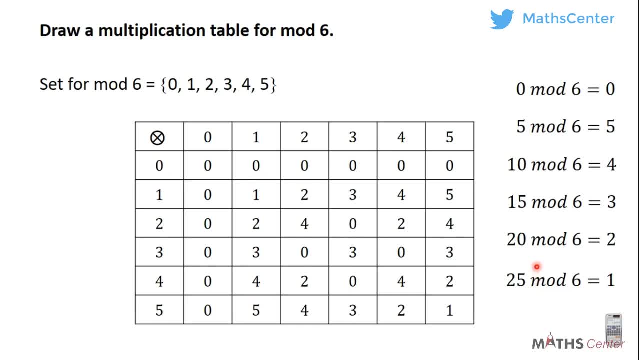 you can use to find a value when the number is bigger than the modulus. So, for example, when you have 25 mod 6, we can see that 25, which is the number, is bigger than 6, which is the modulus. I'm going to show you a trick that you can use: You subtract the modulus from the number. 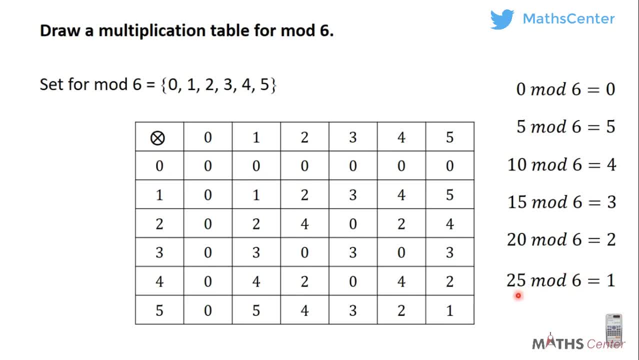 and you keep on subtracting until you get a number that is less than the modulus. This is what I mean. You want to find 25 mod 6.. You switch on your calculator, Subtract 6 from 25.. So you have 25 mod 6.. You subtract 6 from 25 mod 6.. You subtract 6 from 25 mod 6. You subtract 6 from. 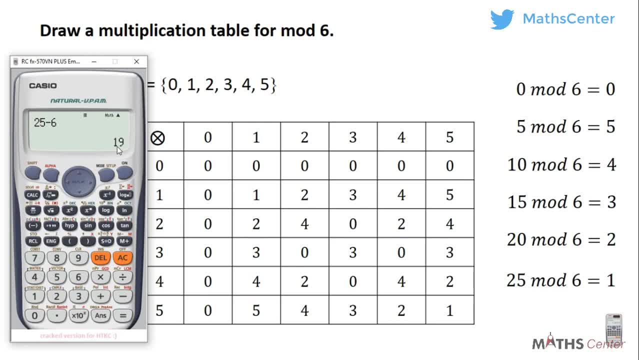 25 mod 6. This will give us 19.. 19 is bigger than the modulus which is 6.. So you subtract 6 from 19 again, So 19 minus 6.. And that will give us 13.. 13 is still bigger than the modulus, which is 6.. 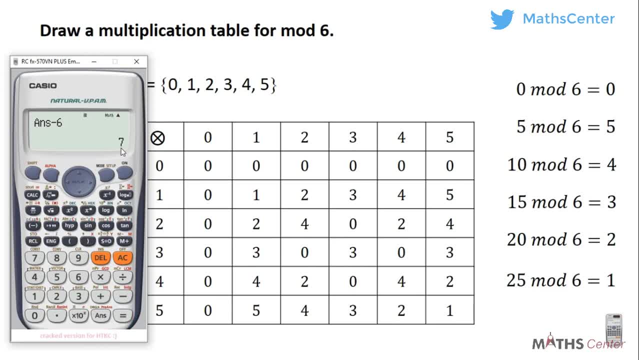 So you subtract 6 again. 13 minus 6 will give us 7.. 7 is still bigger than the modulus, which is 6.. So you subtract 6 again And you have 1.. Now 1 is less than the modulus, which is 6.. So it means that 25 mod 6 is 1.. Let's try for another example. 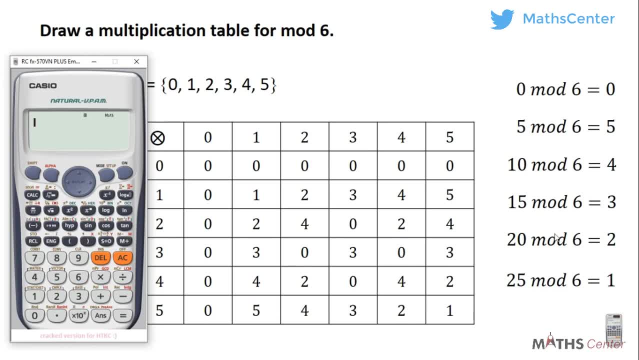 Let's say 20 mod 6.. So we are going to subtract 6 from 20 until we get a number that is less than 6.. So you have 20 minus 6.. 20 minus 6 will give us 14.. 14 is not less than 6.. So you subtract 6 from 14.. 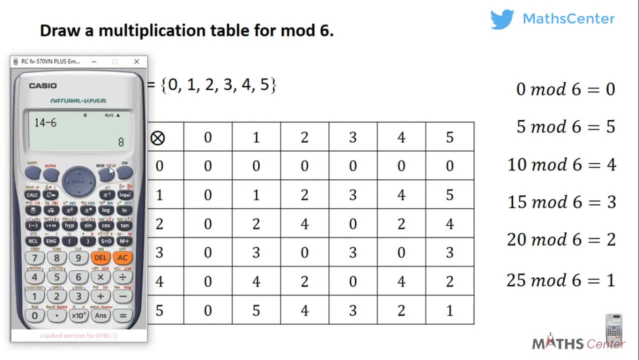 14.. 15 minus 6 will give us 8.. 8 is still not less than 6. So you subtract 6 from it again. 8 minus 6, as we all know, will give us 2.. So we can see that 20 mod 6 will give us 2.. 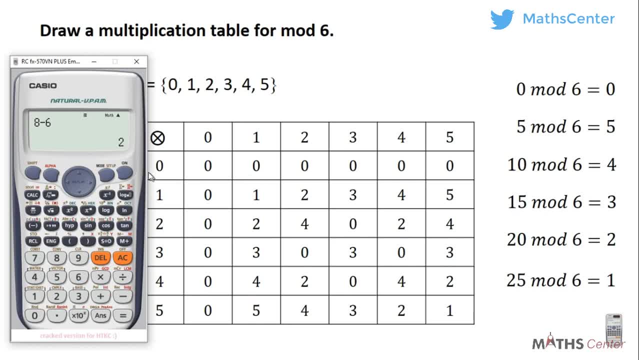 Let's try for another example. Let's say 15 mod 6.. 15 mod 6.. So you subtract 6 from 15 until you get a number that is less than 6. You have 15 minus 6. And that will give us 9.. 9 is not less than 6. So you subtract 6 from it again. 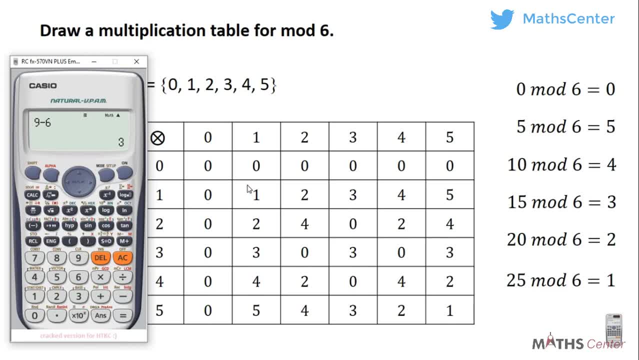 9 minus 6,, as you all know, will give us 3.. So it means that 15 mod 6 will give us 3.. Let's try for 10 mod 6.. 10 is bigger than the modulus, 10 is the number and 6 is the modulus. 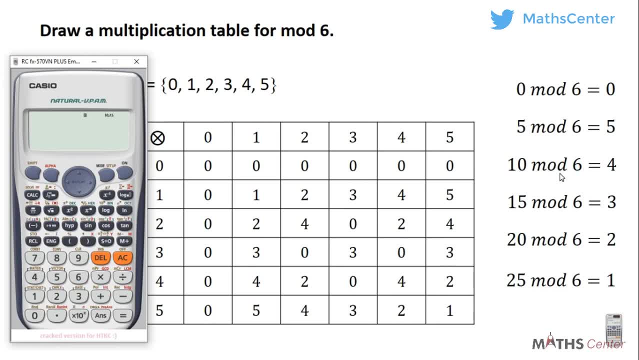 And you can see that 10 is bigger than 6.. So to find 10 mod 6,, if you want to use this trick, all you have to do is to subtract 6 from 10.. 10 minus 6 will give us 4.. 4 is less than 6.. So it means that 10 mod 6 is 4.. 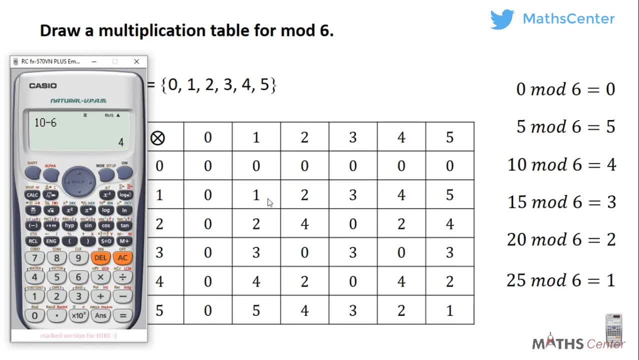 So when the number is bigger than the modulus, you can use this simple trick to find the value of that number in the modulus. You subtract the modulus from the number until you get a value that is smaller than the modulus. This trick can be very helpful when you're drawing addition. 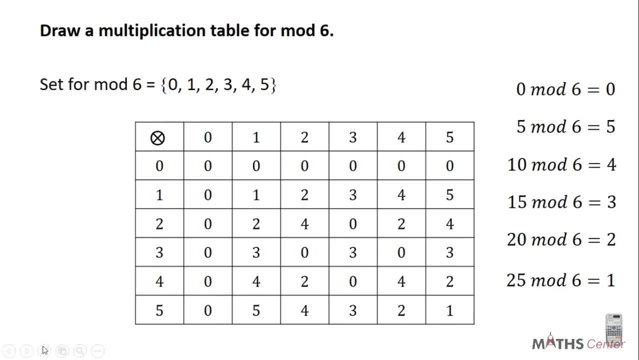 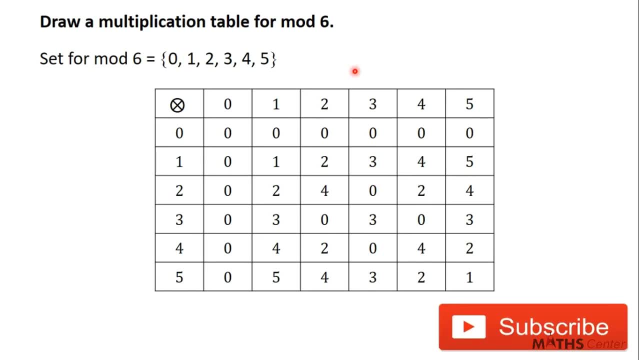 and multiplication tables in modular arithmetic. Let's go back to our question. So you have now completed the multiplication table for mod 6.. Thank you for watching this video. Subscribe to this channel for more videos. In the two examples that you have considered so far, that was the example in the previous. 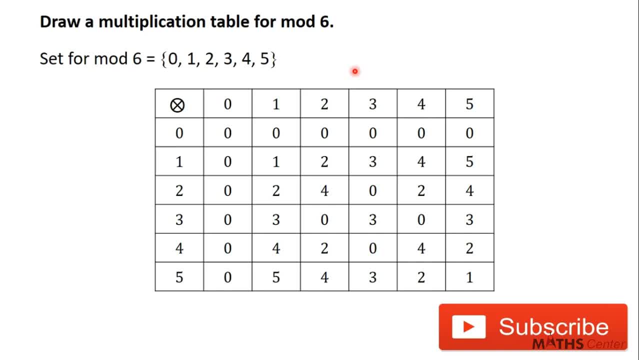 video and the one in this video, We were asked to draw an addition table or multiplication table for a particular modulus. So we defined the set of values in that modulus and we used it to draw the table. Sometimes The set of values that you are going to use to draw the table will be defined for you. 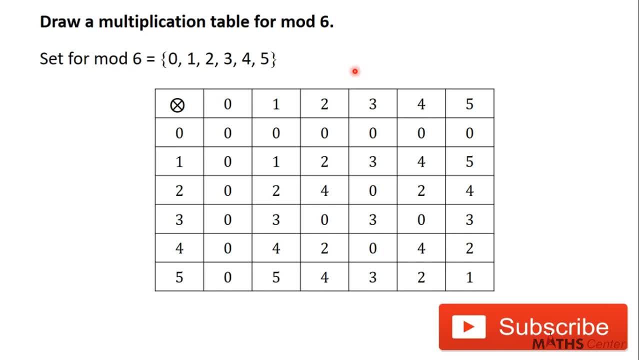 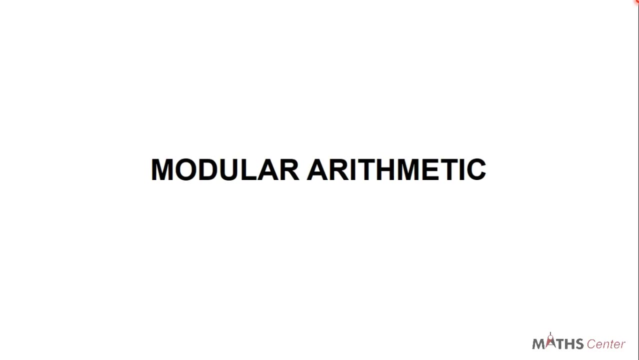 In the next video we are going to solve a question on drawing a table for an operation in a given modulus When the set of values have been defined for you. Bye-bye, Welcome back. We are on the topic: Modular Arithmetic. In the previous video, we solved a question on drawing a table for an operation in a given modulus. 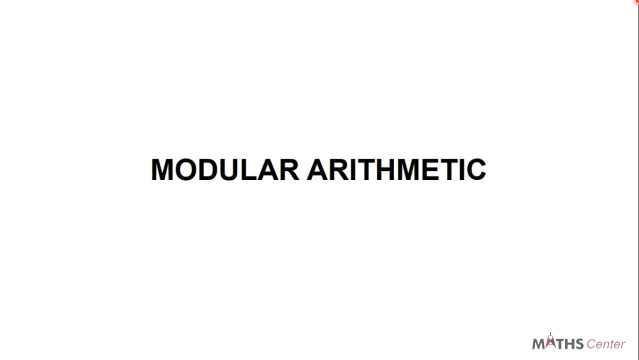 In this video we are going to solve a question on drawing a table for an operation in a given modulus When the set of values have been defined for you. The question for this video is: draw a multiplication table for mode 7 on the set 2,, 3,, 5,, 6.. 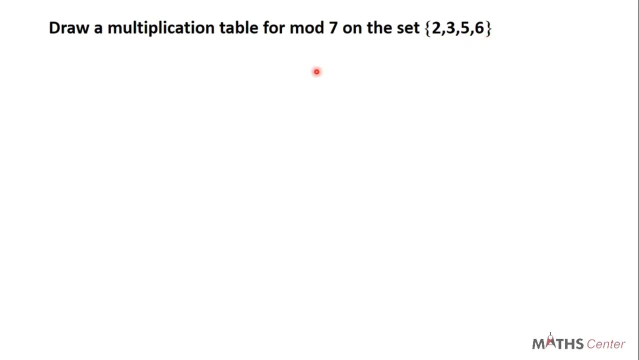 So in this question the set of values that we are going to use in the table Have been defined for us. This is quite different from the questions that we have solved in the previous videos. In those questions we are asked to draw a multiplication or addition table for a particular modulus. 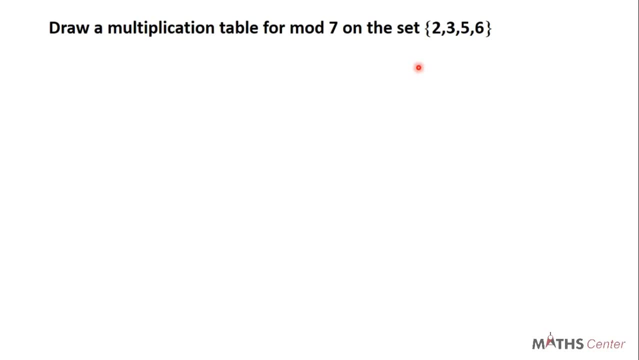 So we list the set of values used in that modulus And then we use that set to draw the table. So, for example, if the question had asked us to draw a multiplication table for mode 7. The first thing we will do is that. 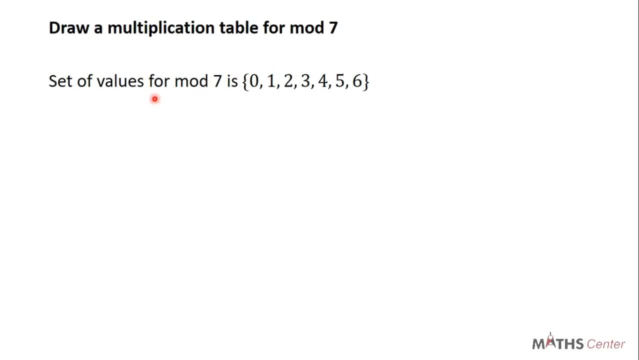 We will define the set of values used in mode 7.. The set of values used in mode 7 are 0,, 1,, 2,, 3,, 4,, 5, 6.. Then we will use this set of values to draw the table. 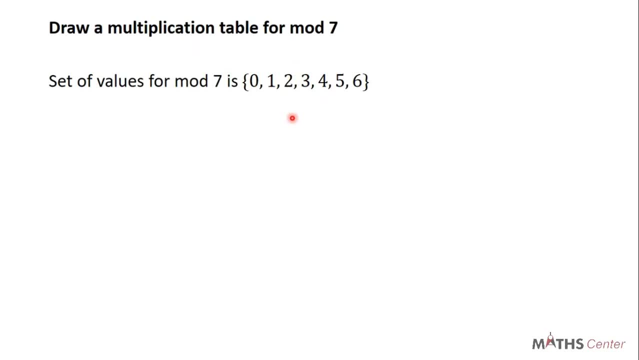 After that we will multiply the numbers in mode 7.. This time the question is asking us to draw a table for mode 7 on the set 2,, 3,, 5, 6.. So the set of numbers that we are supposed to use in the table have been given to us. 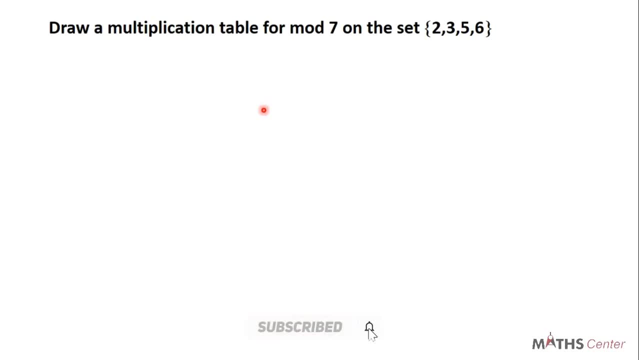 This means that when you are asked to draw a table for an operation in a given modulus And you are given a set of values in the question, You have to use that set of values to draw the table. So for this question, we are going to use the values in this set to draw the table. 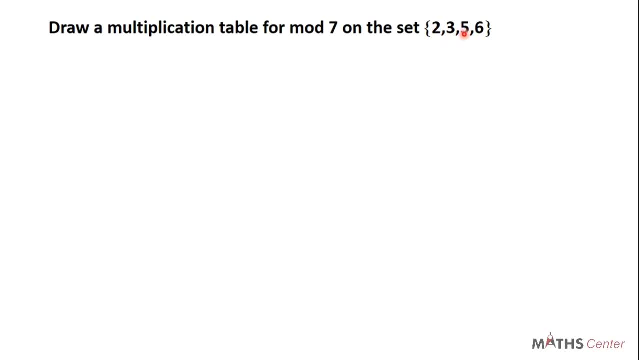 We have 4 values in this set: 2,, 3,, 5, 6.. So we are going to use that set of values to draw the table. We are going to draw a table with 5 columns and 5 rows. 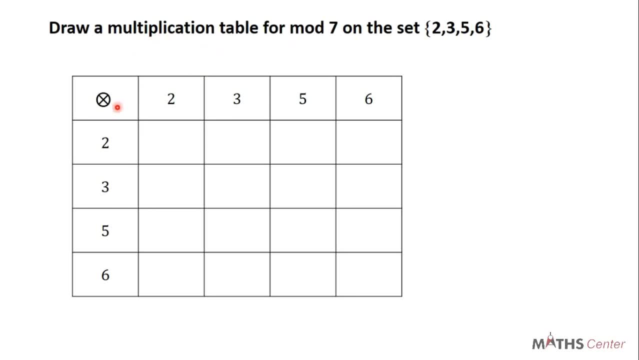 We are going to draw a multiplication table for mode 7.. So the operation is multiplication. You write the multiplication sign in the first cell and then you draw a circle around it. After that you list the numbers in the first row and the first column. 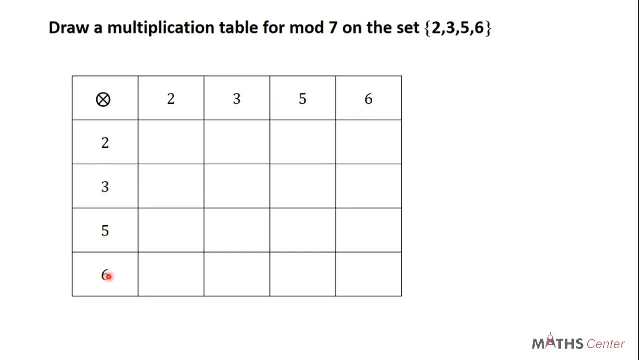 So we have 2,, 3,, 5,, 6.. 2,, 3,, 5,, 6.. We are going to multiply these numbers in mode 7.. So we begin with the first one: 2 times 2.. 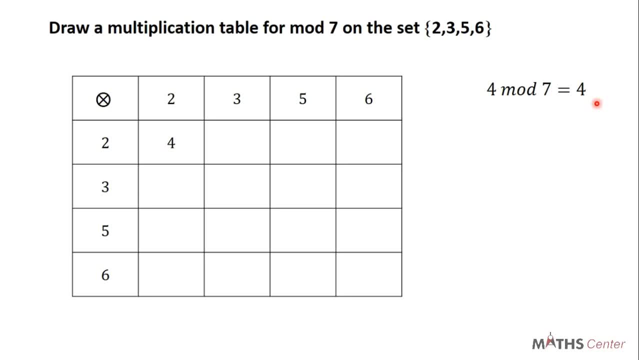 2 times 2 is 4.. 4 in mode 7 is 4.. 2 times 3 is 6.. 6 in mode 7 is 6.. 2 times 5 is 10.. 10 in mode 7 is 3.. 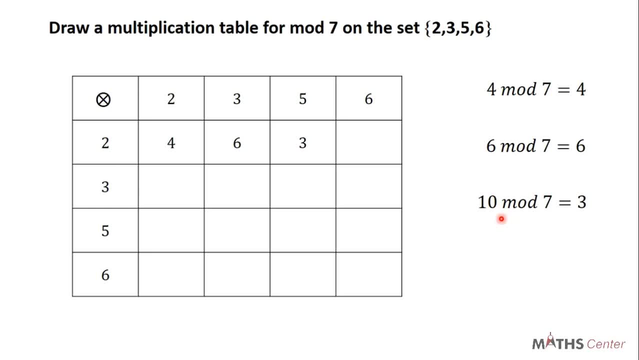 In the previous video I showed you a simple trick you can use to find a value when the number is bigger than the modulus. I said that You just have to subtract the modulus from the number until you get a value that is smaller than the modulus. 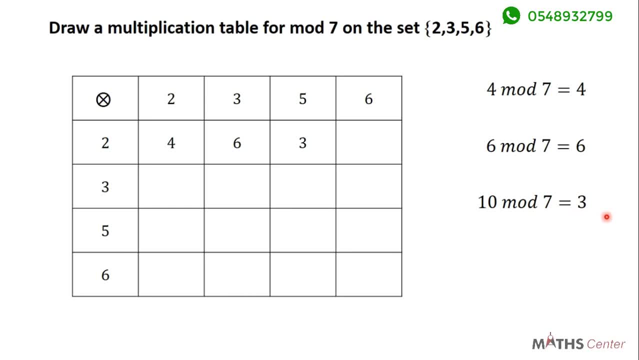 So here we will subtract 7 from 10. 10 minus 7 will give us 3.. 3 is smaller than the modulus, which is 7.. So it means that 10 in mode 7 is 3.. Let's move on. 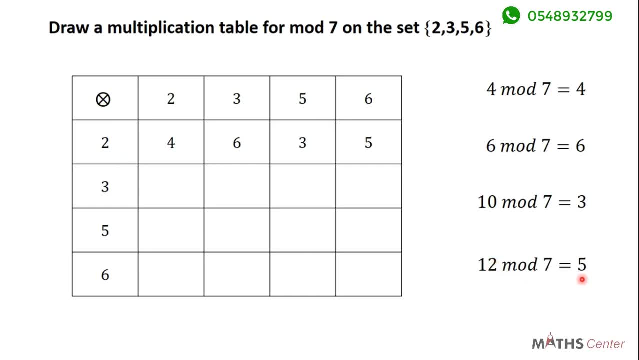 2 times 6 is 12.. 12 in mode 7 is 5.. So when you subtract 7 from 12, you are going to get 5.. 5 is smaller than the modulus. So 12 mod 7 is 5. let's move on to the next rule. 3 times 2 is 6. 6 mod 7 is 6. 3 times 3 is 9. 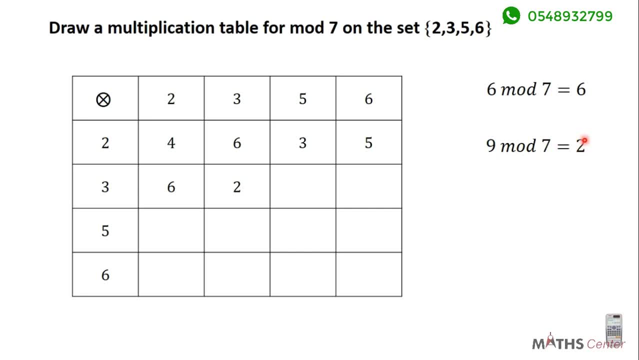 9 mod 7 is 2. so you subtract 7 from 9 and you get 2, and 2 is smaller than the modulo. so nine mod seven is two. three times five is fifteen. fifteen mod seven is one. fifteen is bigger than the modulo of such a seven. so you can use the trick that i showed you in the previous video. 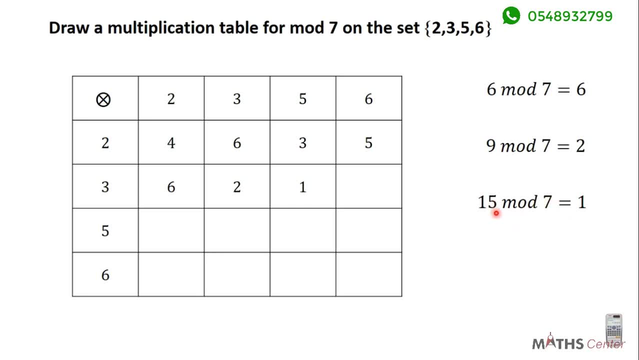 to find fifteen mod seven. you subtract seven from fifteen. fifteen minus seven will give us eight. eight is still bigger than the modulo, just seven. so you subtract seven from eight. again, eight minus seven will give us one. so fifteen mod 7 is 1.. Let's move on. We have 3 times 6.. 3 times 6 is 18.. 18 mod 7 is equal to 4.. 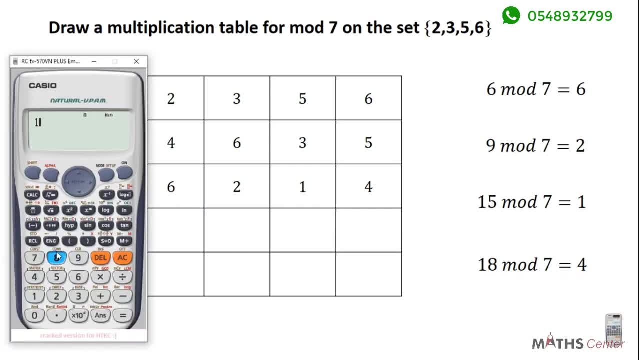 So you subtract 7 from 18.. 18 minus 7 will give us 11.. 11 is still not smaller than the modulo, so you subtract 7 from 11 again. So 11 minus 7 will give us 4. It means that 18. 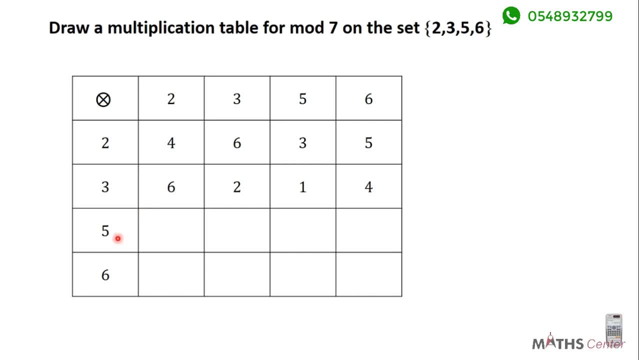 mod 7 is 4.. Let's move on to the next rule. 5 times 2 will give us 10.. 10 mod 7 is 3.. You subtract 7 from 10, you get 3.. 5 times 3 will give us 15.. 15 mod 7 is 1.. You subtract. 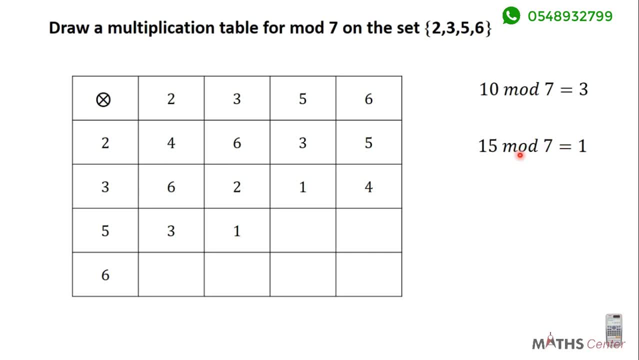 7 from 15, you get 8.. Then you subtract 7 from 8, you get 1.. So you keep on subtracting until you get a value that is smaller than the modulus. Let's move on: 5 times 5 is 25.. 25 mod 7 is 4.. You subtract 7 from 25 and you get 18.. Then you subtract. 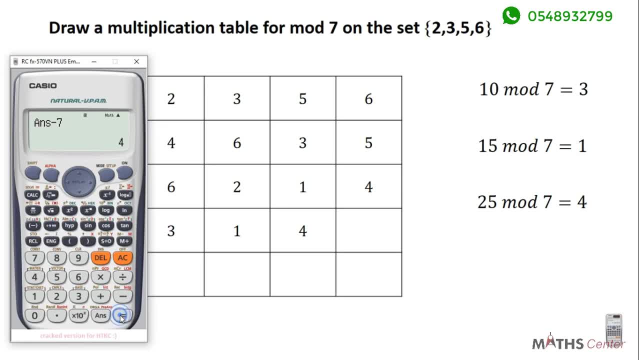 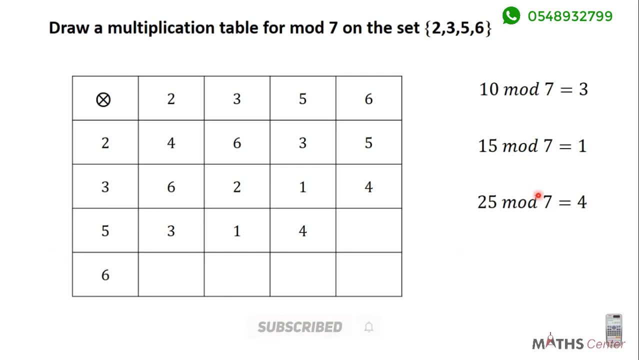 7 from 18, you get 11.. You subtract 7 from 11 and you get 4.. So you keep on subtracting until you get a number that is smaller than the modulus. 25 mod 7 will give us 4. 5 times. 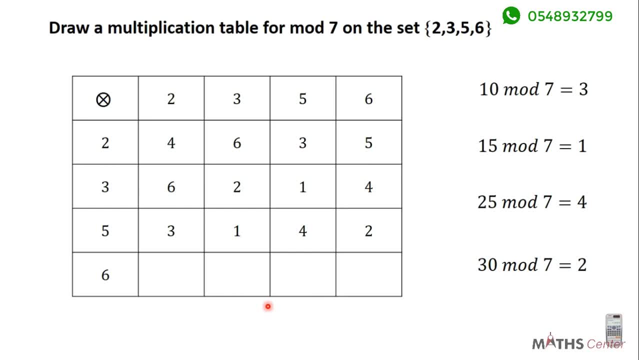 6 will give us 30.. 5 times 6 is 3.. 5 times 6 is 3.. 5 times 6 is 4.. 5 times 6 is 5.. 5 times 30 mod 7 is 2. so once again you subtract 7 from 30, so we have 30 minus 7 and that 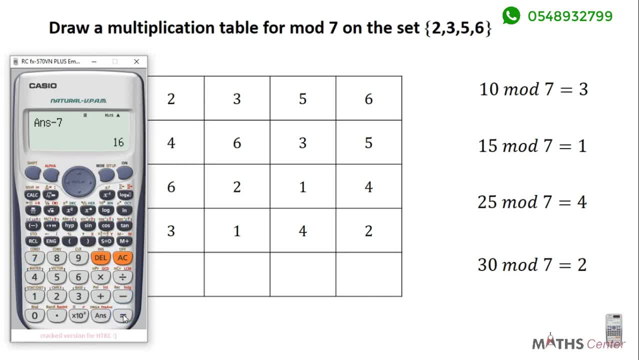 will give us 23. you subtract 7 from 23, that will give us 16. you subtract 7 from 16, you have 9. then you subtract 7 from 9 and you have 2, so it means that 30 mod 7. 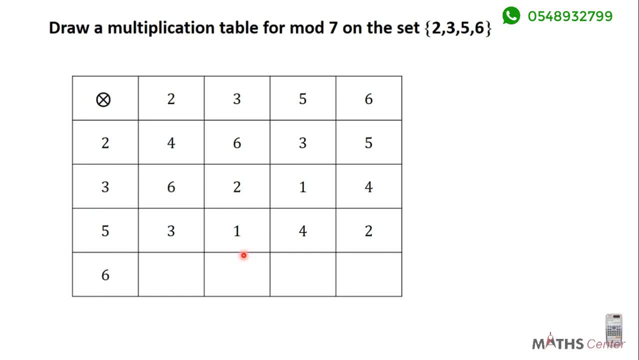 is 2. let's move on to the last rule. 6 times 2 will give us 12. 12 mod 7 is 5. you subtract 7 from 12 and you get 5. 5 is smaller than the modulus, so 12 mod 7. 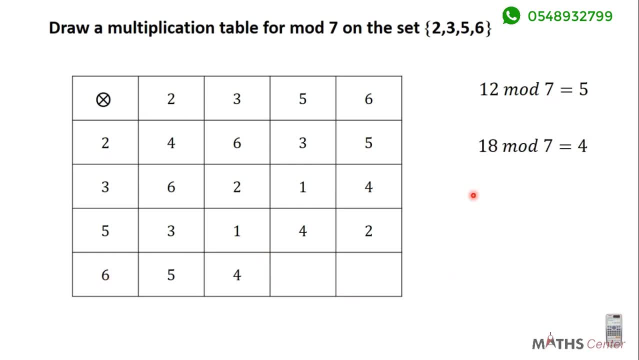 is 5, 6 times 3 is 18. you subtract 7 from 18 and you get 11. you subtract 7 from 11, you get 4. so 18 mod 7 is 4. 6, 6 times 5 is 30,, 30 mod 7 is 2 and finally, 6 times 6 is 36, 36 mod 7 is 1.. 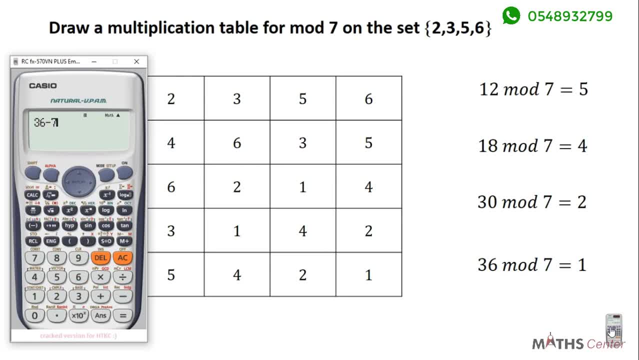 You subtract 7 from 36, so you have 36 minus 7, and that will give us 29.. You subtract 7 from 29, and that will give us 22.. You subtract 7 from 22, that will give us 15.. 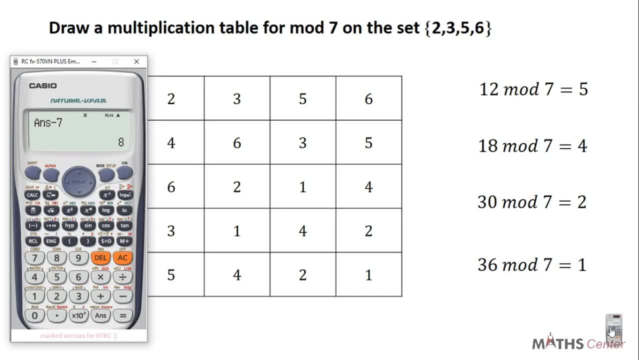 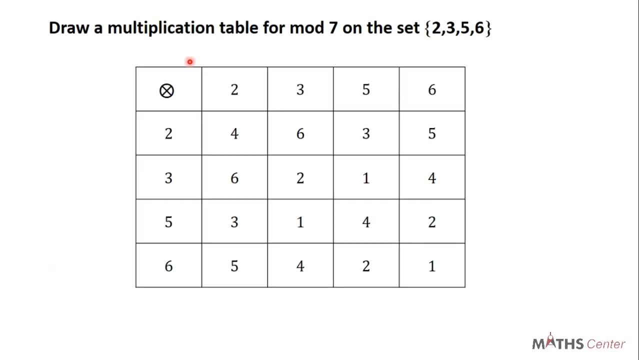 You subtract 7 from 15, you have 8. then you subtract 7 from 8 and you have 1.. So 36 mod 7 is 1.. We have now completed our multiplication table for mod 7 on the set 2,, 3,, 5,, 6.. 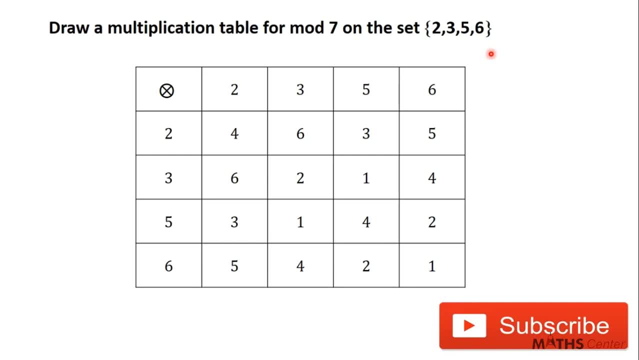 Thank you for watching this video. Subscribe to this channel for more videos. In the next video we are going to solve another question on drawing a table for an operation in a given modulus when the set of values have been defined for you. Bye-bye. 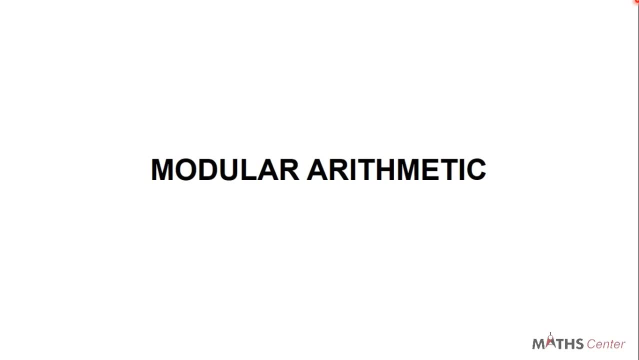 Welcome back. We are still on the topic modular arithmetic. In the previous video we solved a question on drawing a table for an operation in a given modulus where the set of values have been defined for you. In this video we are going to solve another question. 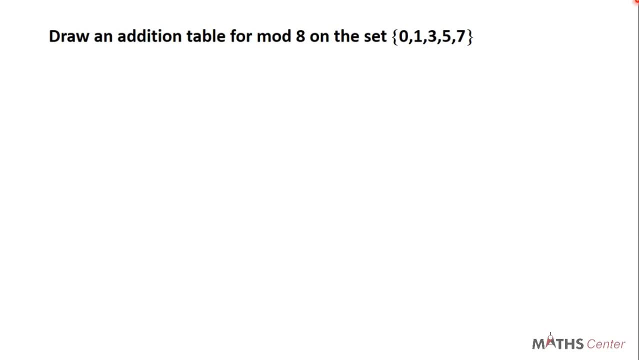 The question for this video is: Draw an addition table for mod 8 on the set 0,, 1,, 3,, 5, 7.. We learnt in the previous video that when you are asked to draw a table for an operation, 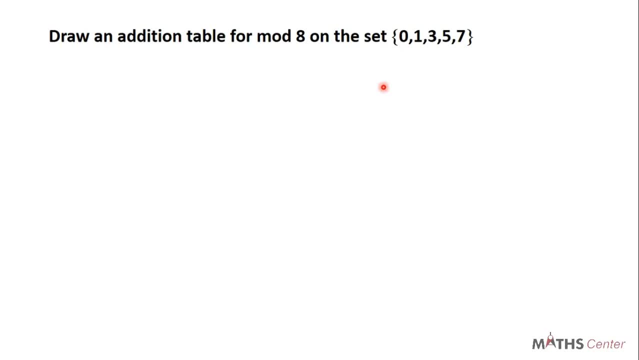 in a given modulus and the question defines the set of values for you. you are supposed to use that set of values to draw the table Here. the question is asking us to draw an addition table for mod 8 on the set 0, 1,. 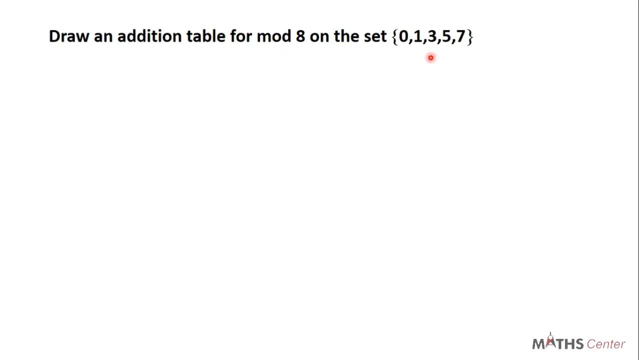 3,, 5,, 6.. So we are going to use the numbers 0,, 1,, 3,, 5,, 7 to draw the table. We have 5 numbers here, so we are going to draw a table with 6 columns and 6 rows. 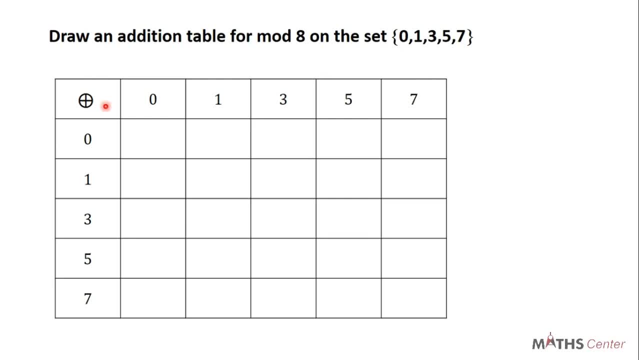 In the first cell you indicate the sign of the operation you are going to perform. We are going to draw an addition table, So you write the addition sign in the first cell And then you draw a circle around it. After that you list the set of numbers in the first row and the first column. 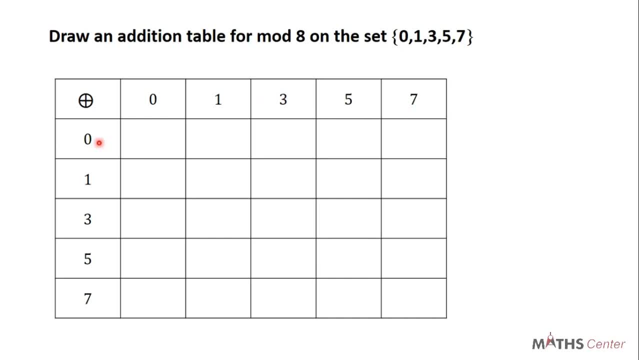 So we have 0,, 1,, 3,, 5, 7 and 0, 1,, 3,, 5,, 7.. We are drawing an addition table for mod 8.. So we will add the numbers in mod 8.. 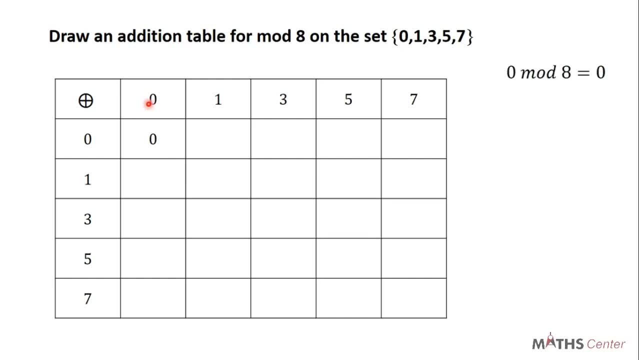 The first one is 0 plus 0.. 0 plus 0 is 0.. 0 in mod 8 is 0.. 0 plus 1 is 1.. 1 in mod 8 is 1.. 0 plus 3 is 3.. 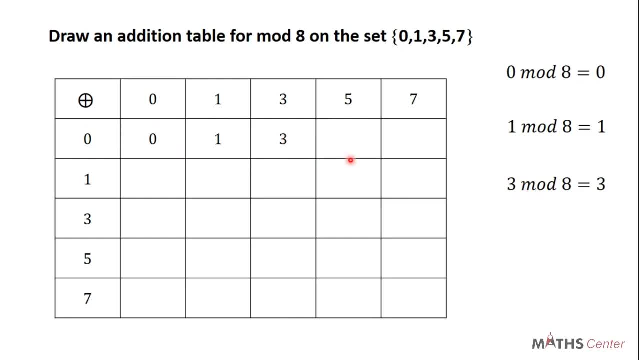 3 in mod 8 is 3.. 0 plus 5 is 5.. 5 in mod 8 is 5.. 0 plus 7 is 7.. 7 in mod 8 is 7.. We move on to the next rule. 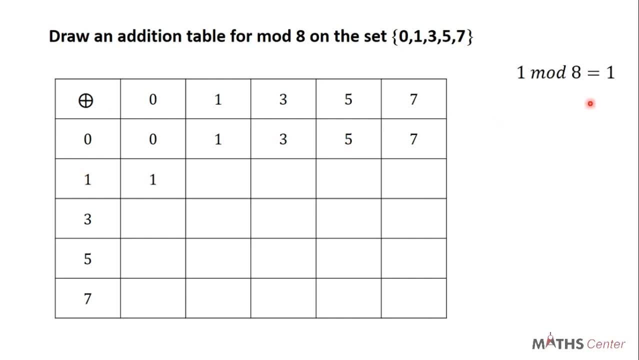 1 plus 0 is 1.. 1 in mod 8 is 1.. 1 plus 1 is 1.. 1 in mod 8 is 1.. 1 plus 1 is 2.. 2 in mod 8 is 2.. 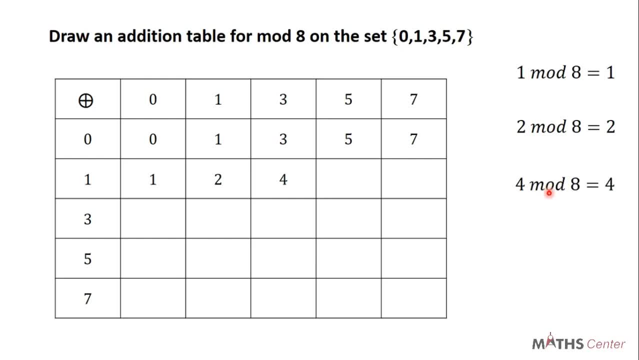 2 in mod 8 is 2.. 1 plus 3 is 4.. 4 in mod 8 is 4.. 1 plus 3 is 4.. 4 in mod 8 is 4.. 1 plus 5 is 6.. 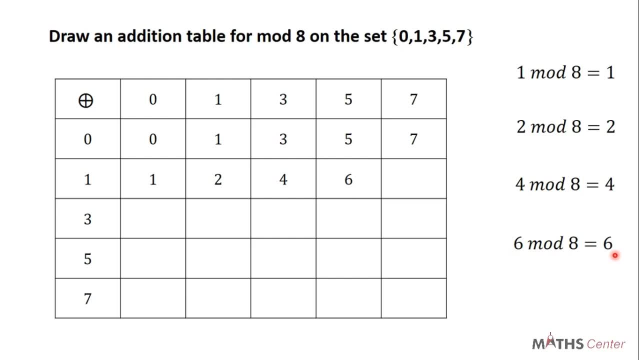 1 plus 5 is 6.. 6 in mod 8 is 6.. 6 in mod 8 is 6.. 1 plus 7 is 8.. 1 plus 7 is 8.. 8 in mod 8 is 0.. 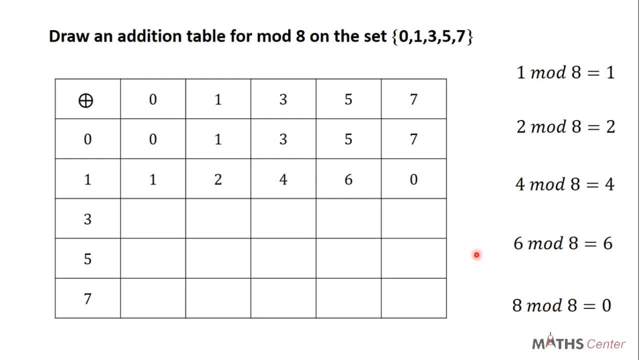 8 in mod 8 is 0.. 8 in mod 8 is 0.. Let's move on to the next rule. 3 plus 0 is 3.. 3 in mod 8 is 3.. 3 plus 0 is 3.. 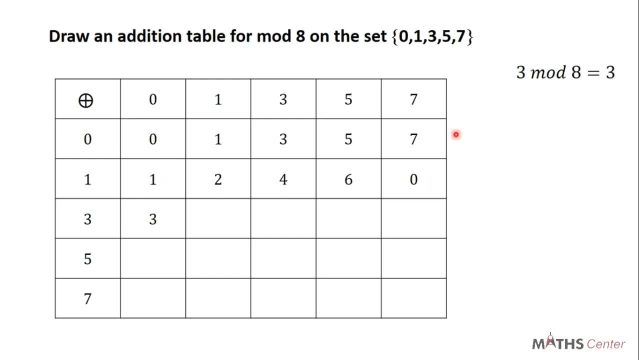 3 in mod 8 is 3.. 3 plus 1 is 4.. 3 in mod 8 is 4.. 3 plus 1 is 4.. 4 in mod 8 is 4.. 1 is 4.. 4 in mode 8 is 4.. 3 plus 3 is 6.. 6 in mode 8 is 6.. 3 plus 5 is 8.. 8 in mode 8. 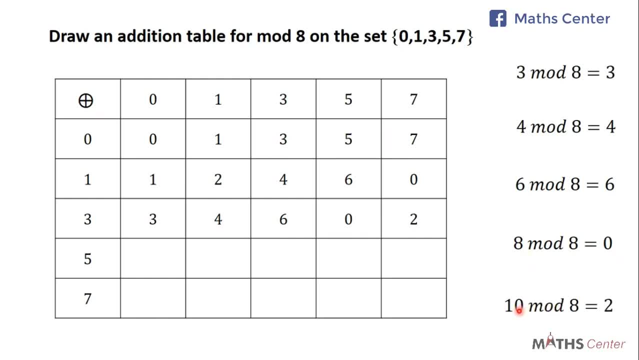 is 0.. 3 plus 7 is 10.. 10 in mode 8 is 2.. The number which is 10 is greater than the modulus 8.. So you divide 10 by 8 and that will give us 1 remainder 2.. So 10 mode 8 is equal to. 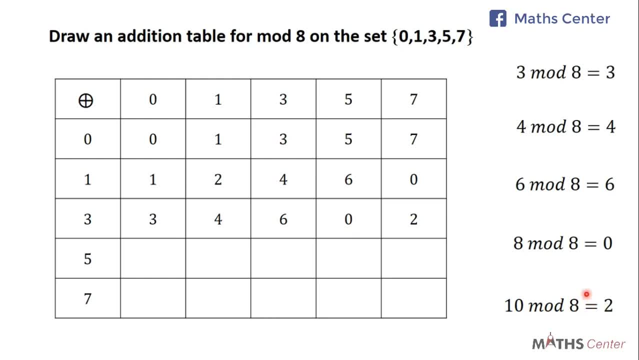 the remainder, which is 2.. You can also use the trick that I showed you in the previous video. You subtract 8 from 10.. 10 minus 8 will give us 2.. 2 is less than the modulus, so 10 mode 8 is equal to 2.. Let's move on to the next rule. 5 plus 0 is 5.. 5 mode 8. 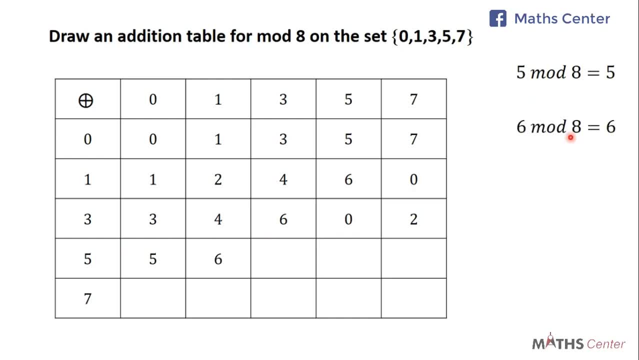 is 5.. 5 plus 1 is 6.. 6. mode 8 is 6.. 5 plus 3 is 8.. 8. mode 8 is 0.. 5 plus 5 is 10.. 10. mode 8 is 2.. 5 plus 7 is 12.. 12. mode 8 is 4.. 12 is greater. 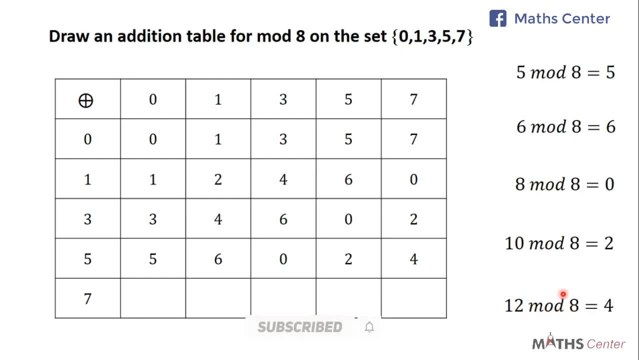 than the modulus, which is 8.. So you divide 12 by 8 and you have 1 remainder, 4.. Or you can use the trick we learnt in the previous video: You subtract 8 from 12 and that will give us 4.. 4 is less than the modulus, which is 8.. So 12 mode 8 is 4.. 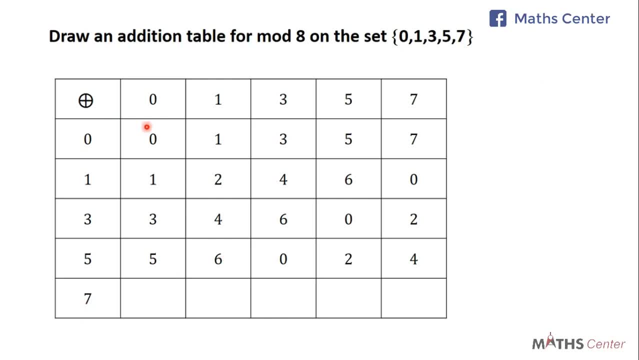 Let's move on to the last rule. 7 plus 0 is 7.. 7 mode 8 is 7.. 7 plus 1 is 8.. 8 mode 8 is 0.. 7 plus 3 is 10.. 10 mode 8 is 2.. 7 plus 5 is 12.. 12 mode 8 is 4.. And finally, 7 plus. 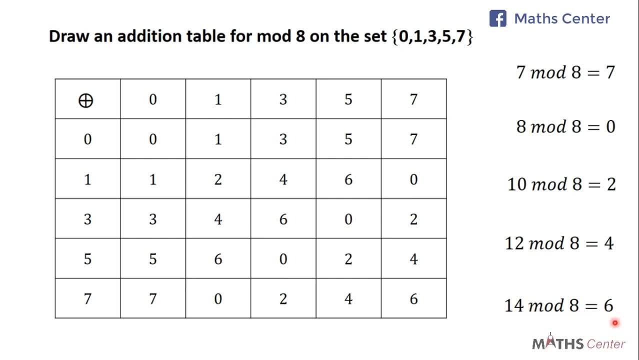 7 is 14.. 14 mode 8 is 8.. 14 is greater than the modulus which is 8.. 14 is greater than the modulus which is 8.. So you divide 14 by 8.. 14 divided by 8 will give us 1 remainder. 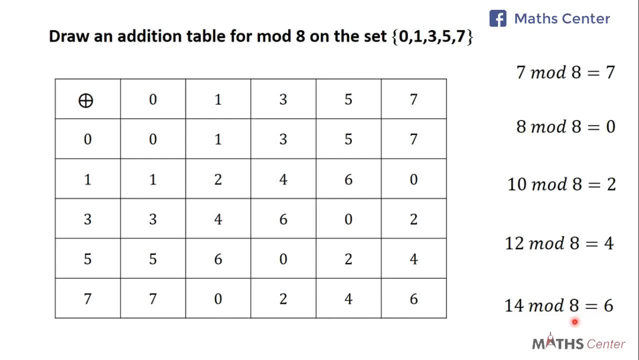 6. So 14 mode 8 is 6.. Or you can use the trick we learnt in the previous video: You subtract 8 from 14 and that will give us 6.. 6 is less than the modulus, which is 8.. So 14 mode 8. 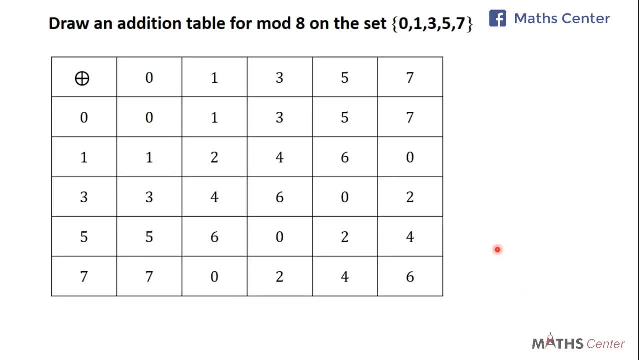 is 6.. We have now completed our addition table for mode 8 on the set 0,, 1,, 3,, 6.. Thank you for watching this video. Subscribe to this channel for more videos. So far, we have solved four questions on drawing a table for an operation in a given modulus. 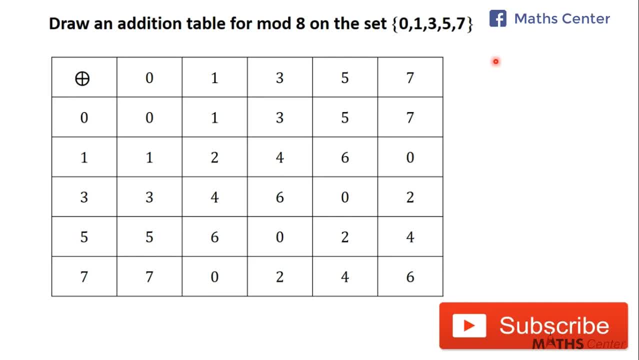 Sometimes, after drawing the table, you may be asked to use your table to answer some questions. In the next video we are going to solve another question on drawing a table for an operation in a given modulus. At this time, after drawing the table, we are going to use it to answer some questions. 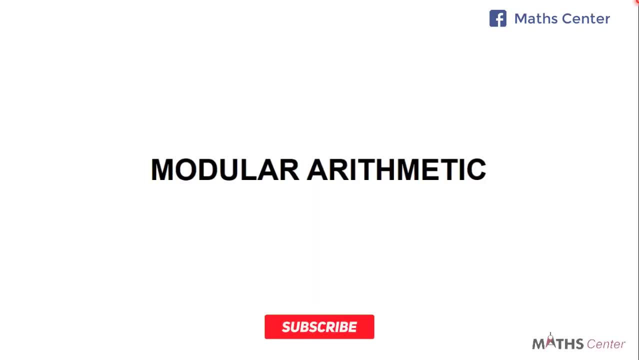 Bye-bye, Welcome back. We are still on the topic Modular Arithmetic. In the previous video we solved a question on drawing a table for an operation in a given modulus. In this video we are going to solve another question on drawing a table for an operation. 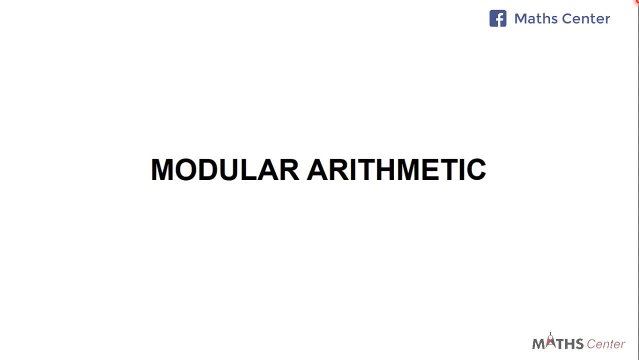 in a given modulus. After drawing the table, We are going to use it to answer some questions. The question for this video is: A- Draw an addition table for mode 5.. B- Use your table to evaluate I 2 plus 4 into brackets plus 3.. 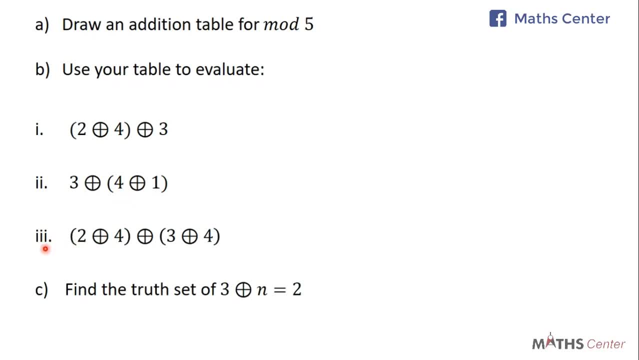 II, 3 plus into brackets 4 plus 1.. III- 2 plus 4 into brackets, plus 3 plus 4 into brackets. III, 3 plus 4 into brackets, plus 3 plus 4 into brackets C. Find a truth: set of 3 plus n is equal to 2.. 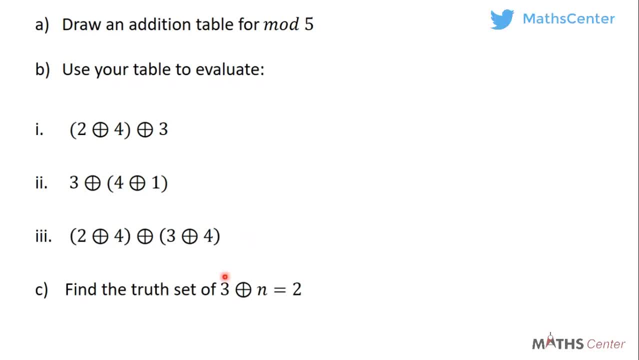 We are going to solve the first two parts of this question in this video and we will solve the last part in the next video. Let's begin with the first part: An addition table for mode 5.. The question did not define a set of values for us. 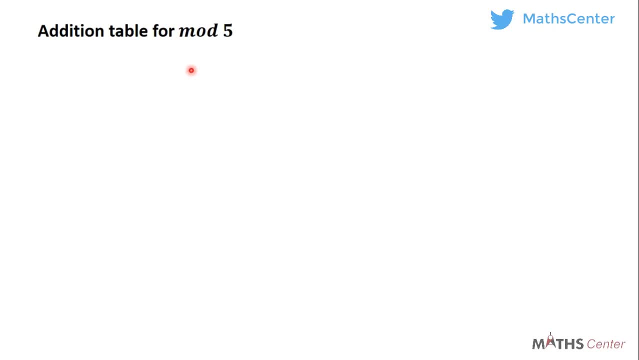 So the question did not define a set of values for us, So we are going to use the set of values in this question. a set of values in this question. So we are going to use a set of values in this question. 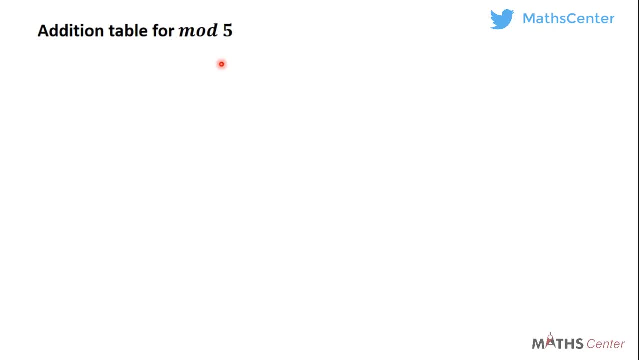 used in mode 5 to draw the table. we have learnt that in mode 5 the set of values used are 0, 1, 2, 3, 4, so we are going to use this set of values to draw our table. there are five values in total, so you draw a table with six columns and six. 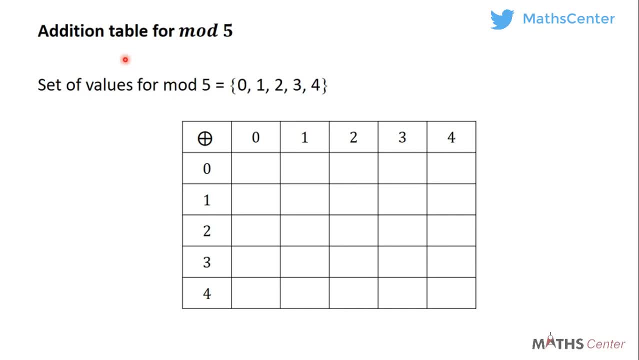 rows. we are going to draw an addition table, so the operation we are performing is addition. you write the addition sign and then you draw the circle around it. we will list the sets in the first row and the first column, just as we have in the table here. we are adding these numbers in mode 5, so you have 0 plus 0. 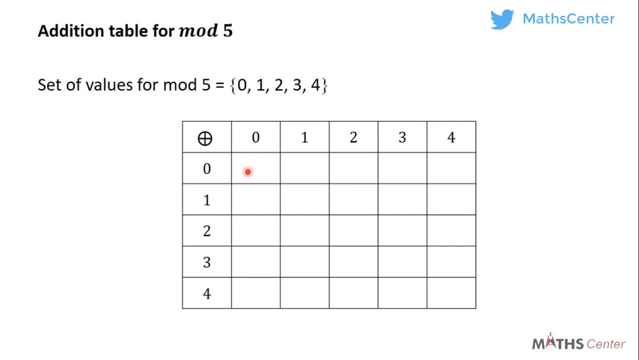 and that will give us 0. 0 in mode 5 is 0. 0 plus 1 is 0. 0 plus 1 is 1. 1 in mode 5 is 1. 0 plus 2 is 2. 2 in mode 5 is 2. 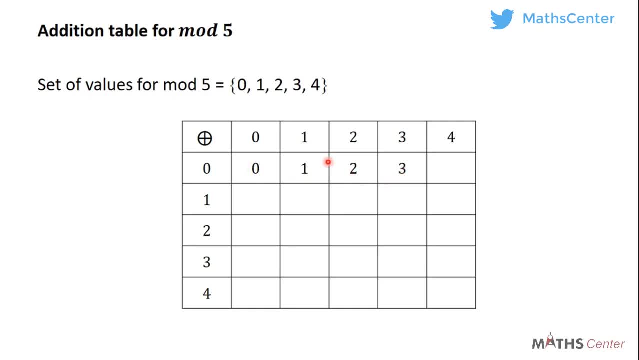 0 plus 3 is 3. 3 in mode 5 is 3. 0 plus 4 is 4. 4 in mode 5 is 4. 1 plus 0 is 1. 1 in mode 5 is 1. 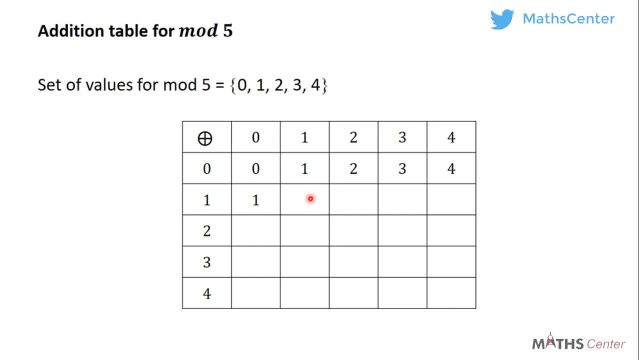 1 plus 1 is 2, 2. in mode 5 is 2. 1 plus 2 is 3, 3. in mode 5 is 2. 1 plus 2 is 3, 3. mood 5 is 3, 1 plus 3 is 4, 4. mood 5 is 4, 1 plus 4 is 5, 5. mood 5 is 0, 2 plus 0 is. 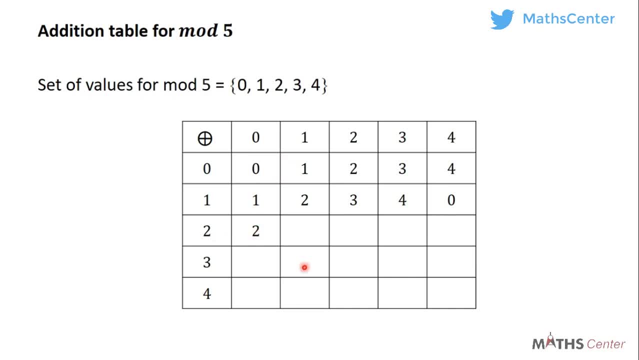 2, 2. mood 5 is 2, 2 plus 1 is 3, 3. mood 5 is 3, 2 plus 2 is 4, 4. mood 5 is 4, 2 plus. 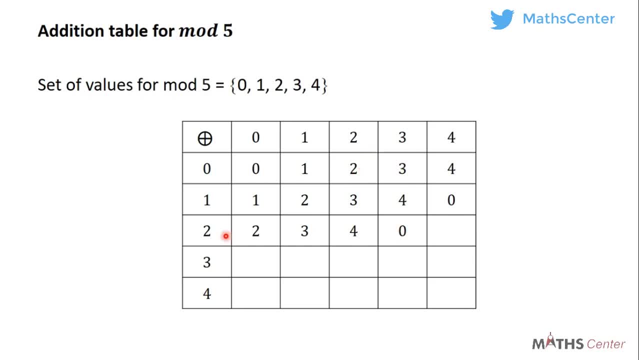 3 is 5, 5. mood 5 is 0, 2 plus 4 is 6, 6. mood 5 is 1, 3 plus 0 is 3, 3. mood 5 is 3, 3 plus. 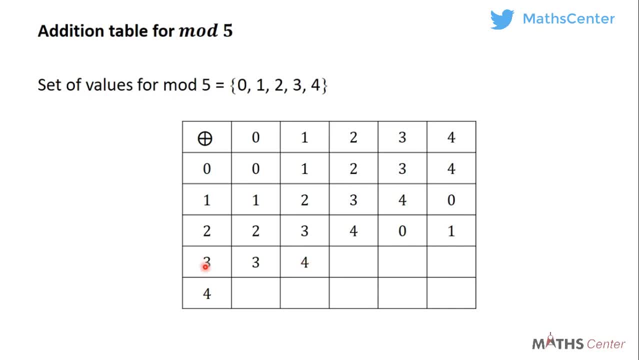 1 is 4, 4. mood 5 is 4, 3 plus 2 is 5, 5. mood 5 is 0, 3 plus 3 is 6, 6. mood 5 is 1, 3 plus. 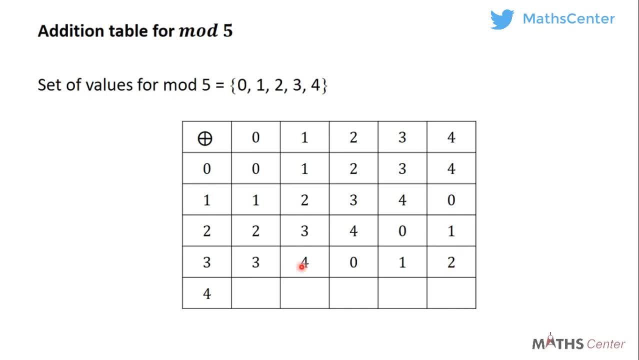 4 is 7.. 4 plus 0 is 4, 4. mood 5 is 4,. 4 plus 1 is 5, 5. mood 5 is 0,. 4 plus 2 is 6, 6 mood 5: 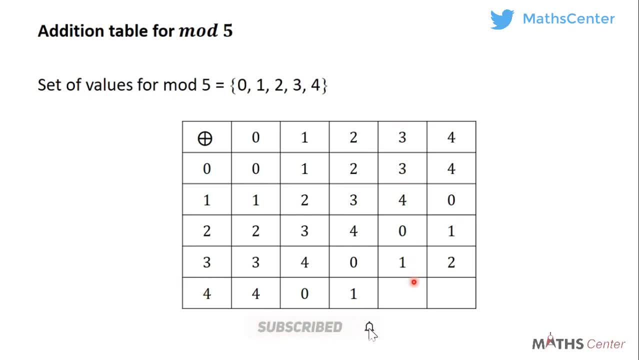 is 1,, 4 plus 3 is 7, 7 mood 5 is 2 and finally, 4 plus 4 is 8, 8 mood 5 is 3.. So we have completed our addition table. We have solved a lot of questions on drawing addition and multiplication tables for a given. 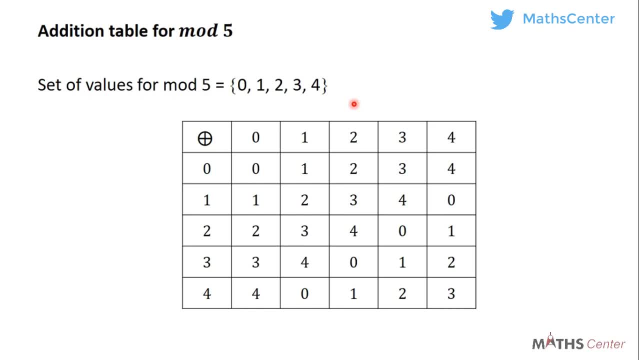 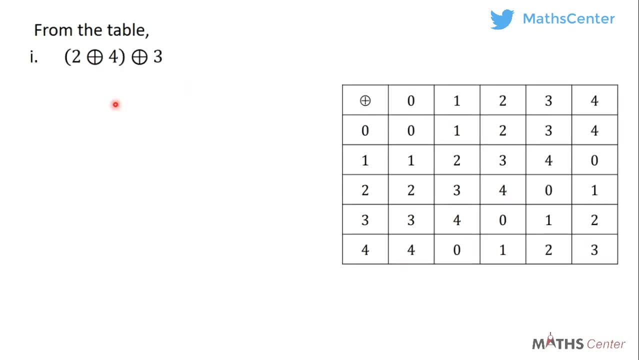 mood loss. So I am very sure that by this time you are conversant with drawing tables for an operation in a given mood loss. Let's move on to the next part of our question. The B part of the question said that we should use our table to evaluate i 2 plus 4 into. 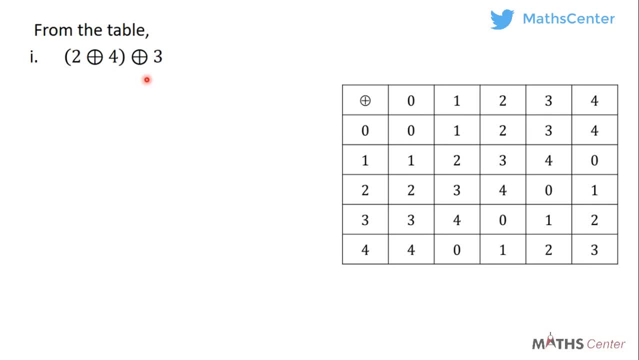 brackets plus 3.. When you are given a question like this, you will begin with the one in the brackets. so you will have to find 2 plus 4.. So you will read 2 plus 4 from the table 2 plus 4.. 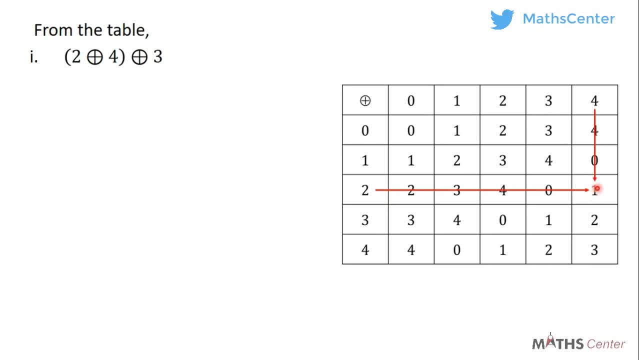 So you will trace 2 and 4 and you will see that they will meet in this cell. This means that from the table, 2 plus 4 is equal to 1.. So 2 plus 4 is now 1, so this becomes 1 plus 3.. 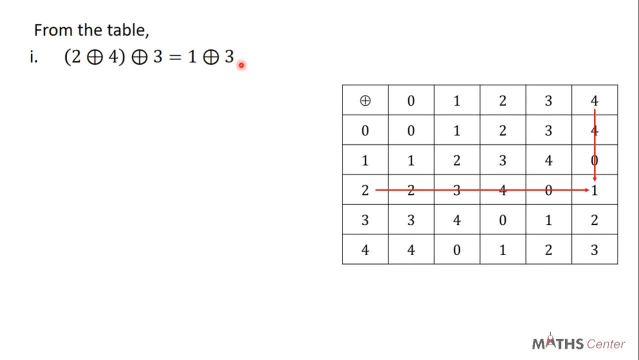 What is in the brackets is 1, so you have 1 plus 3.. So you will now have to read 1 plus 3 from the table 1 plus 3.. You will trace 1 and 3 and you will see that they will meet in this cell. 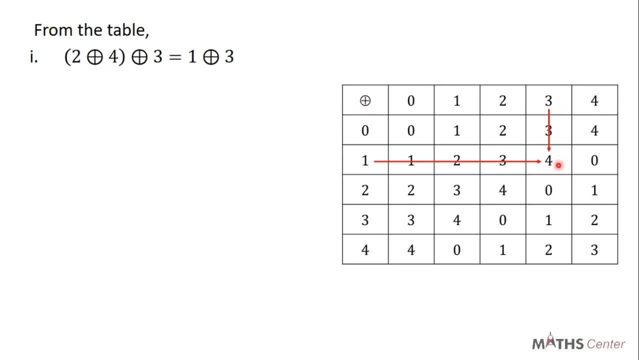 So it means that from the table, 1 plus 3 is equal to 4.. Note that in an examination you don't have to draw the arrows in the table as I have done here. I drew them to show you how to pick the values from the table. 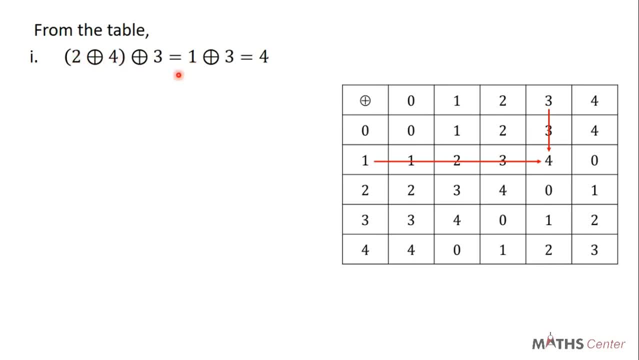 2 plus 4 will give us 1.. So you will have 1 plus 3, and 1 plus 3 from the table is equal to 4.. Let's move on: III, 3 plus into brackets, 4 plus 1.. 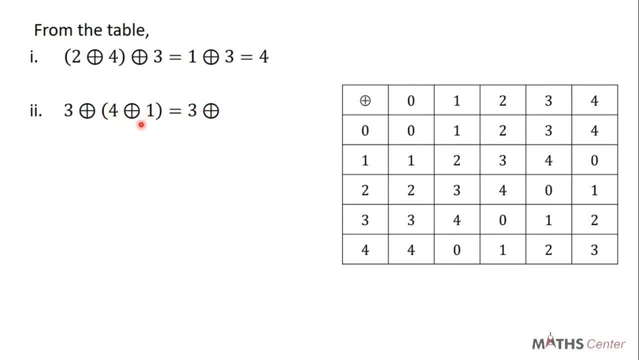 This will give us 3 plus then what we have in the brackets. What we have in the brackets is 4 plus 1.. So you will read 4 plus 1 from the table 4 plus 1.. From the table: 4 plus 1 will give us 0.. 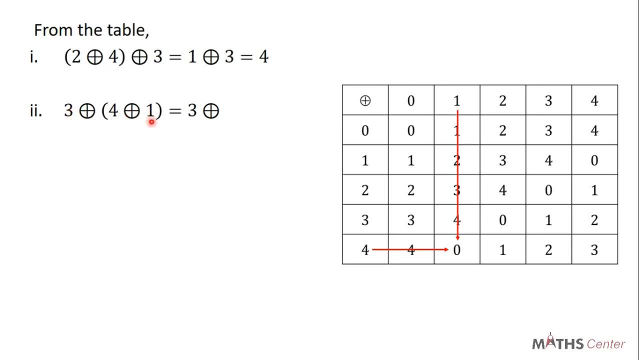 It means that this will become 3 plus 4 plus 1, but 4 plus 1 is now 0. So you have 3 plus 0. So you will read 3 plus 0 from the table. From the table, 3 plus 0 will be equal to 3.. 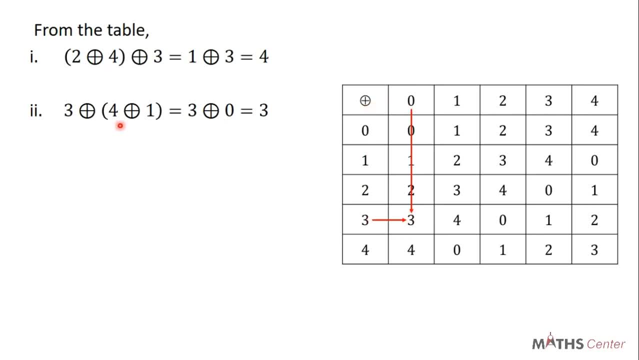 3 plus 0 is equal to 3.. So 3 plus into brackets, 4 plus 1.. 3 plus into brackets, 4 plus 1 is equal to 3 plus 0, which is equal to 3.. Once again I want to stress on the fact that in an examination you don't have to draw. 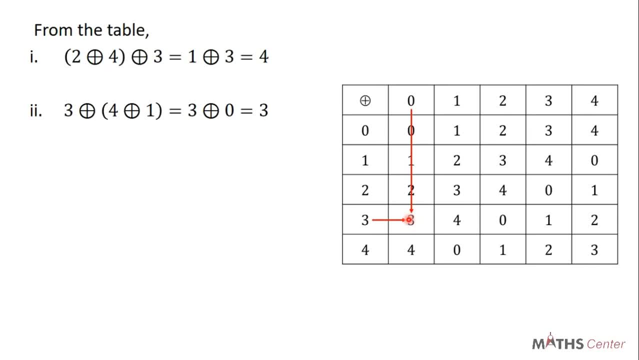 the arrows. I am drawing the arrows to show you how to read the values from the table. Let's move on III, 2 plus 4 into brackets. plus 3 plus 4 into brackets. You will find what is in the first bracket. 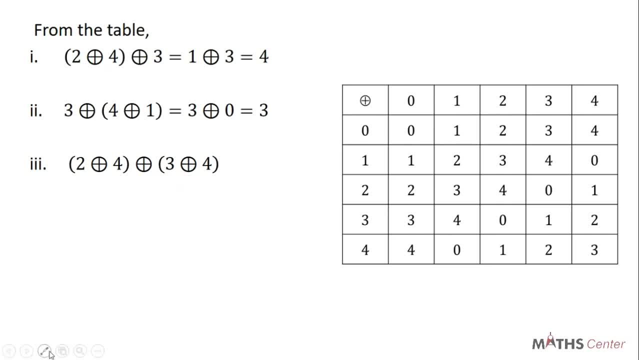 Then you add it to what is in the second bracket. The first bracket is 2 plus 4.. So you will find 2 plus 4.. We can see that from the table. 2 plus 4 will give us 1.. 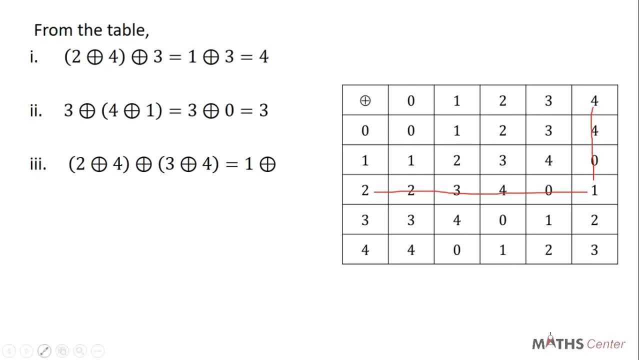 So you have 1 plus. Then we will find what is in the second bracket. The second bracket is 3 plus 4.. So you will find 3 plus 4.. 3 plus 4.. And from the table, 3 plus 4 will give us 2.. 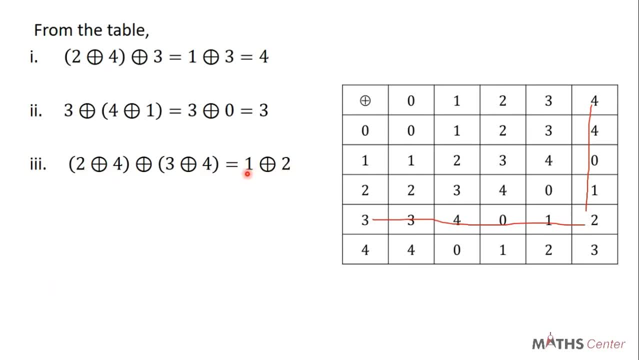 So you have 1 plus 2, because 2 plus 4 is 1 and 3 plus 4 is 2.. So now you have to find 1 plus 2 from the table. You are going to find 1 plus 2 from the table and it will give us 1 plus 2.. 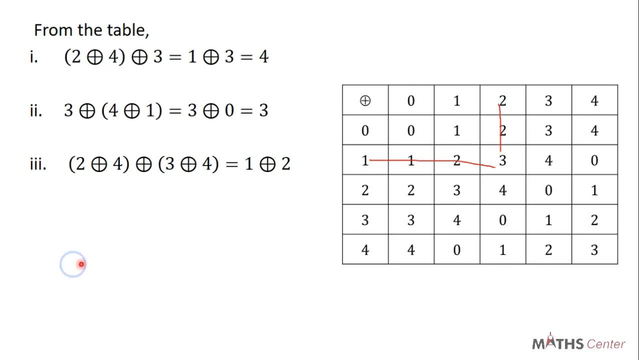 So, from the table, 1 plus 2 will give us 3. 3 plus 2.. 3 plus 2.. 3 plus 2.. This means that 2 plus 4 plus 3 plus 4 is equal to 1 plus 2, which is equal to 3.. 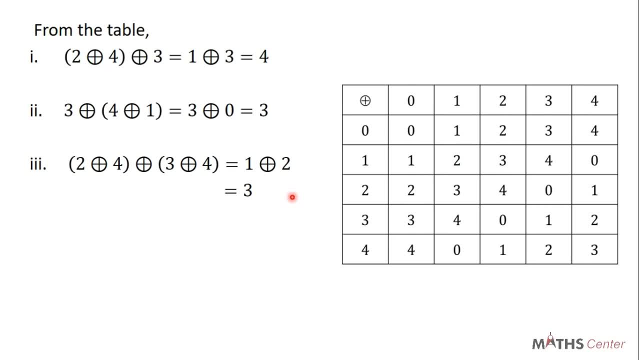 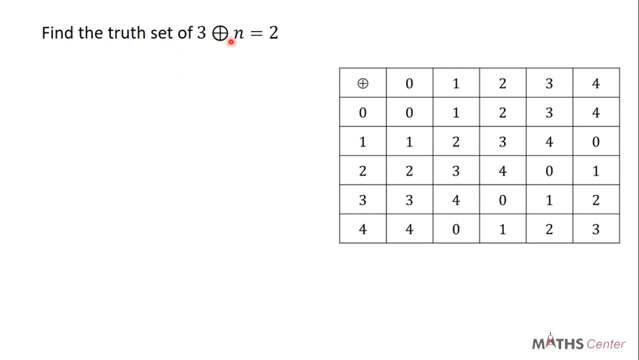 Remember that in an examination you don't have to draw the arrows in the table. I drew them to show you how to pick the values from the table. The next part of the question says that we should find the truth set of the equation. 3 plus n is equal to 2.. 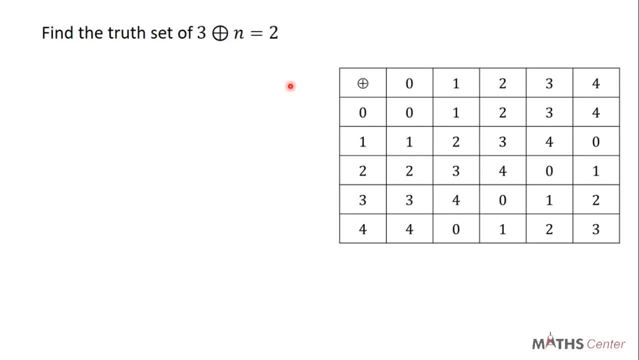 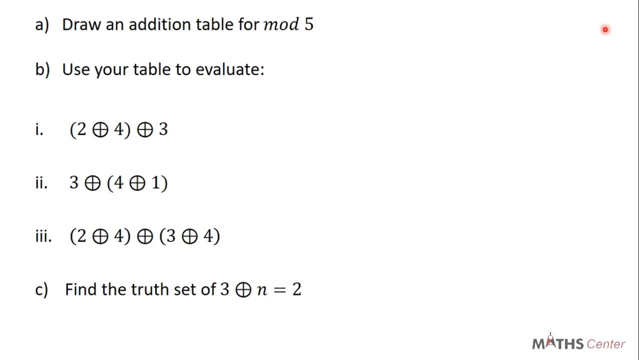 We are going to do that in the next part. So see you in the next video and let's continue solving this question. Bye, bye, Welcome back. We started solving this question. in the previous video, We solved a and b. In this video we are going to solve the last part, that is, c. 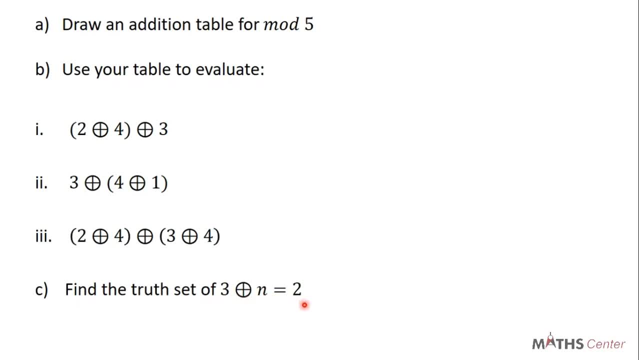 Find the truth set of 3 plus n is equal to 2.. So we are going to use the addition table from mode 5 we drew in the previous video to find the truth set of 3 plus n is equal to 2.. Find the truth set of 3 plus n is equal to 2.. The table we have here is an addition table for mode 5.. We drew this table by using the set 0,1,2,3,4.. The question wants us to find the truth. set of 3 plus n is equal to 2.. 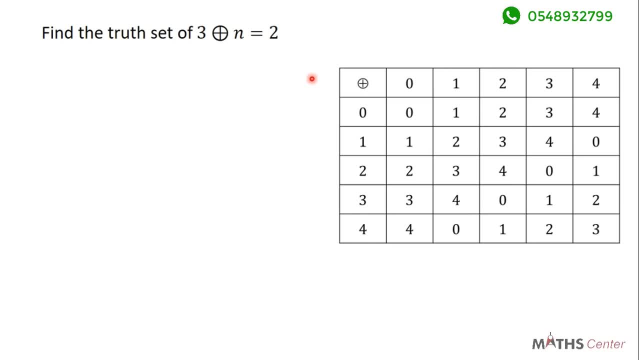 The question wants us to find the truth set of 3 plus n is equal to 2.. The question wants us to find the truth set of 3 plus n is equal to 2.. There are some values in this set that will satisfy the equation 3 plus n is equal to. 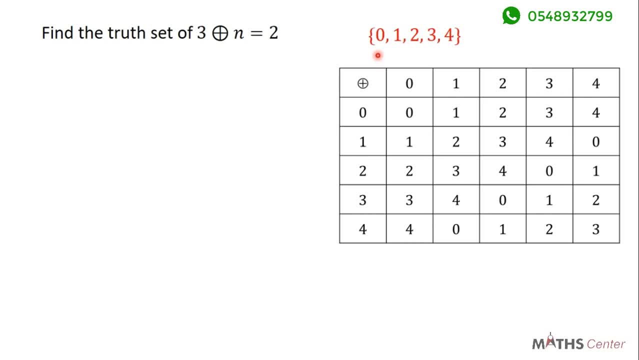 2. We don't know those values. To find it, we are going to try them out one after the other to see which one of them will satisfy the equation. So we will begin with when n is equal to 0.. When n is equal to 0, 3 plus n will become 3 plus 0. 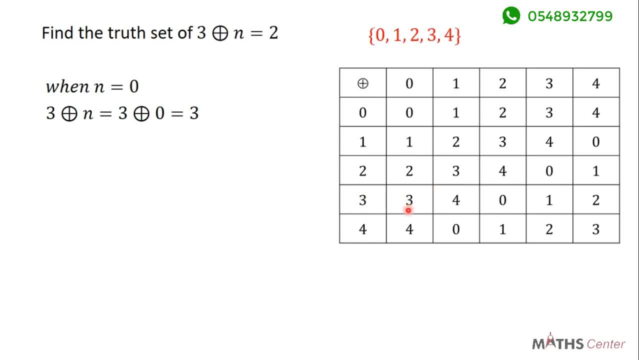 From the table, 3 plus 0 is equal to 3.. So 3 plus 0 will give us 3.. But we know that from our equation 3 plus n is equal to 3. So 3 plus 0 will give us 3.. 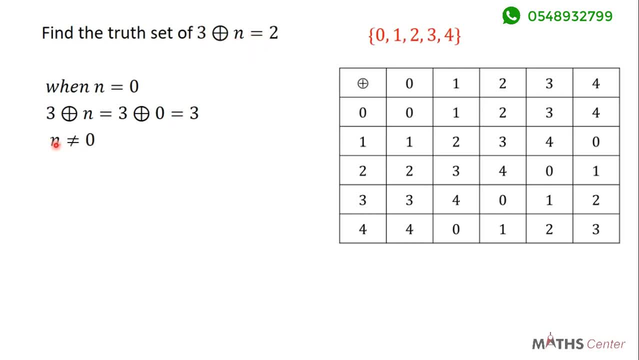 3 plus n is equal to 2. That means that n is not equal to 0, because if n is equal to 0, then 3 plus 0 should give us 2.. But here 3 plus 0 is giving us 3.. 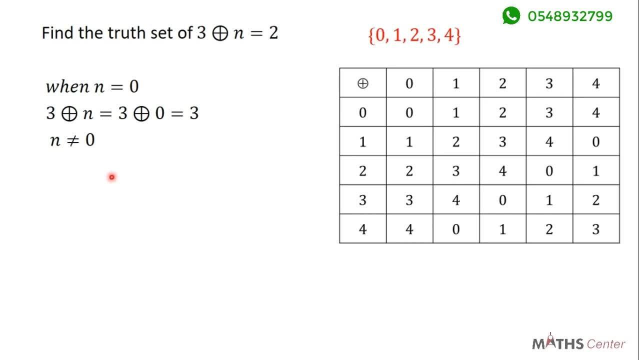 That means that the number we are looking for is not 0.. Let's move on to the next number in the set, which is 1.. So when n is equal to 1.. When n is equal to 1, 3 plus n will become 3 plus 1.. 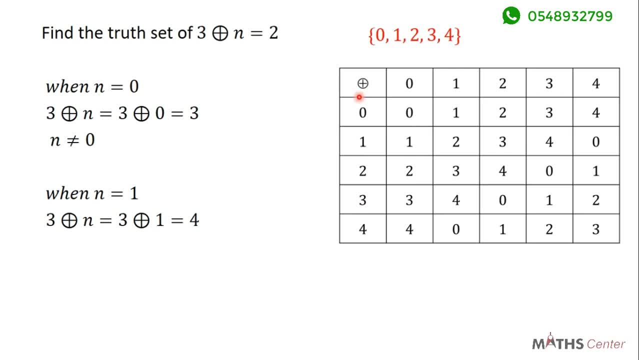 From the table, 3 plus n is equal to 1.. 3 plus n is equal to 1.. From the table, 3 plus 1 will give us 4.. We know that from our equation, 3 plus n is equal to 2.. 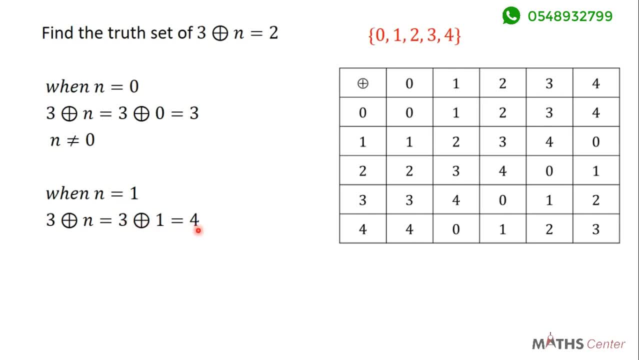 But when n is equal to 1,, 3 plus 1 will give us 4.. That means that n is not 1, because if n is 1,, 3 plus 1 should give us 2.. From the table, 3 plus 1 is equal to 4,, not 2.. 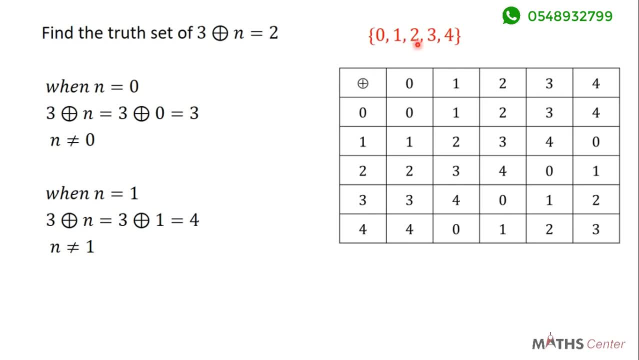 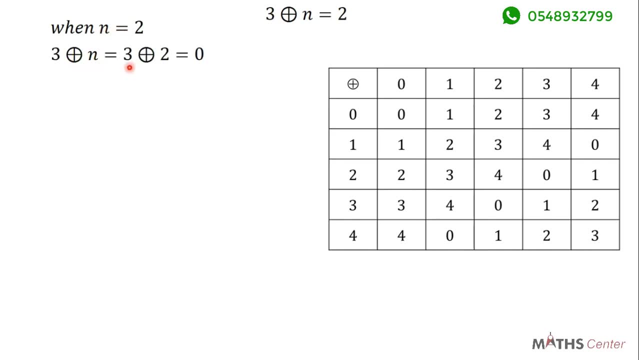 So n is not equal to 2.. So we are going to find out what n is equal to. So we are going to try out the next number in the set, which is 2.. When n is equal to 2, 3 plus n becomes 3 plus 2.. 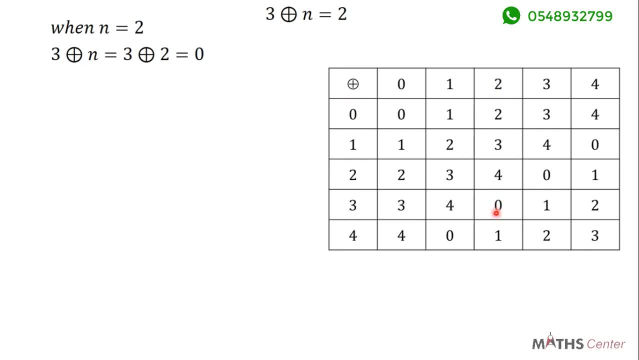 From the table, 3 plus 2 will give us 0. But we know that from our equation 3 plus n is giving us 2.. So if n is equal to 2, then 3 plus 2 should give us 2.. 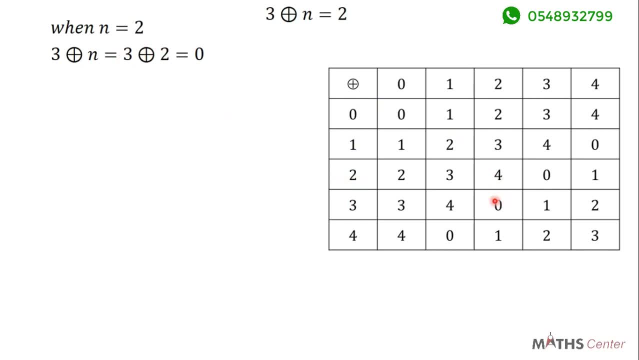 But we have seen from the table that 3 plus 2 is giving us 0. So we are going to try out the next number in the set, which is 2.. When n is equal to 3, 3 plus n is equal to 4.. 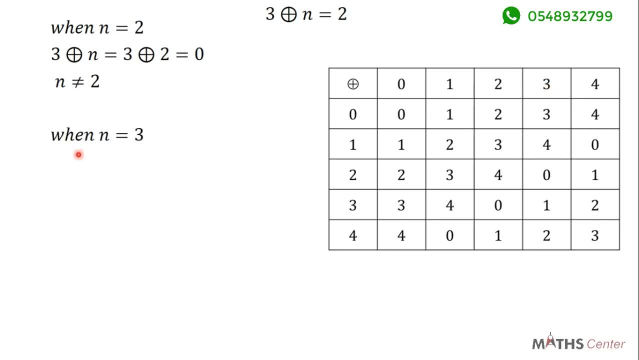 When n is equal to 3, 3 plus n becomes 3 plus 3.. From the table 3 plus 3 gives us 1. From the table 3 plus 3 gives us 1, But from our equation 3 plus n should give us 2.. Here: when n is equal to 3,, 3 plus n gives us 1, But we are going to try out the next number in the set, which is 3.. When n is equal to 3,, 3 plus n, is会 3. 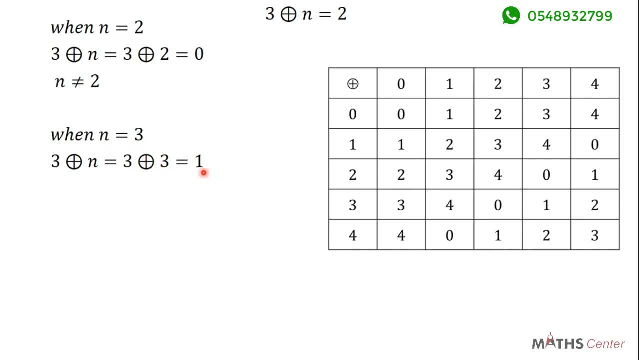 More than that, 2 plus 3 are equal to 1.. 3 plus n would be 3 plus 3.. give us 1: 2 is not equal to 1. this means that n is not equal to 3, so we will try out the last. 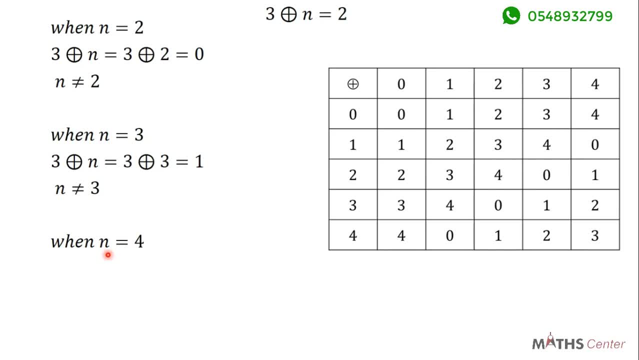 number, which is 4. when n is equal to 4, when n is equal to 4, 3 plus n will be equal to 3 plus 4. from the table, 3 plus 4 is giving us 2. we know that from our equation 3 plus n should give us 2. 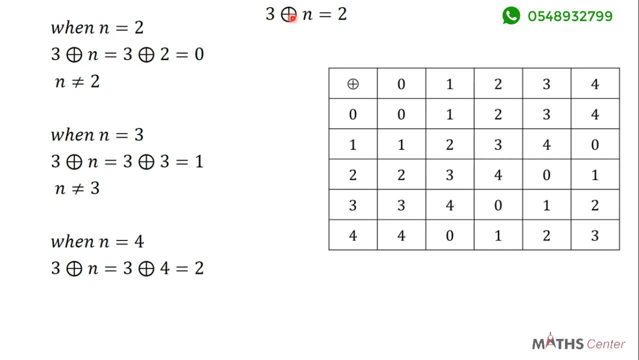 now we can see that when n is equal to 4, 3 plus 4 will give us 2. that means that n is equal to 4, so the number in the set that will satisfy the equation, 3 plus n, is equal to 2. 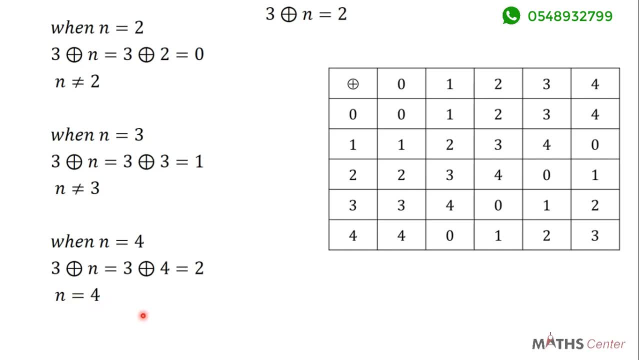 is 4, so n is equal to 4.. the question said we should find the truth set of this equation. in the videos on linear equations and linear inequalities we learned how to write the truth set of an equation. the truth set of this equation is n. is such that n is equal to 4. remember that you write it in. 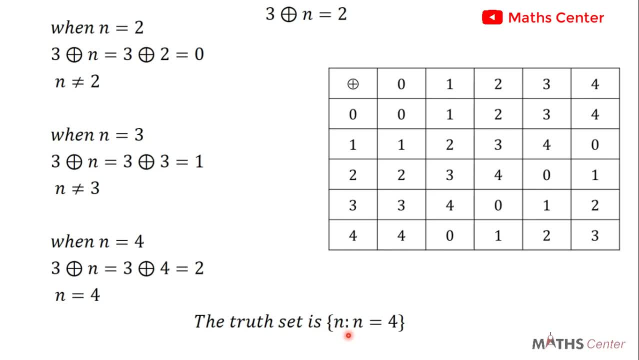 a curly bracket. so the truth set is: n is such that n is equal to 4.. thank you for watching this video. subscribe to this channel for more videos. in the next video we are going to solve another question on drawing a table for an operation in a given modulus. after drawing the table: 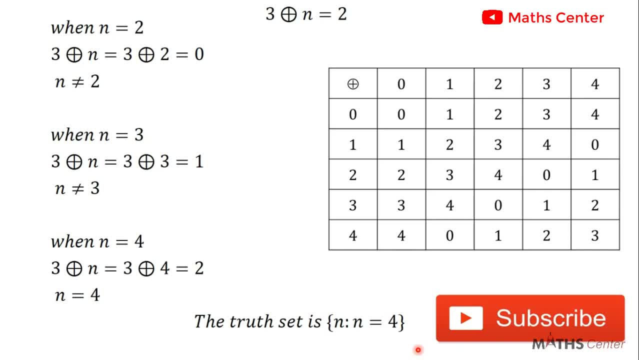 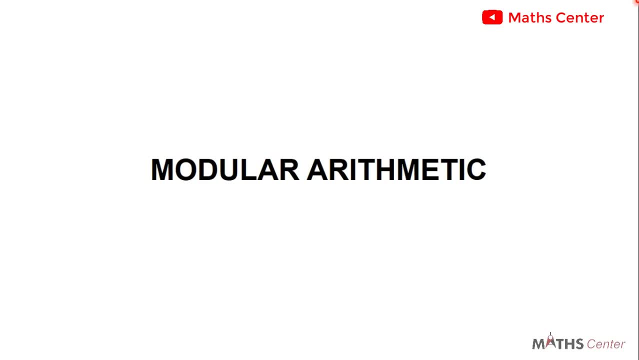 we will use it to answer some questions. bye, bye, welcome back. we are on the topic modular arithmetic. in the previous video we solved a question on drawing a table for an operation in a given modulus. in this video we are going to solve another question. the question for this video is: 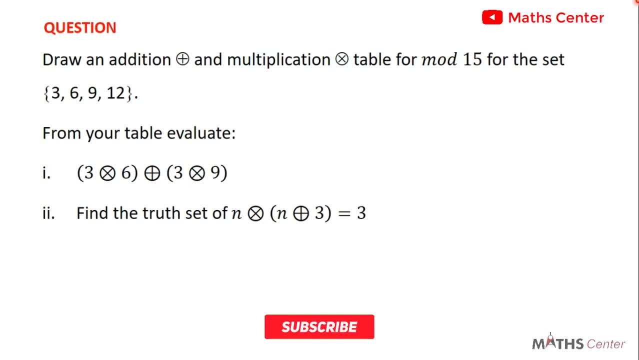 draw an addition and multiplication table. draw an addition and multiplication table for mode 15 for the set 3, 6, 9, 12 from your table. evaluate i 3 times 6 into bracket plus 3 times 9 into another bracket. i i find the truth set of n times into. 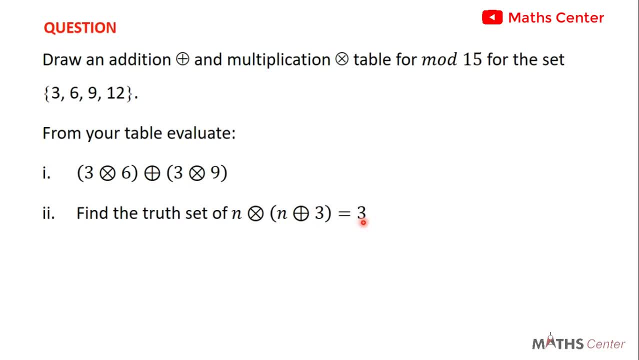 bracket n plus 3 is equal to three to 3.. We will draw the addition and multiplication tables in this video. In the next video we are going to use our tables to solve the remaining part of the question. Let's begin by drawing the. 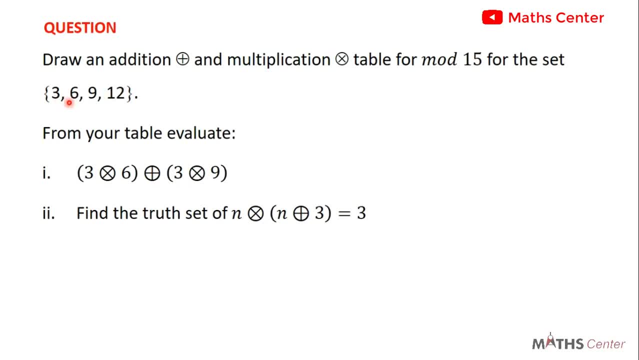 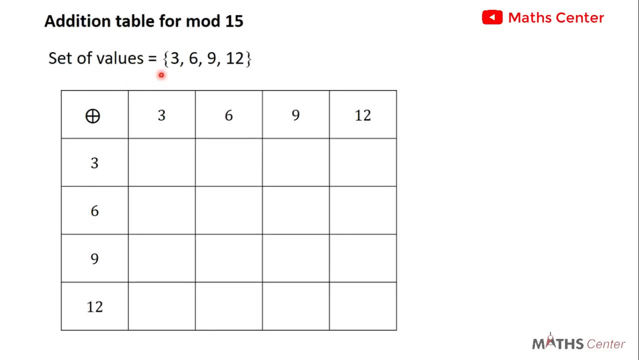 addition table for mode 15 for the set 3, 6, 9, 12.. As you can see, we are given a set of values in the question, So we are going to use that set of values to draw the table. There are four values. 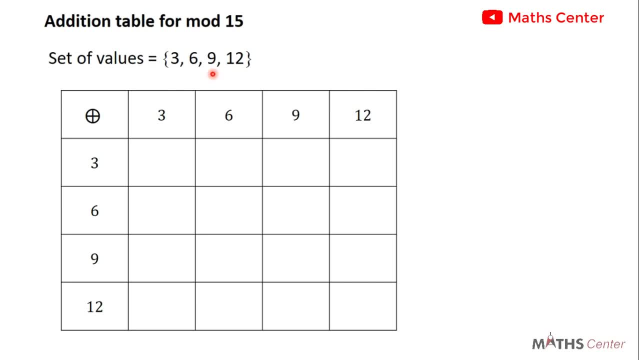 in the set. So we are going to draw a table with five columns and five rows. In the first cell we will indicate the sign of the operation we are going to perform. We are drawing an addition table, So you write the addition sign and you draw a circle around it. You then list the set of numbers. 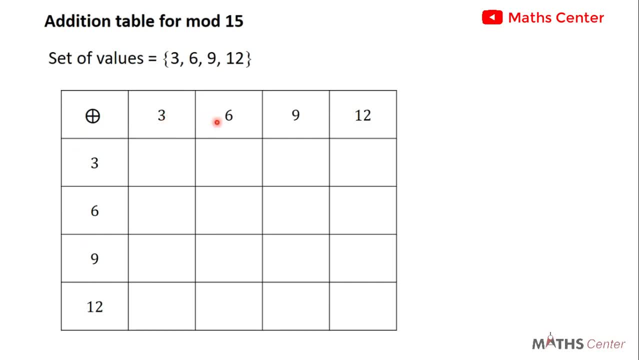 in the first row and the first column: 3, 6, 9, 12 and 3 6 9, 12.. We are adding the numbers in mode 15.. The first one is 3 plus 3.. 3 plus 3 is 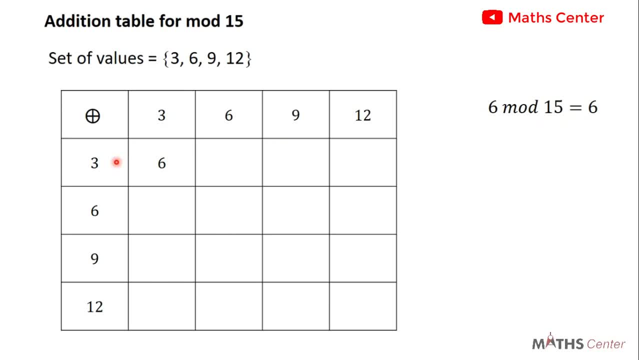 6. 6. mode 15 is 6.. 3 plus 6 is 9.. 9. mode 15 is 9.. 3 plus 9 is 12.. 12. mode 15 is 12.. 3 plus 12 is 15.. 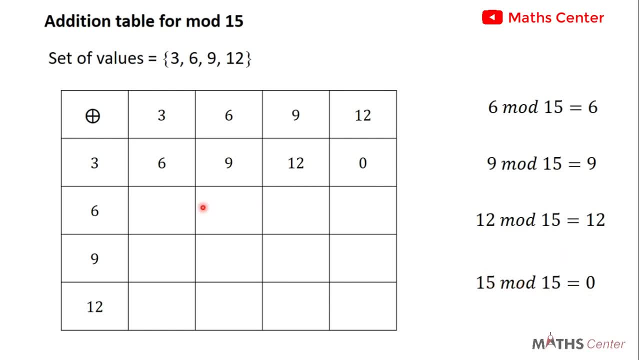 15 mode 15 is 0.. Let's move on to the next rule. 6 plus 3 is 9.. 9 mode 15 is 9.. 6 plus 6 is 12.. 12 mode 15 is 12.. 6 plus 9 is 15.. 15 mode 15 is 0.. 6 plus 12 is 18.. 18 mode 15 is 3.. So 18 is greater. 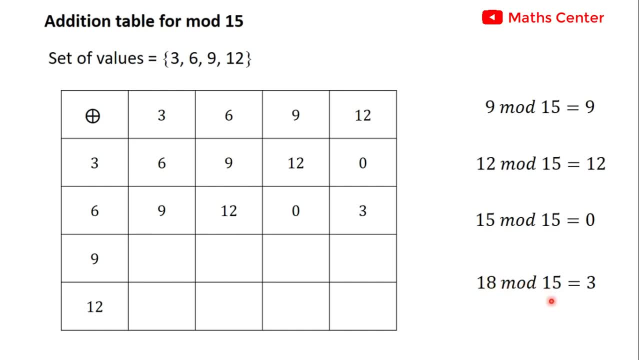 than the modulus, which is 15.. So if you want to draw a set of values in the set- 3, 6, 9, 9, 12. You want to find 18, mode 15. You divide 18 by 15 and that will give us 1 remainder, 3.. Or you can use 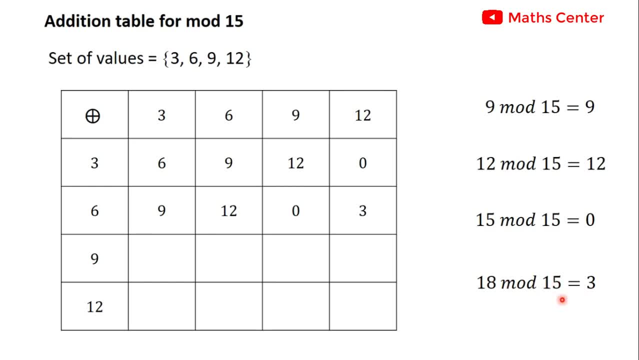 the trick that we've learnt: You subtract 15 from 18 and you get 3.. So 18 mode 15 is 3.. Let's move on to the next rule: 9 plus 3 is 12.. 12 mode 15 is 12.. 9 plus 6 is 15.. 15 mode 15 is 0.. 9. 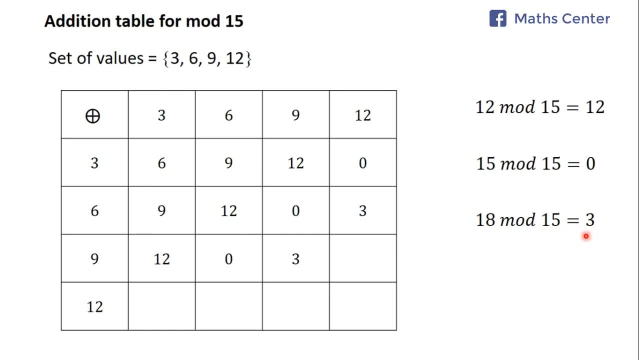 plus 9 is 18.. 18 mode 15 is 3.. 9 plus 12 is 21.. 21 mode 15 is 6.. Because 21 divided by 15 will give us 1 remainder 6.. Or, if you want to use the trick that we've learnt You, 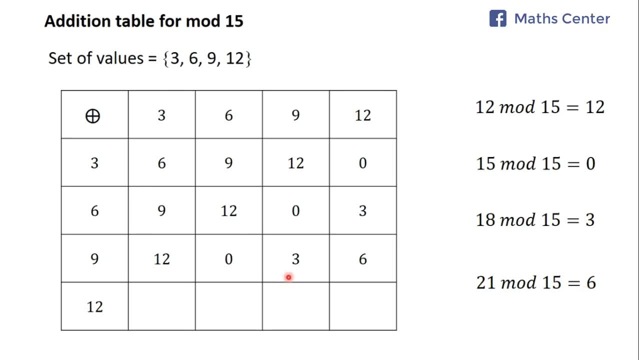 subtract 15 from 21 and you get 6.. so 21 mode 15 is 6.. 12 plus 3 is 15.. 15 mode 15 is 2.. mode 15 is 0.. 12 plus 6 is 18.. 18 mode 15 is 3.. 12 plus 9 is 21.. 21 mode 15 is 6.. And. 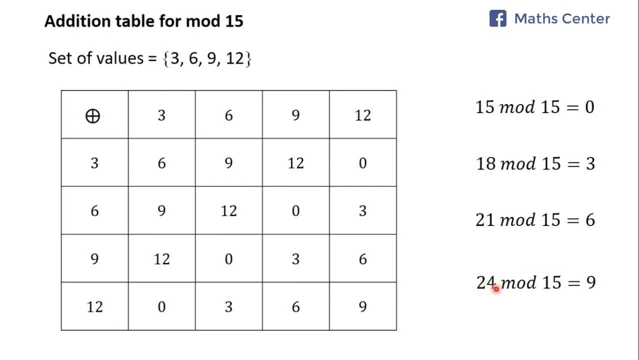 finally, 12 plus 12 is 24.. 24 mode 15 is 9, because 24 divided by 15 will give us 1, remainder 9, or 24 minus 15 will give us 9, which is less than the modulus. So 24 mode 15 is 9.. We have 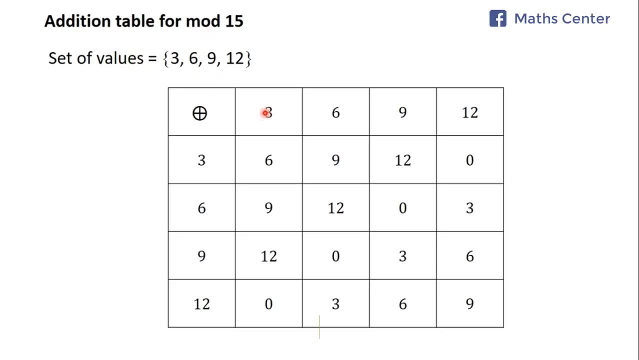 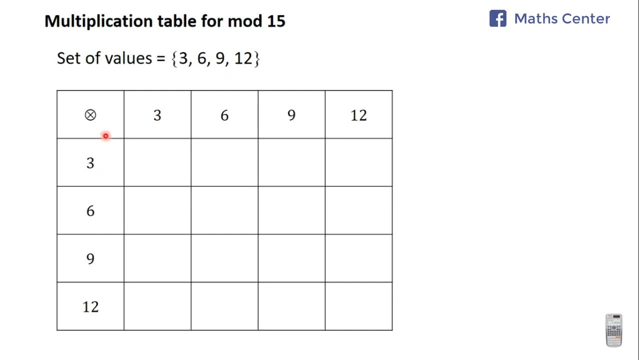 now completed the addition table for mode 15 on the set 3, 6, 9, 12.. Let's move on to the multiplication table. 3 times 3 will give us 9.. 9 mode 15 is 9.. 3 times 6 is 18.. 18 mode. 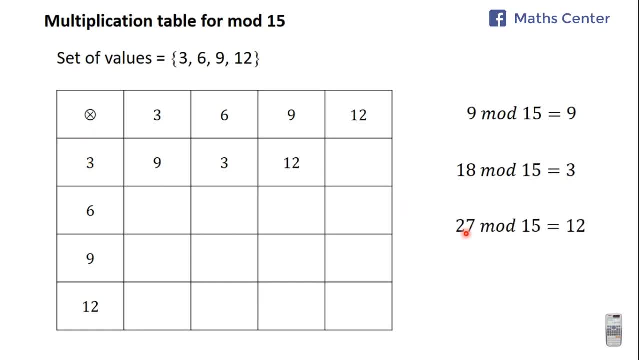 15 is 3.. 3 × 9 is 27,. 27 × 15 is 12. 3 × 12 is 36,. 36 × 15 is 6. 6 × 3 is 18,. 18 × 15 is 3. 6 × 6 is 36,. 36 × 15 is 6. 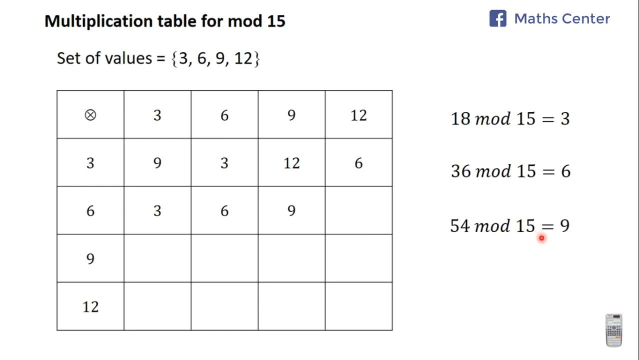 6 × 9 is 54,. 54 × 15 is 9. 6 × 12 will give us 72,. 72 × 15 is 12. Let's move on to the next rule. 9 × 3 will give us 27,. 27 × 15 is 12. 9 × 6 will give us 54,. 54 × 15 is 9. 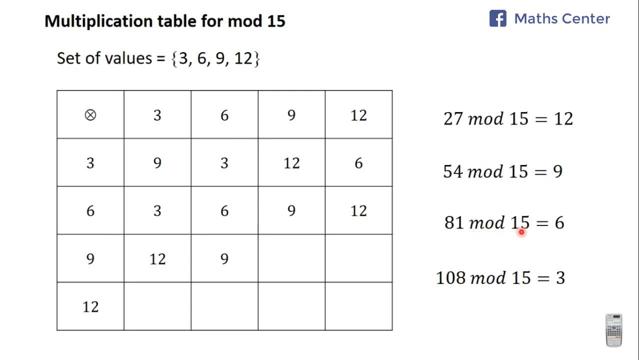 9 × 9 will give us 81,. 81 × 15 is 9. 9 × 12 will give us 108,. 108 × 15 is 3. Let's move on to the last rule. 12 × 3 will give us 36,. 36 × 15 is 6. 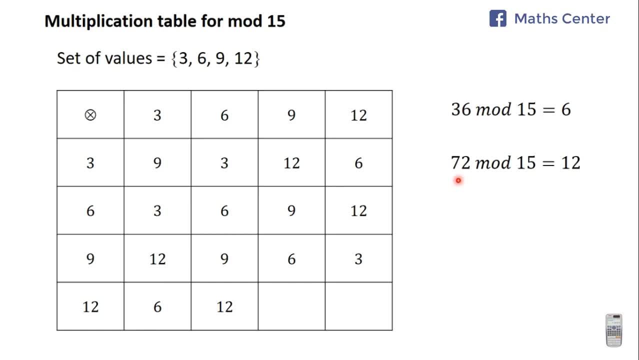 12 × 6 will give us 72,. 72 × 15 is 12. 12 × 9 will give us 108,. 108 × 15 is 3. 12 × 9 will give us 78,. 78 × 15 is 3. 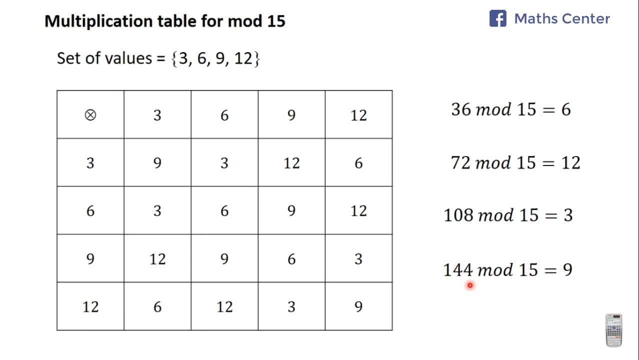 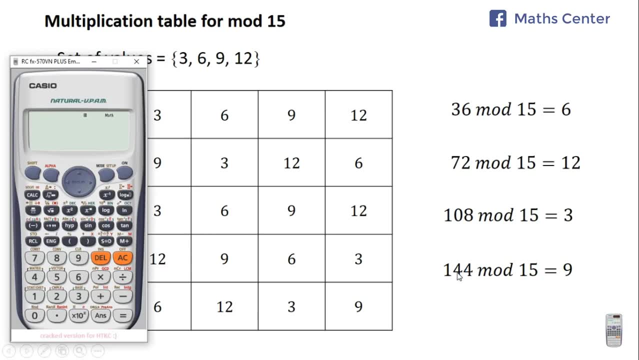 And finally, 12 × 12 will give us 144,. 144 × 15 is 9. If you want to use the trick to find 144 × 15 in a calculator, subtract 15 from 144 and you have 129.. 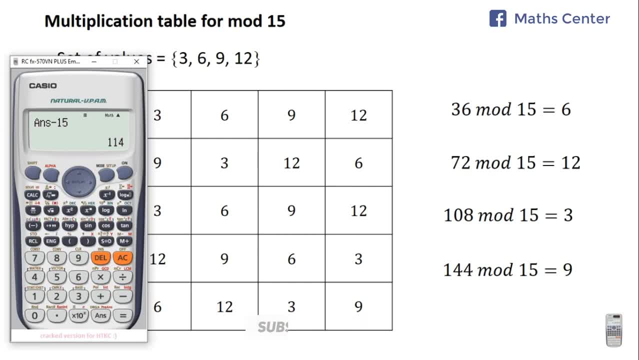 You subtract 15 from 129,, you have 114.. You subtract 15 from 114,, you have 99.. You subtract 15 from it, you have 84.. You subtract 15 from 84,, you have 69.. 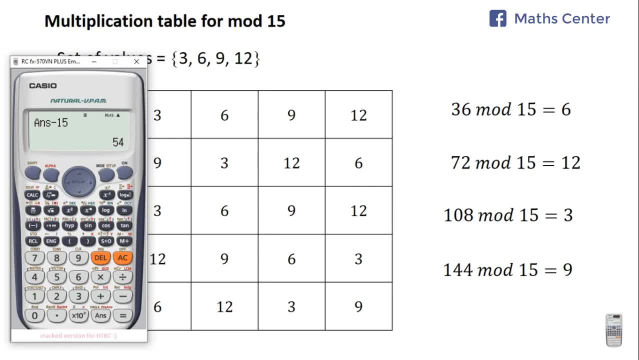 You subtract 15 from 69,, you have 54. Then you subtract 15 from it again, you have 39. You subtract 15 from it again, you have 24.. Then you subtract 15 from it again, and you have 9.. 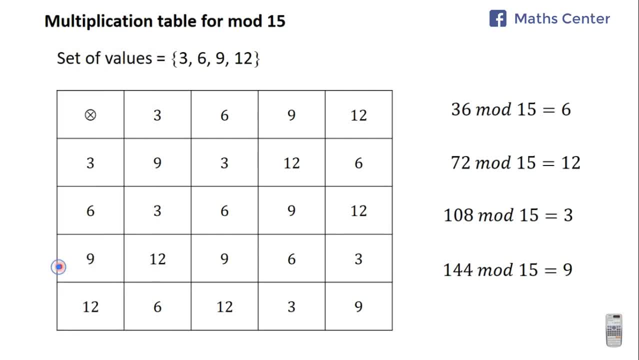 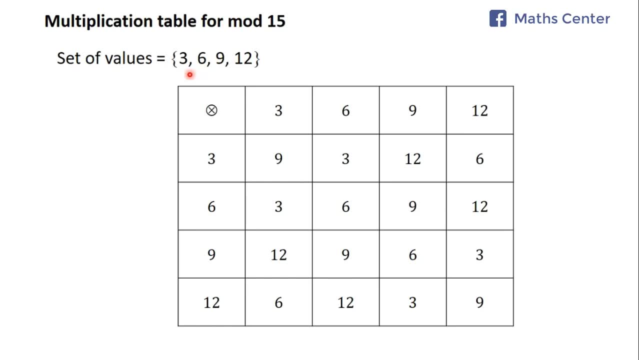 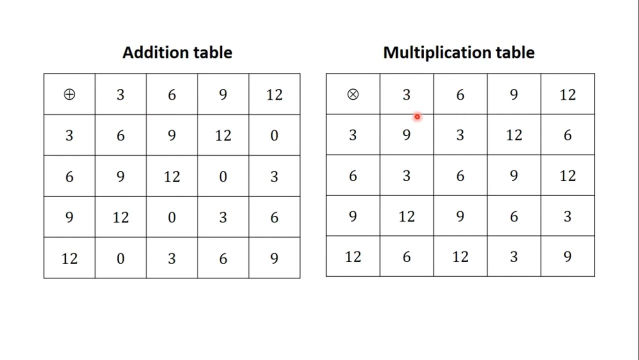 So you keep on subtracting the modulus from the number until you get a value that is less than the modulus. We have completed the multiplication table for mode 15 on the set Threads. So now we have both the addition and multiplication tables for mode 15 on the set 3,, 6,, 9, 12.. 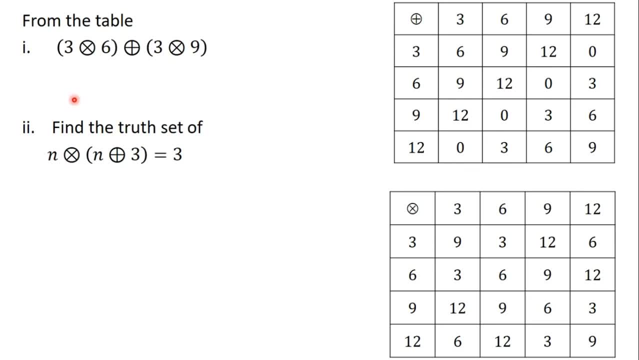 The next part of the question says that we should use our tables to evaluate i 3 times 6 into brackets, plus into brackets 3 times 9, ii find the truth, set of n times into brackets, n plus 3 is equal to 3.. 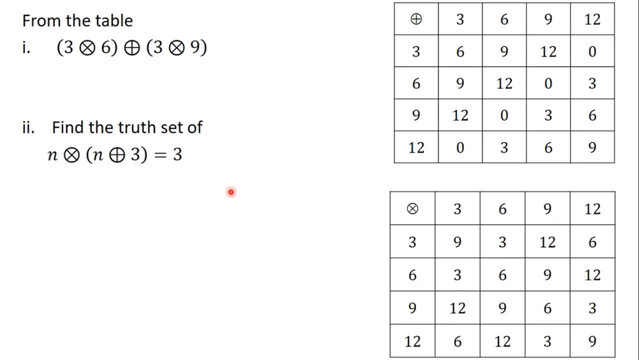 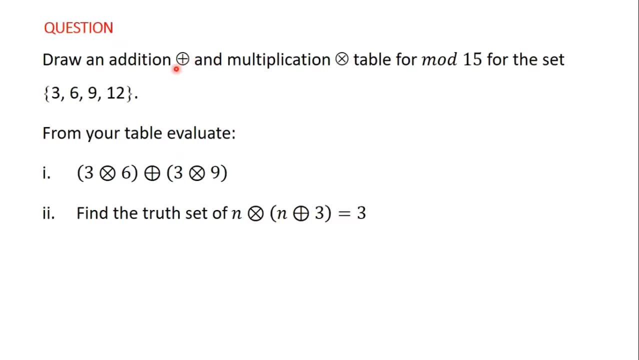 We are going to do this in the next video. So see you in the next video and let's continue solving the question. Bye, bye, Welcome back. We started solving this question. in the previous video We drew the addition and multiplication table for mode 15 on the set 3,, 6,, 9,, 12.. 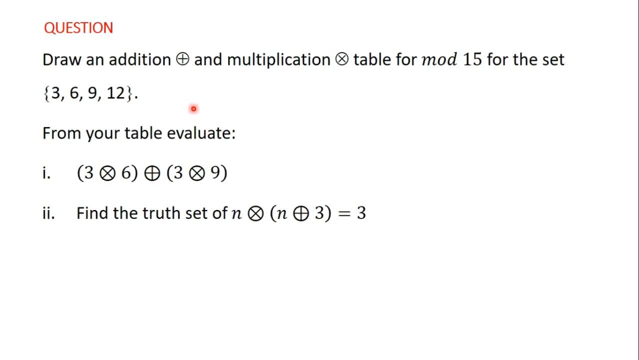 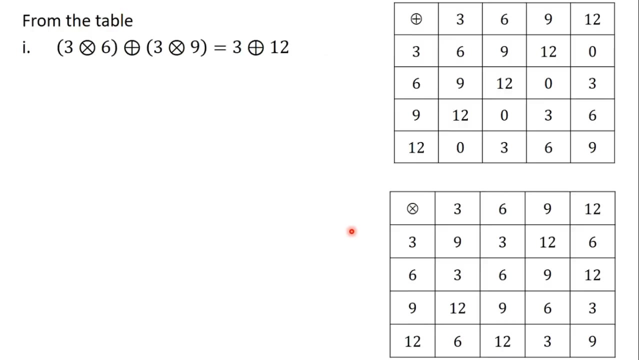 In this video we are going to use the tables that we drew in the previous video to evaluate i 3 times 6 plus 3 times 9 and also find the truth. set of n times into brackets, n plus 3 is equal to 3.. 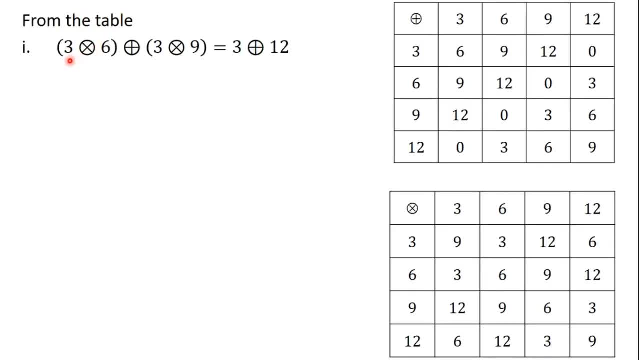 So let's begin. The first one says that we should use our tables to evaluate 3 times 6, plus into brackets, 3 times 9.. So you have to find 3 times 6 from the table. From the table, 3 times 6 will give us 3.. 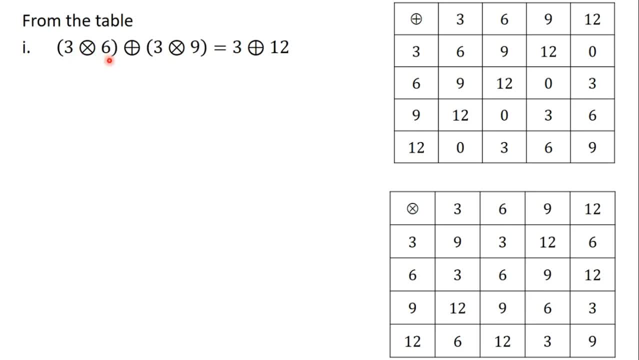 So the content of the first bracket, that is, 3 times 6, will give us 3.. So you have 3 plus. you have to find 3 times 9 from the table. From the table, 3 times 9 will give us 12.. 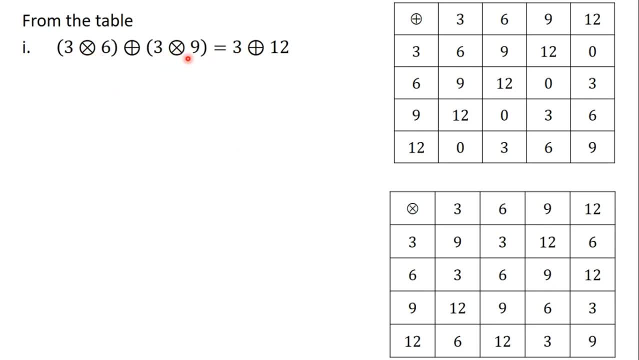 So 3 times 6 will give us 3, and 3 times 9 will give us 12.. So you have 3 plus 12.. From the table, 3 plus 12 is equal to 0. So 3 plus 12 will give us 0.. 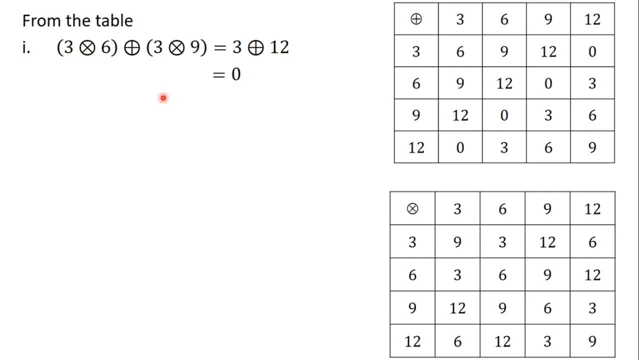 So 3 times 6, we can find it from the multiplication table. 3 times 9, we can find it from the multiplication table. Then we will find 3 plus 12 from the addition table. From the addition table, 3 plus 12 will give us 0.. 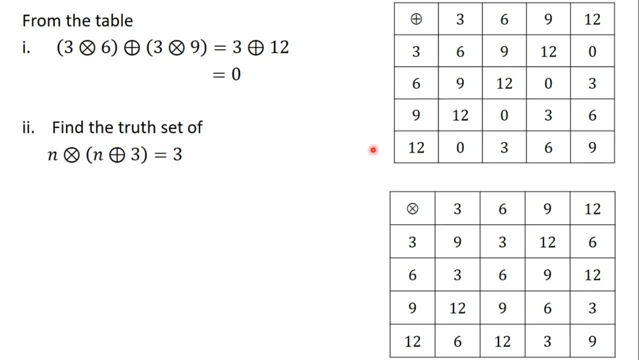 The next part of the question says that We should use our tables to find the truth. set of n times into brackets, n plus 3 is equal to 3.. We drew addition and multiplication tables for mode 15 on the set 3,, 6,, 9,, 12.. 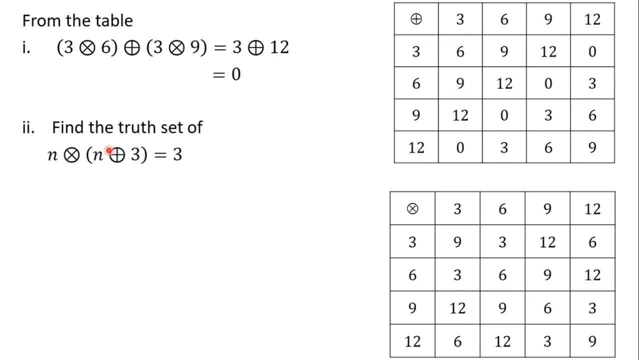 There are some values in the set- 3,, 6,, 9,, 12- that will satisfy this equation. To find those values, we are going to try them out one after the other. We will begin with the first set. We will start with the first one, which is 3.. 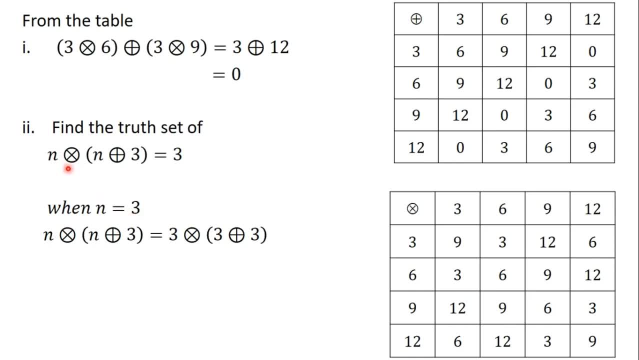 So when n is equal to 3. When n is equal to 3, n times into brackets n plus 3 will become 3 times into brackets 3 plus 3, because n is now 3.. You have to find what is in the brackets. 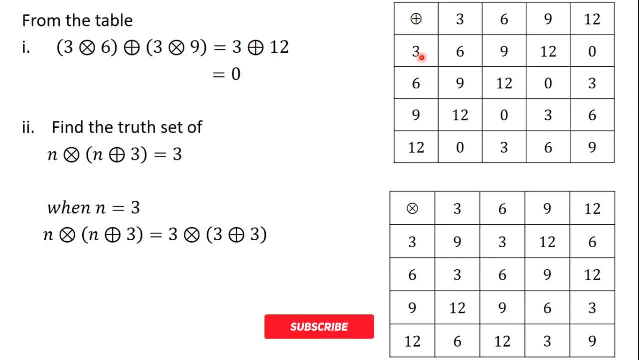 3 plus 3.. So you go to the addition table. From the addition table, 3 plus 3 is 6.. So this will become 3 times n plus 3. So n is equal to 3.. So n is equal to 3.. 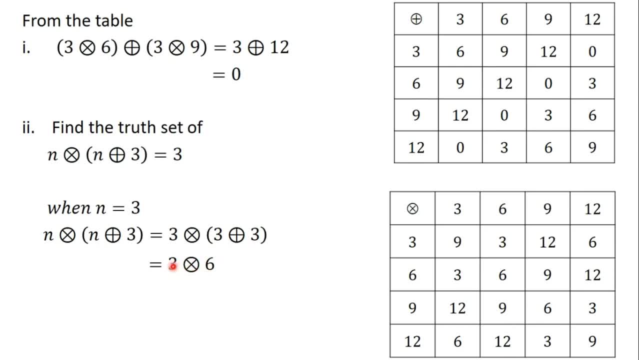 So n is equal to 3.. 3 plus 3 is now 6.. So 3 times 6. To find 3 times 6, we will go to the multiplication table. From the multiplication table, 3 times 6 will give us 3.. 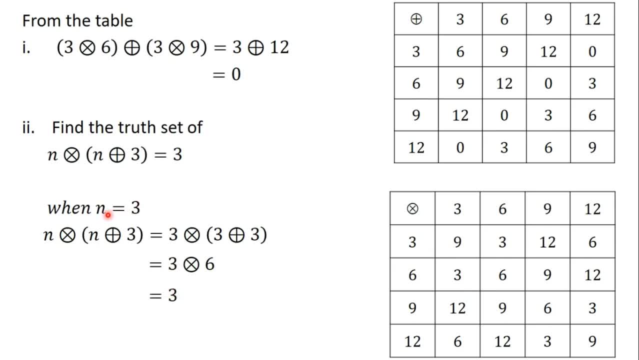 So 3 times 6 is 3.. We can see that n is equal to 3 satisfies this equation because when we substitute n is equal to 3 into the expression n times into brackets n plus 3, we are having a final answer of 3.. 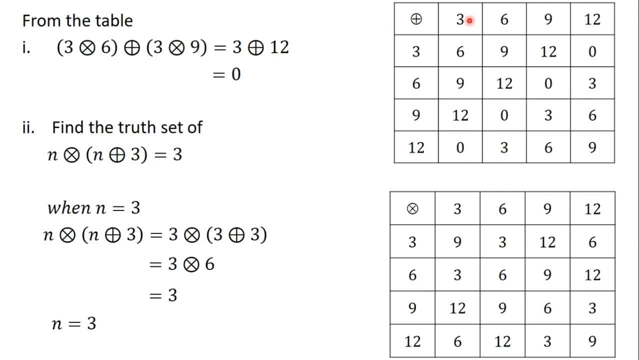 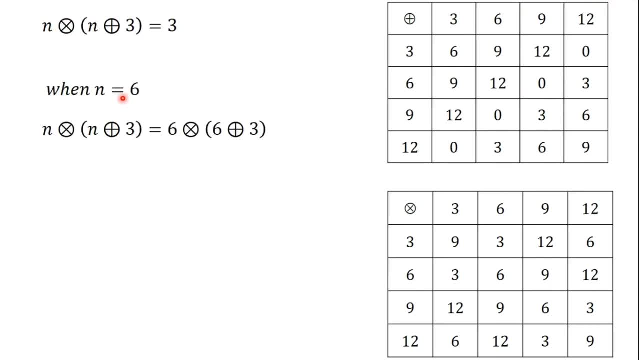 One of the numbers in this set that will satisfy the equation is 3.. Let's try out the other numbers and see. The next one is when n is equal to 6.. When n is equal to 6, n times into brackets. n plus 3 will become 6 times into brackets. 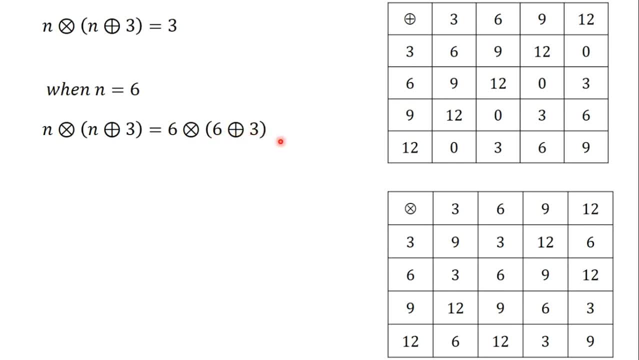 6 plus 3.. We are going to find 6 plus 3 from the addition table. From the addition table, 6 plus 3 will give us 9.. So you have 3 times 6 plus 3.. So you have 3 times 6 plus 3.. 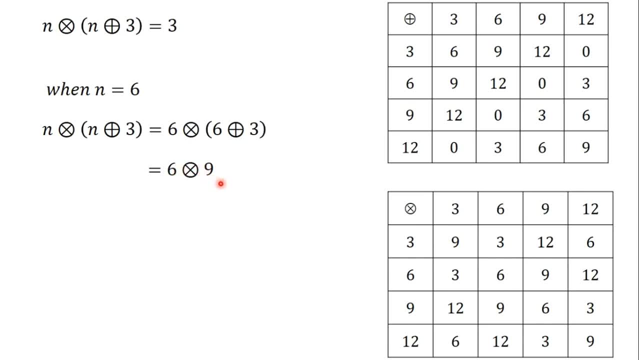 So you have 6 times 9.. You will find 6 times 9 from the multiplication table. From the multiplication table, 6 times 9 will give us 9.. But we know that from our equation, n times into brackets, n plus 3 should give us 3.. 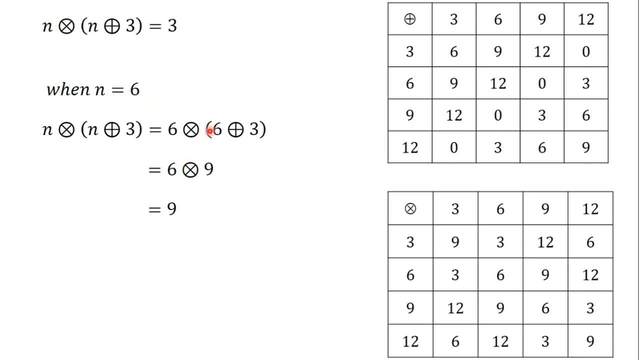 But here, when n is equal to 6,, 6 times into brackets, 6 plus 3, will give us 9.. That means that 6 will not satisfy the equation, So n is not equal to 6.. Let's try out the next number, which is 9.. 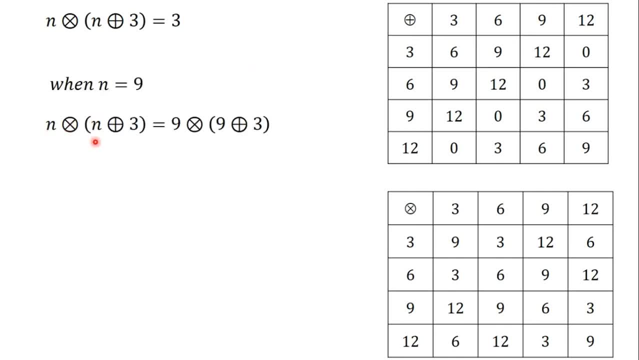 When n is equal to 9, the expression n times into brackets 9 plus 3 will become 9 times into brackets 9 plus 3.. 9 plus 3 from the addition table will be: 9 plus 3 is 12.. 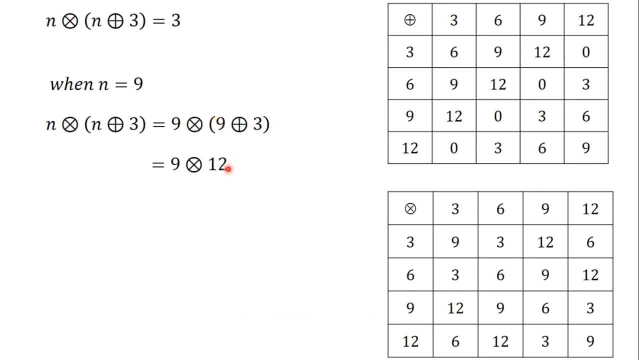 So you have 9 times 9 plus 3, which is 12.. 9 plus 3 is 12.. Just find 9 times 12 from the multiplication table. From the multiplication table, 9 times 12 is 3.. 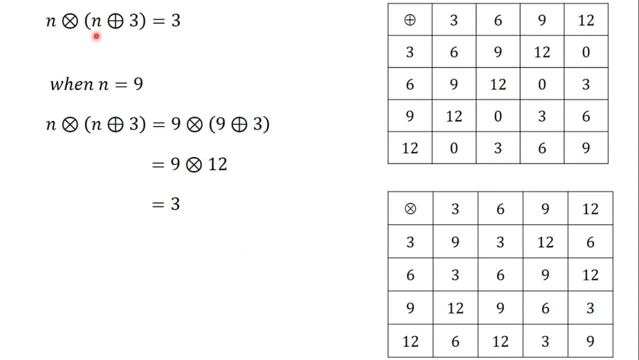 So we can see that n is equal to 9 will also satisfy the equation, because when n is equal to 9, the expression 9 times into brackets, 9 plus 3, will give us 3.. So one of the values in this set that will satisfy the equation is 9.. 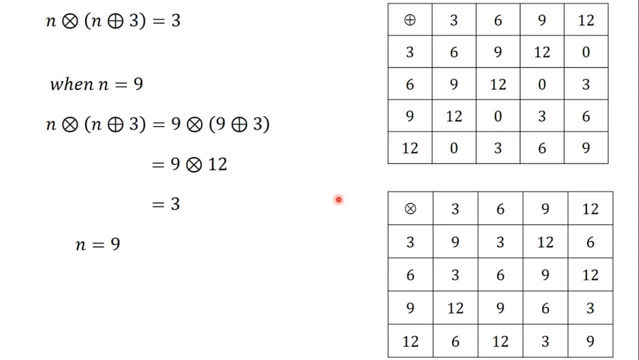 So we have seen that 3 will satisfy the equation and 9 will also satisfy the equation. Let's try out the last number, which is 12.. When n is equal to 12.. When n is equal to 12, the expression n times. 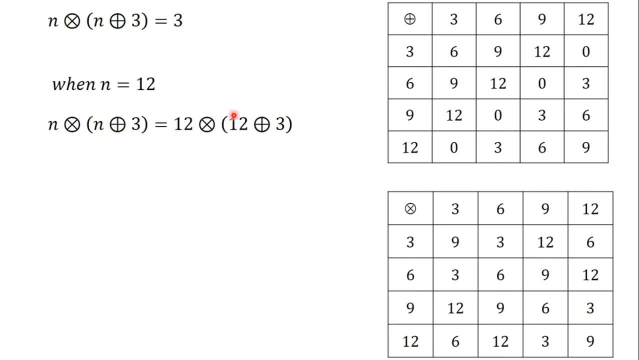 into brackets n plus 3 will become 12 times into brackets 12 plus 3.. From the addition table, 12 plus 3 is 0. So you will have 12 times 0. We don't have 0 in the set of numbers. we used to draw the table. 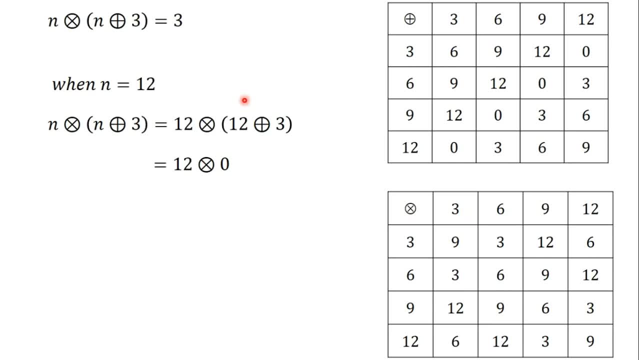 So we can't find 12 times 0 from the table. What this means is that n is equal to 12 will not satisfy the equation, So n is not equal to 12.. From our calculations we have seen that the two numbers that satisfy the equation n times. 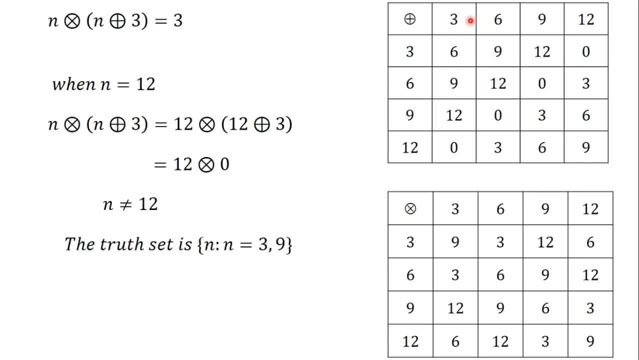 into brackets. n plus 3 is equal to 3 are 3 and 9.. The question said we should find the truth set of this equation. So the truth set is n is such that n is equal to 3 and 9.. Remember that when you are writing your truth set you will put it in a curly bracket. 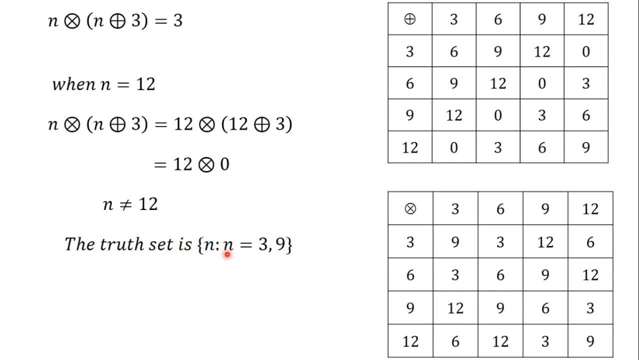 So the truth set of the equation is n is such that n is equal to 3 and 9.. Thank you for watching this video. Subscribe to this channel for more videos. In the next video we are going to learn how to solve questions involving binary operation. 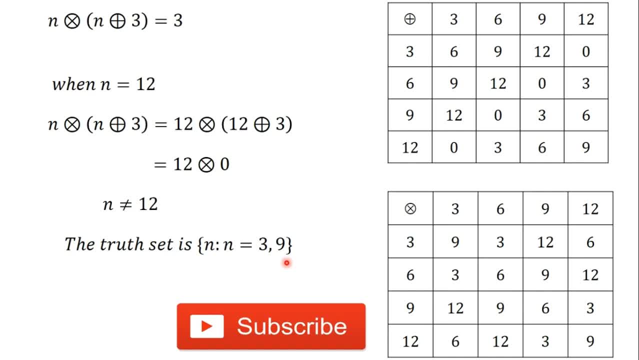 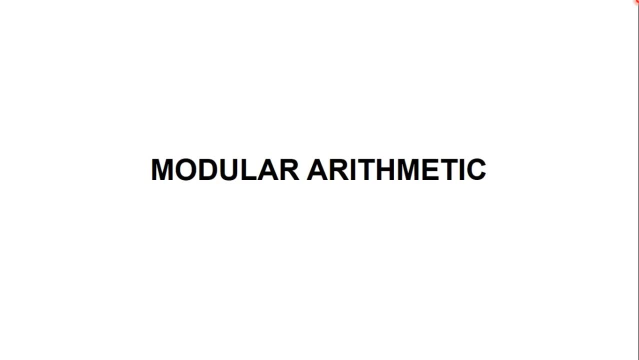 and Mulder Arithmetic. Bye-bye, Welcome back. We are still on the topic Mulder Arithmetic. In the previous video we drew a table for an operation in a given modulus and we used our table to solve some questions. In this video we are going to learn how to solve questions involving binary operation. 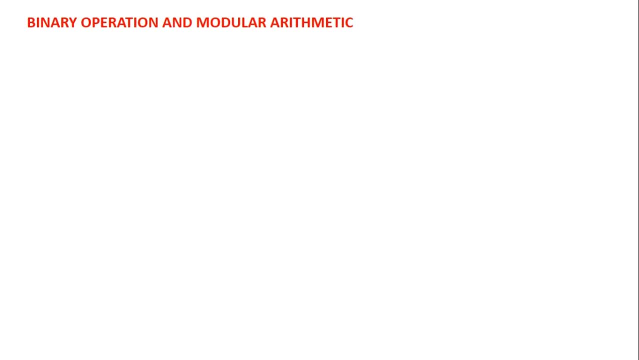 and Mulder Arithmetic- Binary operation and Mulder Arithmetic. In the second video, we are going to learn how to solve questions involving binary operation and Mulder Arithmetic. In the second and third videos, on the topic Real Number System, we considered binary operation. 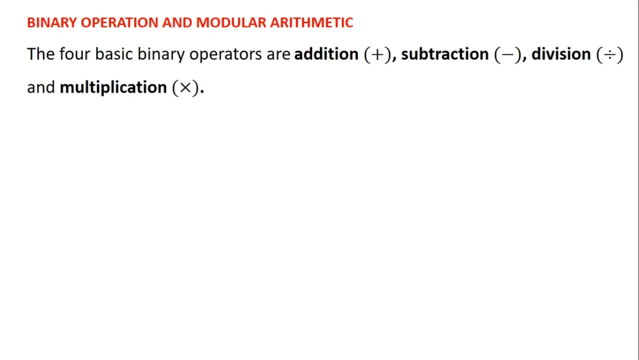 into details In those videos we learnt that the four basic binary operators are addition, subtraction, division and multiplication. These binary operators combine numbers to produce a result. So, for example, 2 plus 3 will give us 5.. So, for example, 2 plus 3 will give us 5.. So, for example, 2 plus 3 will give us 5.. So for 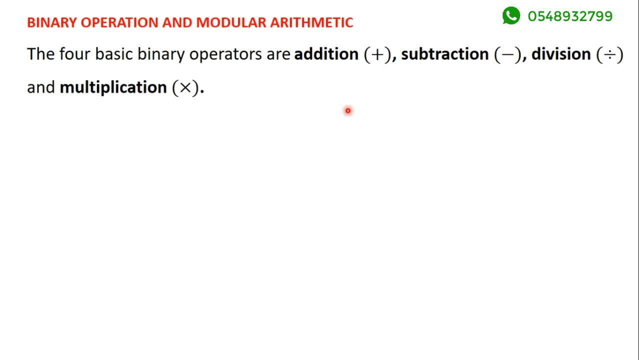 example, 2 plus 3 will give us 7.. are other binary operators and they can also combine numbers to produce a result. So, for example, let's consider this operator, star, which is defined as a star. b is equal to a plus b minus 2.. 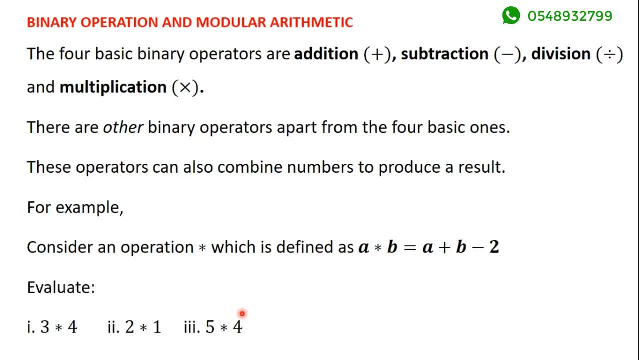 We can use the definition of this operator star to evaluate the following: i- 3 star 4, ii- 2 star 1,. iii- 5 star 4.. In the videos on binary operations and the real number system, we learnt how to evaluate. 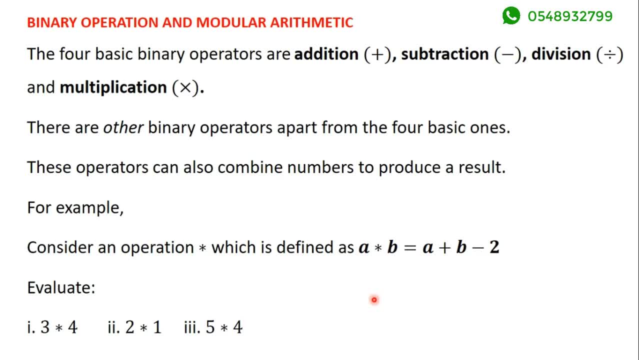 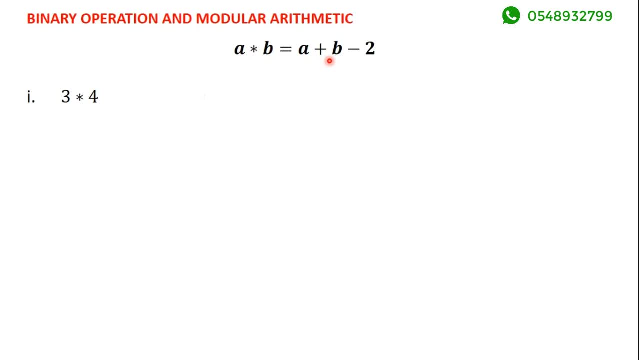 these by using the definition. I'm going to go over it quickly in this video. So the definition of star is a star b is equal to a plus b minus 2.. We are going to use this definition to evaluate 3 star 4.. 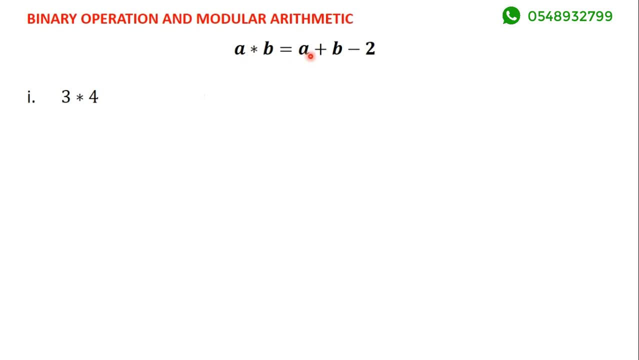 From the definition we can see that a star b is equal to a plus b minus 2.. So it means that the first number, which is a, plus the second number, which is b, then minus 2.. We want to evaluate 3 star 4.. 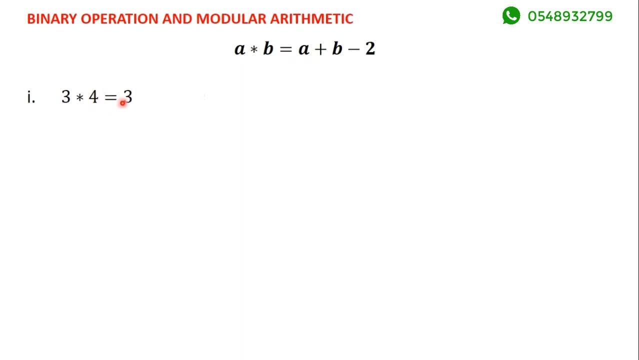 So 3 star 4 is going to be the first number, which is 3, plus the second number, which is 4 minus 2.. 3 plus 4 minus 2 will give us 5.. The next one is 2 star 1.. 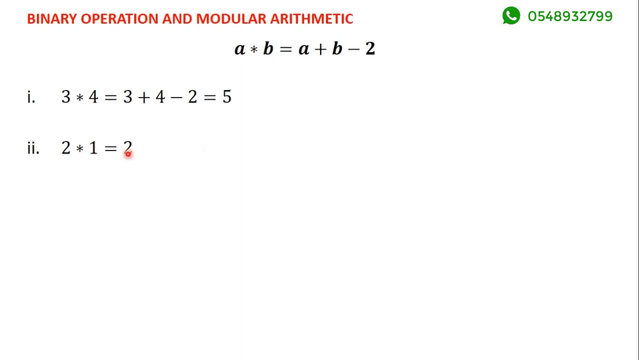 So 2 star 1 will be equal to the first number, which is 2, plus the second number, which is 1 minus 2.. 2 plus 1 minus 2 will give us 1.. The next one is 5 star 4.. 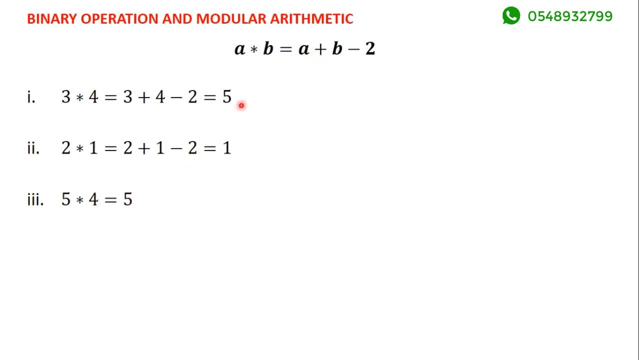 From the definition 5 star 4 will be equal to the first number. so 5 plus the second number, 4, then minus 2.. 5 plus 4 minus 2 will give us 7.. So you can see that using the definition a star b is equal to a plus b minus 2, we have 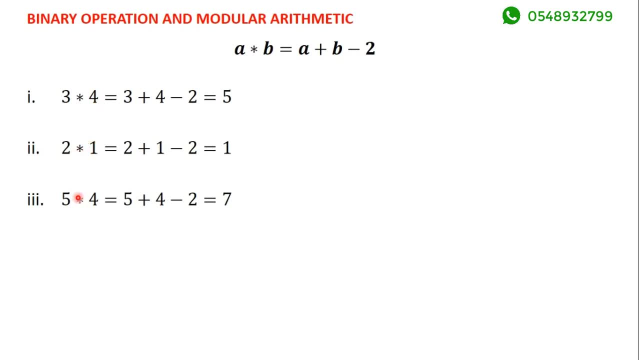 been able to evaluate 3 star 4, 2 star 1 and 5 star 4.. We learnt this in the video on binary operations under real numbers assessment. We are going to go over it quickly in this video. So the definition of a star b is equal to a plus b minus 2.. 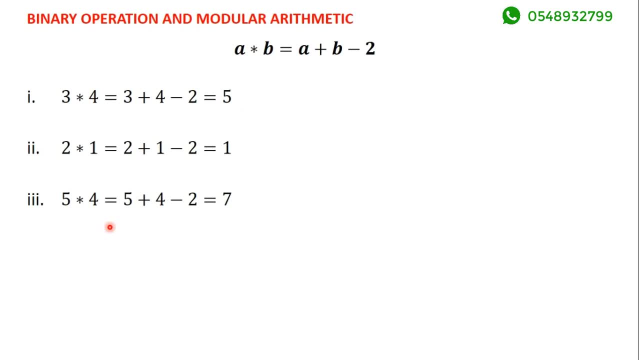 Now let's consider something. What if this operation star, which is defined as a star b, is equal to a plus b minus 2 is defined in a certain modulus? So, for example, consider the operation star, which is defined as a star b is equal to a. 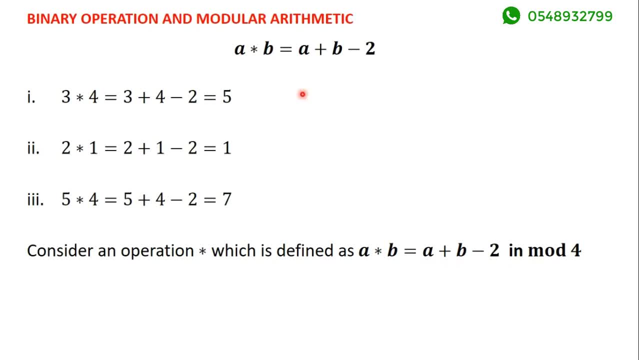 plus b minus 2 in mode 4.. So you can see that this time the definition of a star b is equal to a plus b minus 2 in mode 4.. is given to us in mode 4.. We can use this definition to evaluate 3 star 4, 2 star 1. 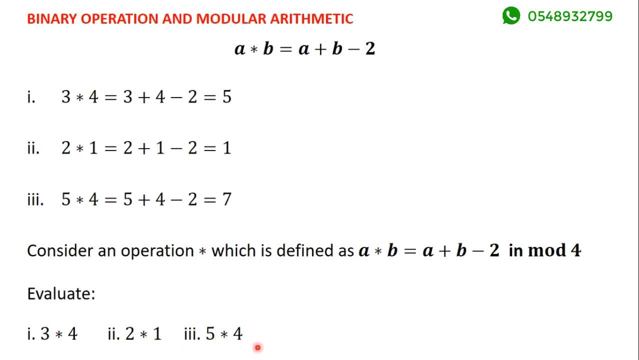 and 5 star 4.. Let's see how to do that. So now the definition is: a star b is equal to a plus b minus 2 in mode 4.. To find 3 star 4, we will first use the binary equation to evaluate 3 star 4.. 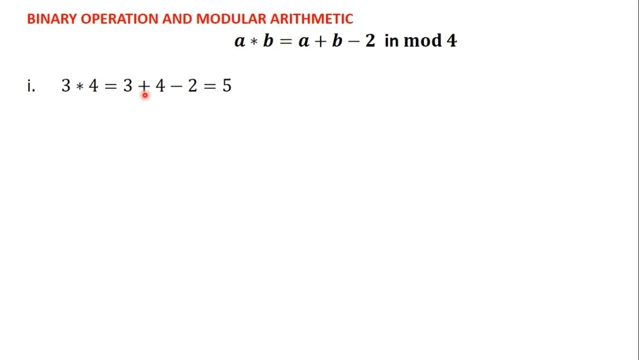 We have seen how to do it. We are going to have 3, which is the first number, plus 4, which is the second number, minus 2.. 3 plus 4 minus 2 give us 5.. But this time the definition of the binary. 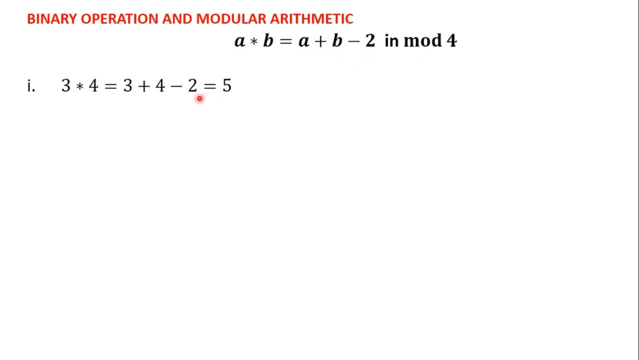 equation was given to us in mode 4.. So if we have been able to evaluate 3 star 4 and we are having 5, you have to find 5 in mode 4.. 5 in mode 4, which is written as 5 mode 4 is equal to 1.. 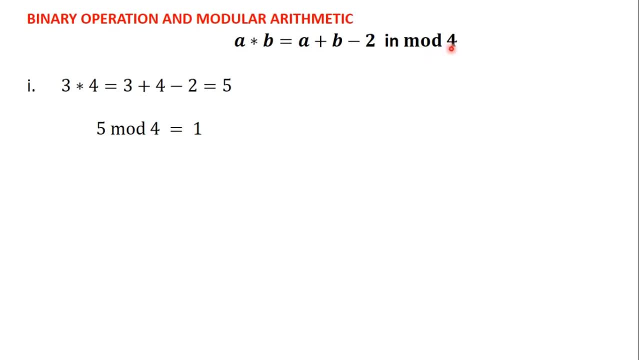 So 3 star 4 in mode 4 will give us 1, because 3 star 4 is 5 and 5 in mode 4 is 1.. Let's try out the next question: 2 star 1.. We will first use the definition of the binary. 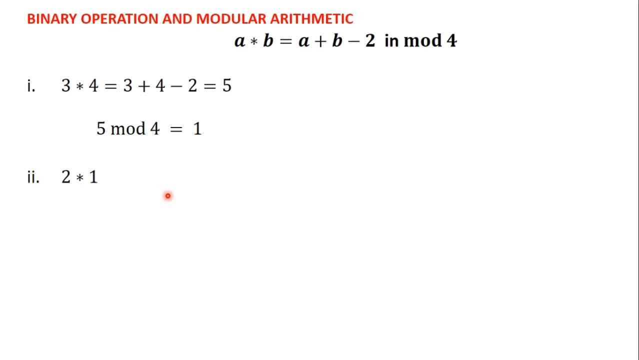 equation to find 2 star 1.. We have seen how to do that. We are going to have 2, which is the first number, plus 1, which is the second number, minus 2.. And 1 minus 2 will give us 1.. The definition of the binary equation was: 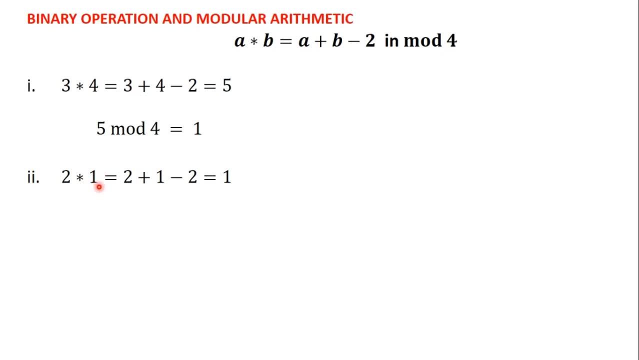 given to us in mode 4.. So if 2 star 1 is 1, we will have to find 1 in mode 4.. 1 in mode 4, which is written as 1, mode 4 is equal to 1.. So, using the definition, 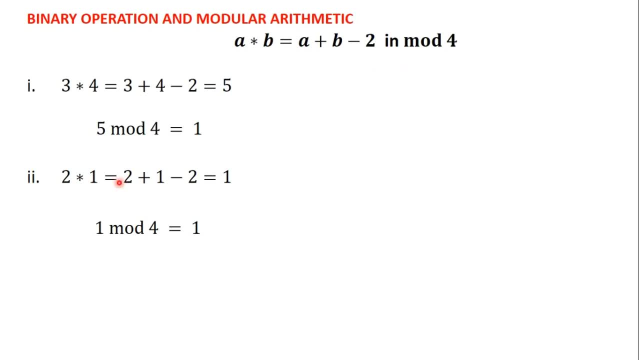 we have been able to find 2 star 1 in mode 4.. 2 star 1 is 1 and 1 mode 4 is 1.. last one: five star four. we are going to use the definition to find five star four. so you have. 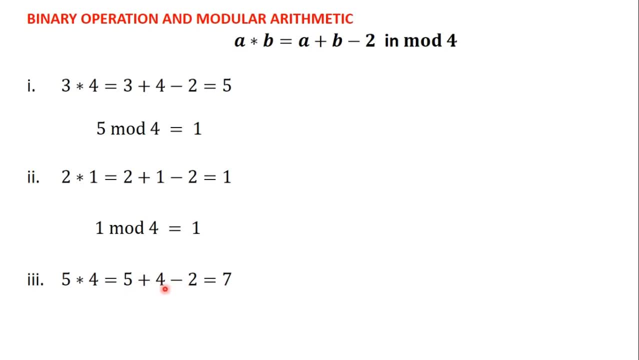 five, which is the first number, plus four, which is the second number, because five star four means that a is now five and b is four. so you have five plus four minus two. five plus four minus two give us seven. but the definition of the binary equation was given to us in mode four. we have: 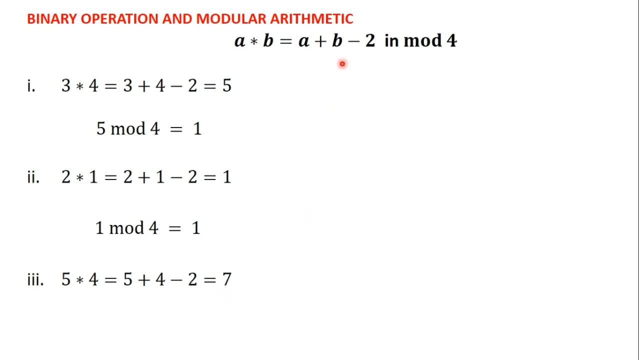 found out that five star four is seven. so you have to find seven in mode four. seven in mode four, which is written as seven. mode four is equal to three. so we can see that when a binary equation is defined in a certain modulus, you will first use the definition of the binary equation to 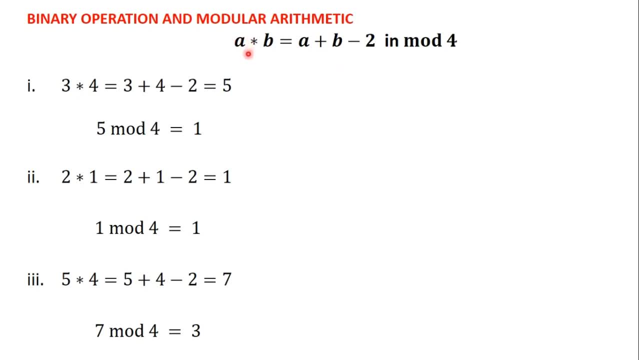 evaluate the expression. so, for example, we use the definition a star b is equal to a plus b minus two to evaluate three. so we have found out that five star four is seven. so you have to find seven in mode four and you have five. after that you find the value of the expression in the modulus. so after we have 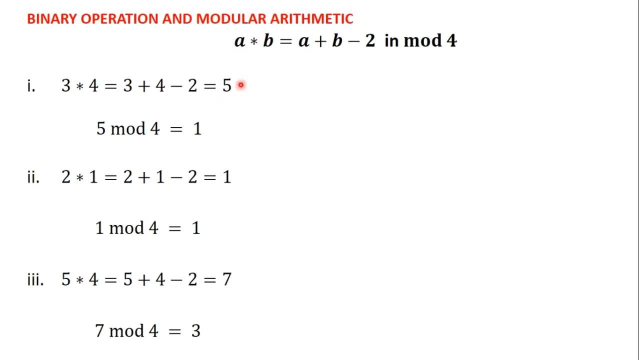 evaluated three star four and we are having five. you find a value of five in mode four. five in mode four will give us one. we used the definition to evaluate two star one and we got one. after that, you find a value of one in mode four and that will give us one. we used the definition to evaluate five. 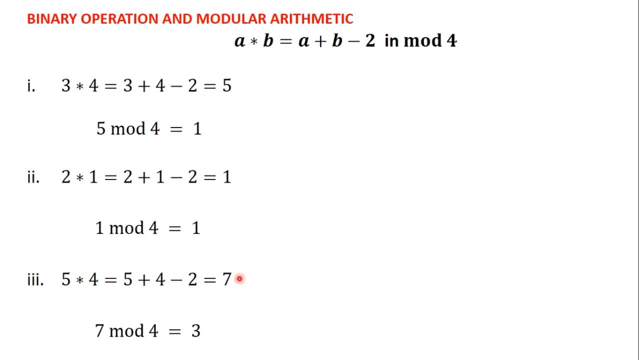 star four and we got seven. after that, we find the value of seven in mode four. Seven mode four will give us three. Thank you for watching this video. Subscribe to this channel for more videos. in this video, We have learned how to solve questions involving binary operation and modular arithmetic. in the next video, 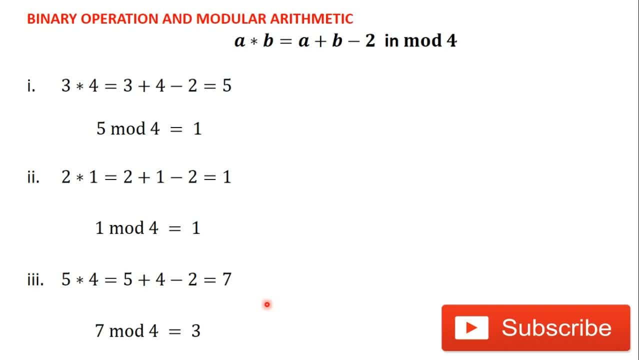 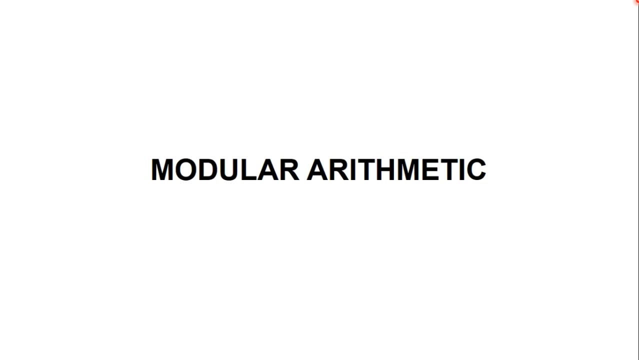 We are going to apply what you have studied in this video To solve a question on drawing tables for binary operation in a given modulus. bye, bye, welcome back. we are still on the topic: modular arithmetic. in the previous video we learned how to solve questions involving modular arithmetic and 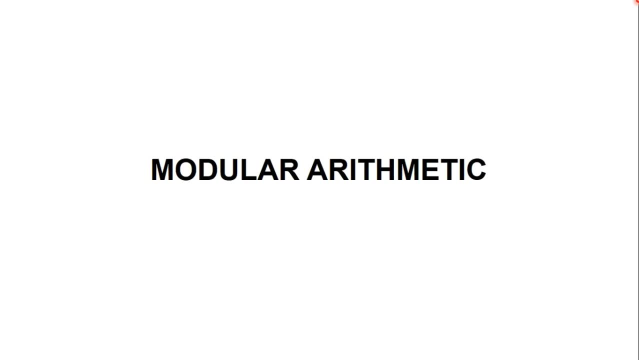 binary operation. in this video we are going to apply what we studied in the previous video to solve a question on drawing a table for a given binary operation in a given modulus. the question for this video is the operation star is defined by x, star y is equal to x, y plus 2 in. 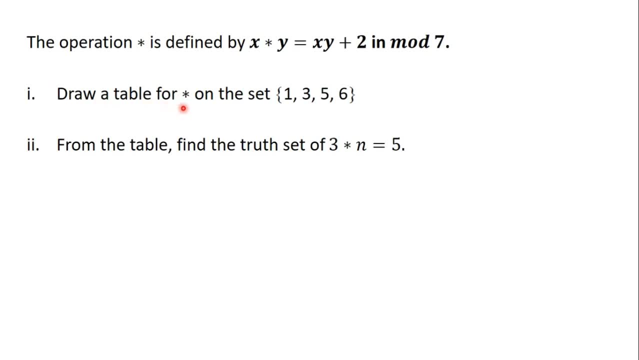 mode 7. i draw a table for star on the set 1, 3, 5, 6, i. i from the table find the truth: set of 3, star n is equal to 5.. so in this question the operation star has been defined for us as x. star y is equal. 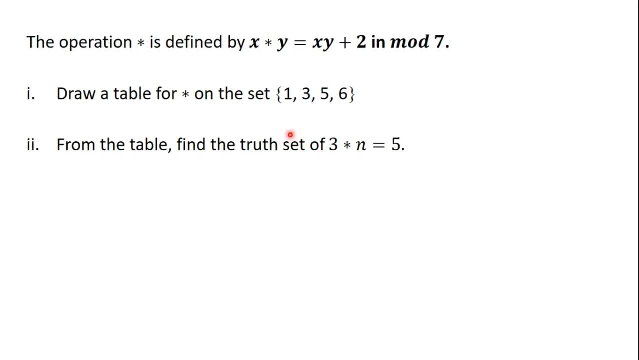 to x, y plus 2 in mode 7.. we have been asked to draw a table for star on the set 1, 3, 5, 6 and after that we will use our table to find the truth. set of the equation 3, star n is equal to 5.. 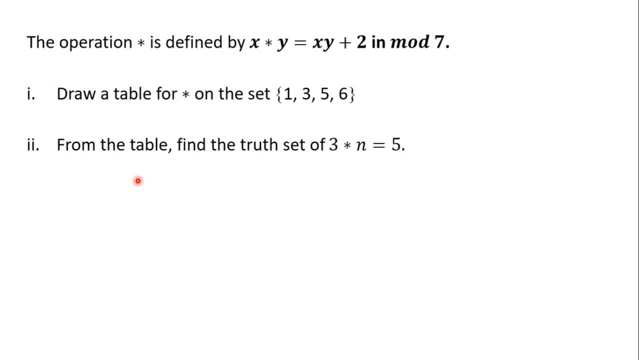 we have the first part in this video and in the next video we will use the table that you draw to find the truth. set of 3, star n is equal to 5.. so let's begin by drawing the table for star on the set. 1, 3, 5, 6. we have been given a set of numbers in the question. the set is one, three, five, six, so we 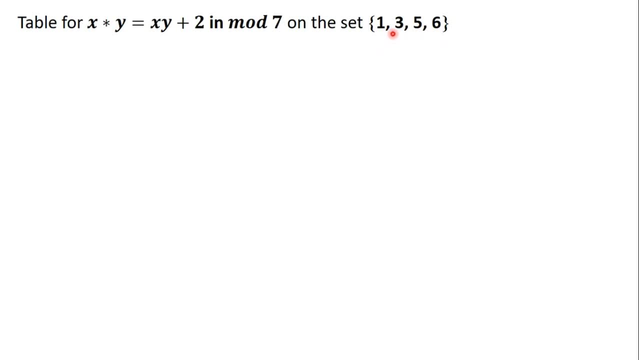 are going to use this set to draw the table values in the set. so we are going to draw a table with five columns and five rows. in the first cell you indicate the operation you are going to perform. the operation is star, so you indicate star in the first cell, then you list the. 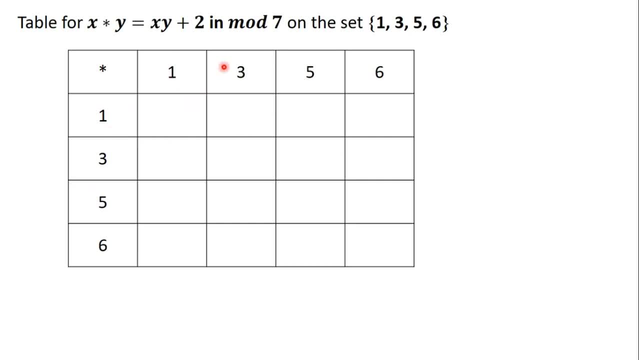 members. in the first row and the first column we have 1, 3, 5, 6 and 1, 3, 5, 6. the definition of star is X. star Y is equal to X, Y plus 2, so X star Y is equal to X. 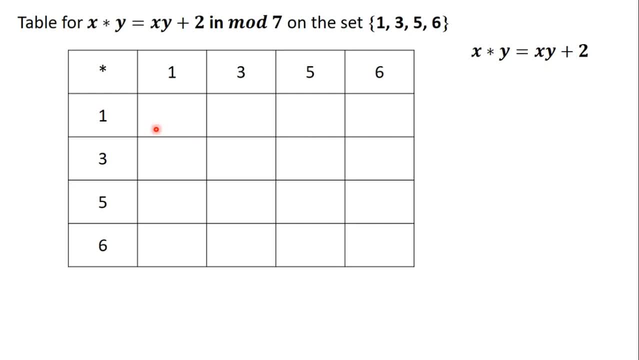 times Y plus 2. let's fill the table. the first one is 1 star 1, so it means that X is 1 and Y is 1, so 1 star 1 will be equal to X- Y, which is X times Y, so 1. 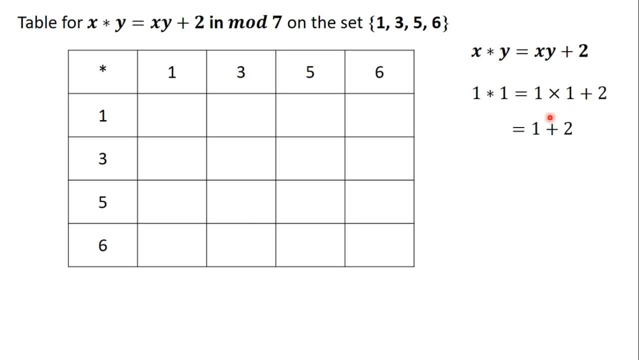 times 1 plus 2, 1 times 1 is 1, so you have 1 plus 2, and 1 plus 2 give us 3, but remember that the operation star is defined in mood 7, so after you have found 1 star, 1, you have. 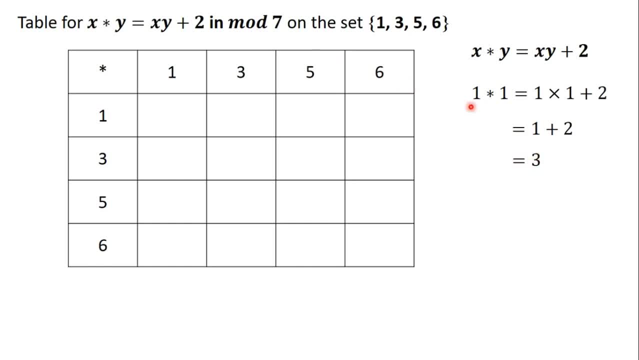 to find the value of 1 star 1 in mode 7. 1 star 1 is 3, so you have to find 3 in mood 7, 3 in mode 7 is equal to 3, that means that 1 star 1 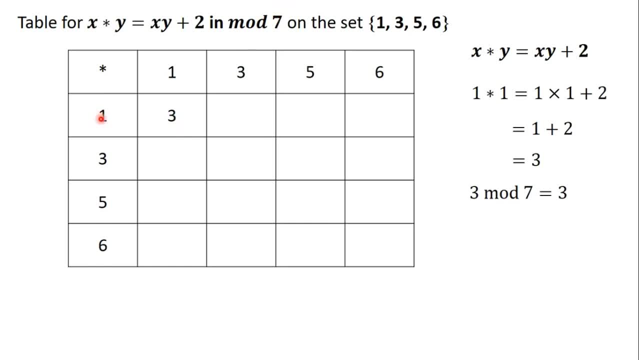 in mood, 7, 7 is 3.. The next one is 1 star 3.. 1 star 3 will be equal to 1 times 3 plus 2, because x is 1 and y is 3. So you have 1 times 3 plus 2.. 1 times 3 is 3.. 3 plus 2 will give us 5.. So we have now found. 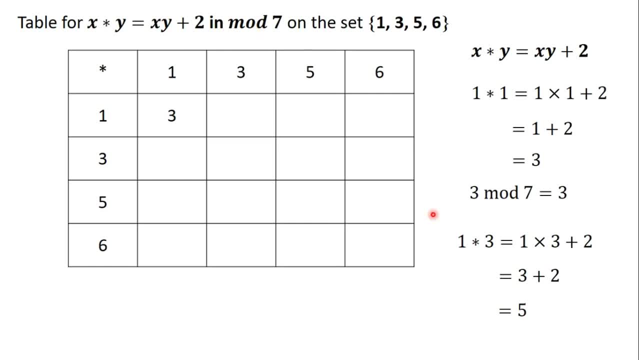 1 star 3.. But the operation is defined in mode 7.. So we have to find the value of 1 star 3 in mode 7.. 1 star 3 is 5.. 5 in mode 7 will give us 5.. Let's move on. The next one is 1 star 5.. 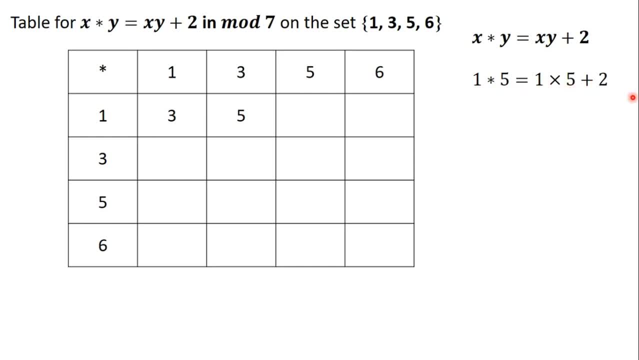 1 star 5 will be equal to 1 times 5 plus 2.. 1 times 5 is 5.. So we have 5 plus 2.. And 5 plus 2 will give us 7.. We will find 7 in mode 7, since the operation is defined in mode 7.. 7 mode 7 is 0. So 1 star 5. 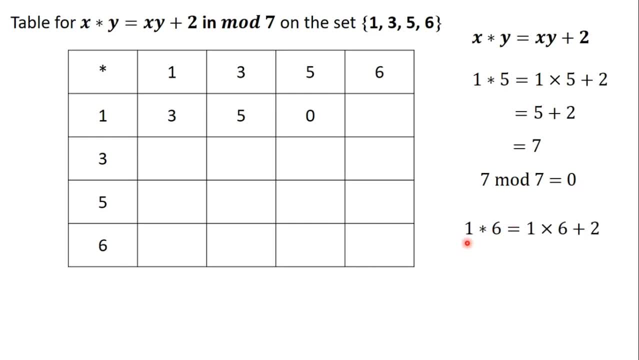 mode 7 is 0.. The next one is 1 star 6.. 1 star 6 is equal to 1 times 6 plus 2.. 1 times 6 is 6.. 6 plus 2 is 8.. We will find 8 in mode 7.. 8 mode 7 is 1.. 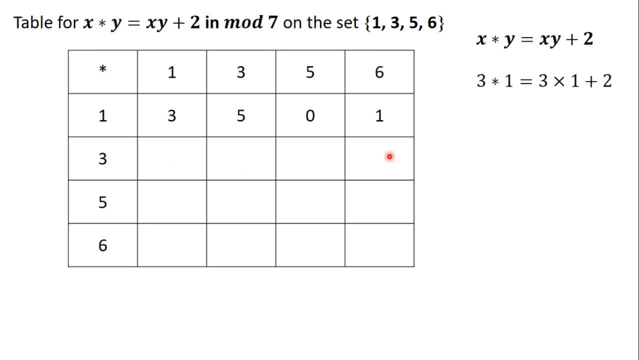 Let's move on. Let's move on to the next rule: 3 star 1.. 3 star 1 will be equal to 3 times 1 plus 2, because x is 3 and y is 1.. So 3 times 1 plus 2.. 3 times 1 is 3.. You have 3 plus 2.. And 3 plus 2 will give us 5.. 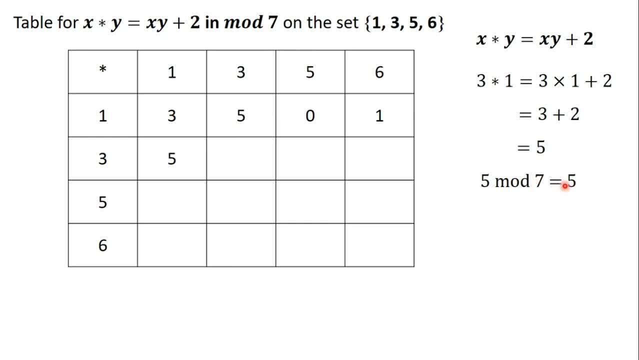 Then you find 5 in mode 7.. 5 mode 7 will give us 5.. The next one is 3 star 3.. 3 star 3 will give us 3 times 3 plus 2.. 3 times 3 will give us 9.. 9 plus 2 will give us 11.. You will find 11 in mode 7.. 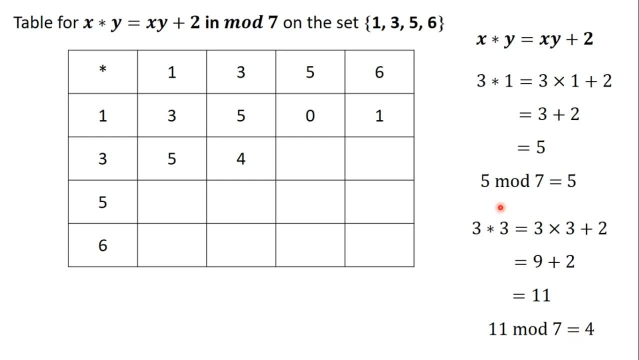 11. mode 7 will give us 4.. The next one is 3 star 5.. 3 star 5 will give us 3 times 5 plus 2.. 3 times 5 is 15.. 15 plus 2 is 17.. You will find. 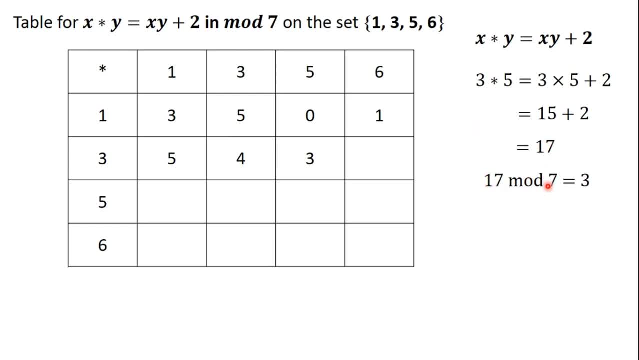 17 mode 7. And 17 mode 7 is equal to 3.. The next one is 3 star 6.. 3 star 6 will be equal to 3 times 6 plus 2.. 3 times 6 is 18.. 18 plus 2 will give us 20.. You will find 20 mode 7. And 20 mode. 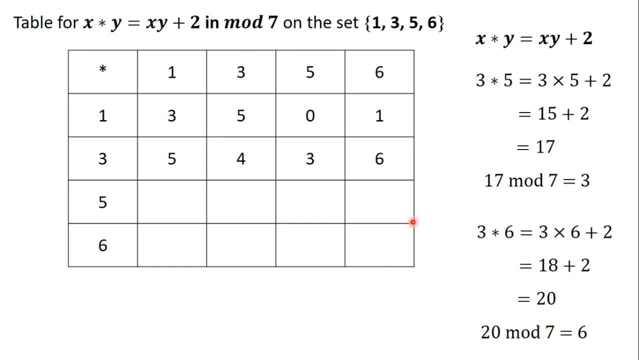 7 is equal to 6.. Let's move on to the next rule: 5 star 1.. 5 star 1 will be equal to 5 times 1 plus 2. Because x is 5 and y is 1. So you have 5 times 1 plus 2.. 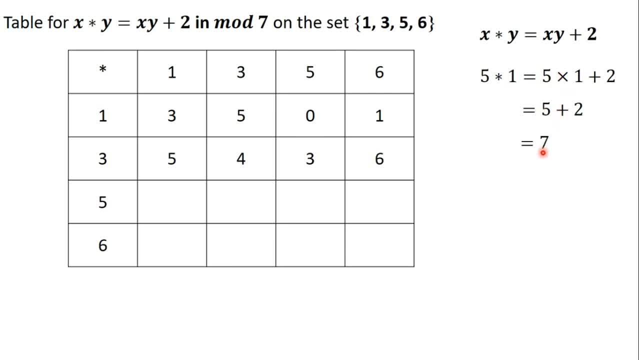 5 times 1 is 5.. 5 plus 2 will give us 7.. 7 mode 7 is 0.. The next one is 5 star 3.. 5 star 3 is equal to 5 times 3 plus 2.. 5 times 3 is 15.. 15 plus 2 will give us 17.. We will find 17 mod 7 and 17 mod 7. 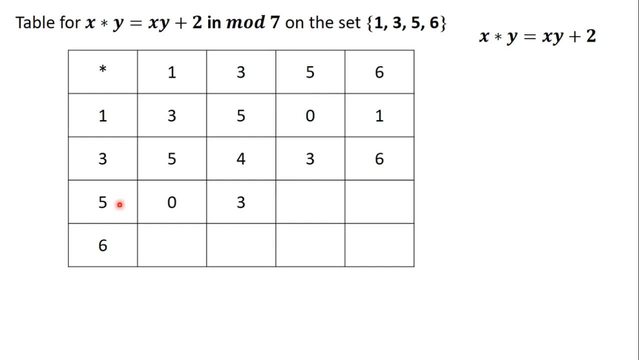 is equal to 3.. The next one is 5 star 5.. 5 star 5 is equal to 5 times 5 plus 2.. 5 times 5 will give us 25.. 25 plus 2 will give us 27.. We will find 27 in mod 7, and 27 mod 7 is equal to 6.. The next one: 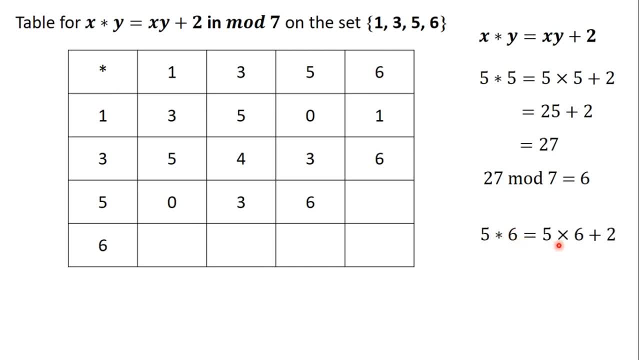 is 5 star 6.. 5 star 6 is equal to 5 times 6 plus 2.. 5 times 6 is 30.. 30 plus 2 is 32.. We will find 32 mod 7, and 32 mod 7 is equal to 5.. 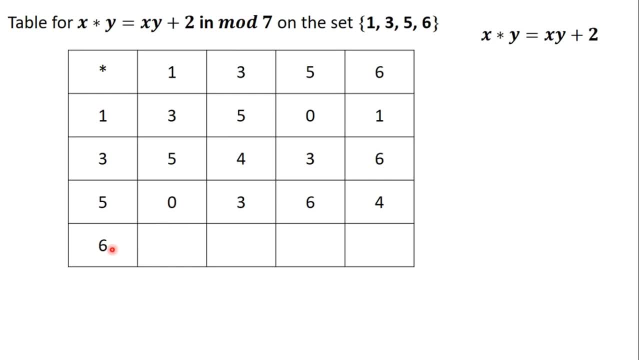 4.. Let's move on to the last rule: 6 star 1.. 6 star 1 is equal to 6 times 1 plus 2.. 6 times 1 is 6.. 6 plus 2 is 8.. 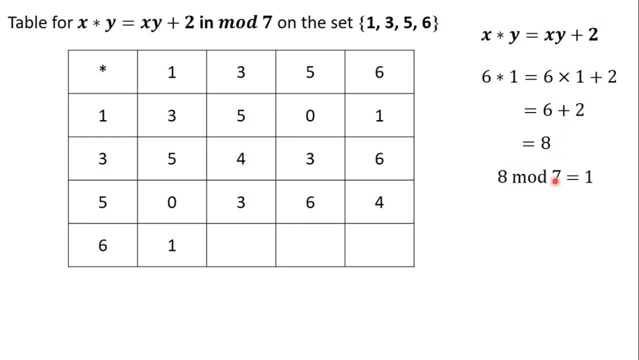 We will find 8 in mod 7.. 8 mod 7 is 1.. 6 star 3 is equal to 6 times 2 plus 2.. 6 times 2 is is 18, 18 plus 2 is 20. you find 20 in mod 7. 20 mod 7 is equal to 6. the next one is 6 star 5. 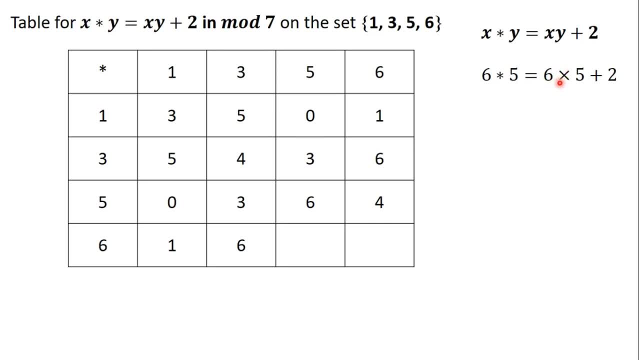 6 star 5 is equal to 6 times 5 plus 2. 6 times 5 is 30. 30 plus 2 is 32. 32 mod 7 is 4, and the last one is 6 star 6. 6 star 6 is equal to 6 times 6 plus 2. 6 times 6 is 36. 36 plus 2 is 38. 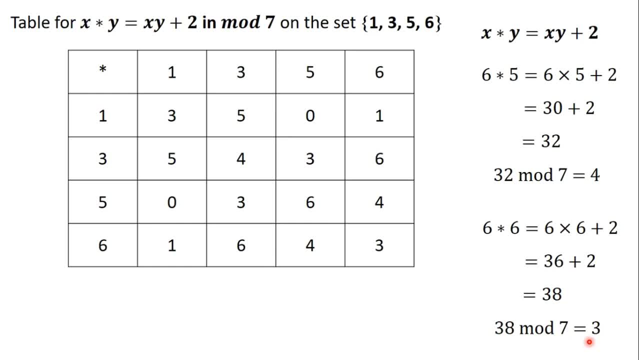 and 38, mode 7, is equal to 3.. we have now completed the table for star, which is defined as x. star y is equal to x, y plus 2 in mode 7 on the set 1, 3, 5, 6.. the next part of the question says that we should use our table to find the truth set. 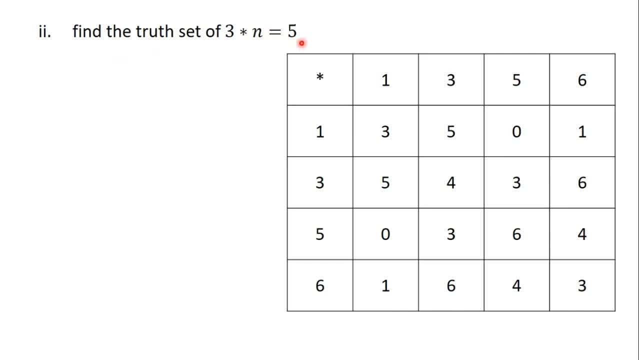 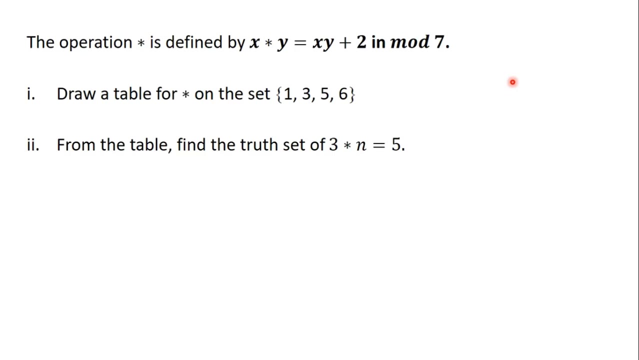 of the equation 3, star n is equal to 5.. we are going to do that in the next video, so we'll see in the next video and let's continue solving the question. bye, bye, welcome back. we started solving this question in the previous video and we drew the table for star on the set 1. 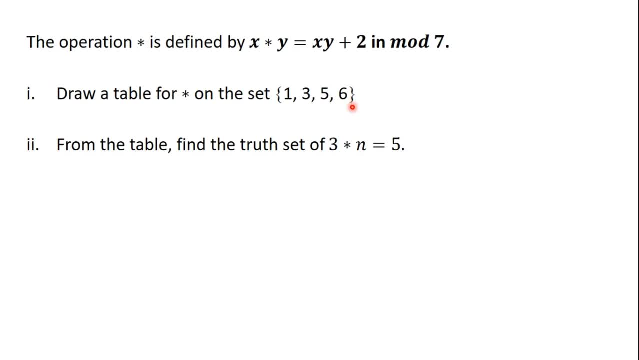 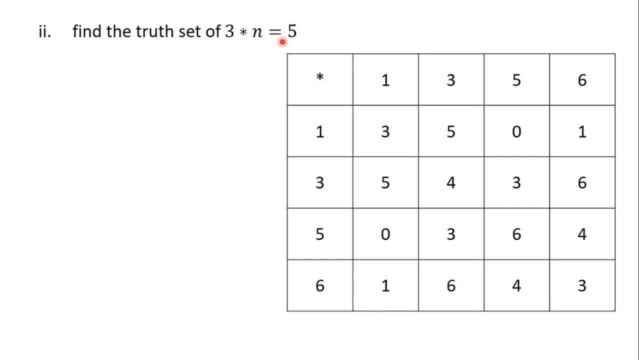 3, 5, 6.. in this video we are going to use the table we drew in the previous video to find the truth set of the equation 3 star n is equal to 5.. so we are going to use this table to find the truth set of 3 star n is equal to 5.. we drew the table for the operation star on the set. 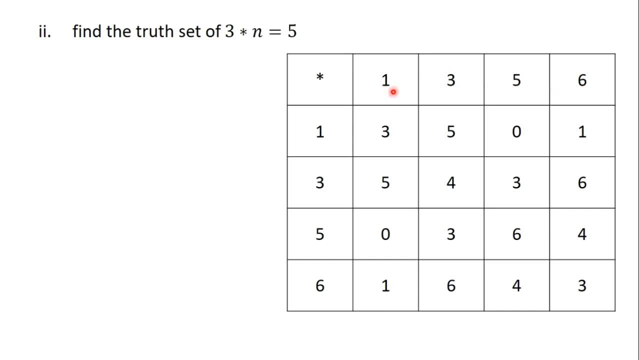 1, 3, 5, 6.. there are some values in this set that will satisfy the equation 3 star n is equal to 5.. equation 3, star n is equal to 5.. To find those values, we are going to try them out one after. 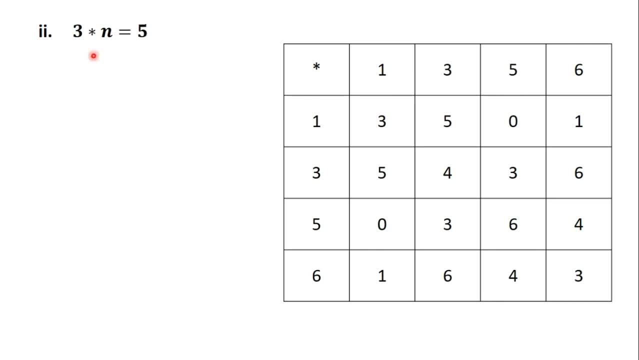 the other. We will begin with the first one, which is 1.. Remember that the equation is 3 star n is equal to 5.. When n is equal to 1, the expression 3 star n will be equal to 3 star 1.. From the table, 3 star 1 will give us 5.. So from the table we can see that 3. 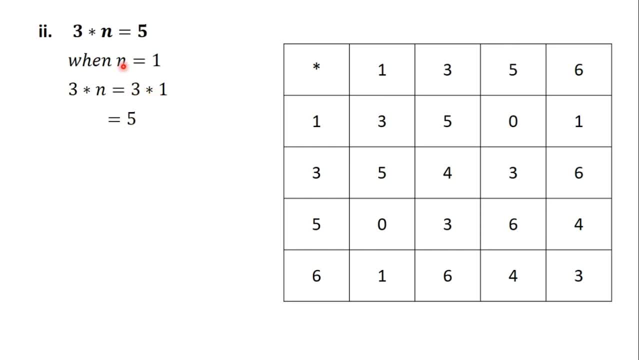 star 1 is equal to 5.. That means that when n is equal to 1,, 3 star 1 will be equal to 5.. So 1 will satisfy this equation. So n is equal to 1.. Let's try out the other numbers. 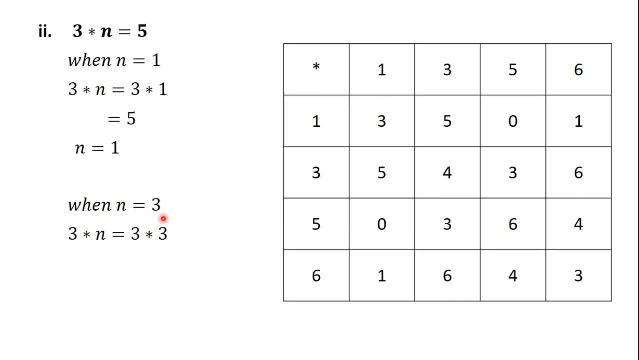 and see. The next one is 3.. When n is equal to 3, the expression 3 star n will be equal to 3 star 3.. From the table, 3 star 3 is equal to 4.. But we know that from the equation, 3 star n should give us 5. When 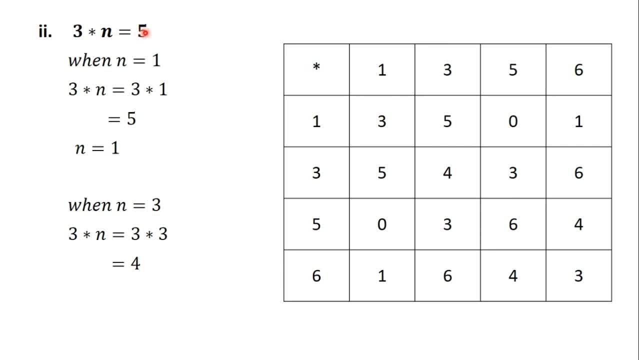 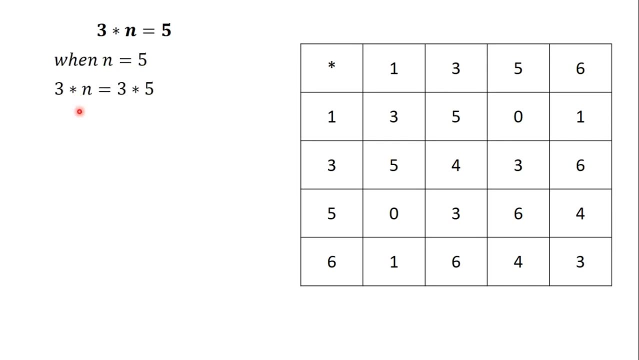 n is equal to 3, 3 star 3 is giving us 4.. That means that n is equal to 3 will not satisfy this equation, So n is not equal to 3.. Let's try the next one: 5.. When n is equal to 5, the expression 3 star n will be equal. 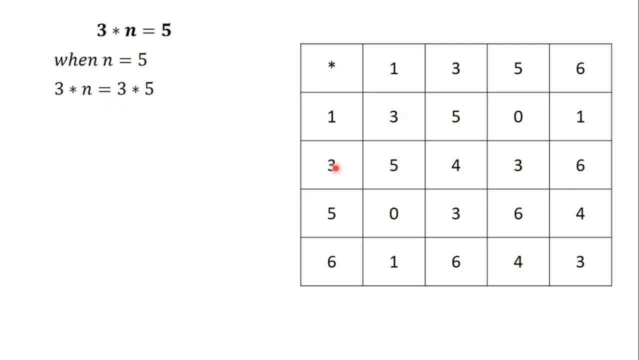 to 3 star 5.. From the table, 3 star 5 will give us 3.. So 3 star 5 is 3.. But from our equation we know that 3 star n should give us 5.. When n is equal to 5, 3 star 5 is giving. 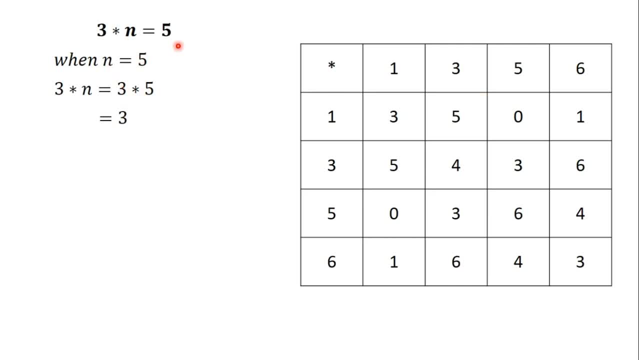 three- that means that n is equal to five- will not satisfy the equation. so n is not equal to five. let's try the last one and see if it will satisfy the equation. the last one is six. when n is equal to six, when n is equal to six, three star n will be equal to three star six from the table three. 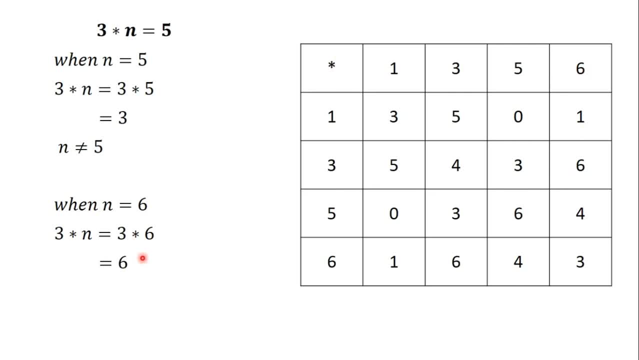 star six is six. so three star six is equal to six. but for my equation three star n should give us five. when n is equal to six, three star six is given as six. six is not equal to five. that means that n is equal to six. will not satisfy the equation, so n is not equal to six, so the only 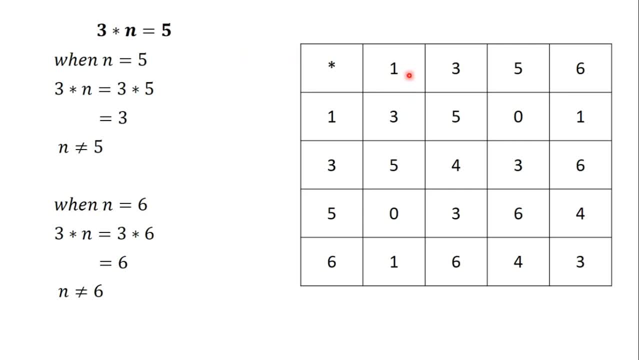 number in the set that satisfied the equation was one. the question said we should find the truth set. so the truth set of the equation, three star n is equal to five, is equal to n, is such that n is equal to one. remember that it is a truth set. so you are going. 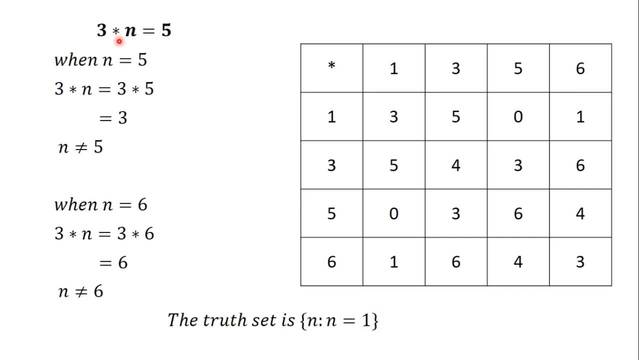 to write your answer in a carry bracket. so the truth set of this equation is: n is such that n is equal to one. thank you for watching this video. subscribe to this channel for more videos in the future. we are going to solve another question on drawing a table for a binary operation in a given 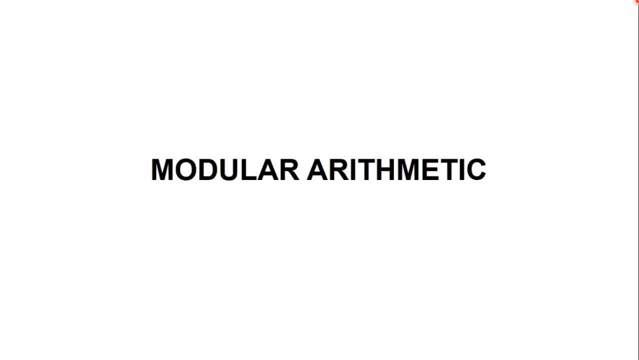 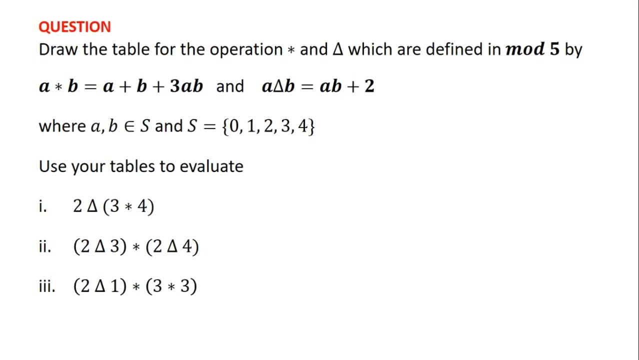 modulus. bye, bye, welcome back. we are still on the topic modular arithmetic. in the previous video we solved a question on drawing a table for a binary operation in a given modulus. in this video we are going to solve another question. the question for this video is not Arguing as a abortifact, gelT. 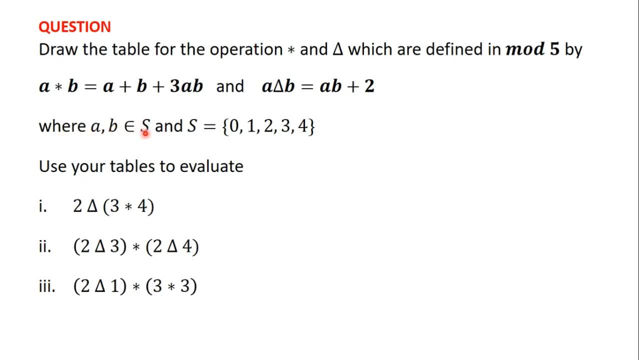 we are going to solve another question on drawing a table for a binary operation in a given modulus in this video. we are going to solve another question on drawing a table for a linear operation in a given modulus in this video: 1, 2, 3, 4.. Use your tables to evaluate i: 2 delta into brackets: 3, star 4, ii: 2 delta. 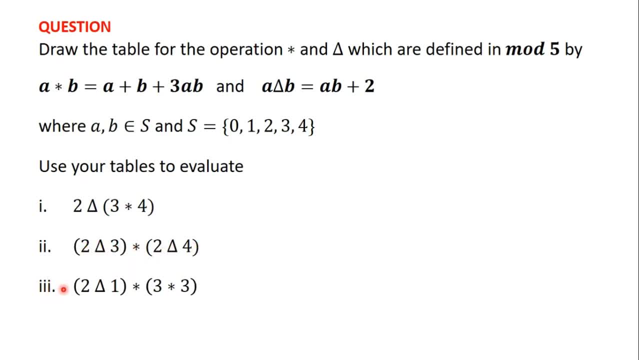 3- star 2 delta 4, iii- 2 delta 4. star 3 delta 3.. So we are being asked to draw two tables. We will draw one for star, which is defined as a star. b is equal to a plus b plus 3ab. 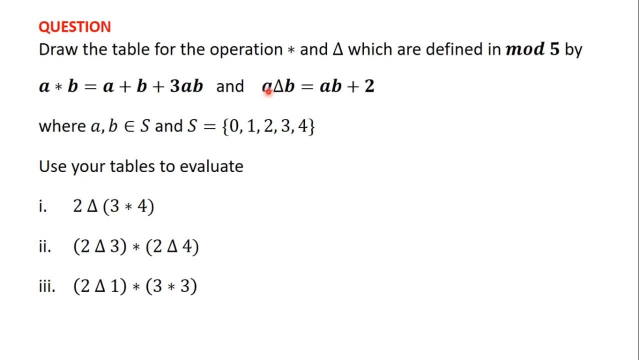 and then we will draw another one for delta, which is defined as a delta. b is equal to ab plus 2, where a and b belongs to the set S and the set S is given as 0,, 1,, 2,, 3,, 4.. 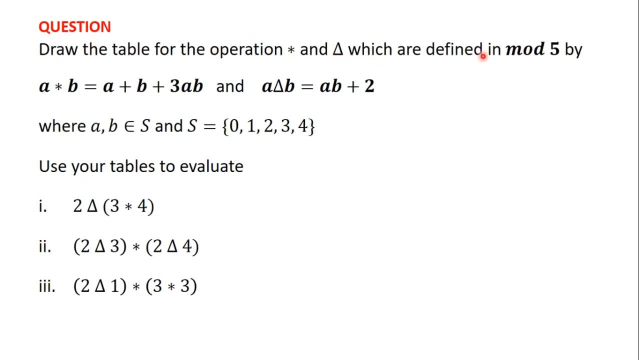 Note that the operations star and delta are defined in mode 5.. So we are going to use the definition for star and delta to draw a table for the set 0,, 1,, 2,, 3, 4 in mode 5.. After that, we will use the 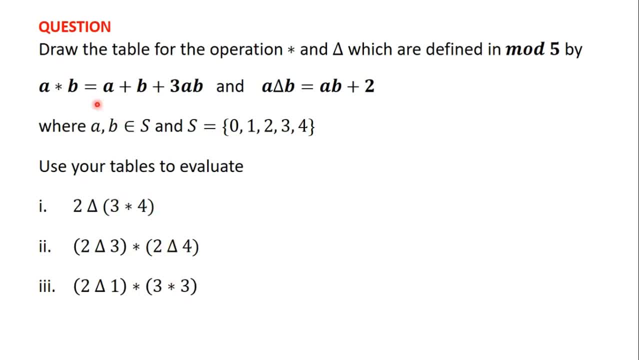 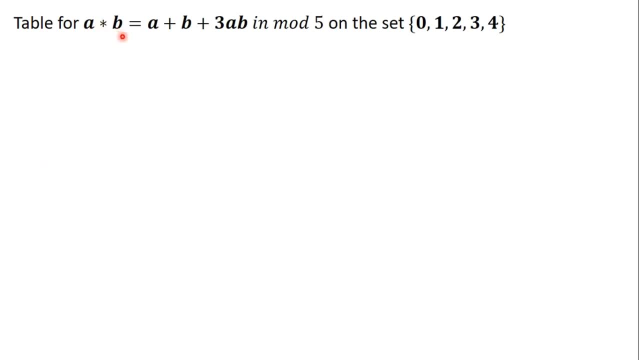 tables to evaluate the following. Let's begin by drawing the table for star. The definition for star is: a star b is equal to a plus b plus 3ab. A star b is equal to a plus b plus 3ab and a plus 2ab. A star b is equal to a plus b. 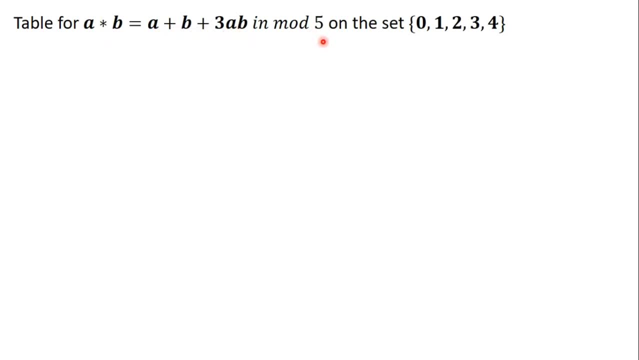 plus 3ab in mode 5 on the set S, which is 0,, 1,, 2,, 3, 4.. So we have been given a set of values in the question. We are going to use that set of values to draw the table. Remember. 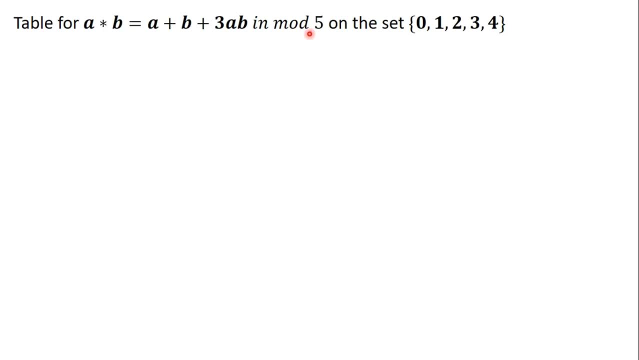 that we are drawing a table for star in mode 5.. We have 5 values in the set, so we will draw a table with 6 columns and 6 rules. In the first cell you indicate the operation you are going to perform. The operation is star, so you indicate star in the first cell. 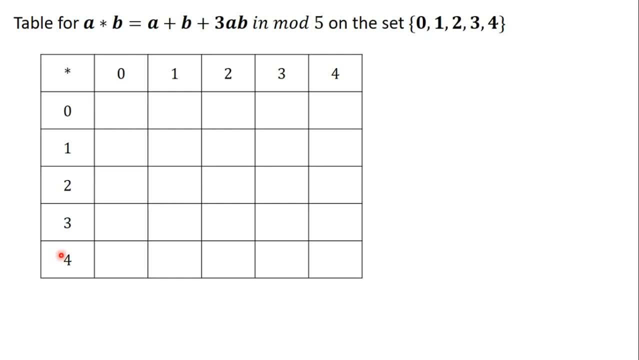 Then you list the set of numbers in the first rule and the first column. The definition of star is a star. b is equal to a plus b plus 3ab. That means that the first number plus the second number plus 3ab is equal to a plus b plus 3ab. 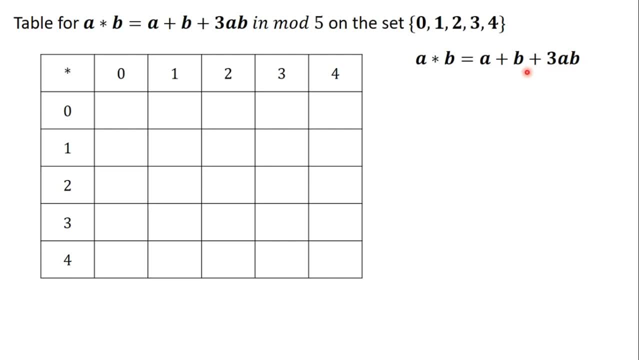 So we have 3 times the first number times the second number. Let's fill the table. The first one is 0 star 0.. 0 star 00 is equal to 0 plus 0 plus 3 times 0 times 0, because 3ab is the same as 3 times a times b. So 0 star 0 is equal to 0 plus. 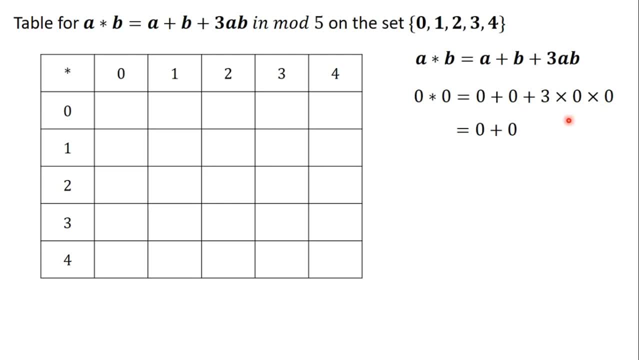 0 plus 3 times 0 times 0.. And this will give us 0 star 0.. 0 plus 0.. 0 plus 0 is 0.. You will find 0 in mode 5, because star is defined in mode 5.. 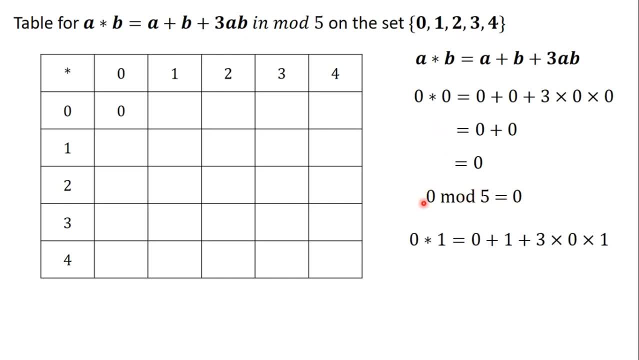 0 in mode 5 is 0.. Let's move on to the next one: 0 star- 1.. 0 star 1 will be equal to 0 plus 1 plus 3 times 0 times 1.. 0 plus 1 is 1.. 3 times 0 times 1 is 0.. 1 plus 0 is 1.. 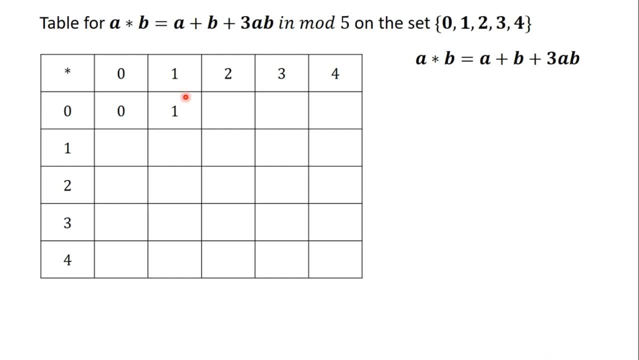 And 1 in mode 5 is 1.. The next one is 0 star 2.. 0 star 2 is equal to 0 plus 2 plus 3 times 0 times 2.. 0 plus 2 is 2.. 3 times 0 times 2 will give us 0.. 2 plus 0 is 2.. 2 in mode 5 is 2.. 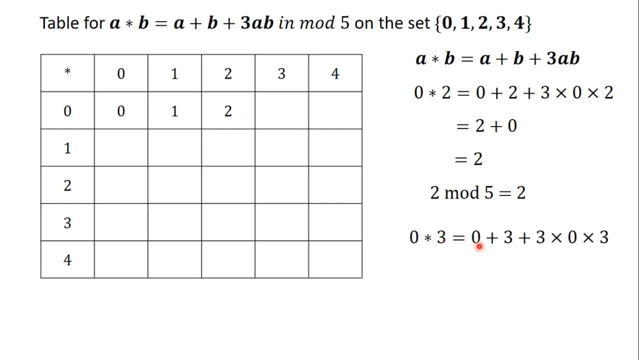 The next one is 0 star 3.. 0 star 3 is equal to 0 plus 3.. Plus 3 times 0 times 3.. 3 plus 0 will give us 3.. 3 times 0 times 3 is 0.. 3 plus 0 will give. 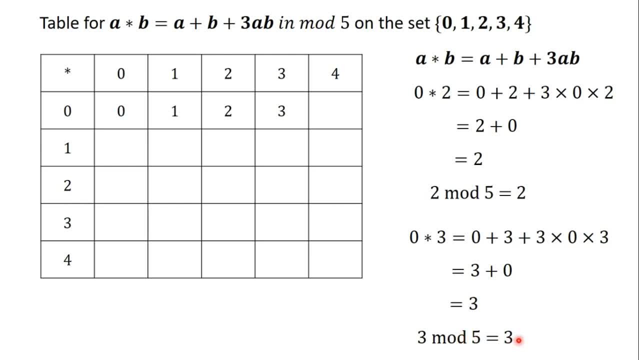 us 3.. 3 in mode 5 is 3.. The next one is 0 star 4.. 0 star 4 will be equal to 0 plus 4 plus 3 times 0 times 4.. 0 plus 4 is 4.. 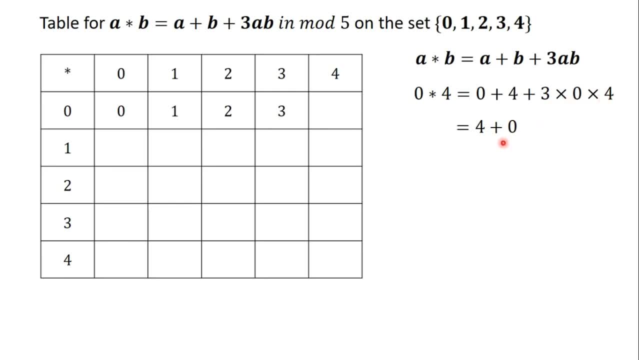 4.. 3 times 0 times 4 will give us 0.. 4 plus 0 is 4.. And 4 in mode 5 is 4.. Let's move on to the next rule: 1 star 0.. 1 star 0 will be equal to 1 plus 0 plus 3 times 1 times. 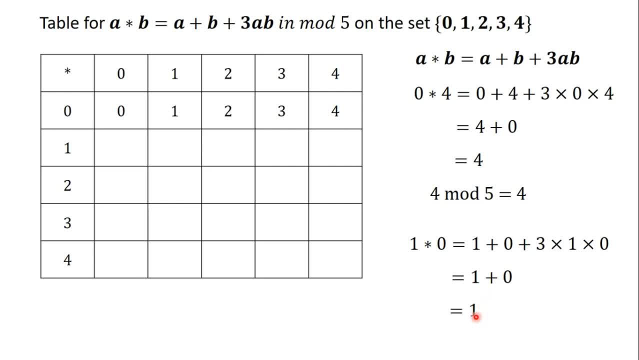 0. And this will be equal to 1 plus 0.. 1 plus 0 is 1.. 1 in mode 5 is 1.. The next one is 1 star 1.. 1 star 1 is equal to 1 plus 1 plus 3 times 1 times 1.. And this will give us 2. 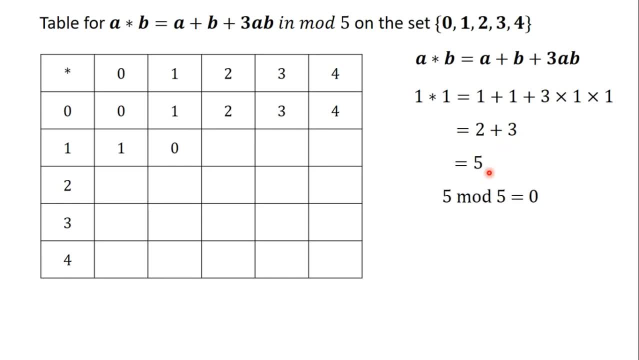 plus 3.. 2 plus 3 is 5.. 5 in mode 5 is 0.. The next one is 1 star 2.. 1 star 2 is equal to 1 plus 2 plus 3 times 1 times 2.. This will give us 3 plus 6.. 3 plus 6 is 9.. And 2 in. 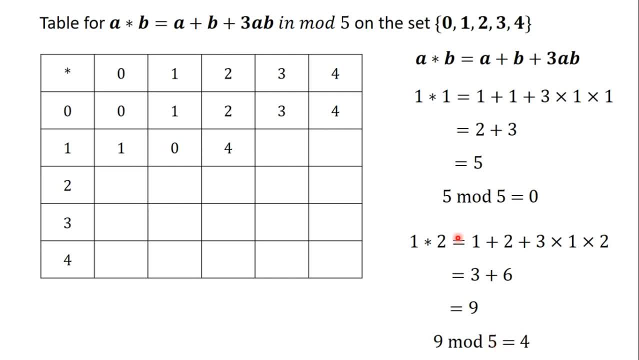 and 9 in mode 5 is 4.. The next one is 1 star 3.. 1 star 3 is equal to 1 plus 3 plus 3 times 1 times 3.. 1 plus 3 is 4.. 3 times 1 times 3 is 9.. 4 plus 9 will give us 13.. 13 in mode 5 is 3.. 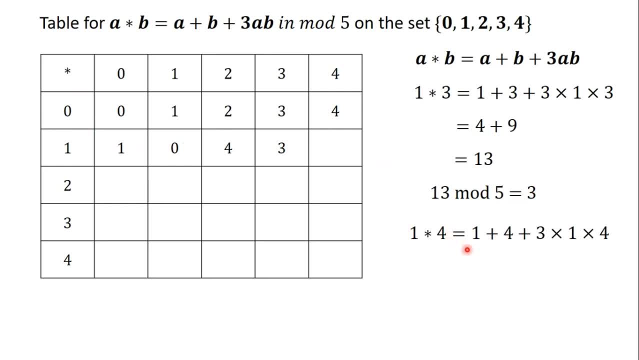 1 star 4.. 1 star 4 is equal to 1 plus 4 plus 3 times 1 times 4.. 1 plus 4 is 5.. 3 times 1 times 4 is 12.. 5 plus 12 will give us 17.. 17 in mode 5 is 2.. The next one is 2 star 0.. 2 star 0 is equal. 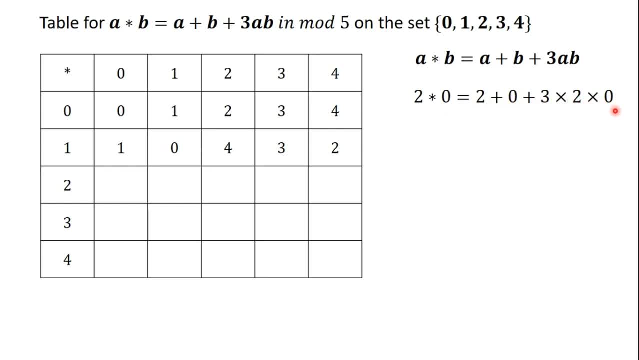 to 2 plus 0 plus 3 times 2 times 0. This will give us 2 plus 0, and 2 plus 0 is equal to 2.. 2 mode 5 is 2.. The next one is 2 star 1.. 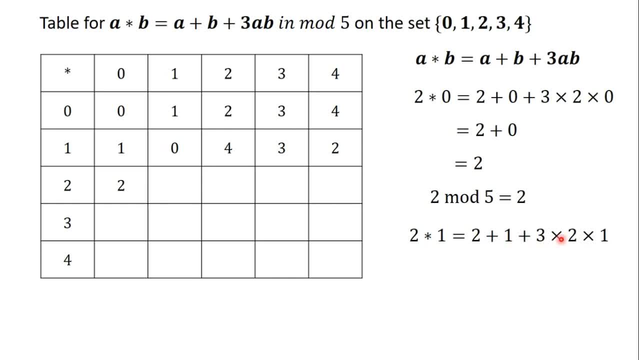 2 star 1 is equal to 2 plus 1 plus 3 times 2 times 1, and this is equal to 3 plus 6.. 3 plus 6 is 9.. 9 mode 5 is 4.. 2 star 2.. 2 star 2 is equal to 2 plus 1 plus 3 times 2 times 1.. 2 star 2 is equal to. 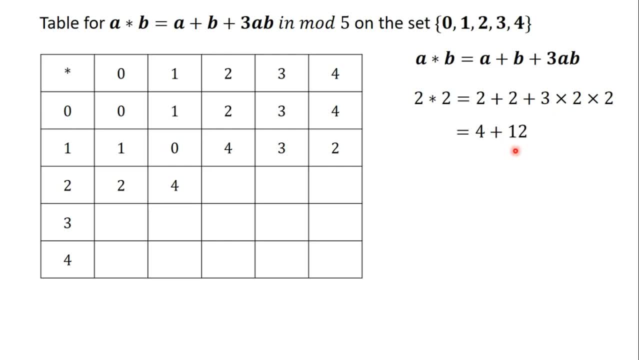 2 plus 2 plus 3 times 2 times 2.. This will be equal to 4 plus 12.. 4 plus 12 is 16.. 16 with 5 is 1.. The next one is 2 star, 3.. 2 star 3 is equal to 2 plus 3 plus 3 times 2 times. 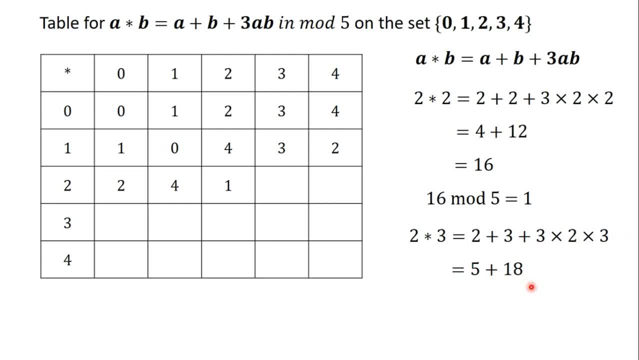 3. And this is equal to 5 plus 18.. 5 plus 18 is 23.. 23 with 5 is 3.. The next one is 2 star 4.. 2 star 4 is equal to 2 plus 4 plus 3 times 2 times 4.. 2 plus 4 is 6. 3 times. 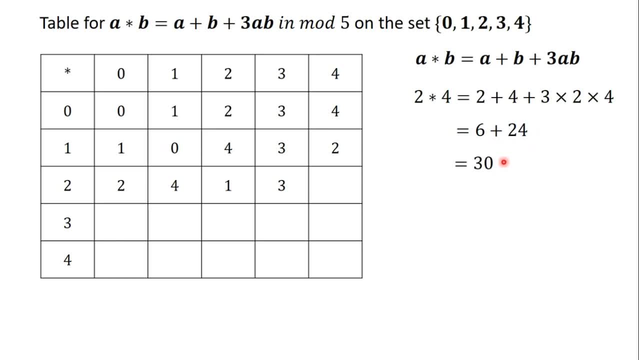 2 times 4 is 24.. 6 plus 24 is 30.. 30 with 5 is 0.. Let's move on to the next rule: 3 star 0.. 3 star 0 will give us 3 plus 0 plus 3 times. 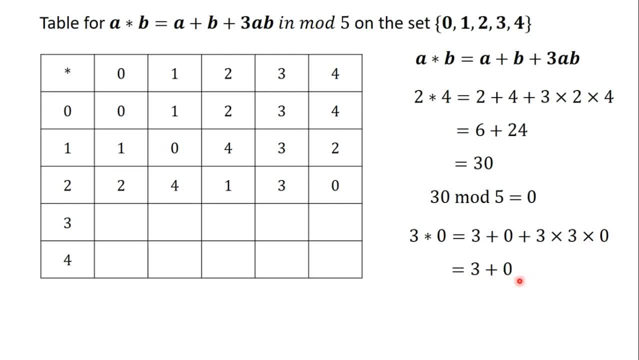 3 times 0. And this will give us 3 plus 0.. 3 plus 0 is 3.. 3 with 5 is 3.. 3 star 1.. 3 star 1 is equal to 3 plus 1 plus 3 times 3 times 1.. And it's equal to 4 plus 1 plus 3 times. 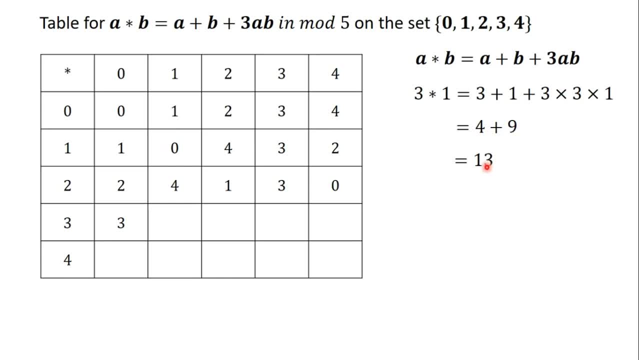 3 times 1.. And it's equal to 4 plus 1 plus 3 times 3 times 1.. And it's equal to 4 plus 4 plus 9,. 4 plus 9 will give us 13,. 13 multiplied by 5 is 3.. 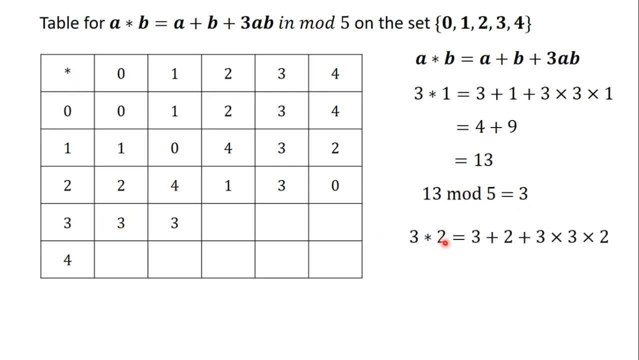 The next one is 3 star 2, 3 star 2 is equal to 3 plus 2 plus 3 times 3 times 2, and it will give us 5 plus 18, 5 plus 18 is 23,. 23 multiplied by 5 is 3.. 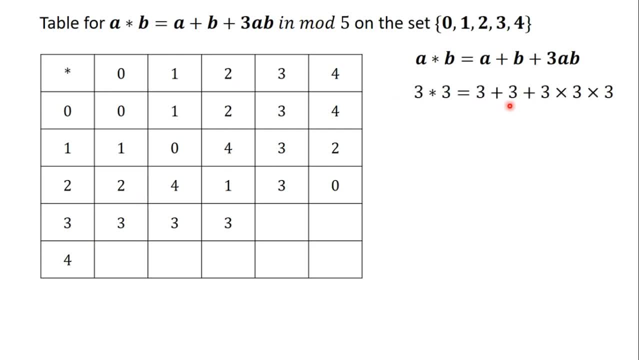 The next one is 3 star 3, 3 star 3 will give us 3 plus 3 plus 3 times 3 times 3, 3 plus 3 will give us 6, 3 times 3 times 3 will give us 27,. 6 plus 27 is 33, 33 multiplied by 5. 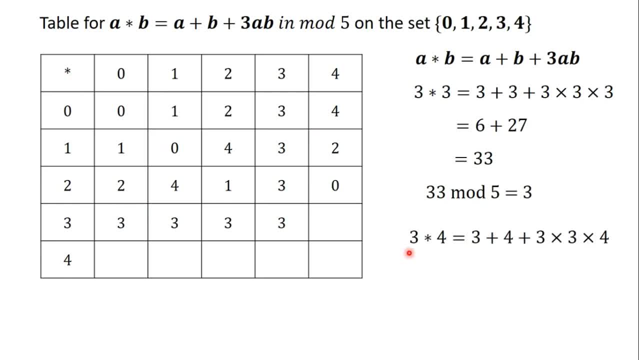 is 3.. The next one is 3 star 4, 3 star 4 is equal to 3 plus 4 plus 3 times 3 times 3 plus 3 times 4, and it will give us 7 plus 36,. 7 plus 36 is 43,. 43 multiplied by 5 is 3.. 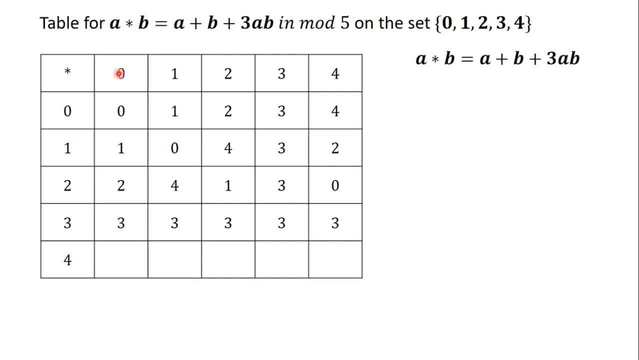 We move on to the last rule: 4 star 0, 4 star 0 is equal to 4 plus 0 plus 3 times 4 times 0, and it will give us 4 plus 0,. 4 plus 0 is 4.. 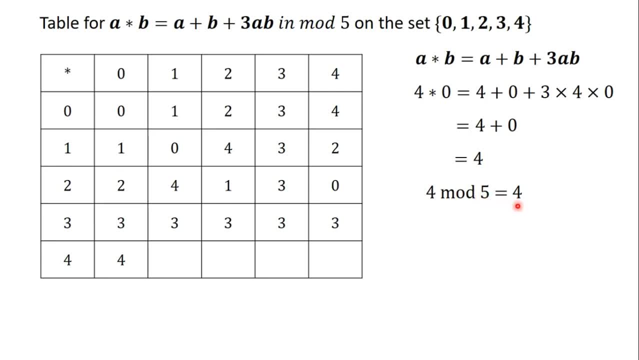 4 multiplied by 5 is 4.. 4 multiplied by 5 is 4. 4 star 1, 4 star 1 is equal to 4 plus 1 plus 3 times 4 times 1, 4 plus 1 is 5, 3 times. 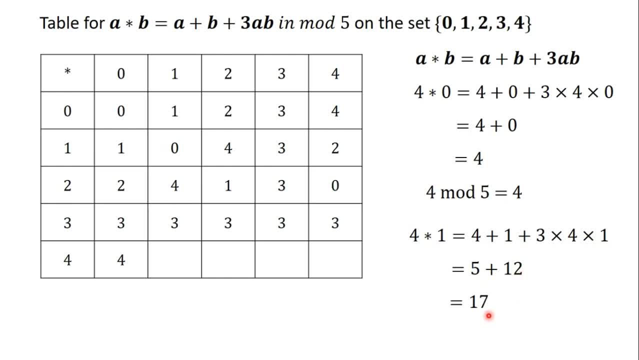 4 times 1 is 12, 5 plus 12 will give us 17, and 17 in mode 5 or 17 mode 5 is 2.. The next one is 4 star 2.. 4 star 2 is equal to 4 plus 1 plus 3 times 3 times 3 times 3 plus 3 times 3 plus 3 times. 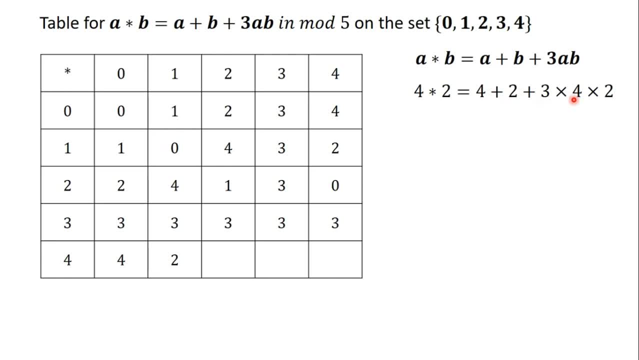 2. 4 plus 1 is equal to 4 plus 2 plus 3 times 4 times 2.. 4 plus 2 is 6.. 3 times 4 times 2 is 24.. 6 plus 24 is 30.. 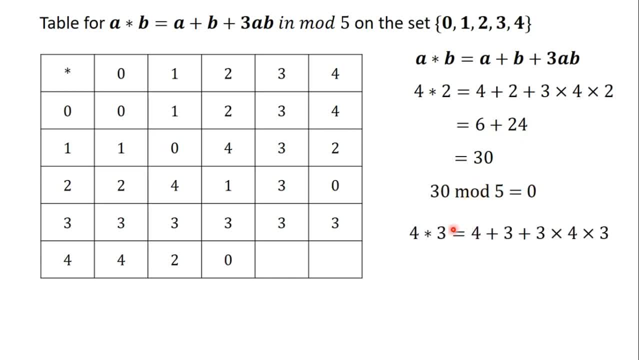 30 move. 5 is 0.. The next one is 4 star 3.. 4 star 3 is equal to 4 plus 3 plus 3 times 4 times 3. And we will have 7 plus 3.. 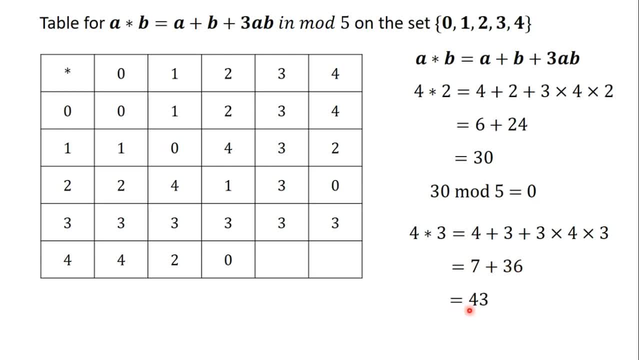 4 star 3 is equal to 4 plus 3 plus 3 times 4 times 3.. 36, 7 plus 36 is 43, 43 move 5 is 3 and the last one is 4 star 4, 4 star 4 is equal to. 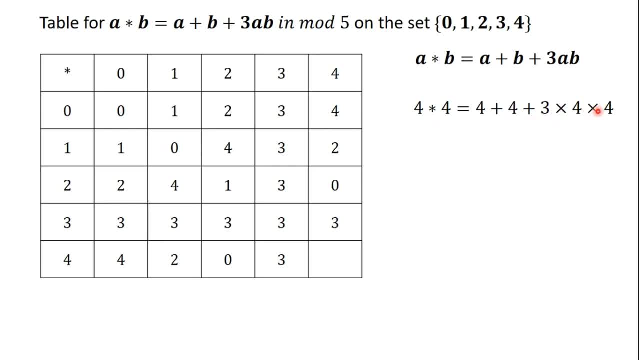 4 plus 4 plus 3 times 4 times 4,. 4 plus 4 is 8,. 3 times 4 times 4 will give us 48,. 8 plus 48 is 56, and 56 move 5 is 1.. So we have now completed the table for star, which is: 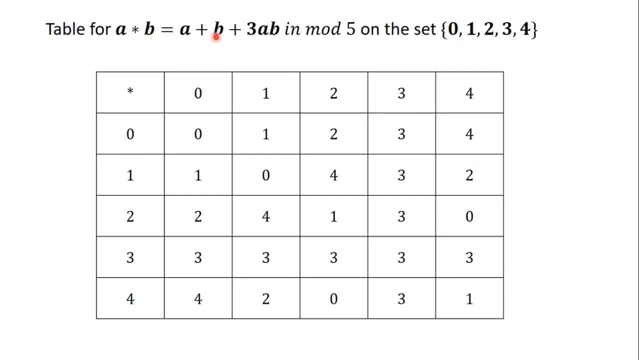 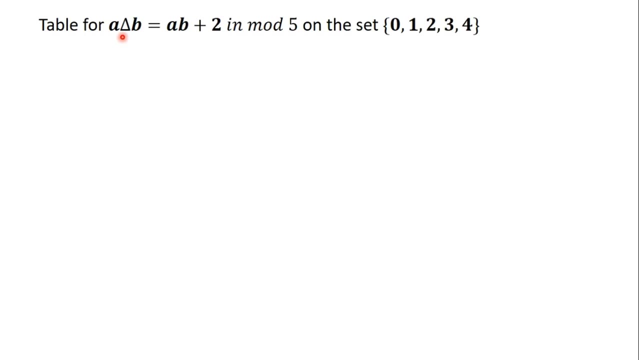 defined as a star b is equal to a plus b plus 3ab in mode 5 on the set 0,, 1,, 2,, 3, 4.. The question said that we should draw a table for delta, which is defined as a delta b is. 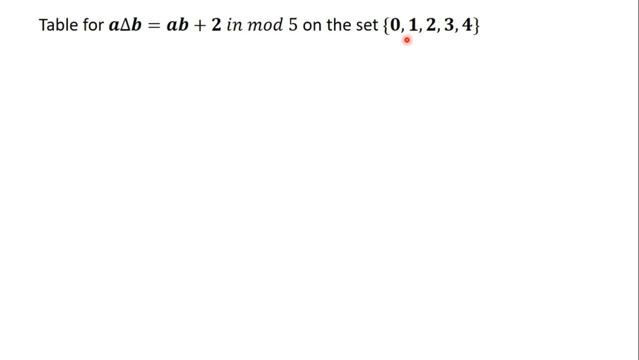 equal to ab plus 2.. In mode 5, on the set 0,, 1,, 2,, 3,, 4.. We are going to do that in the next video. So you see, in the next video and let's continue with the solution. Bye, bye. 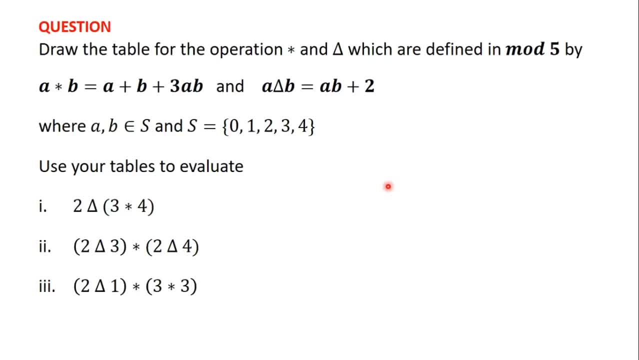 Welcome back. We started solving this question in the previous video. We drew the table for star, which is defined as a star. b is equal to a plus b plus 3ab in mode 5 on the set 0,, 1,, 2,, 3,, 4.. 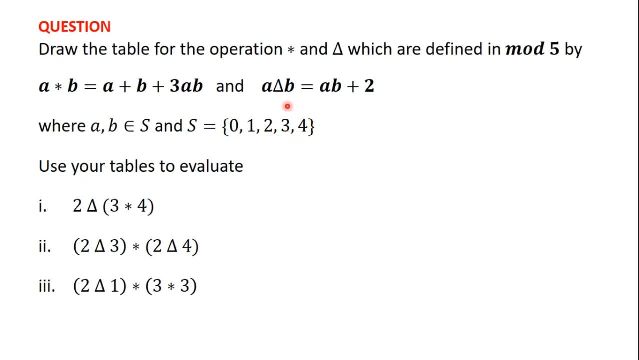 In this video we are going to draw a table for the operation мер ž, which is defined as a star. b is equal to b plus 2 in mode 5 on the set 0, 1, 2, 3, 4.. So we are going. 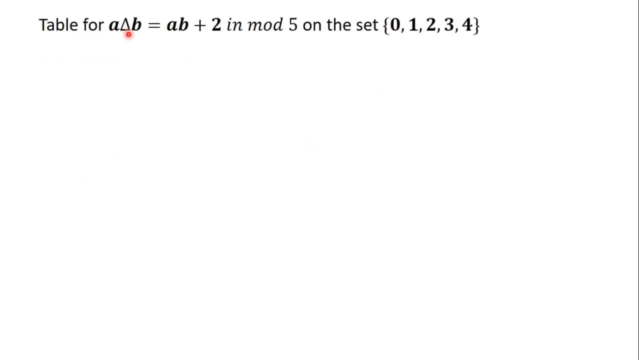 to draw a table for depends which is defined as a star. b is equal to ab plus 2 in mode 5 on the set: 0, 1, 2, 3, 4. 4.. There are 5 values in the set, so we are going to draw a table with 6 columns and 6 rules. 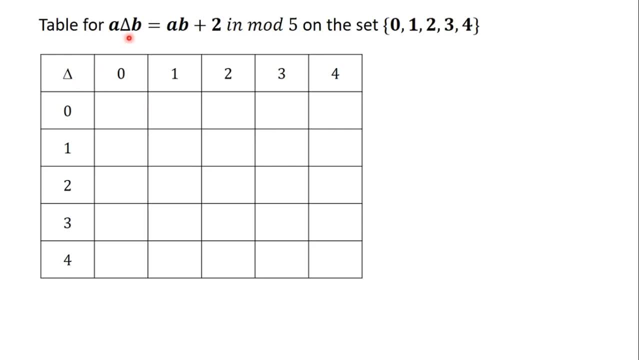 In the first cell you indicate the sign of the operation we are going to perform. The operation is delta, so you indicate delta in the first cell. Then you list the set of values in the first rule and the first column. You have 0, 1,, 2,, 3, 4 and 0, 1,, 2,, 3, 4.. 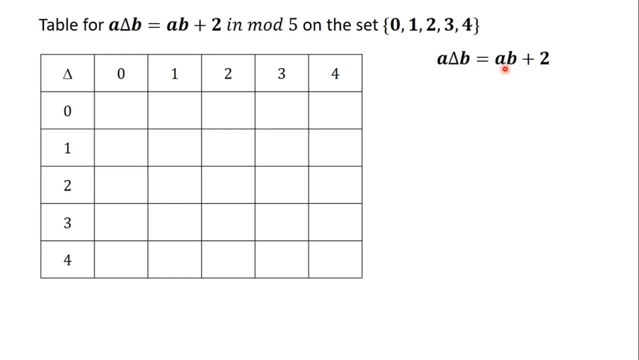 The definition of delta is a delta b is equal to a b plus 2 in mode 5.. Let's fill the table. The first one is 0 delta 0.. a delta b is equal to a b plus 2.. That is, a delta b is equal to a times b plus 2.. 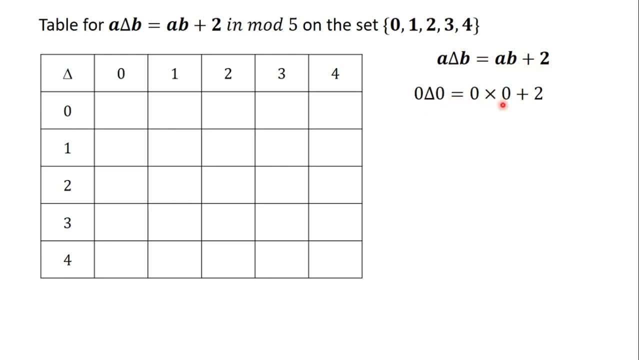 So 0 delta 0 will be equal to 0 times 0 plus 2.. So the first number times the second number plus 2.. 0 delta 0 is equal to 0 times 0 plus 2.. 0 times 0 is 0.. 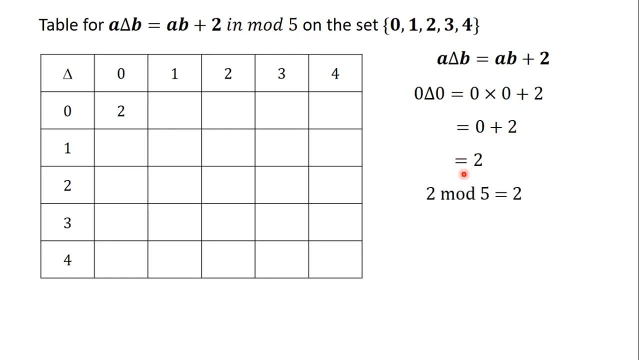 0 plus 2 is 2.. And 2 in mode 5 is 2.. The next one is 0 delta 1.. 0 delta 1 is equal to 0 times 1 plus 2.. This will give us 0 plus 2, and 0 plus 2 will give us 2.. 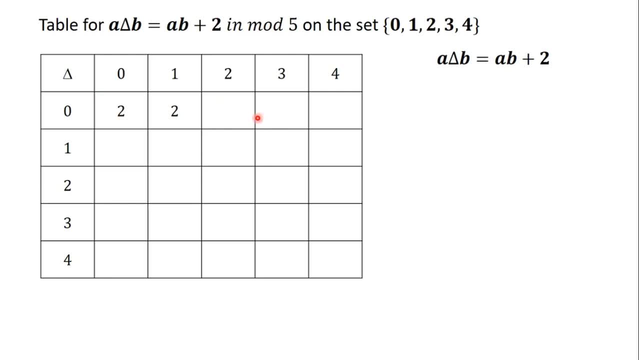 2. mode 5 is 2.. The next one is 0 delta 2.. 0 delta 2 is equal to 0 times 1 plus 2.. This will give us 0 plus 2.. 0 plus 2 is 2.. 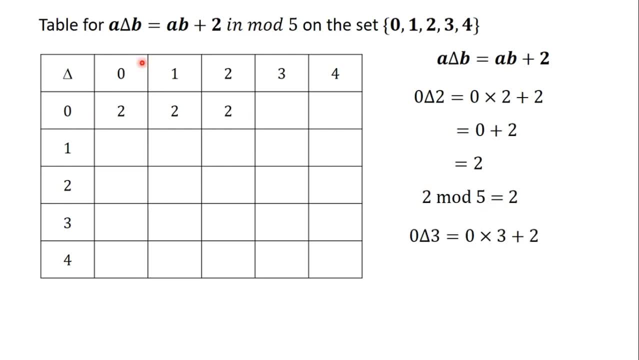 2. mode 5 is 2.. The next one is 0 delta 3.. 0 delta 3 is equal to 0 times 3 plus 2.. 0 times 3 is 0.. 0 plus 2 is 2.. 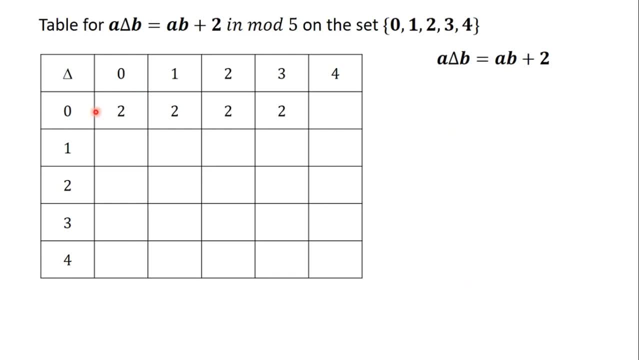 2 mode 5 is 2.. The next one is 0 delta 4.. 0 delta 4 is equal to 0 times 4 plus 2.. 0 times 4 is 2.. zero plus two will give us two. two mod five is two. let's move on to the next rule. you have one delta. 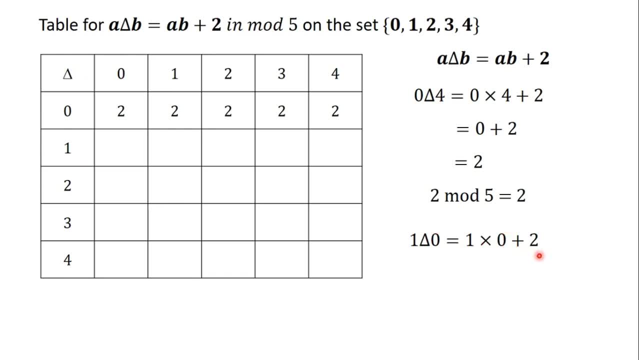 zero. one delta zero is equal to one times zero plus two. this will give us zero plus two, and zero plus two is two. two mod five is two. the next one is one delta one. one delta one is equal to one times one plus two. this will give us one plus two. one plus two is three. three mod five is three. 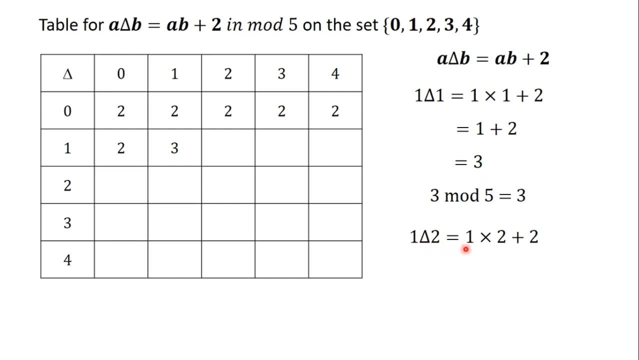 the next one is one delta two. one delta two is equal to one times two plus two. this will give us two plus two. two plus two is four and four mod five is four. the next one is one delta three. one delta three is equal to one times three plus two. 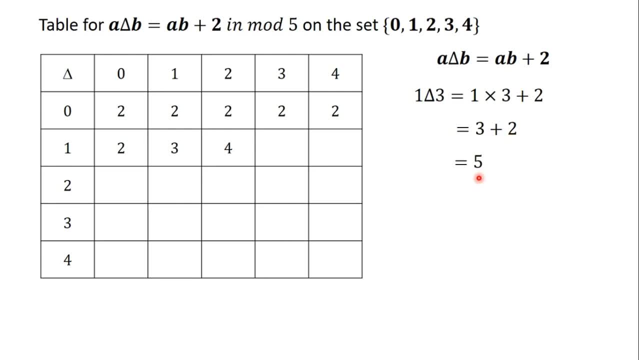 This will give us 3 plus 2.. 3 plus 2 is 5.. 5 multiplied by 5 is 0.. The next one is 1 delta 4.. 1 delta 4 is equal to 1 times 4 plus 2.. 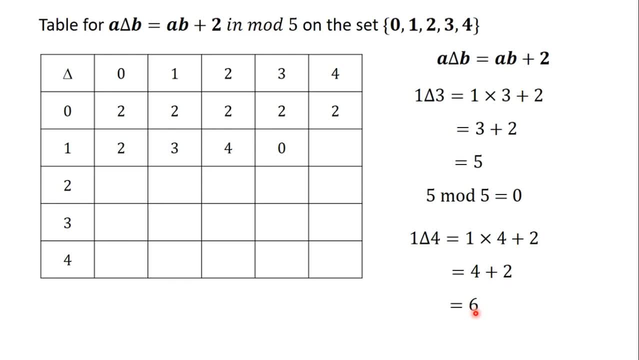 This will give us 4 plus 2.. 4 plus 2 is 6.. 6 multiplied by 5 is 1.. Let's move on to the next rule: 2 delta 0.. 2 delta 0 is equal to 2 times 0 plus 2.. 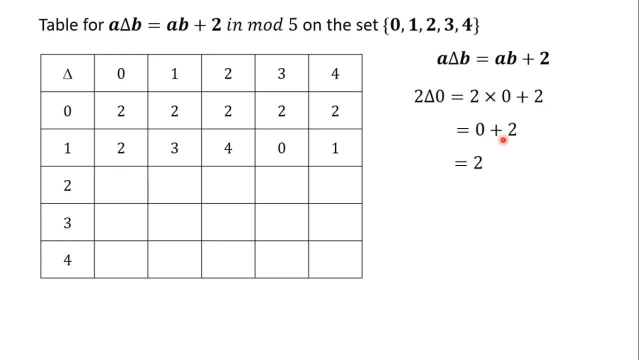 2 times 0 is 0. So you have 0 plus 2.. And 0 plus 2 will give us 2.. 2 multiplied by 5 is 2.. The next one is 2 delta 1.. 2 delta 1 is equal to 2 times 1 plus 2.. 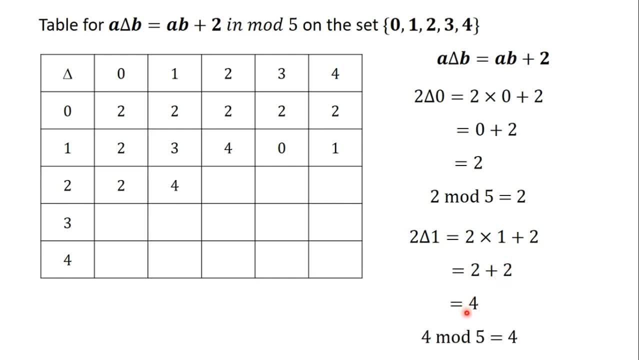 2 times 1 is 2.. 2 plus 2 will give us 4.. 4 multiplied by 5 is 4.. The next one is 2 delta 2.. 2 delta 2 will be equal to 2 times 2 plus 2.. 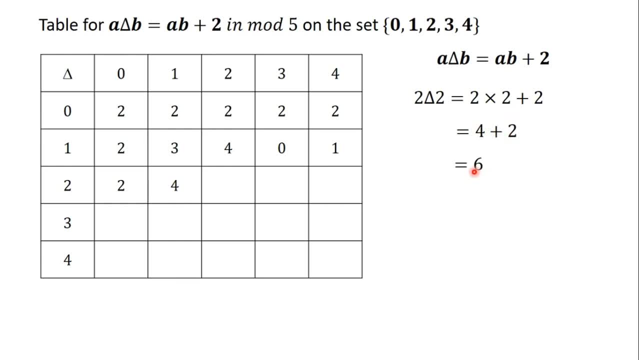 2 times 2 is 2.. 2 times 2 is 2.. So you have 4 plus 2.. 4 plus 2 is 6.. 6 multiplied by 5 is 1.. The next one is 2, delta 3.. 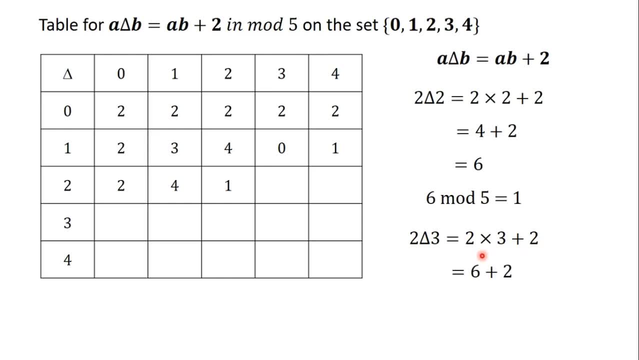 2 delta 3 is equal to 2 times 3 plus 2.. 2 times 3 is 6.. 6 plus 2 is 8.. 8 multiplied by 5 is 3.. The next one is 2 delta 4.. 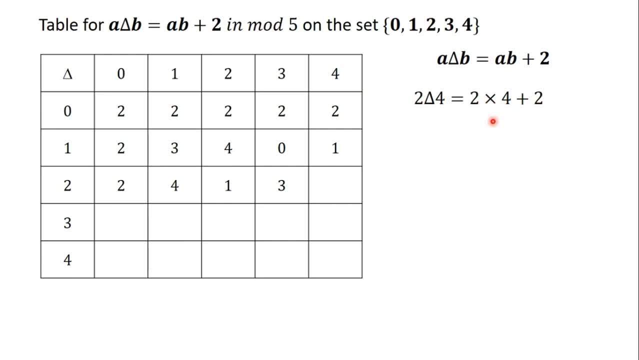 2 delta 4 is equal to 2 times 4 plus 2.. 2 times 4 is 8.. 8 plus 2 is 8.. 8 plus 2 is 10.. 10 multiplied by 5 is 0.. 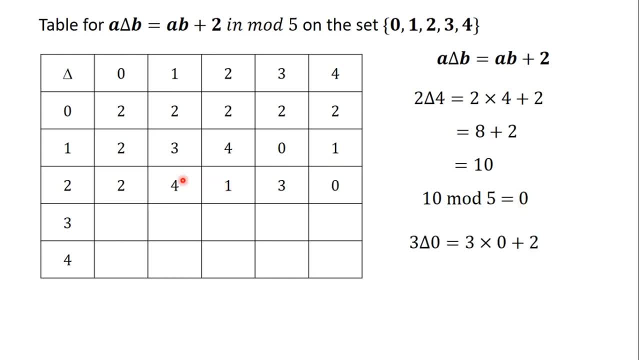 10 multiplied by 5 is 0.. Let's move on to the next rule: 3 delta 0.. 3 delta 0 is equal to 3 times 0 plus 2.. 3 times 0 is 0.. 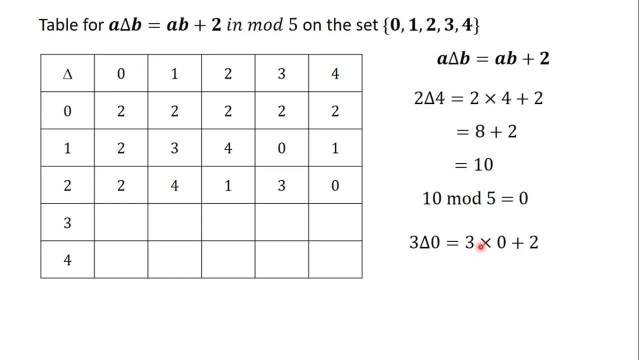 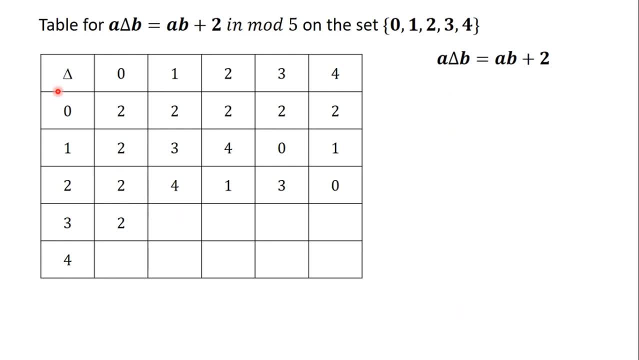 3 times 1 is equal to 3 times 1 plus 2.. The next one is 3 delta 1. 3 delta 1 is equal to 3 times 1 plus 2. 3 times 1 is 3. 3 plus 2 is 5. 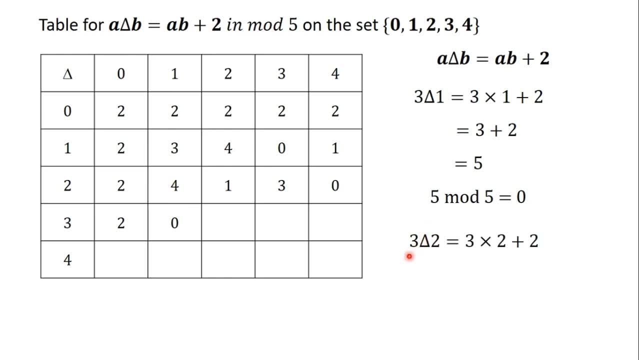 5 plus 5 is 0. The next one is 3 delta 2. 3 delta 2 is equal to 3 times 2 plus 2. 3 times 2 is 6. 6 plus 2 is 8. 8 plus 5 is 3. 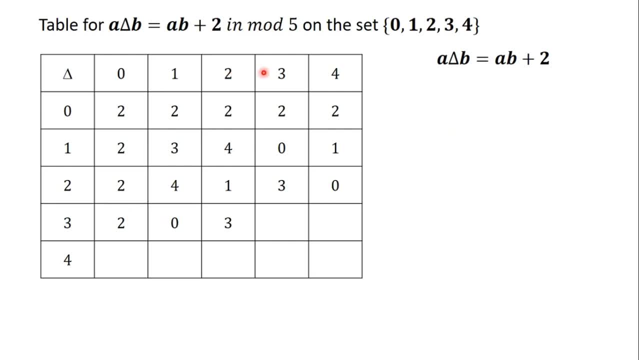 The next one is 3 delta 3. 3 delta 3 is equal to 3 times 3 plus 2. 3 times 3 is 9. 9 plus 2 is 11, 11 plus 5 is 1. The next one is 3 delta 4. 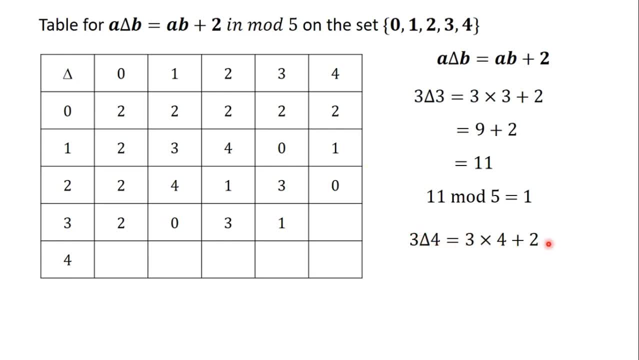 3 delta 4 is equal to 3 times 4 plus 2. 3 times 4 is 12, 12 is 8. 9 plus 2 is 7. 12 plus 2 is 14. 14 plus 5 is 4. 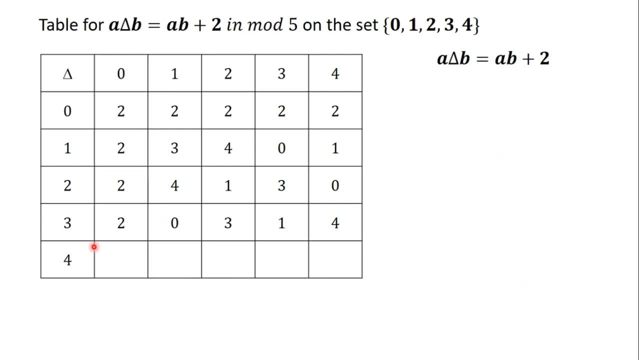 Let's move on to the last rule: 4 delta 0, 4 delta 0 is 4 times 0 plus 2, 4 times 0 is 0, 0 plus 2 is 2 and 2 plus 5 is 2. 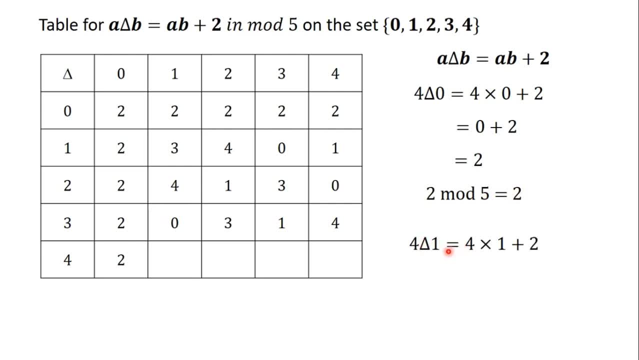 The next one is 4 delta 1. 4 delta 1 is equal to 4 times 1 plus 2. 4 times 1 is 4. 4 times 1 is 2. 4 times 1 is 4. 4 times 1 is 2. 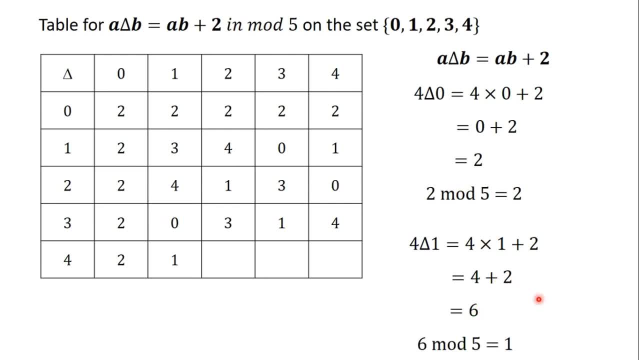 4 times 1 is 4, 4 times 1 is 2, 4 plus 2 is 6 and 6 in mode 5 is 1. The next one is 4 delta 2. 4 delta 2 is equal to 4 times 2 plus 2. 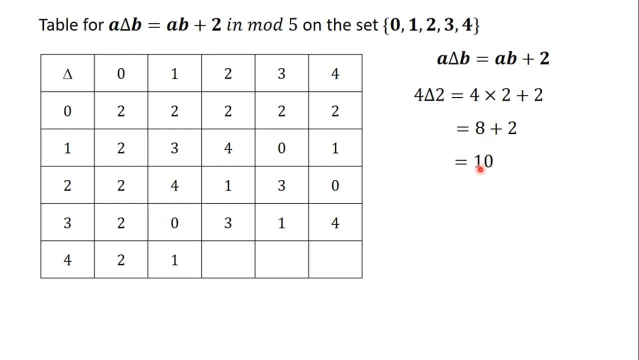 4 times 2 is 8. 8 plus 2 is 10. 10 in mode 5 is 0. The next one is 4 delta 3. 4 delta 3 is equal to 4 times 3 plus 2. 4 times 3 is 12. 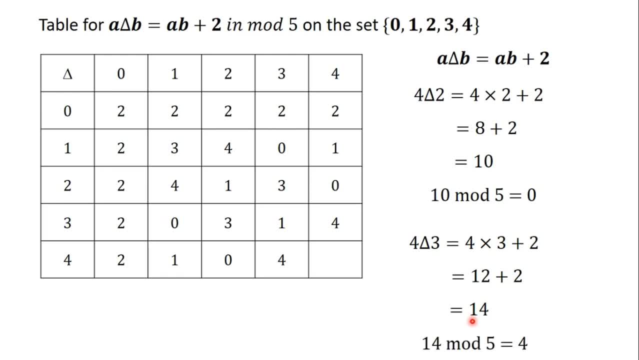 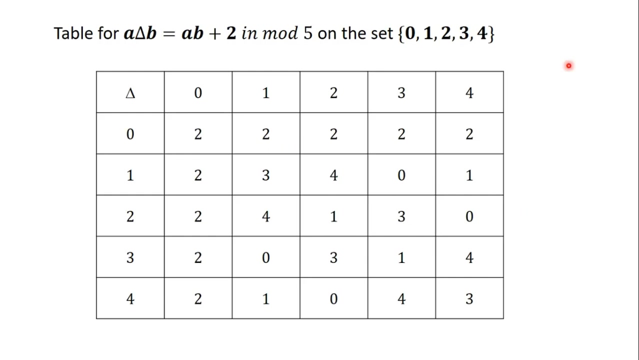 And 12 plus 2 is 14, And 12 plus 2 is 14, 12 plus 2 is 14 and 14 in mode 5 is 4. The last one is 4. delta 4 b is equal to ab plus 2 in mode 5 on the set 0,, 1,, 2,, 3,, 4.. 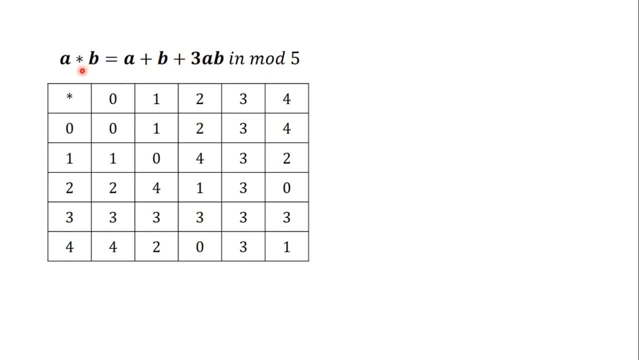 In the previous video we completed the table for star, which is defined as a star. b is equal to a plus b plus 3ab in mode 5 on the set 0,, 1,, 2,, 3, 4.. In this video we have completed the table for delta, which is defined as a delta b is: 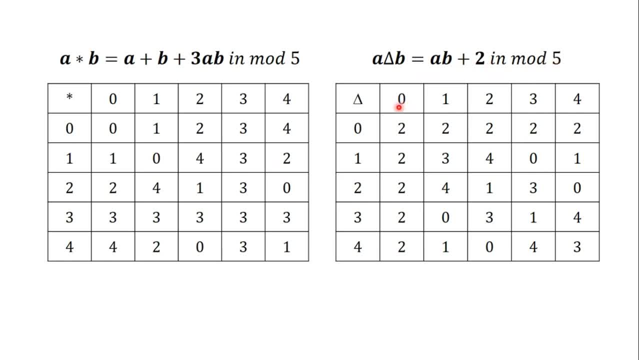 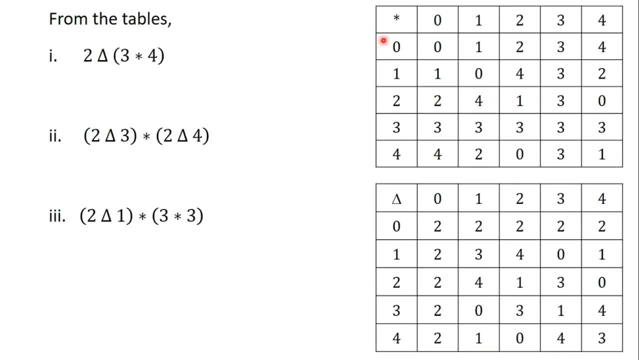 equal to ab plus 2 in mode 5 on the set 0, 1,, 2,, 3, 4.. The question said that we should use our tables for star and delta to evaluate i 2 delta into bracket 3, star 4, ii 2 delta 3 into bracket star. 2 delta 3 into bracket star. 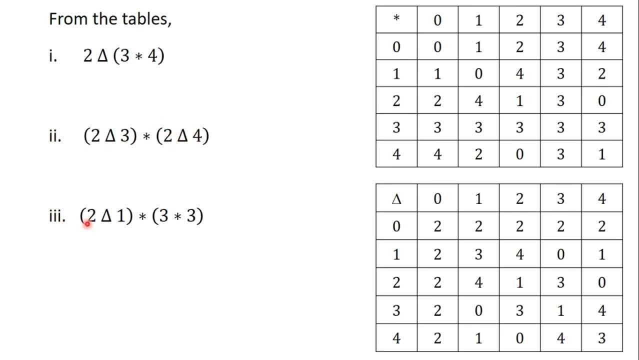 2 delta 4 into bracket iii. 2 delta 1 into bracket. star 3: star 3 into bracket. We will do this in the next video. so see you in the next video and let's continue with the solution. bye, bye. 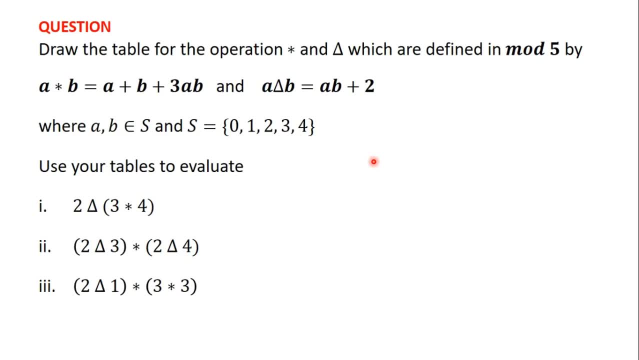 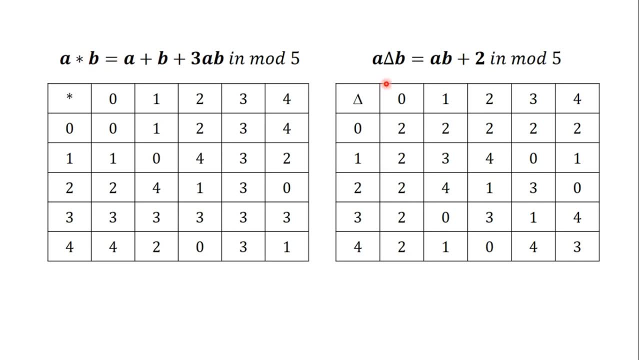 Welcome back. We are still on the solution to this question. We have completed the tables for star and delta in the previous videos. In this video, we have completed the tables for star and delta in the previous videos. In this video we are going to use the tables to evaluate the following. 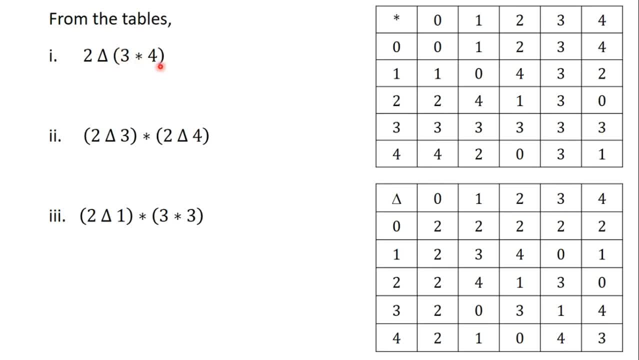 The first one is 2 delta into bracket: 3 star 4.. The second one is 2 delta 3 star, 2 delta 4.. And the last one is 2 delta 1 star, 3 star 3.. Let's begin with the first one: 2 delta into bracket, 3 star 4.. 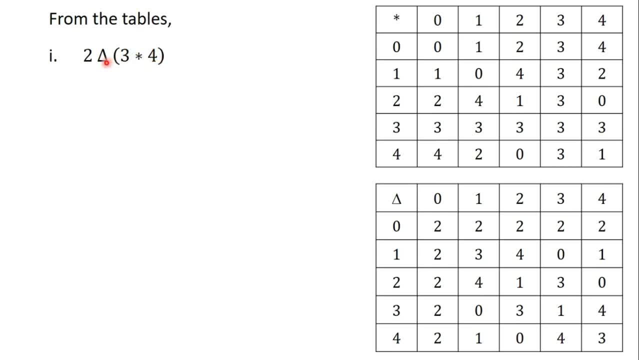 So you will first have to find what is in the bracket. you have 2 delta. then we find what is in the bracket which is 3 star 4. 3 star 4 from the table will give us 3. so you have 2 delta 3. then you read 2 delta 3 from the delta table. you have 2. 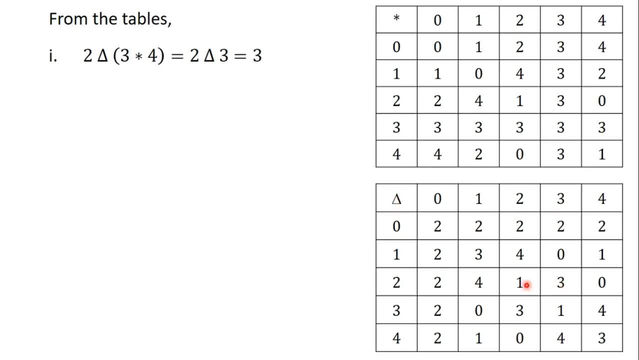 delta 3, which is 3. so from the table 2 delta into bracket 3, star 4 is equal to 2 delta 3, which is equal to 3. the next one is 2 delta 3, star 2 delta 4. so you read what is in the first. 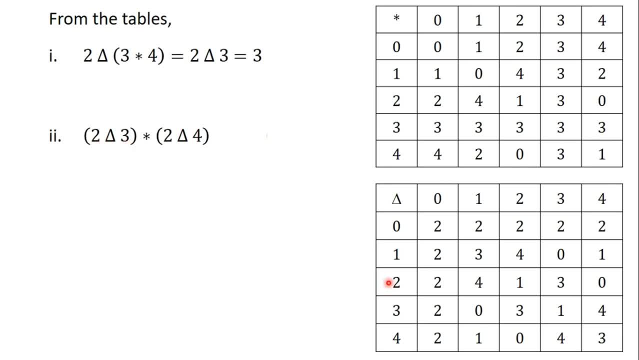 bracket 2 delta 3 from the table. 2 delta 3 will give us 3, so you have 2 delta 3, then star 2 delta 4. 2 delta 4 will give us 0, so 2 delta 3 will give us 3 and 2 delta 4 will give us 0. you will now have to find 3 star 0. 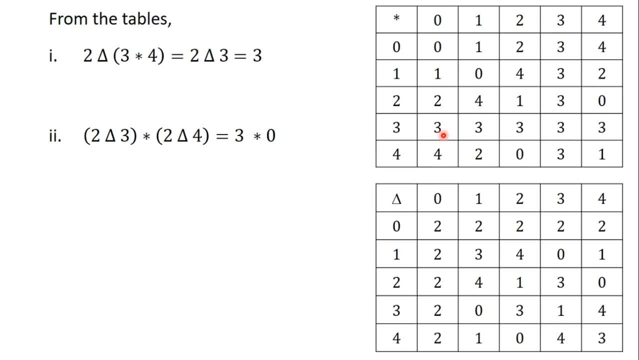 3. star 0 from the table will give us 3, so 2 delta 3. star 2 delta 4 is equal to 3. star 0 from the table will give us 3, so 2 delta 3. star 2 delta 4 is equal to 3. 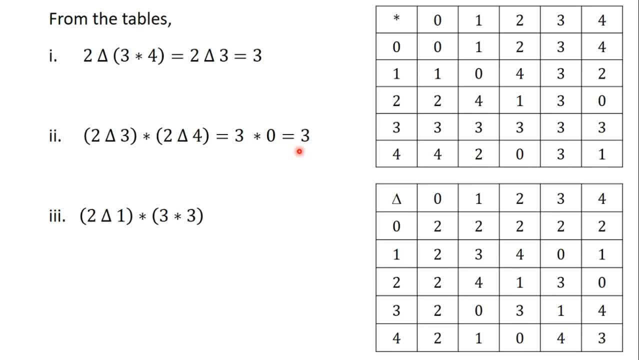 3 star 0 from the table will give us 3. so 2 delta 3 star 2 delta 4 is equal to 3 star 0, which is equal to 3. the last one is 2 Delta 1 star 3 star 3. so you begin. 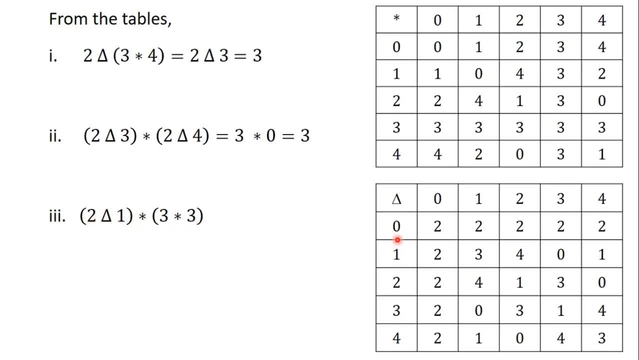 with the first brackets: 2 Delta 1, 2 Delta 1 will give us 4, so we have 4 star. you have to find the second. what is in the second brackets, which is 3 star 3. 3 star 3 will give us 3, so now we have 4 star 3. 4 star 3 from the table will give us 3. 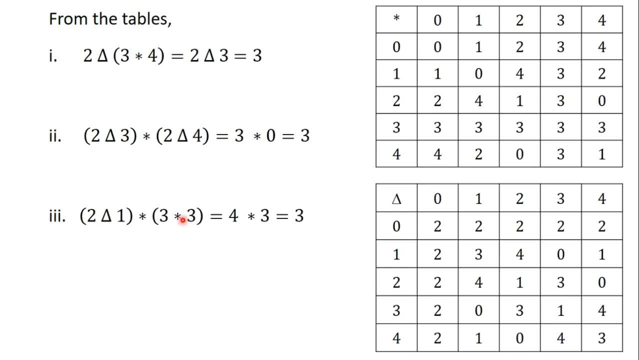 so 2 Delta 1 is 4, 3 star 3 is 3 and 4 star 3 will give us 3. thank you for watching this video. subscribe to this channel for more videos. this is the end of the videos on Moodle arithmetic. pick more examples on your own and try your hands on them, if you.